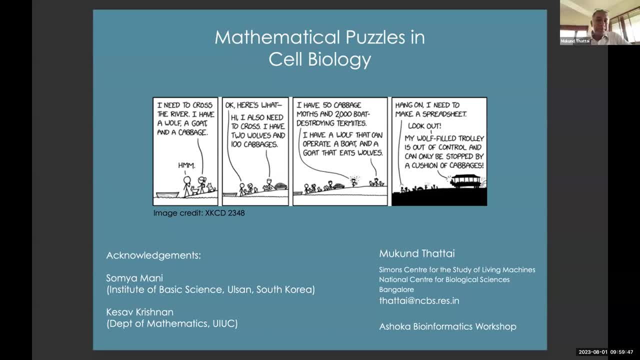 Yes, we can see the pointer. Okay, so here we go. So this is a sort of spoof of these old puzzles that we used to do in in school a long time ago, where you were supposed to cross the river with a wolf, a goat and a cabin. Typically it's a herbivore, a carnivore and and some vegetables. 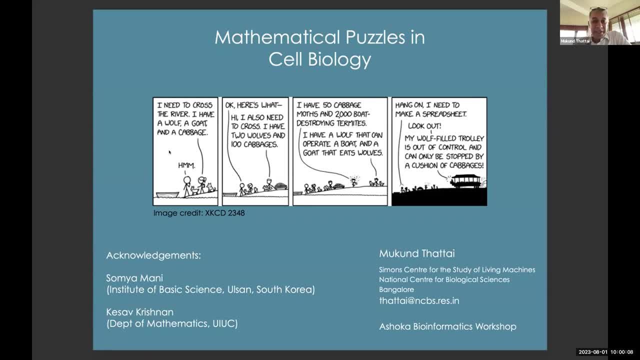 okay, And you have a boat and the boat. Obviously you could, I'll go on the boat, but then the wolf would eat the goat and the goat would eat the cabbage. So you have to somehow go back and forth across this river and make sure that you get everybody. 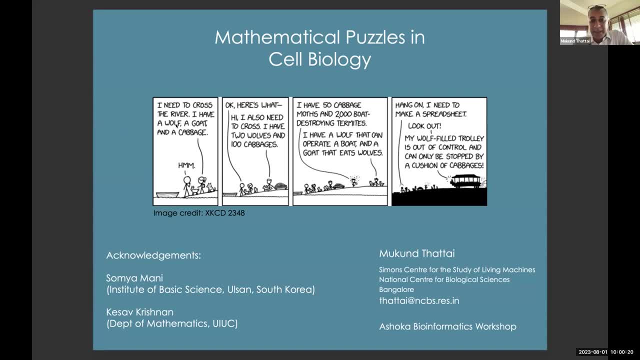 across. So here's the XKCD cartoon. I need to cross the river. I have a wolf, a goat and a cabbage. That's the standard right, And sort of cue ball says, okay, here's what. because he knows. 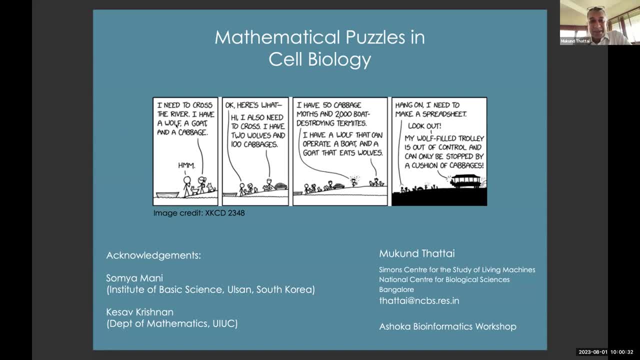 the answer, But then the puzzle gets more complicated. Hi, I also need to cross. I have two wolves and 100 cabbages. I have 50 cabbage moths to 200 boat destroying termites. I have a wolf that can operate a boat and a goat that eats wolves. Hang on, I need to make a. 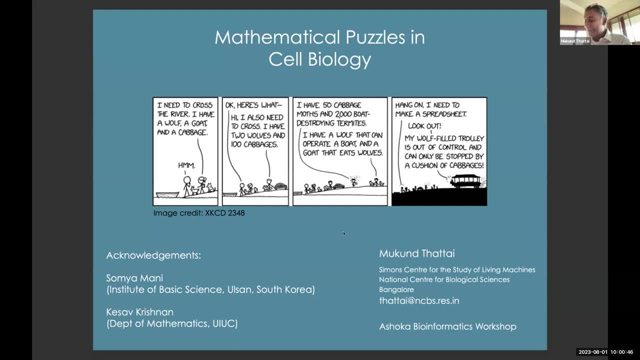 spreadsheet and so on. So so this is actually pretty much a visual abstract of the talk I'm going to give you today And the transport steps we're going to be talking about in our course. a river, but inside a set, And before I start, I should say that this work is done along with a 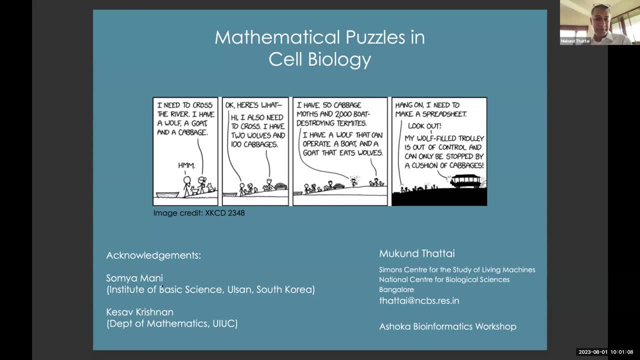 former PhD student of mine, Somya, who is now working in the R&D department at the University of working at the IBS in Korea, and with a collaboration from a math student, Keshav Krishnan, who is now at UIUC, And you can reach me at this email id if you have any questions about. 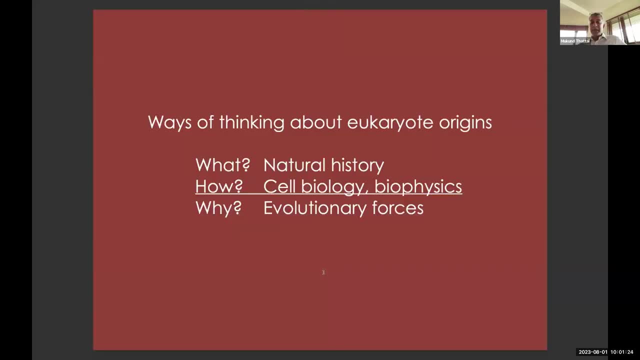 the talk. Okay, so I, as was indicated in the introduction, I think about eukaryotic cells. So eukaryotes, you all know, are cells like ours, or like plants, or single cell microbes like amoeba and ciliates and yeast, and so on. There's a huge diversity of eukaryotes. 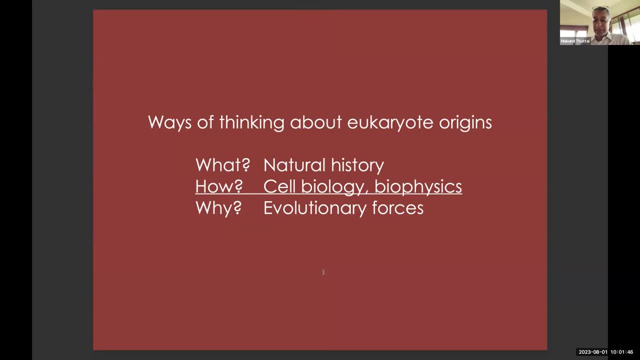 and people are really not aware of. you know, the textbooks don't give the right impression about how broad this group is And, yes, they all have some characteristics, which is they have a nucleus, but there's many other things that they share And, of course, there's many other things that 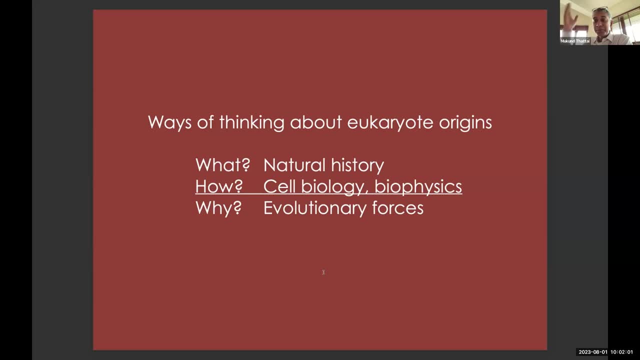 are different across all these different lineages of eukaryotes. So I like to think about this entire tapestry of eukaryotic diversity which is, you know, falls under this rubric of natural history. What are the cells that are? 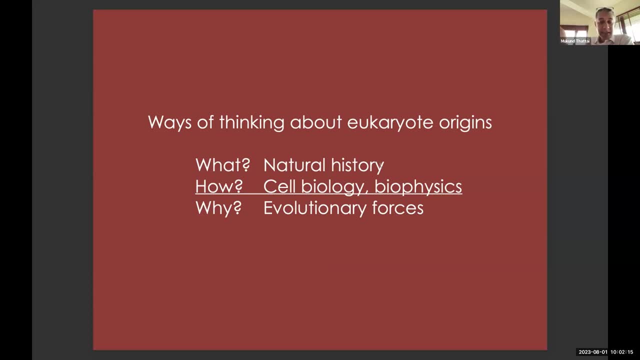 alive today And how are they related to cells that existed in the past? And we use bioinformatic approaches- phylogenetics, genomics, a lot of protein sequence reconstruction and so on- to do that, And I had initially thought to give a talk about that, since this was a bioinformatics. 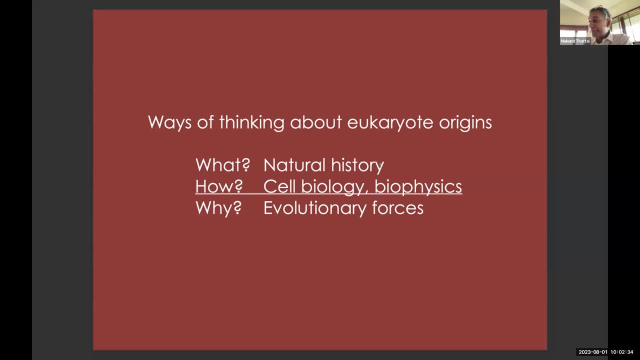 workshop, but then I decided to do something a little more different. a little more different so that you would learn something about it. So I'm going to start with the bioinformatics workshop. So I'm a physicist and as a physicist, we like to think about how interactions between 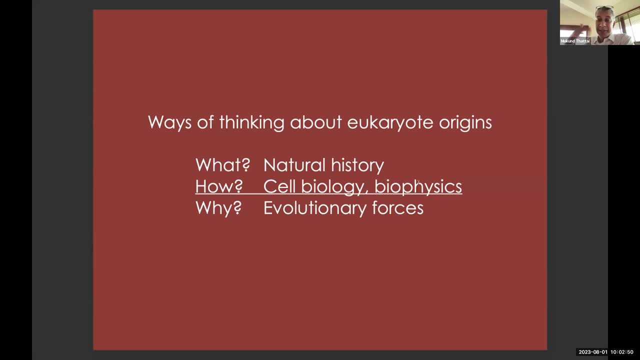 small components can lead to large emergent patterns and phenomena dynamics. So the question we ask is: you know, how do known molecular interactions between things that happen inside a cell set up the architecture, the fairly sophisticated architecture of a standard eukaryotic cell, And I'll show you some pictures to see just how complicated 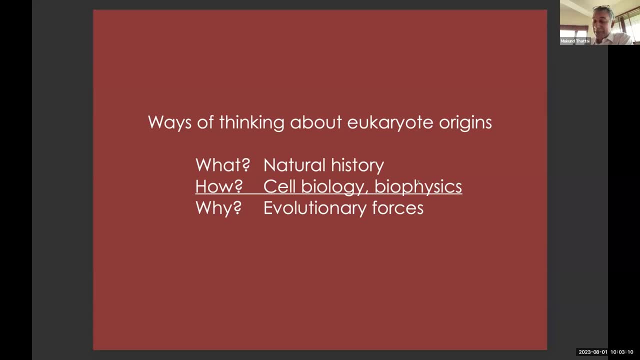 that beast is. And the third is actually a very difficult question. It's the why question, in the sense: what are the selective pressures, the evolutionary forces that happened over a very long time span that led to the present day cell and present day diversity? 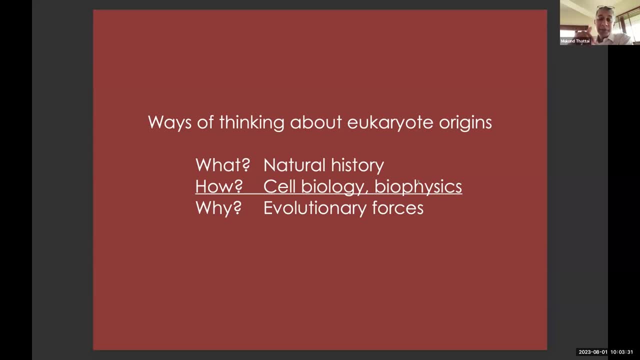 of different cell types. So again, the three categories are: what natural history? how, how do molecules conspire to generate these patterns, and why? what exactly was the selection pressure that led to the present day? And of course we don't have answers to. we have hardly any. we've only scratched the surface about this. 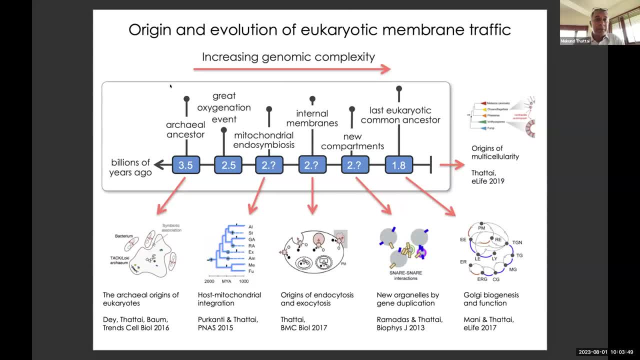 So here's a broad overview of what I'm talking about. This timeline that you see in the box starts from the present day and sort of goes back in time over billions of years. So you started about three and a half billion years ago. be slightly closer to the present, but around that. 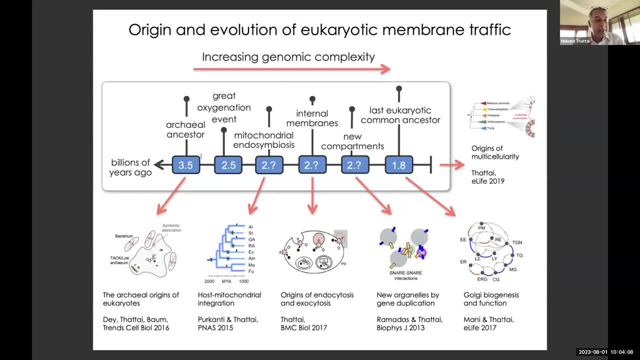 time is when you have some evidence that there were already cellular structures and fossils that you find, And so the idea is that some sort of prokaryotic ancestor already existed at that time. Now, on present day earth, there are two kinds of prokaryotes. These are organisms without nuclei. 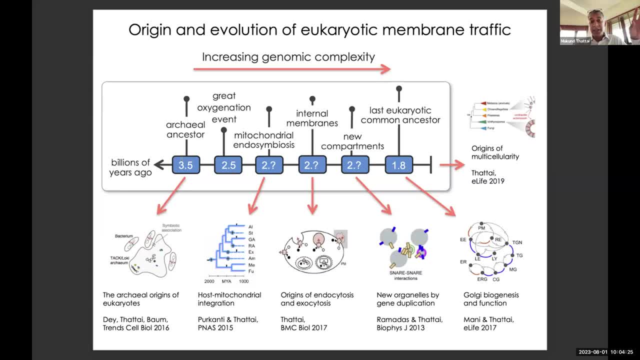 but they're very different from eukaryotes and they're very different from each other. They're as different from each other as we are from them, And they're called archaea and bacteria. They're both called prokaryotes, but you should really keep in mind that it's bacteria and archaea and these are two. 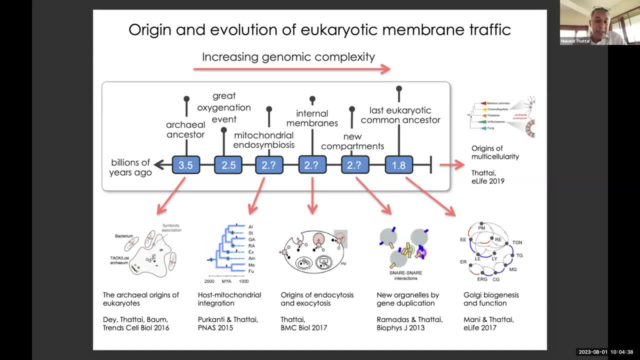 major kingdoms of life on earth that are still existing. At some point around two and a half billion years ago, the evidence of mineralization and oxidation states in rocks indicate that there was an increase in oxygen availability, which eventually actually changes the atmosphere of the earth. And so this is, you know, an example of a great episode of climate change, if you want. 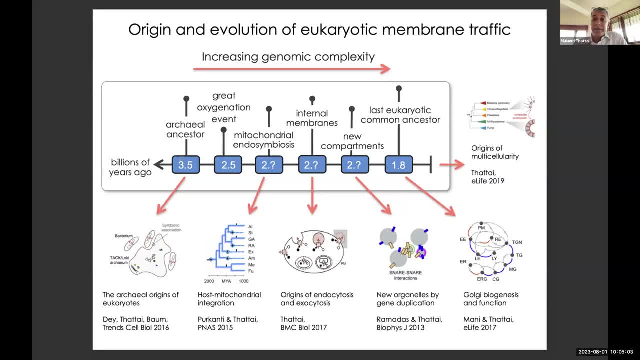 to think of it that way, And the reason it happens is because of the invention of photosynthesis, So prior to this date, life exists and extracts energy based on chemical gradients. You want to think about, for example, hot springs, deep sea vents and things like that, where there's a lot of 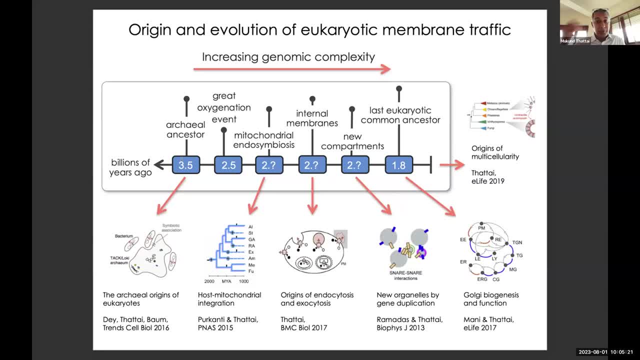 temperature. there's a lot of chemistry that the cell can make use of to survive, But with the invention of photosynthesis, then what you do is you directly take the heat from the sun, you take the light from the sun and you take CO2 from the air and you make sugars. 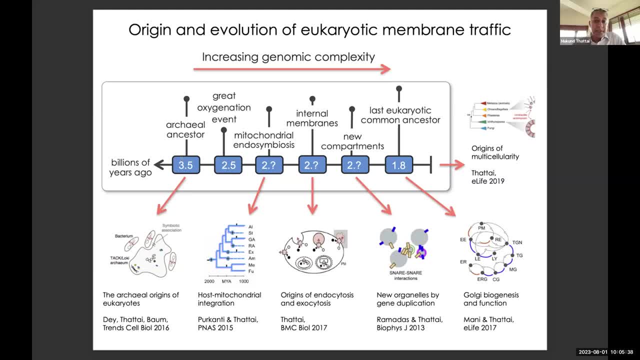 which you can then use as a fuel to run all your other cellular processes And you can make ATP, for example, And this leads to a byproduct oxygen which floods the atmosphere and then leads to a niche for a new type of organism, which is a respiratory one. So the invention of 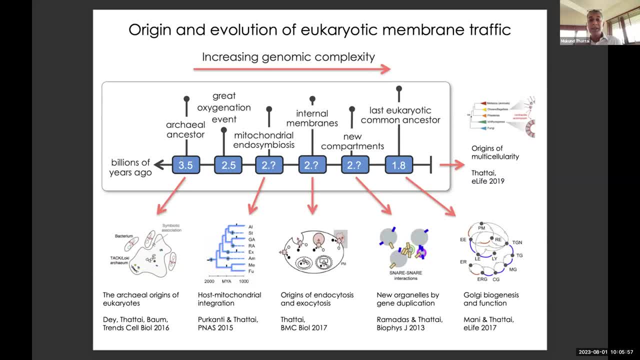 oxidative respiration, the use of oxygen to more efficiently utilize carbon sources comes into being And again, these are all prokaryotes that do this. it's a. it's a prokaryotic world at some point about, uh, two billion years ago, maybe 1.5 billion. 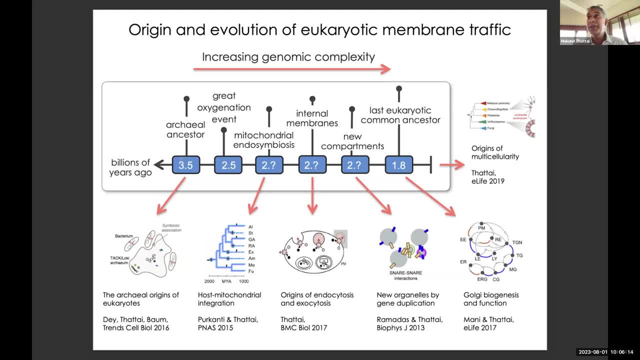 years ago. there's um a strange uh niche again somewhere in the earth, perhaps in the north sea, um, which is where present-day uh lineages that represent that ancestral state seem to have been discovered, where a group of archaea which are presently called the loki archaeota or the, or the 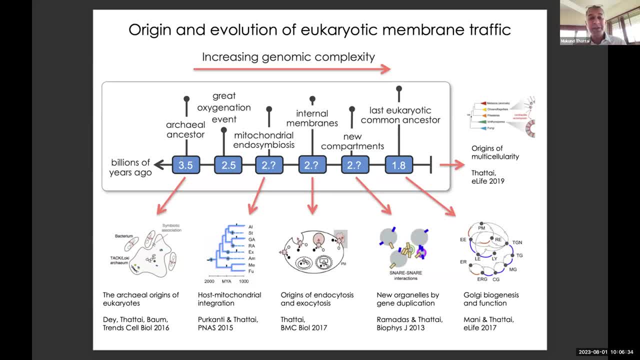 what is the new word? they're all named after norse gods. okay, so there's this, this big clade of archaea which tend to live today in symbiosis with bacteria. they are, um, they're studded with bacteria on the surface and they do gas exchange, and this is how they actually survive. they. 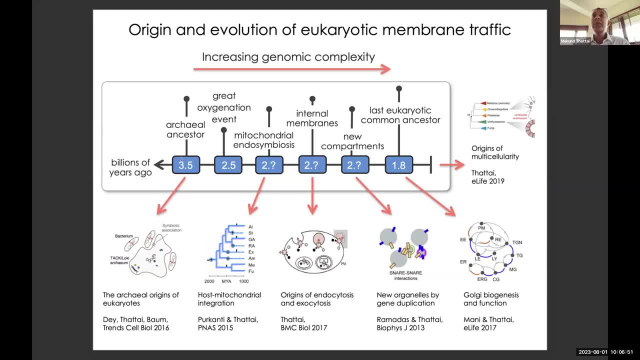 there's a symbiotic relationship. one of those, um- oh yeah, they're called the asgard super phylum, so one of those ends up, um, entering into a very tight symbiotic relationship, so tight that the bacterial partner ends up living inside the archaeal partner, and this is the, the first proto-eukaryote, the bacterium over there is actually what we see as 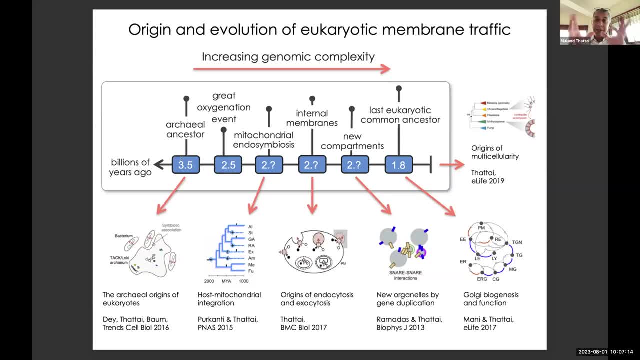 the mitochondria. today it continues to do oxidative respiration. the archaeon provides the, the host environment, the cytoplasm um and all the transcriptional and translational dna replication machinery, while the bacterium provides the metabolism. so that's the um, it's not, you know. 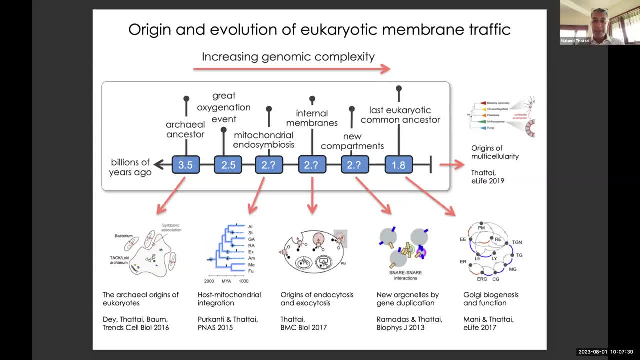 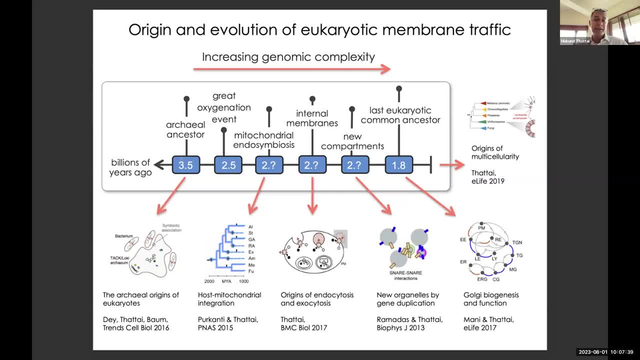 were living together, uh, ended up cementing this symbiosis. so i'm interested in the period after that point. uh, so what happens is eukaryotes then develop what we think of as the standard eukaryotic traits, not just the nucleus, but also these internal organelles, the er, the golgi. 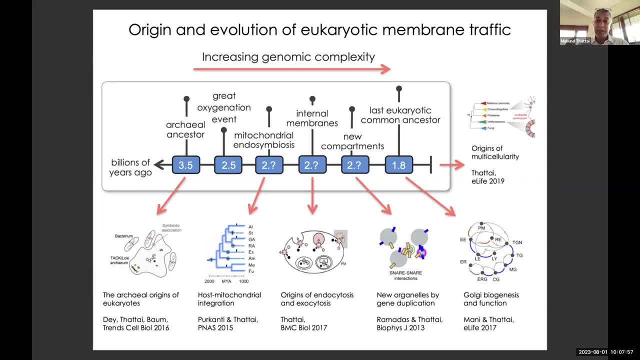 endosomes and so on, cytoskeleton, the actin and tubulin cytoskeleton, um uh, changes of shape, sexual reproduction, mitosis, meiosis, all this stuff that eukaryotes invent happens after that stage. um, and then we reach this point called the last eukaryotic common ancestor leaka, about 1.8. 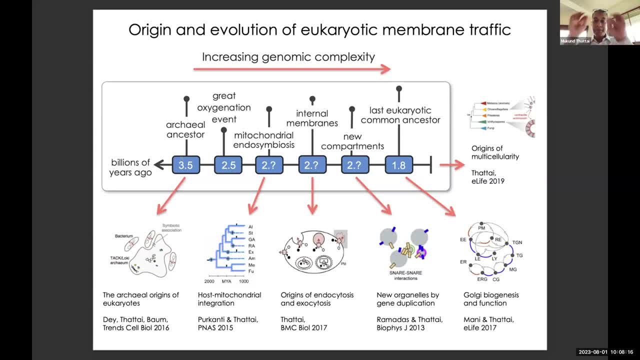 billion years ago or slightly more recently, um, and that organism is called the last eukaryotic common ancestor because if you trace back all the existing eukaryotic lineages, uh, that's the most recent ancestor. that's common to all these. it doesn't mean it was the first eukaryote, in fact. 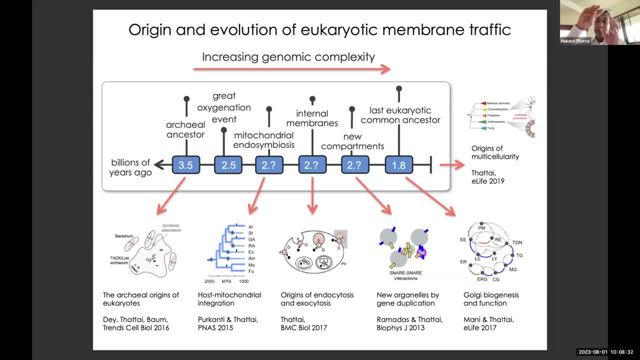 it's much more recent than the first eukaryote and it's not the first eukaryote. it's the first eukaryote. it's just that there are no descendants of those first organisms left today. okay, so i haven't given you that uh overview of the timeline. um, i'll just tell you some of the work we've done across the. 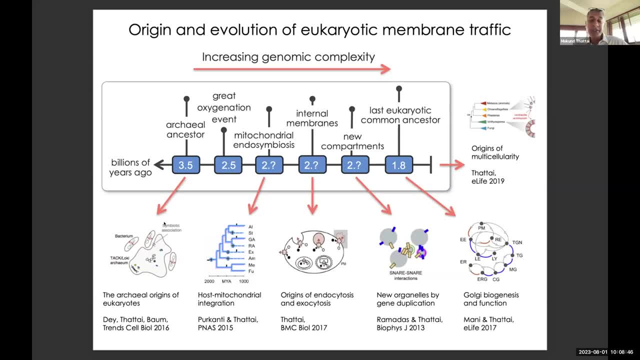 spectrum. so we've worked on these archaeal origins by using bioinformatic tools, using present-day archaeal genomes to see what fraction of eukaryotic genomes are made from archaeal components and what fraction from bacterial. we've looked at the integration of the bacterium with the host to 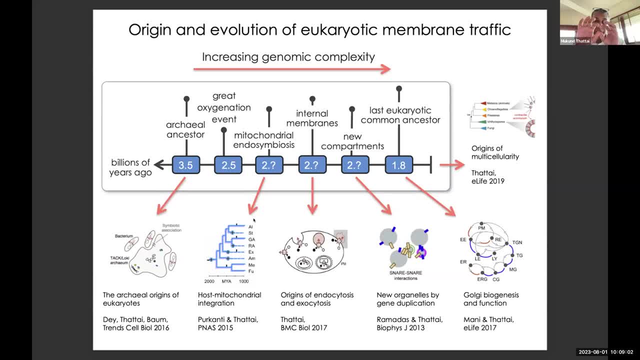 become mitochondria. in particular, we've looked at the mitochondrial division machinery. mitochondria actually divide inside the host, almost as if they were free-living organisms. they have their own genomes, as you know. we've looked at the origin of endocytosis and more recently we've started thinking about how new compartments, not just the first in the 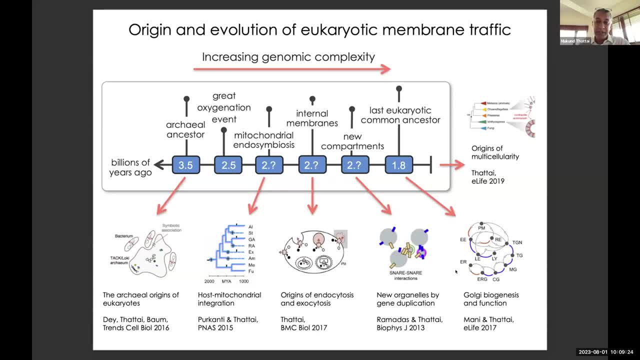 first proteocaryote, but this whole full-blown apparatus of er, golgi, secretory vesicles, endocytic endosomes, lysosomes, all those things came into being. the golgi has been a particular favorite organelle of mine and, uh, touching upon multicellularity, but it's not something i'm going to talk about today. 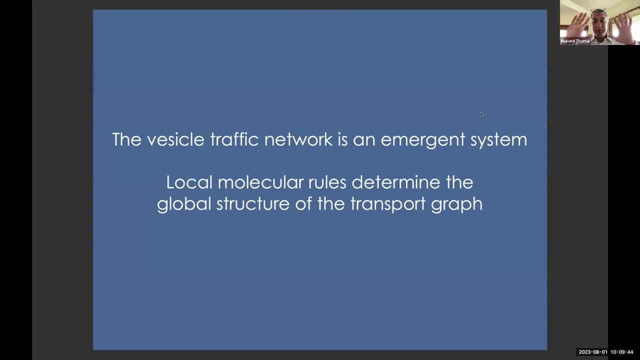 okay. so, having given you the, the, the natural history, um, let's look at the second part of what we work on, which is the how? how do local molecular rules, small microscopic interactions give rise to the sort of cellular state? so somehow, um, we need to provide a theory for this right. it's not enough just to hand wave. 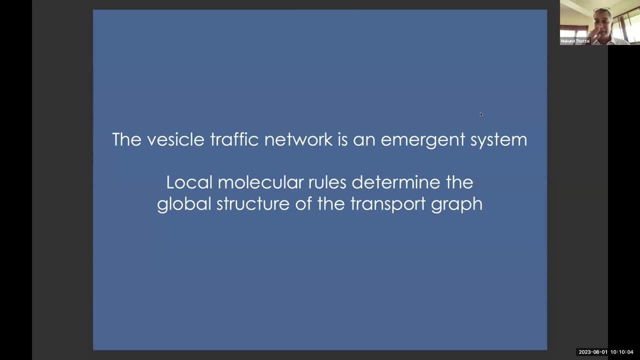 say, we know what these molecules do and we know what the cell looks like and there's a causal relationship. often when you do genetics, uh, you knock out a molecule, a snare, protein or an r for whatever it is, and you get this very big phenotype. the whole organism has a big change and if it's an 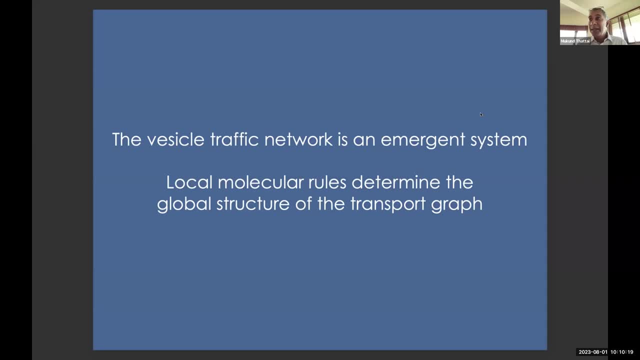 animal. you see a macroscopic change just by eye. that doesn't mean that the role of that molecule is to make that whole process right. that molecule is working as part of a system and when you break the molecule, break the system and then of course the the consequences of that can be very huge. 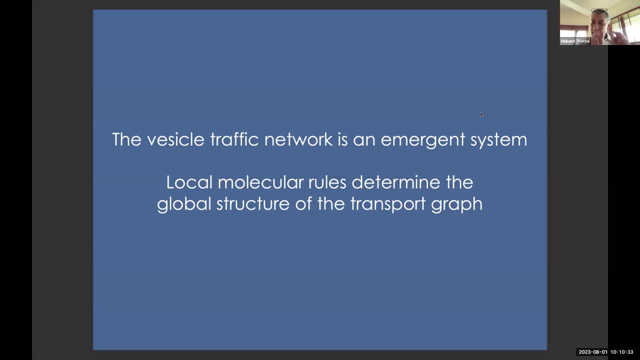 but the actual effect of the molecule is very local, which then has secondary consequences. tertiary, and it spreads through the system. so you want to build a theory that's able to take this local perturbation and connect it to something macroscopic. and so what i'm going to be? 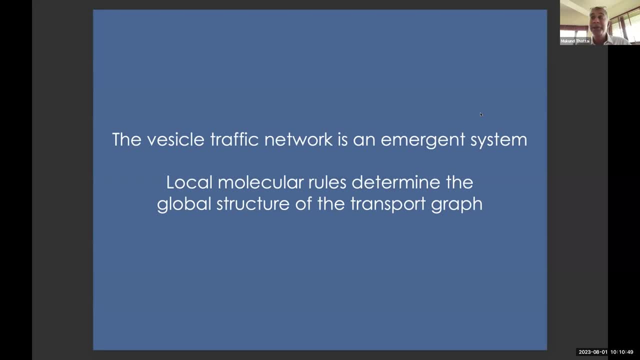 describing to you today is an example of such a theory. there are, of course, many ways to do modeling, and i could give i could teach an entire semester class on how you build a mathematical model and how you build a mathematical model. and how you build a mathematical model and how you. 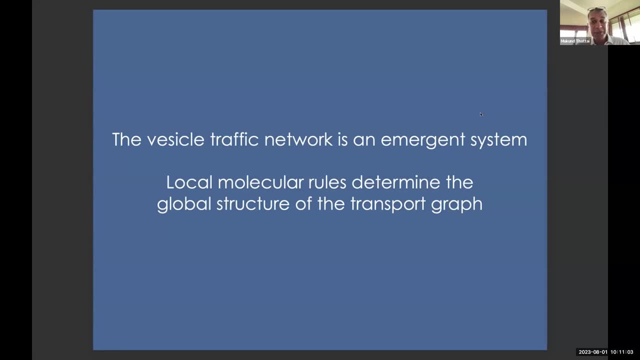 build a mathematical model of a system: how much to leave in, how much detail to leave out, how many approximations you need to make, and so on. but what i'm going to give you is an example of a theory that actually goes from micro to macro, and today's example actually in a sense. 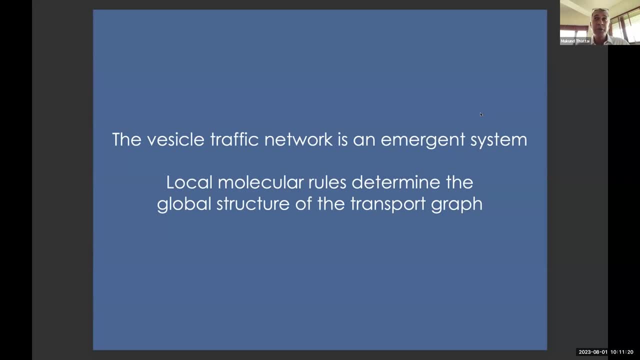 is unusual because, unlike typical models, where you make the model and you see what it does, in this case we've made the model and we can fully understand what it does. so in that sense, it's not just a model, but it's also a theory. and, if we want, during the question and answer session after the talk, 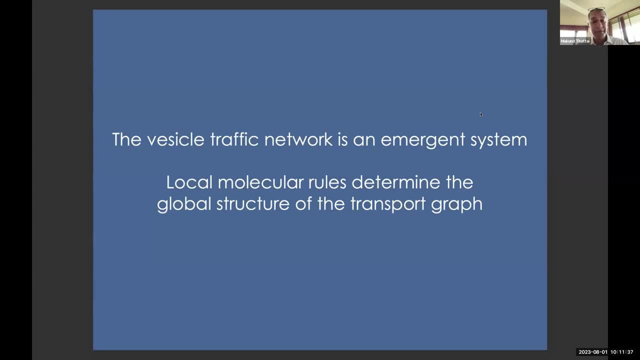 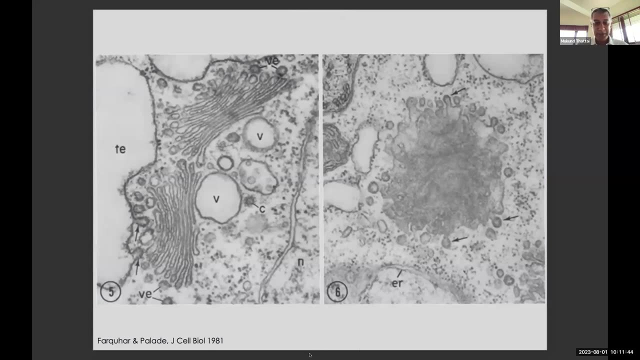 we can understand the difference between models and theories in that sense. so i'm going to pause, just check if there are any questions and, if not, take a few seconds. okay, i don't see any hands up, okay, so let's keep going. so this is a beautiful um em if you actually look at the ems. uh, from um. 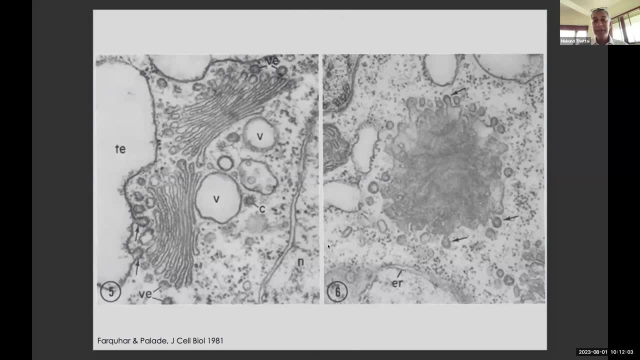 the 70s and 80s. they really are, um, in many ways more detailed, more informative than what people look at today, because at that time people were interested in exploring the structure of a cell in an open-ended way, whereas typically today you use em as a way to look at some particular. 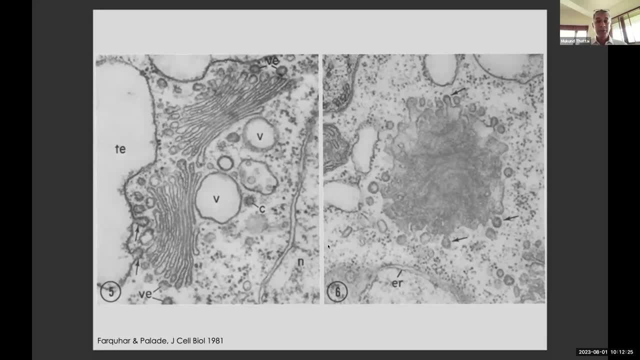 subsystem of interest to you, and so you, so you. you tend to lose the idea of the, the whole cell, as a single entity. but uh, so here's uh palade's very, very beautiful ems. this is a typical eukaryotic cell, um, and when i say typical eukaryote, you know when you read a textbook it there's a book for. 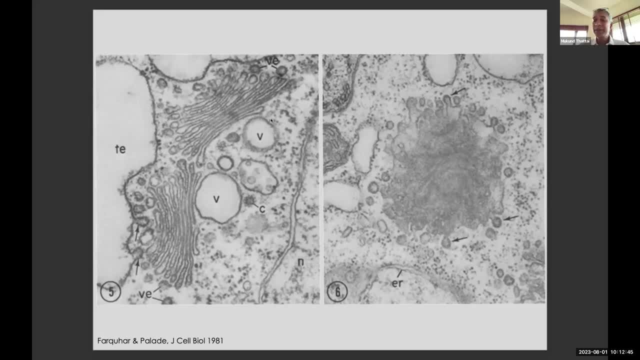 example called molecular biology of the cell, and immediately you should ask in which cell and when. you read that book, mainly they talk about eukaryotes. okay, fair enough, but i already told you there's so many different kinds of eukaryotes, right? so you should say which eukaryote which. 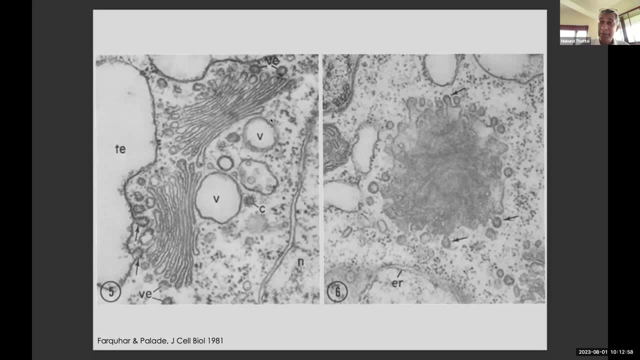 cell um? is it in a multicellular organism? if it is, then which cell type in the multicellular? and so you should never take anybody seriously when they say they make a claim that cells do this unless they have some proof, which is that they've looked at lots of different cells and they all do. 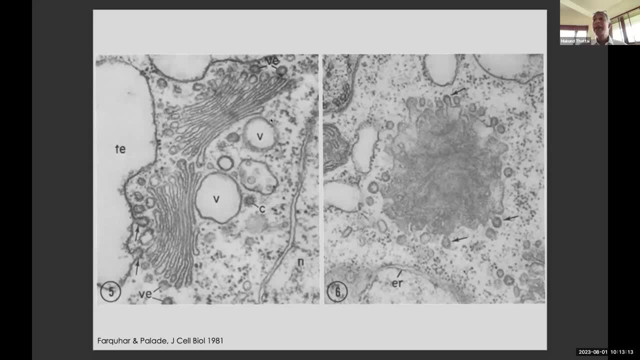 this now the features that you see in the cells i'm showing you here. every eukaryote has them. they have a nucleus, which is not shown over here. they have an endoplasmic reticulum started with ribosomes, as you can see. they have these vacuoles. they have these small transport vesicles which you 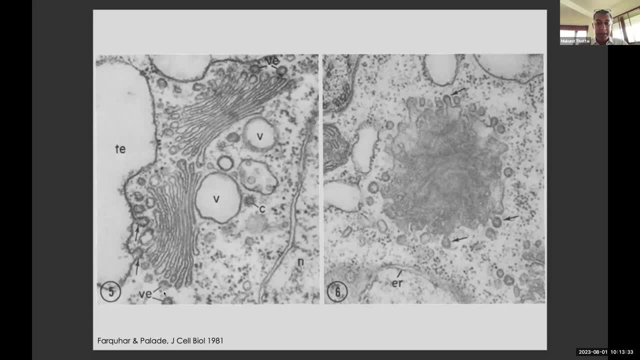 see them beautifully budding out from some source, compartment um, and then they have all eukaryotes also have this structure. it may not always look like this, but it's called the Golgi apparatus, okay. so I mean, this is just a little slice of a cell and you can see how much is going on, right? 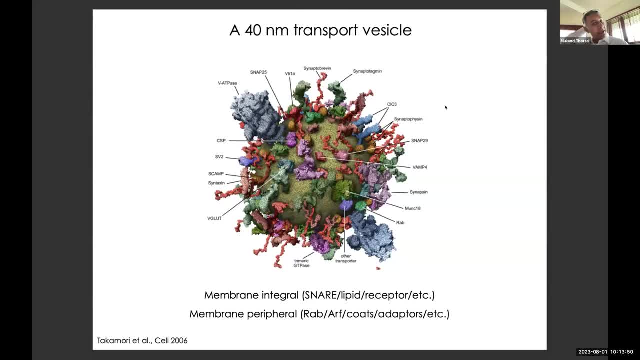 now let's zoom in on that vesicle which I showed you. it's just 40 nanometers- 40, 50 nanometers. this sort of greenish, yellow color on the inside is a lipid bilayer. so this vesicle is a hollow ball and on the inside it will contain all kinds of chemicals and on its surface it has these: 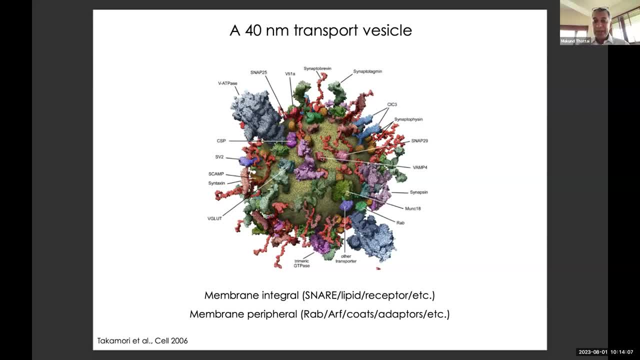 transmembrane proteins, lots of them, and membrane associated proteins, and every single vesicle will be covered with a lot of different proteins. some important ones that will come up later are these snaps and the synaptotagments and so on. these are called snare proteins, which will come up. 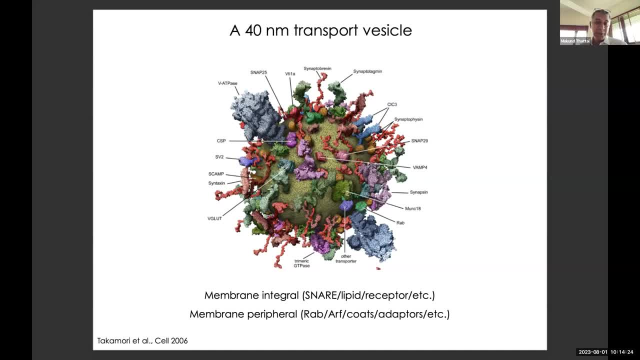 later in the talk. now, the point about this is first to show, yes, it's complicated, um, but also that, uh, there's some reason why these transport vesicles have so much decoration on the surface, and the reason is because these are almost like a, like an Amazon package, right? so if you pick up an 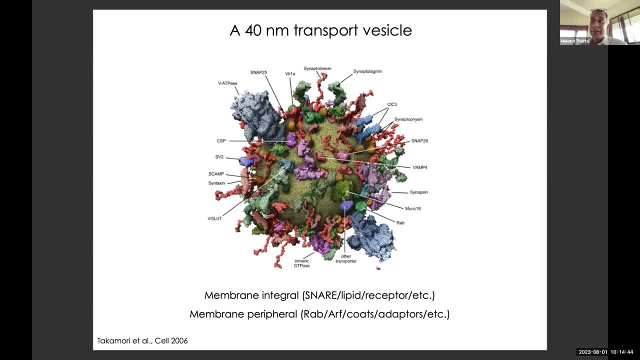 Amazon package anywhere in its delivery process, you'll find that it has a QR code or some other kind of barcode that digitally will tell you where it came from, where it's going, and therefore anybody locally can pick it up and make sure it gets to the correct destination next. so the just like the 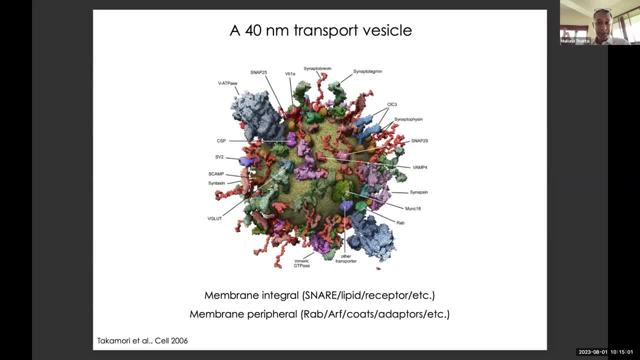 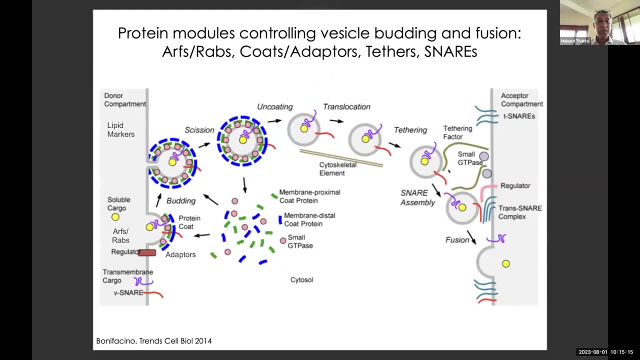 package itself contains its identity and contains its instructions. the vesicle itself contains its own instructions. so, no matter where the vesicle was made, as long as you've made it correctly, it's going to go to the right place, and I'll show you a little bit more what I mean by: uh, go to the right place. okay, so 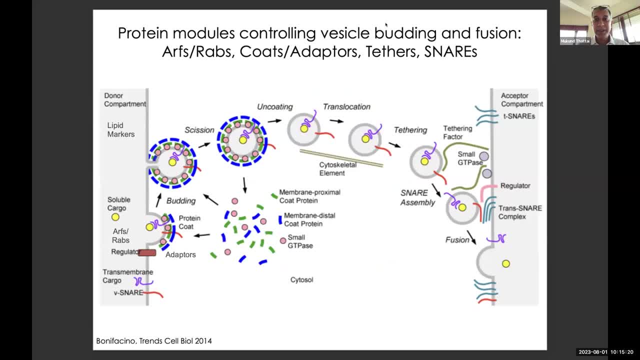 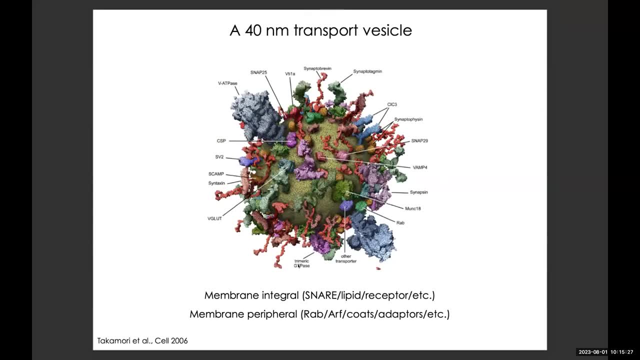 eukaryotic cell has many compartments. these are all different. uh, there's a hand up. yeah, I'll take a question. I had a quick question uh. so, uh, you know, to kind of follow up on the all package analogy, so if, like a you know, like uh, there's like a cell lineage right, like uh, 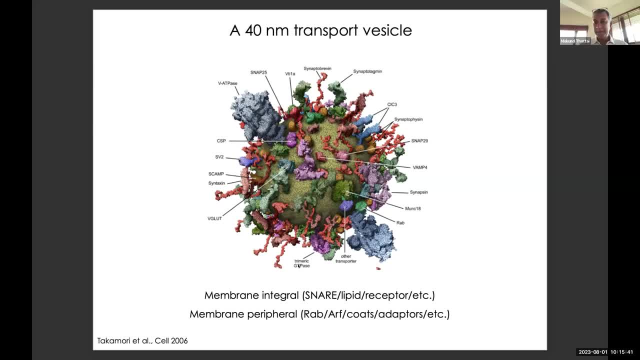 especially in the immune system, right, they differentiate and uh, so I was wondering, can you also find out where it is in its differentiation timeline? right, I think can you find out where the cell is? but this is not a cell, this is a vesicle inside a cell. 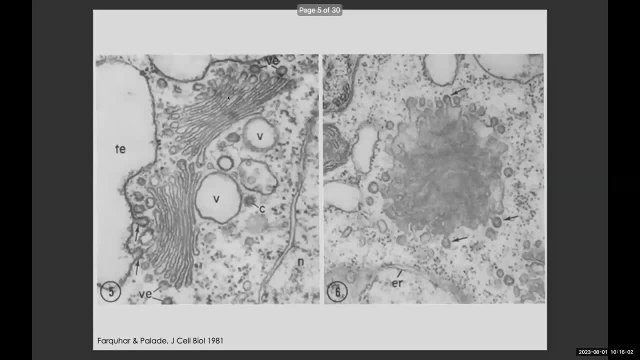 okay, right, the cell is huge, the vesicle is tiny, it's just 40 nanometers- and these vesicles will be pretty much the same, no matter which cell you're looking. they'll have slightly different, slight differences in composition, but you know, they're remarkably similar between between humans. 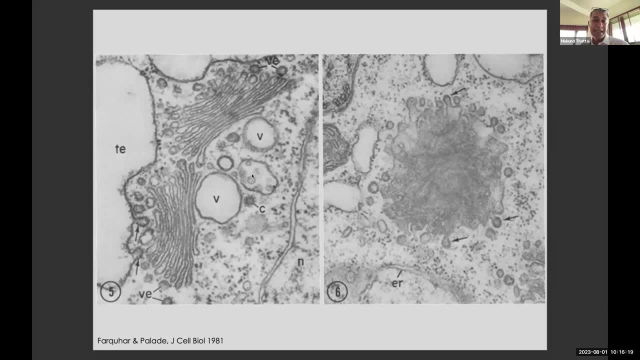 and ciliates and plants and yeast and so on. so these these are absolutely standard across all eukaryotes, so the question of minor differences in different human cells almost doesn't even matter. i'm talking about things that are conserved between animals and plants and and everything. 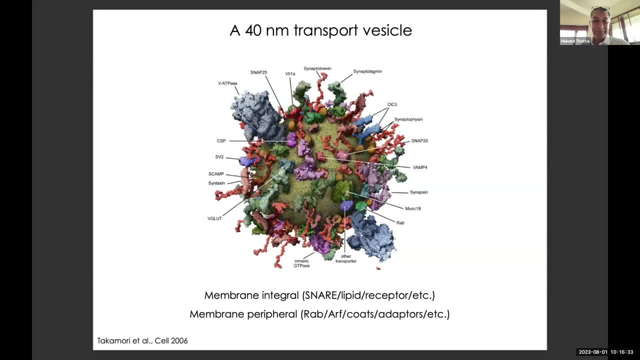 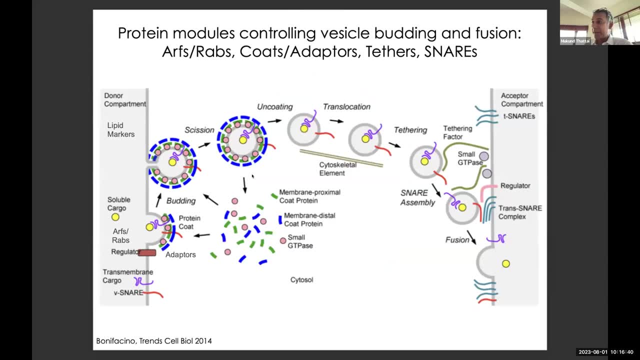 in between. yeah, yeah, yeah, okay. so inside a cell there are these different locations. i think of them as places, right? you can think of them. to extend the analogy, you can think of them as warehouses, where things move right. so there'll be a source warehouse and a target warehouse. 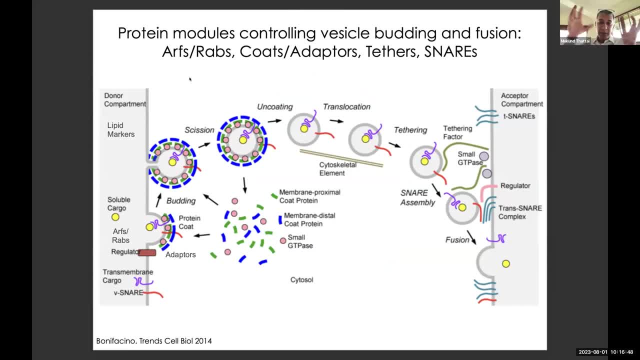 these are called compartments. they're bounded by membranes. you can think of big hollow sacks that are inside a cell. could be the er or the golgi or the endosome, whatever it is right. so they're called compartments. they're bounded by membranes. you can think of big hollow sacks that are inside. 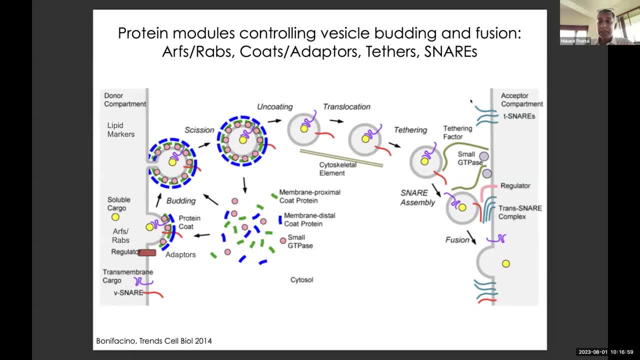 called compartments, so they're called organelles, and there are donors and acceptors. i sometimes call them source compartments and target compartments between which stuff has to move. and the important stuff is not the stuff in the white space which is in the cytosol of the cell, the cytosol of the cell, um, everything is shared by everyone, but inside a compartment. 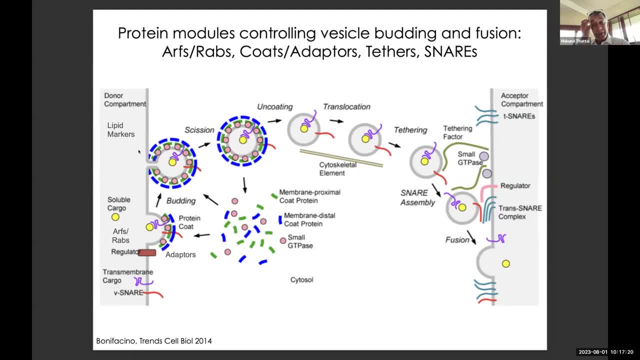 it contains its own unique stuff, and that's the important thing about compartments, right. there's something different about its composition that allows it to have a different function. for example, the lysosome has one of its functions is to degrade stuff, right. or the er one of its 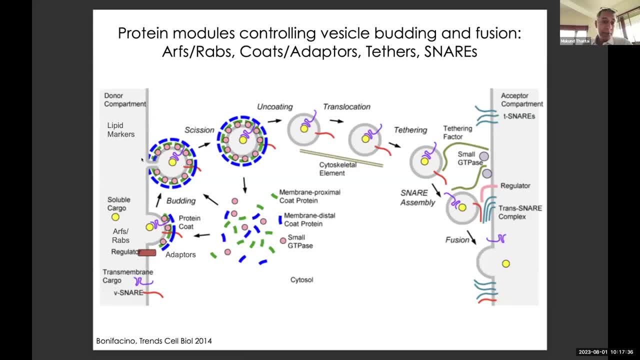 functions is to make molecules. so inside the donor compartment there will be stuff, but also across the membrane of the donor compartment there'll be transmembrane cargo, which is this purple thing. similarly, inside the target compartment there will be stuff in the gray area and there'll be these transmembrane proteins and the goal of the whole system is to take the. 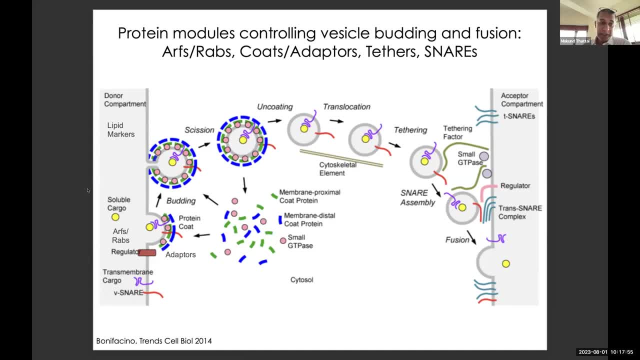 right stuff from here and deliver it to here. not all the stuff that's in the target compartment. all the stuff from here, of course. right, you don't want to take everything from a warehouse. when a truck shows up at a warehouse, it picks up the right thing and uh and moves um. so what i have? 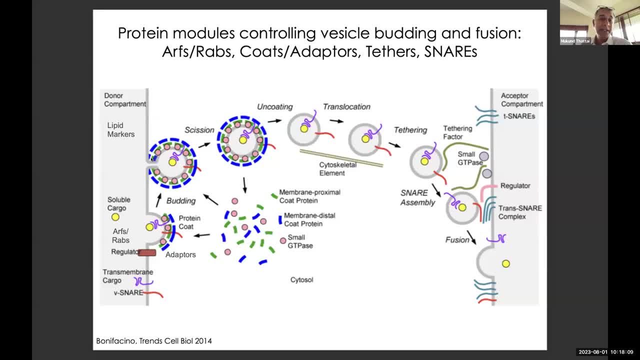 here. so maybe the correct analogy is: these vesicles are not packages. in fact the vesicles are trucks and these little molecules are the packages. but anyway, let's not belabor that, uh, that analogy. so what happens is: uh, there's these things called coats and adapters which create, um, a little ball. 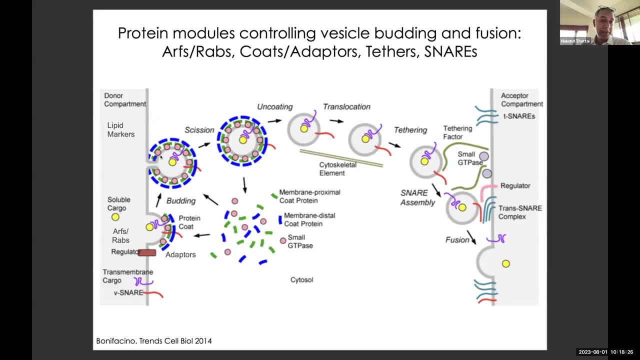 and they actually attract the right cargo from the source compartment and they undergo scission and they become their own little package. now, among other things, some of the cargo that they picked up okay were in fact the identity markers. there's a whole bunch of other cargo which is just along for the ride, but some of these are the. 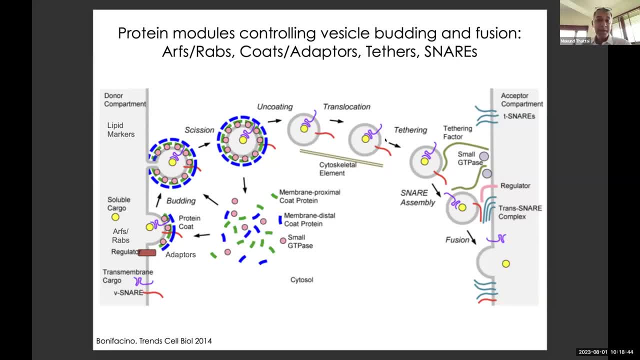 things that tell it where it needs to go. most vesicles just diffuse around the cell till they hit a certain acceptor or target compartment and then they check using a lock and key mechanism. they have a sort of key template, called a v snare or a vesicle snare, which checks against a molecule on the target compartment, called 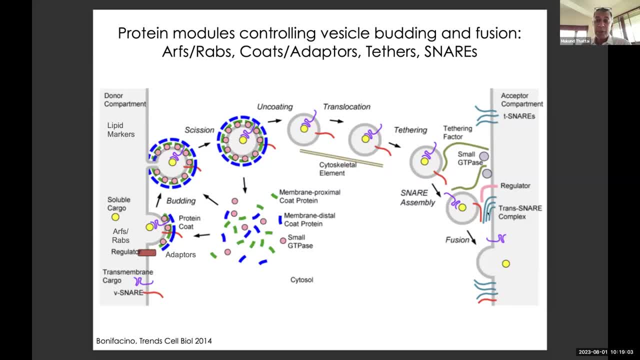 the t snare, and if those two undergo the right complementarity, exact protein pairing, um- then this thing actually fuses and it delivers this cargo, in which this case is the yellow- uh, the yellow- molecule. okay, so, as you can see, it's a very, very sophisticated process involving lots of molecules. 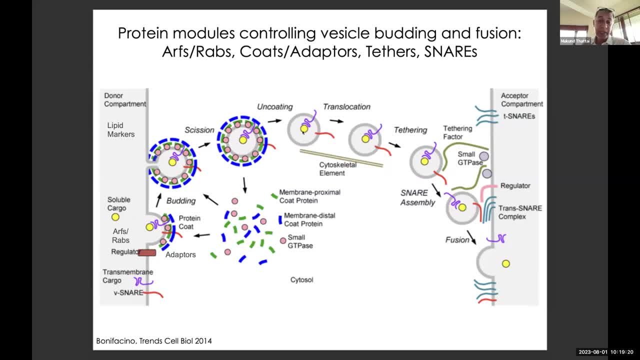 the code which recruits the cargo, some of the cargo which test whether it's the right target, some stuff on the target compartment, which is the target compartment, which is the target compartment which tests if it's the right package, and then it fuses um. so in this whole process, um, you know, 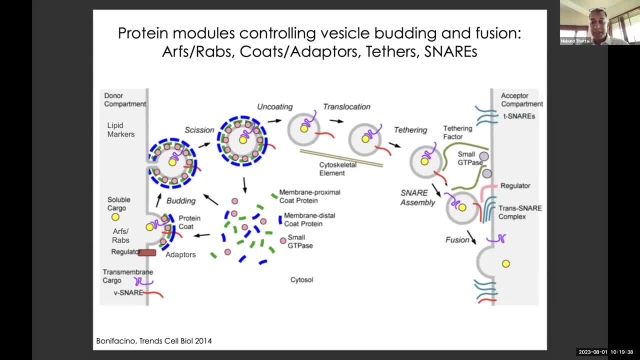 what we'd like to do is model this whole thing, but it doesn't even give you the right impression, because the important thing is stuff inside these compartments and stuff that are transmembrane cannot, cannot escape into the cytoplasm and go where they want to. 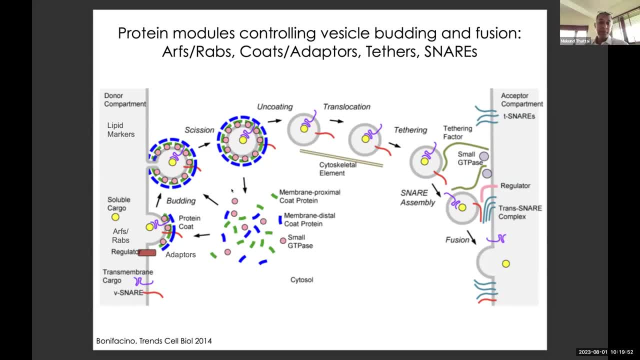 because the energy barrier to cross the lipid bilayer is actually quite immense. so the energy barrier to cross the lipid bilayer is actually quite immense. so if some of this stuff which goes there has to get recycled, it has to come back on a different vesicle, it can't just exit. so, for example, this red guy. 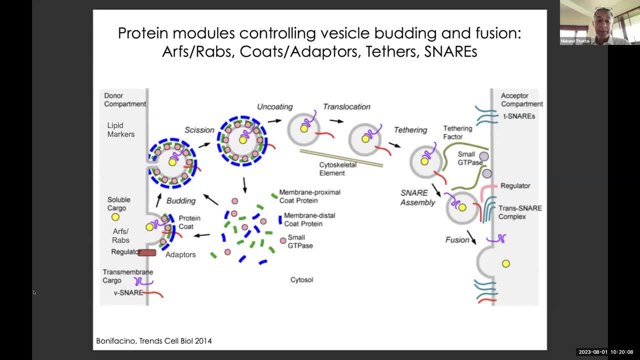 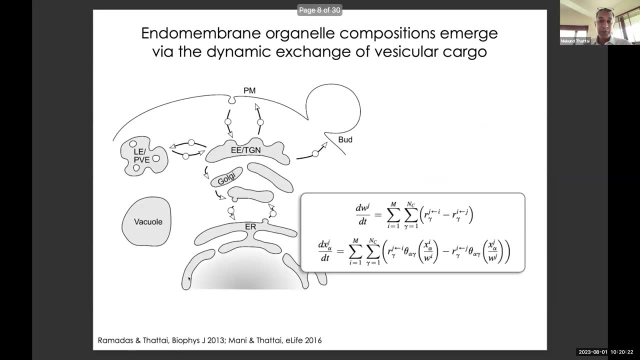 which started here, the v snare. it reaches the target, but how does it get back right? this textbook picture doesn't actually give you, uh, the solution. in fact, we don't really know the answer, but i'll present a potential answer. okay, so that's one picture of, uh, you know, from one source to one. 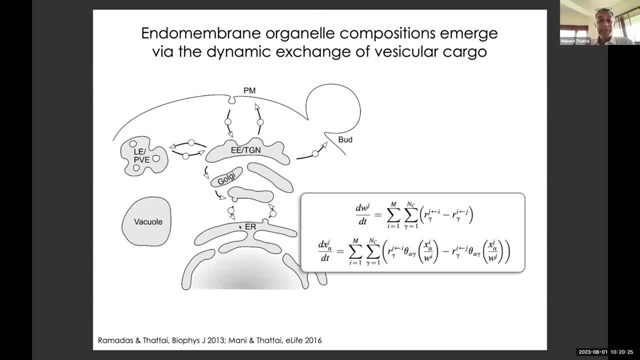 target, but that doesn't even give you the right image. the right image is you have a whole cell. you have different source and target compartments and lots of them are connected to each other by these vesicles that keep moving between them. and the vesicles move at a rate. 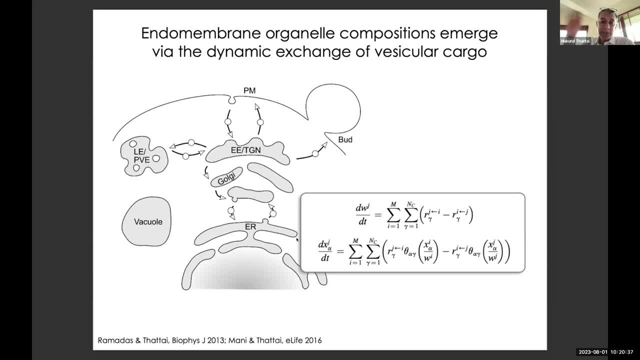 of tens per minute. they're always budding from one side and fusing to the other side right, and the issue is actually quite complicated because when you bud from the source compartment- and i've shown that by representing these differential equations here, which represent the composition of chemicals x, okay on compartment j. 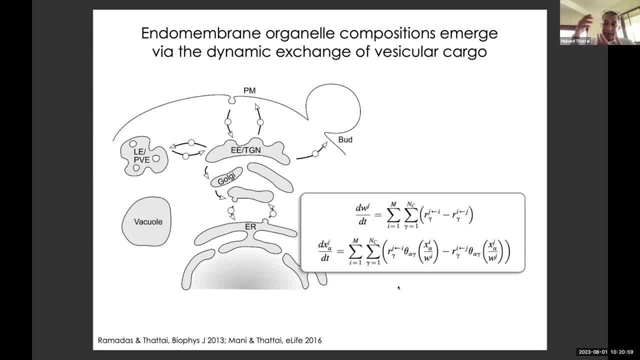 right, so j can go from one to ten, meaning the er, the early endosome, late endosome, lysosome, whatever it is, and the chemicals subscript. alpha can go over thousands of different chemicals in the same. every time a vesicle buds from a source compartment, it changes the composition of that. 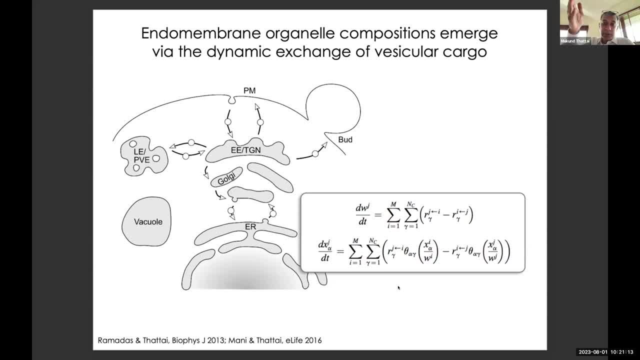 compartment because it took away stuff, and every time it fuses to a target compartment it changes the composition of the compartment because it gave stuff. now this is constantly going on. why, when we look at a cell, does it look more or less constant over time? and the answer is: because everything is balanced. okay, so all the stuff that's coming in from some 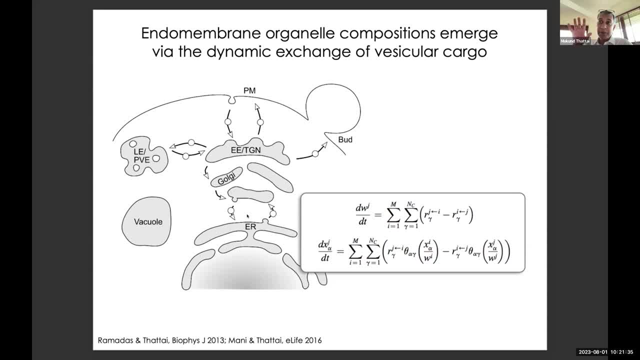 place is also going away from some place, and so the actual composition of a compartment doesn't change much, right? and this is, uh, something which the cell actually achieves by using various types of feedbacks and so on. you can actually make mathematical models of this and show how that. 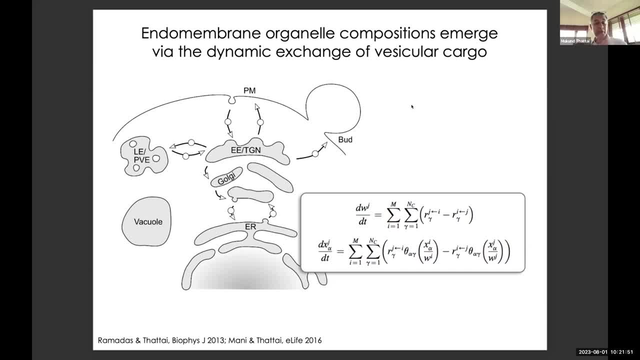 balance is achieved. yeah, but the main point i'm making is that you have to think of the global system, and the main point i'm making is that you have to think of the global system, and the main point i'm making is that you have to think of the global system, and it's really these: 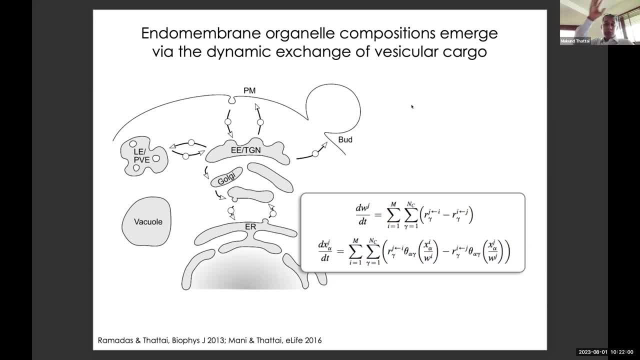 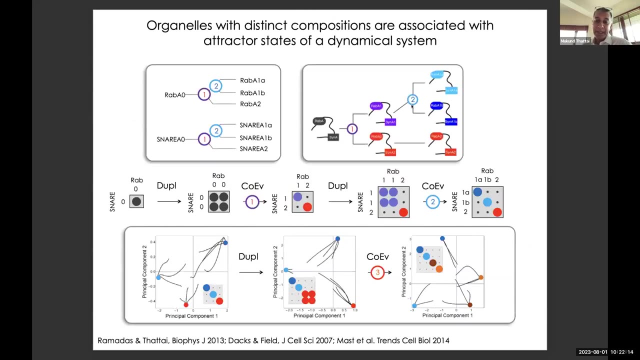 microscopic vesicles moving that eventually lead to compartments having the right compositions, right. so that's an amazing change of scale. control at one level leads to outcomes at a much higher level, orders of magnitude bigger in size, um, okay, so we've done some work on this and we've- we've actually modeled how different compartments using differential 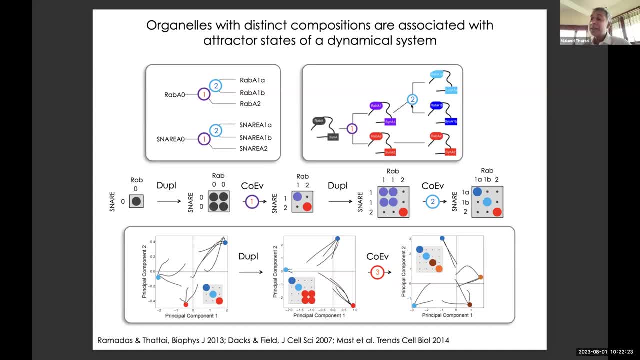 equations of the type i showed in the previous slide, how these different compartments arise. um, and you can actually show that it's possible to encode a certain number of compartments and a little bit about how they couple to each other, but uh, it doesn't really when, at this level, the 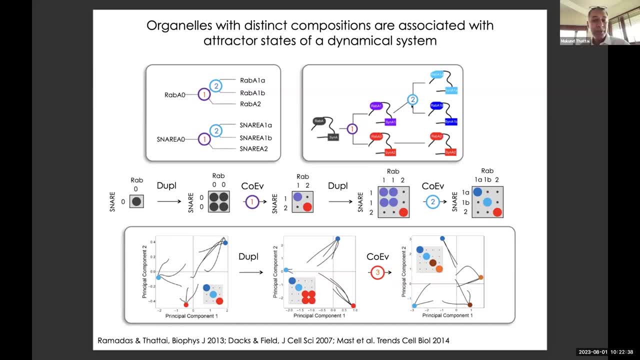 model is a model in the sense we don't really understand why it's doing what it's doing. if you put in some ingredients, it does something. if you get the ingredients wrong, it doesn't do it- typical with many models, and so we'd like to have a better explanation. 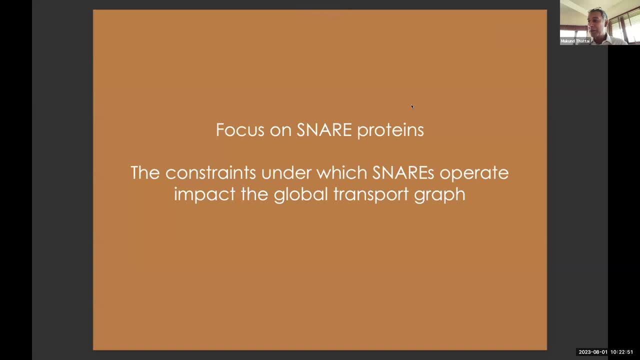 okay, so to do that? um, today i'm going to focus on something which is a very interesting aspect of what's happening in these very complicated systems, because i can't imagine addressing the entire cell biology of all those molecules i showed you. i'm going to focus on one type of molecule which is extremely interesting, extremely potent and, in some sense, 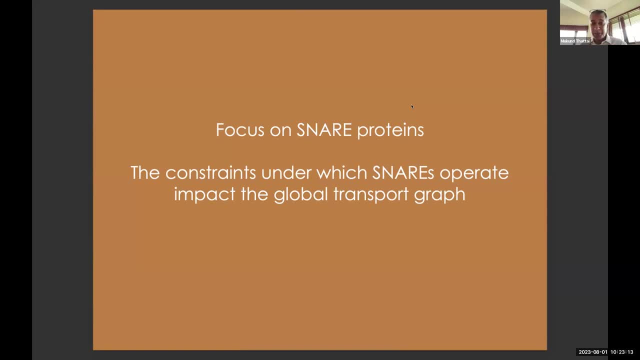 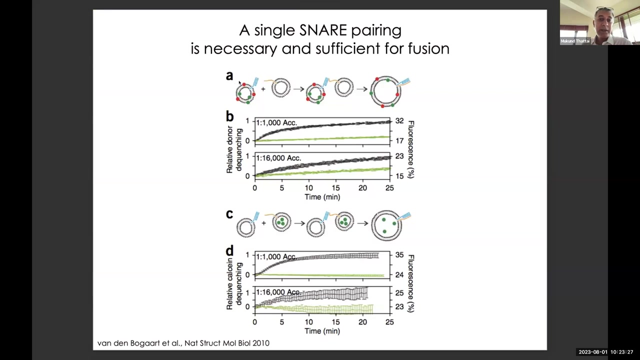 is the linchpin of all the complexity of this system. these are called snare proteins, so let me explain what they are. snare is actually a very long acronym, um. you can look it up, okay. so what is this name? as i showed you, if you have a lipid um vesicle, a lipid bilayer in this vesicular form, and you have two lipid, 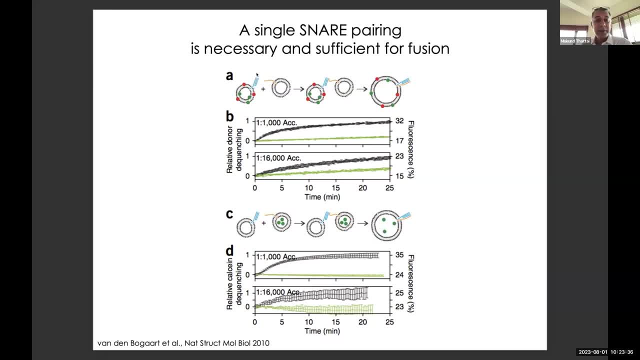 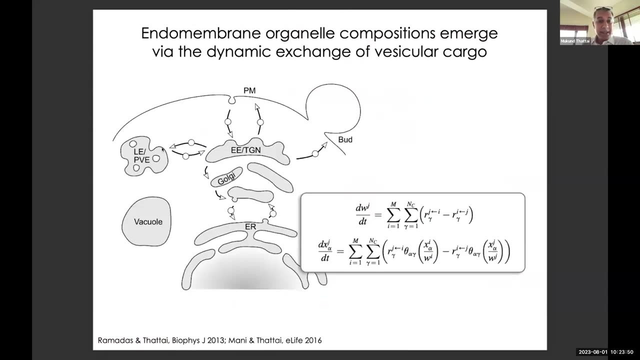 bilayer vesicles, one with a, with what's called a v snare, and another one which is called a t snare, and these have the right lock and key complementarity. then they will fuse. and what i failed to mention, um, and i'll go back and really reiterate this different vesicle. 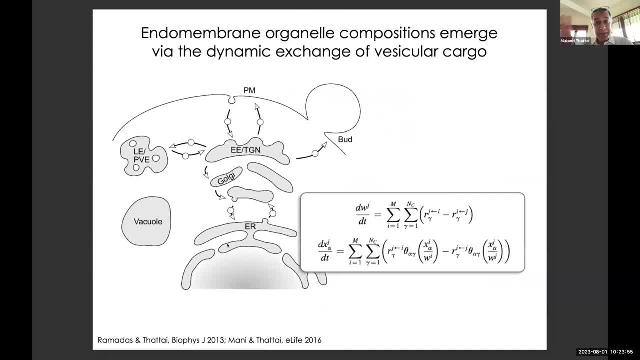 fusions in different parts of the cell again use v and t snares. but there are dozens of v snares and dozens of t snares encoded in the same genome and expressed in the same cell. and v snare one fuses with t snare one. v snare two fuses with t snare two and not with t snare one. 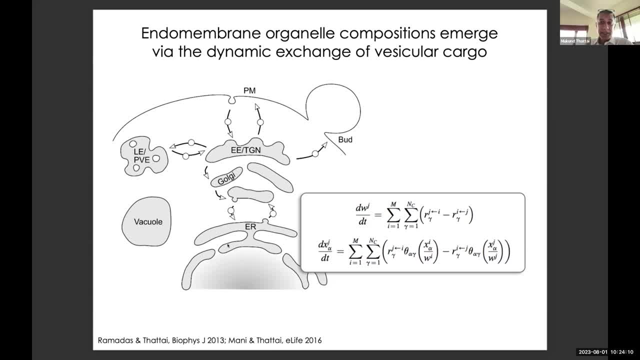 and so on. right, so there are very specific interactions. similarly, with these so-called gtps's that give identity, there are different rab and r gtps's that decorate different membranes, so even though they are homologous proteins. so, as bioinformaticians, you know about homology. 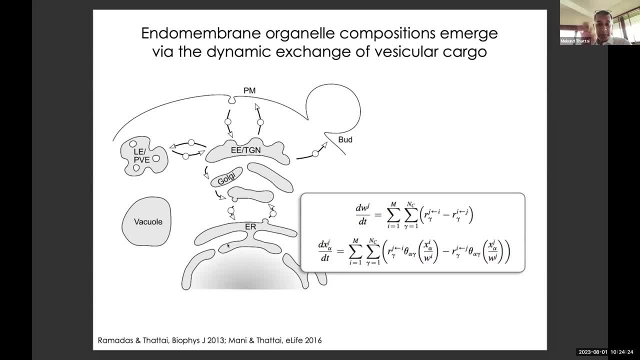 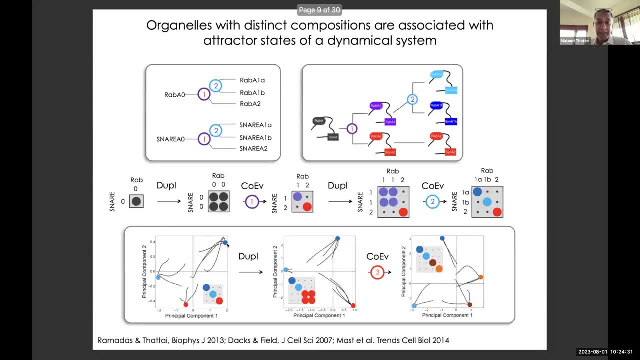 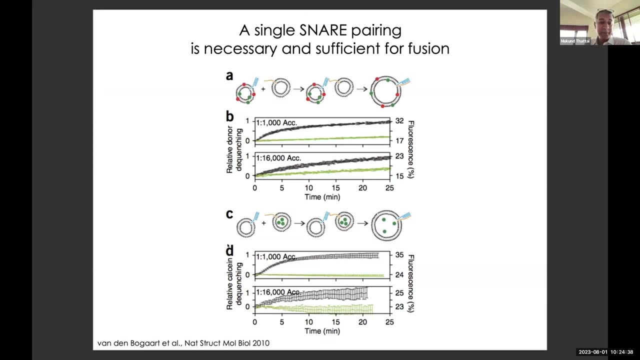 the same protein family, exactly the same domain structure, but with a few changes in residues. those proteins are in different parts of the cell, and that's what makes different parts of the cell behave in different ways. right, so here you have the snare proteins and the important thing about snare proteins, and that's what this experiment rather. 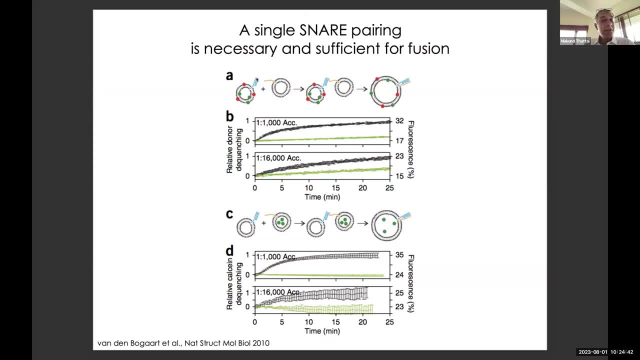 beautiful experiment shows: a single copy of a snare protein on a vesicle is enough to make it fuse. okay, so you should think of these as extremely potent, uh, fusogens extremely potent. so you can imagine that if you do that, you would have an infinite amount of energy to fuse. 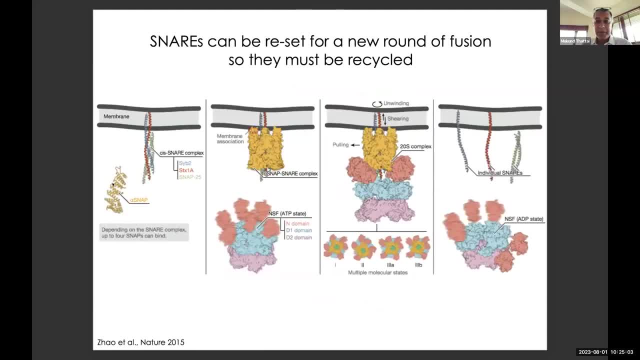 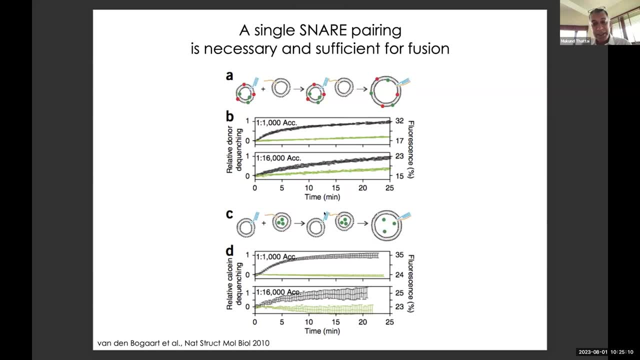 the snares, and that's what happens. you know, once you fuse the snares, you're in a process of the direction of this, of this process. um, you know, you can zoom in on this a little bit more, but, of course, once the snare fuses- and you can see that over here- what happens is: 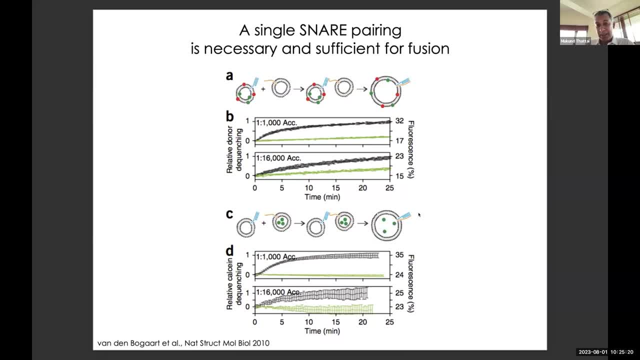 you have a snare. it turns out to be a triple helix on one side and a single helix on the other. after they fuse it forms a four helix bundle- details are not important- of association of those residues is what drives the force that causes fusion Spontaneously. 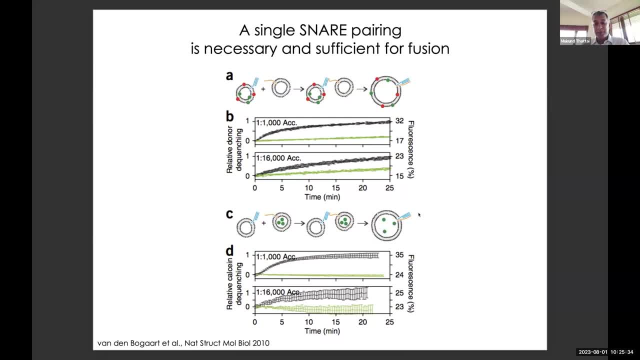 these vesicles tend to not fuse with each other because there's an energy barrier to overcome. But now you have a very tightly zipped up, complex right. So you have two options. you can either just throw it away- this is all just like a one-time use snare- or, of course, 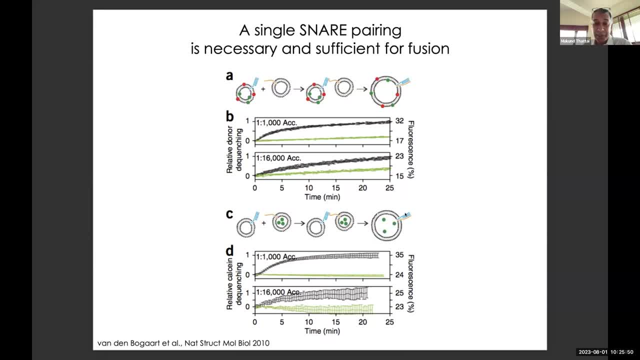 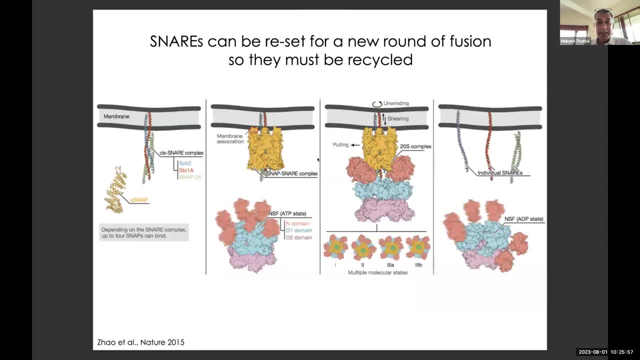 cells are not interested in synthesizing huge complex proteins and throwing them away after one use. you'd like to recycle. That's what cells do. So once you have a four helix bundle snare complex, there's an ATP burning machine which actually comes in. it's called NSF. 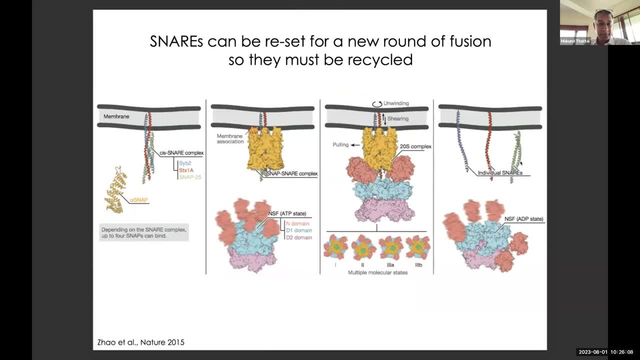 and it unwinds the snares and splits them apart And this harks back to the original question I had. So a snare that was brought in, once it gets split apart, needs to be taken out of this particular compartment and sent back to the source compartment. 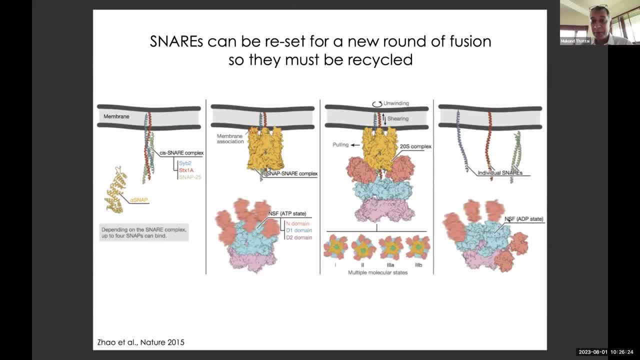 If you really want to recycle it, And that's the process I'm going to focus on today. So again in the textbooks you'll see this process very beautifully. the snare is unwound, but nobody tells you what prevents the red and the blue which, remember, are very tightly. 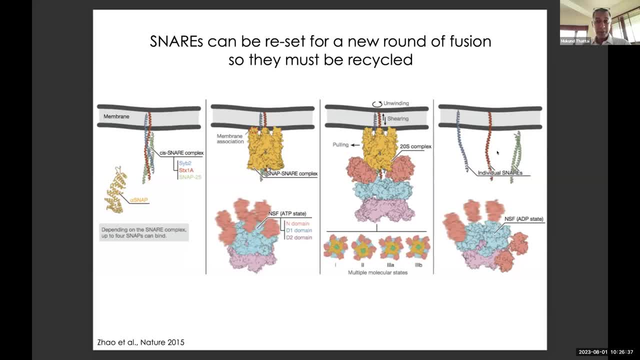 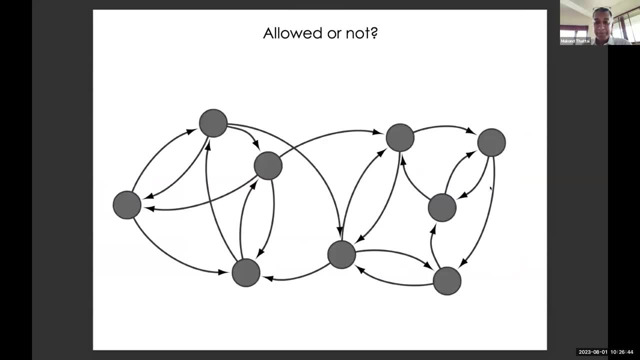 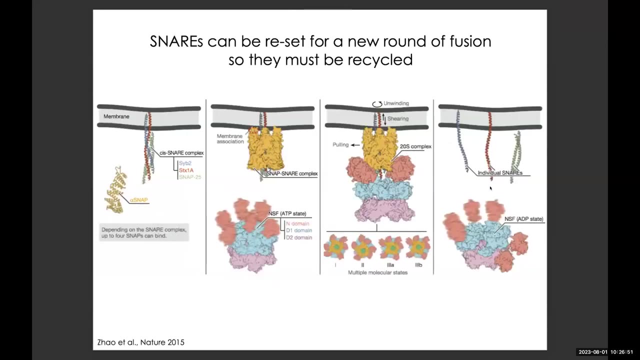 associating proteins to refuse. The only way to stop them from refusing is to pull out one of these things and send them back. So how does that work? Okay, Yes, question, Hi Mukund. this is Kasturi Hi. So this snare, fusion of one molecule being enough, 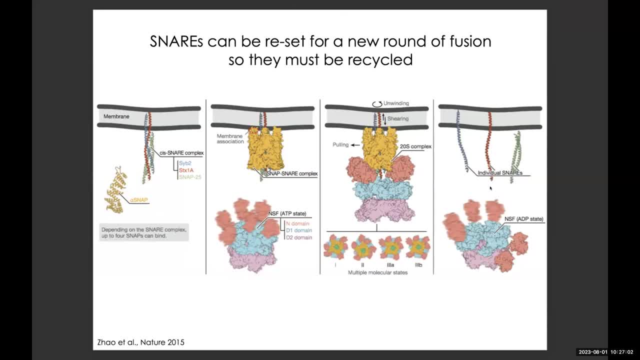 we are still assuming that it's 14 nanometer right vesicle in that ballpark, correct Sure for small vesicles. Yes, And then that's done in vitro or in vivo. I mean it goes together, Yeah. Yeah, that experiment is in vitro, It's reconstituted, Okay. 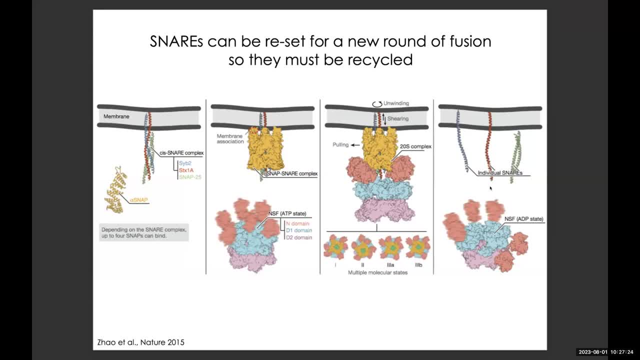 Right, Okay. So then maybe when it's happening in vivo, the density of the cytosol, or even the cytoskeletal elements, simplistically, can have a factor where the time they're close together, the fusing partners, matters. I mean, does it Or it does not matter because it happens in vitro? 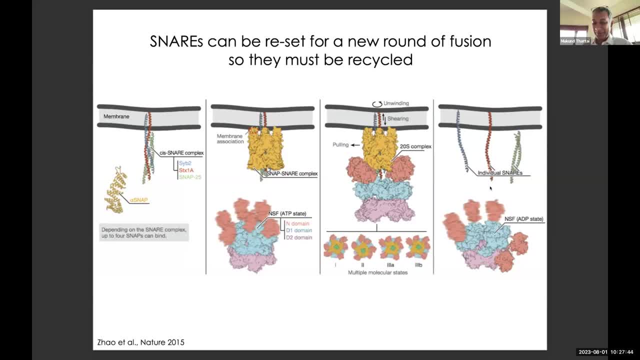 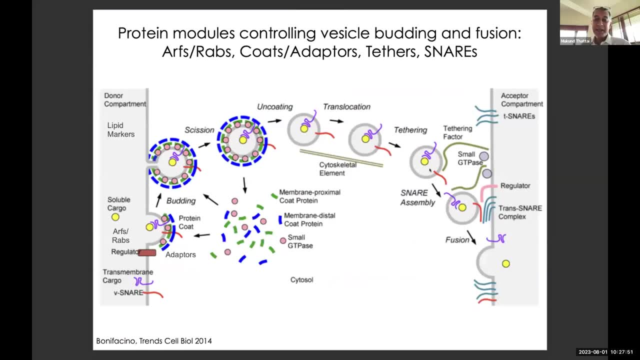 without them. No, it's okay. So I'm going to go back here. Okay, So this cartoon gives the impression. this cartoon, coupled with that reconstitution experiment, gives the impression that you just need this thing and that thing and you're done. But of course the cell is a. 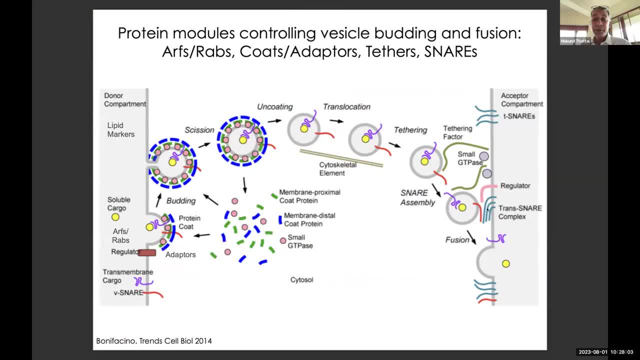 three-dimensional object. So for this to even start to take place, the vesicle has to be close to the target, And sources and targets are sometimes close to each other, like the ER and the Cisco, but sometimes they're quite far away, like the ER and the plasma membrane, And so the geometry of the cell does matter. 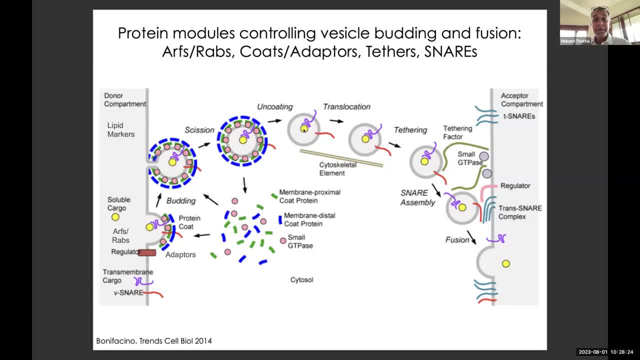 Secondly- in fact, the problem is the other way around. So often these vesicles will take a long time diffusing between places before they get to the target, And so you have a factor called a tether, which tends to have very. these are very, very long proteins which tend to 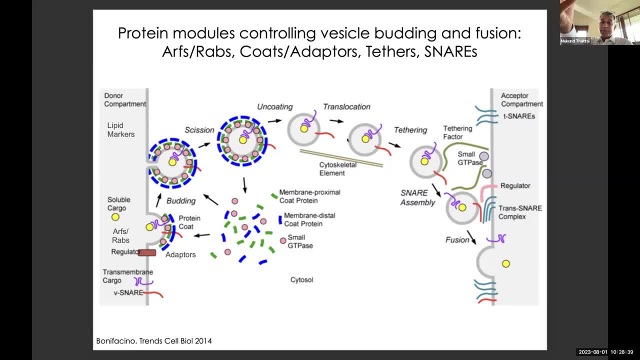 sort of flop around like seaweed and bring vesicles in and test them for fusion. So the tethers will be sort of promoting the testing for fusion. But the third piece, which I will mention shortly, is that the point I'm making is that, yes, if snares were so fusogenic, everything in the cell would just 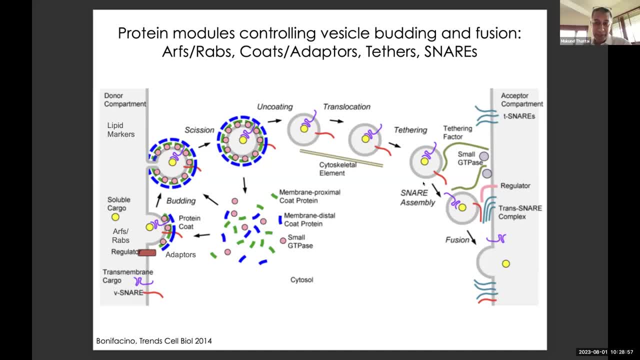 fuse and you wouldn't actually have this beautifully separated cell that you see today. There must be something preventing the fusion- which is sort of what I hear from your question- from happening inside the cell, although it's happening so quickly inside a tube. 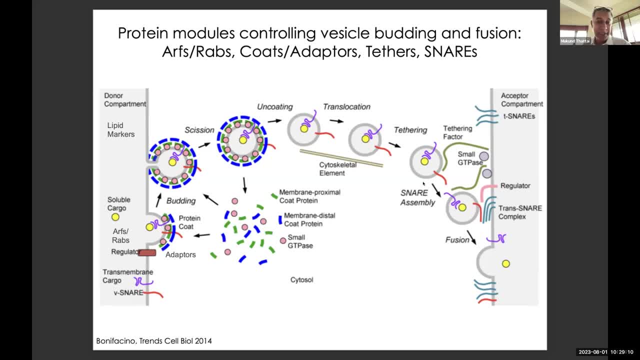 And indeed that's the ingredient which we're going to add today, something which actually regulates snares and prevents the vesicles from fusing so rapidly and in some sense indiscriminately, because that would not help the cell achieve its goal. 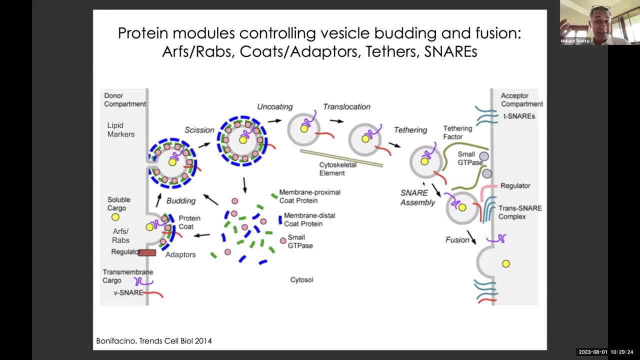 So there's the geometry, there are tethers, and then there's additional factors which are not shown, obviously, in this figure which I'm going to then bring up. Thanks, Yep. So I do not mean to at all give the impression that these things are so simple that they're. 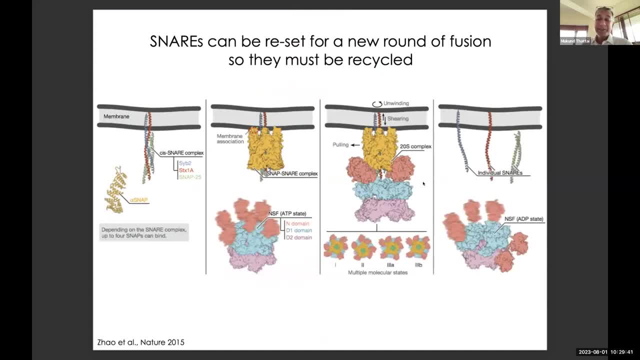 run by, in fact you know. this is why you keep going back to look at the old EMs, because in the textbooks they look very simple, but in practice you have to keep track, as Kasturi said, for all the other stuff that's happening. 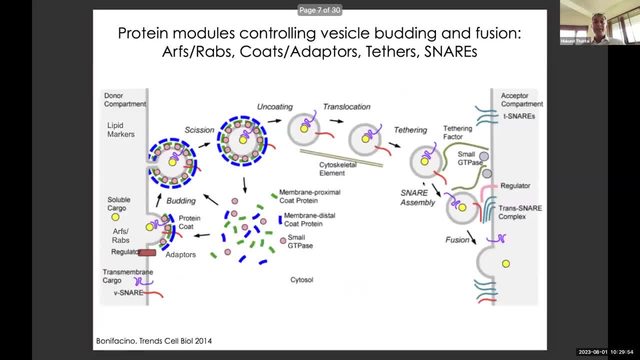 One recent result which is actually interesting: the textbooks. you know I'm sorry to keep going on about textbooks, but you may get the wrong impression by reading them, so it's my duty to correct your wrong impression. The textbooks give the impression that vesicles. 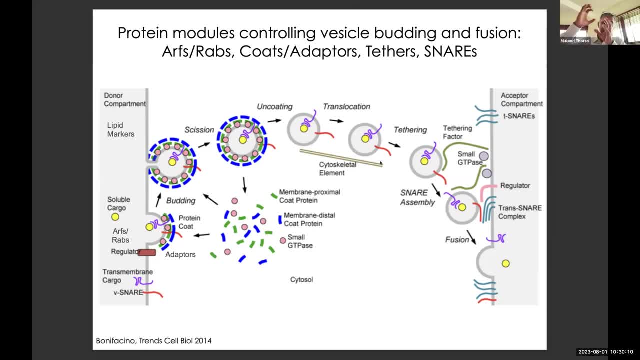 jump onto cytoskeletal elements, move with motors. there's this famous video of a vesicle moving along a track and pulled by a motor and walking and all that. 95% of vesicles don't do that, they just diffuse. Some vesicles do that and they're quite glamorous, and so we tend to focus on them. 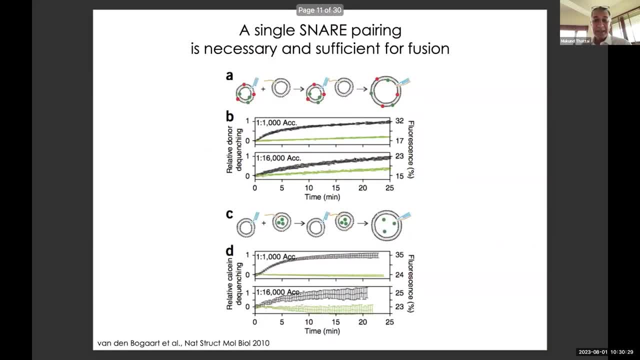 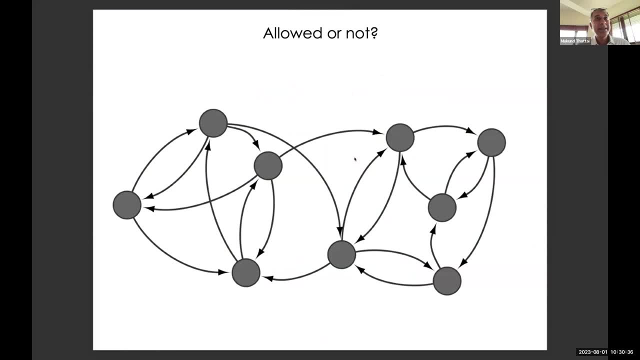 Yeah, but a lot of this is quite random, Okay, so now I promised in the title of the talk that I'm going to bring in some mathematical puzzles, so I've sort of dosed you with a huge amount of molecular biology and cell biology. 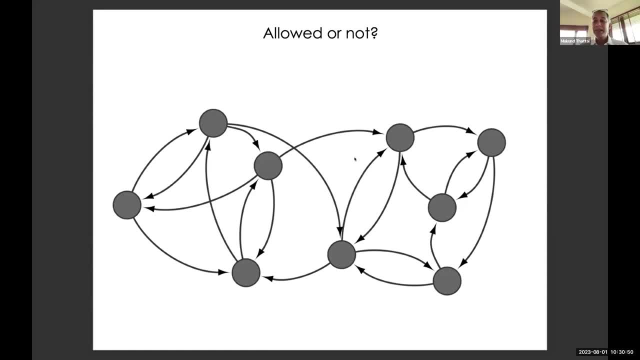 you've sort of I hope- digested a little bit. you don't have to know all of it. No, you don't have to know all of it. you're fine, But I'm going to bring in the mathematical. so now I'm going to bring in the mathematical. So now our goal as modelers is to keep the. 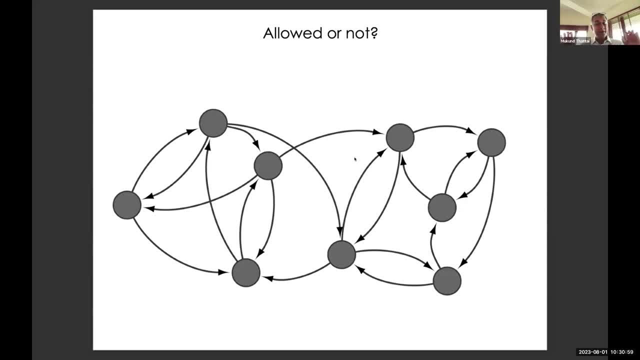 important details and remove not the unimportant details, but the details that are too complex to deal with at the beginning. you incorporate them later, And so what we're going to use is an abstraction, and it's an extremely powerful abstraction. it comes from a field called graph. 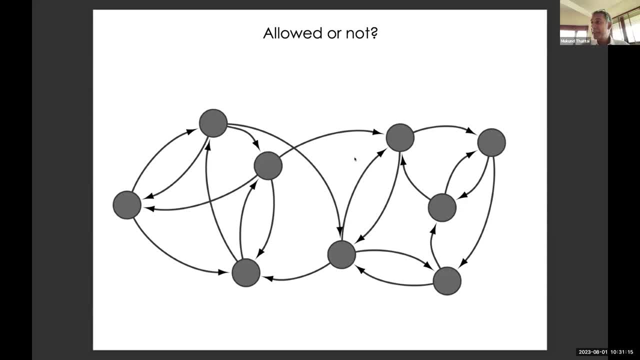 theory. So unfortunately the word graph has two meanings in math. one is a graph of y versus x, which is not what I'm talking about, so that's a little bit out of the question, but that's also a talking about. the graph i'm talking about is a, is a structure which has nodes and edges. so this thing- 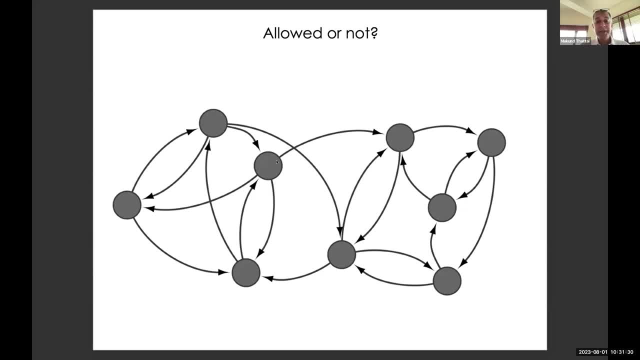 i've shown you is a graph, and it's not just a graph. it's a directed graph, because the edges have an arrowhead which gives you a sense of flow. um, so, what should we be thinking about this graph? what does this graph got to do with the cell? well, this node, for example, is the eon. this node is the. 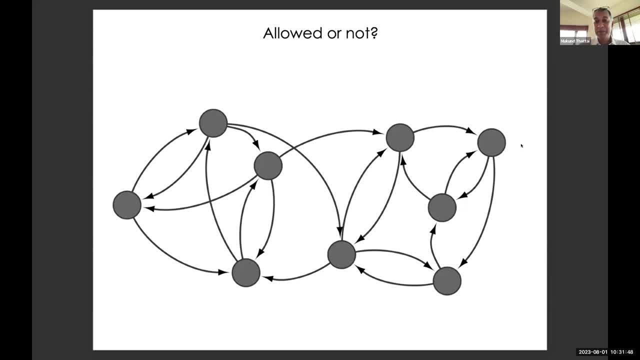 cis golgi. okay, or maybe i've made a bad choice. so this is cis golgi, medial golgi, trans golgi, plasma membrane, early endosome, late endosome, lysosome. okay, so these, these are all places inside the cell, the inside of the er, the inside of the golgi, these are all things you're used to. 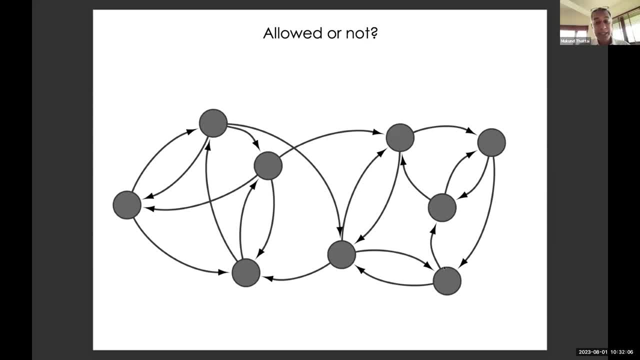 thinking about because they contain the cargo. one thing you may not be used to thinking about is the inside of the plasma membrane. but when you're in, when you're sitting inside a cell in the cytosol, looking into the plasma membrane membrane is not very different from looking into the ER. 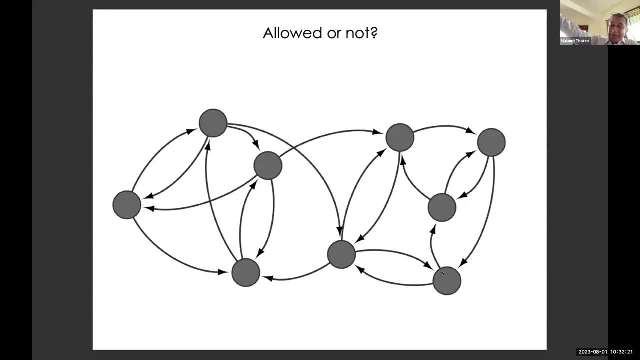 Although the rest of the universe is inside the plasma membrane, for the cell it's still something that's contained as part of the plasma membrane, So that's what this is. So this is something which it wouldn't be drawn in this way. 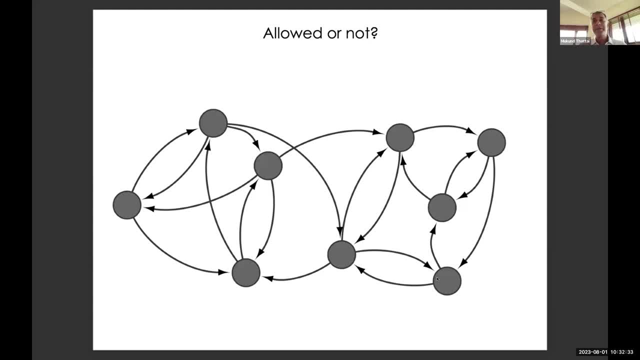 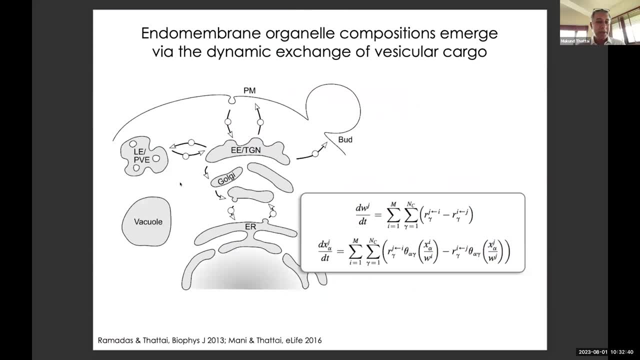 but when you read a paper about the discovery of a new vesicle traffic pathway, they'll draw a cell, a schematic cell perhaps, like I've drawn over here, and they'll draw the shapes very nicely and so on. And the point I'm trying to make here is that 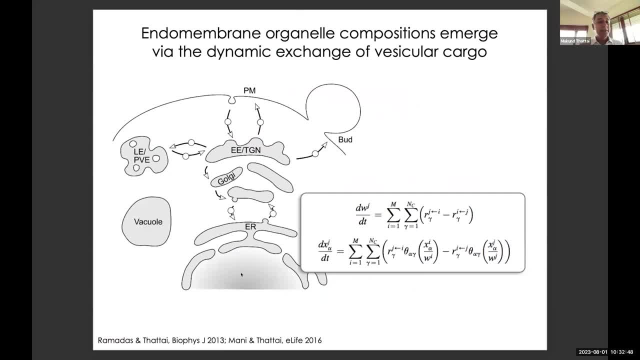 for the moment, let's ignore the shapes, the sizes, the locations, although they're very important, as we just heard. but let's ignore all that and come down to the topology: Who is connecting with whom by what vesicles? So then I can just convert every compartment. 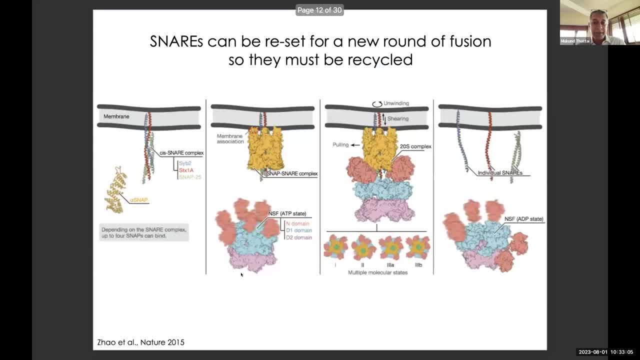 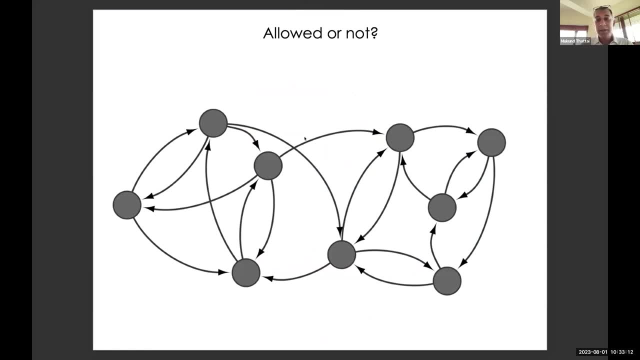 to a big gray blob and every vesicle to a small white blob. Okay, I haven't shown the vesicle blobs here. So these are compartments and vesicles move, not in three dimensions, but they flow from this compartment to that compartment. Okay, so that's the abstraction. 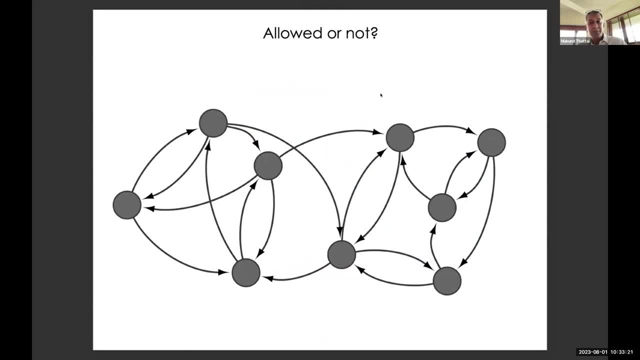 And somebody says: this is my guess. for what? the special cell type? maybe that immune cell? that was part of the question. I've studied this immune cell for a long time And I think these are the compartments And I think these are the edges after a lot of work. 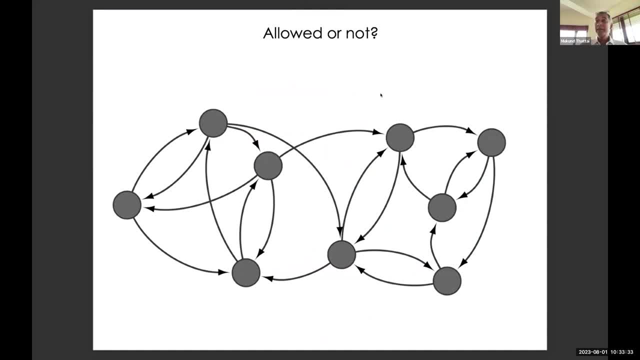 And now I have to say: well, from what we know about molecules, can this thing exist or not? And you may think there's too much of a question to ask, but it turns out it's not. This is where graph theory comes into it. 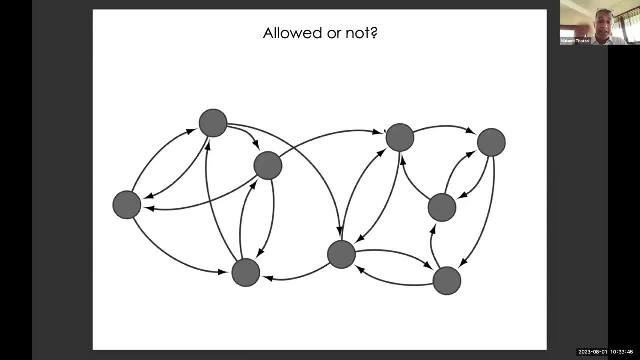 So I've told you already that every vesicle fusion has to have a V-snare on the vesicle and the T-snare on the target. V is for vesicle, T is for target. Without the snares they won't fuse. 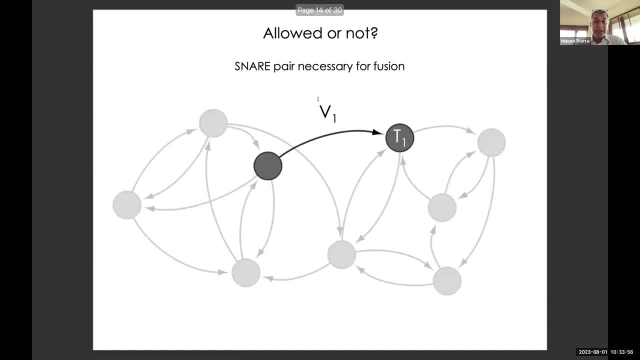 That is true in vivo or in vitro. So we posit that there's a V-snare, that's a transmembrane protein traveling along this vesicle, and a corresponding T-snare, the one it likes, on the target. V1 loves T1.. 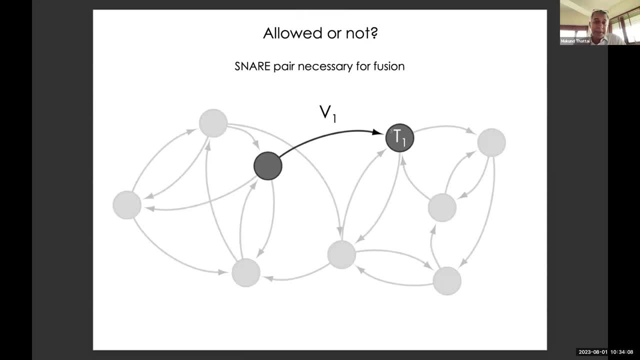 So a vesicle carrying V1 will fuse to compartment T1. That's great. So we're just focusing on this pathway, right? So you think that's done, and all I have to do is then make similar V's and T's for all the other pathways. 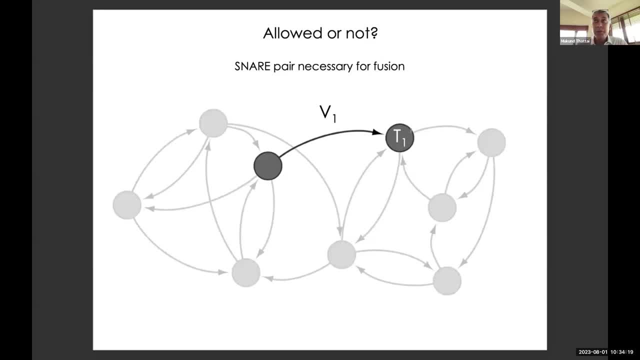 But that's not so easy, because once the vesicle, the snares fuse, maybe you have to pull them apart. And then you have to send the V-snare back to the origin because- and this is true- it's not destroyed after one use, it is reused. 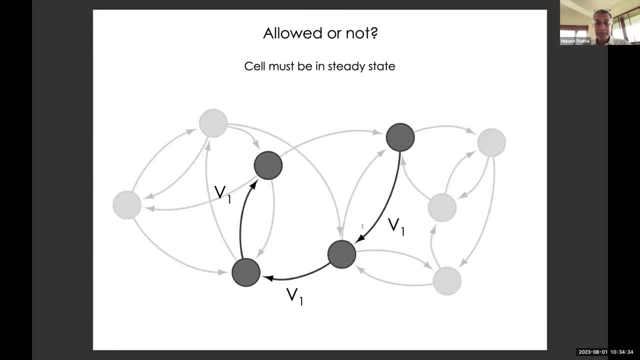 So you say, okay, I'm going to find a path. There's one, there could be others, but I'm going to find a path that takes me back to the source compartment. There's one right there. And you think now you're done, because now the V-snare. 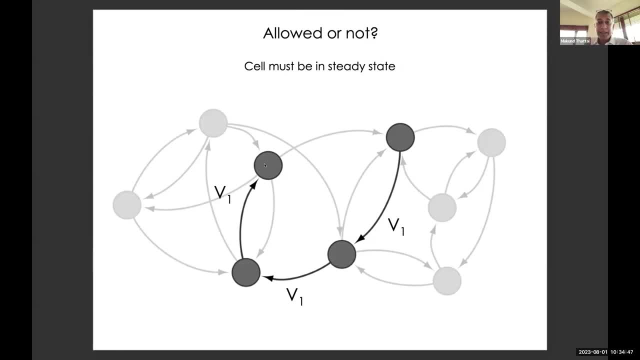 is back where it started and you need to fuse again. So you send it back along this vesicle. But now you're in trouble And does anybody notice the trouble? The trouble is that if this is what is being carried on this vesicle, this vesicle carries V-snare V1.. 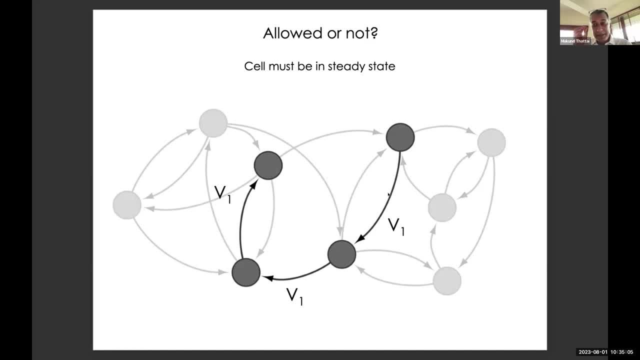 And I told you that a vesicles properties are determined purely by the cargoes they carry. We've already agreed that a vesicle that carries V1 will fuse to compartment T1. So why doesn't this vesicle fuse back? And that's the major issue. 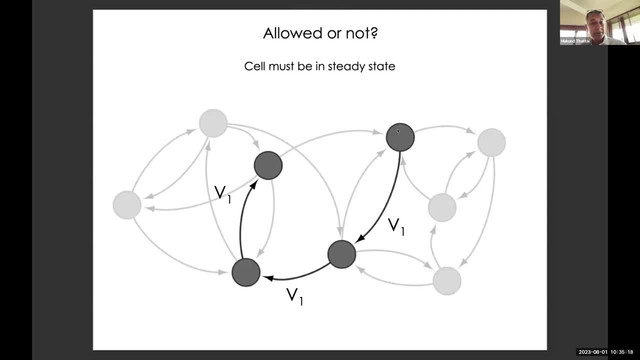 We actually don't fully understand, right, But there are some patterns and I'll show you one example of how you can do that. So the immediate thing you should think of is: well, let's inhibit it. So I make up an inhibitor. 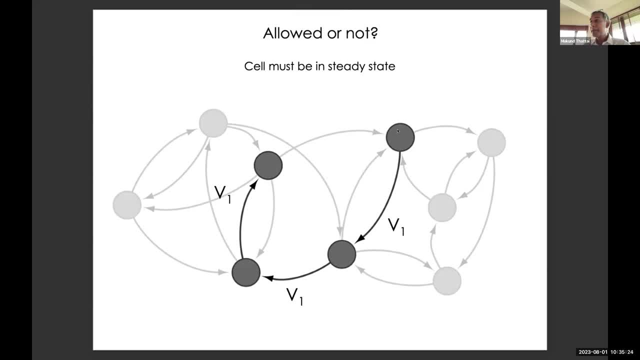 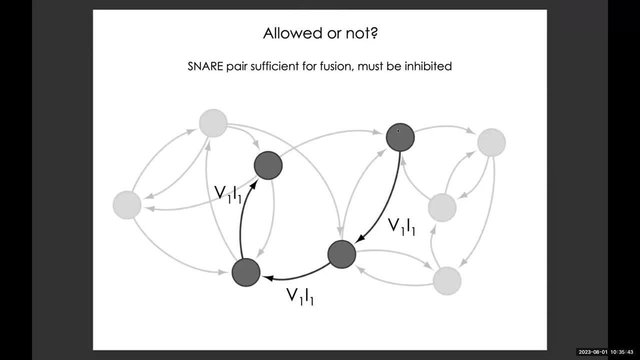 Question Question. Question Question. A reading earlier says: if I put two compartments to the second compartment, usually it reaches T1, because it had T1 for accepting Yes. Now when you're saying that this reverts back to the form, 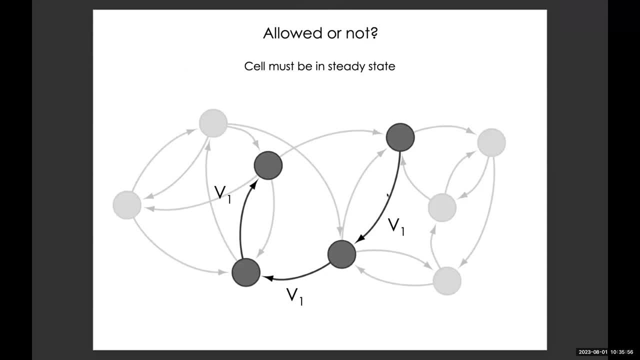 where it has started. so move from the second compartment to the third compartment. there should be some receptor also, right? Yes, but that's if it reaches there. The first thing it sees when it comes out of here is its own source compartment. 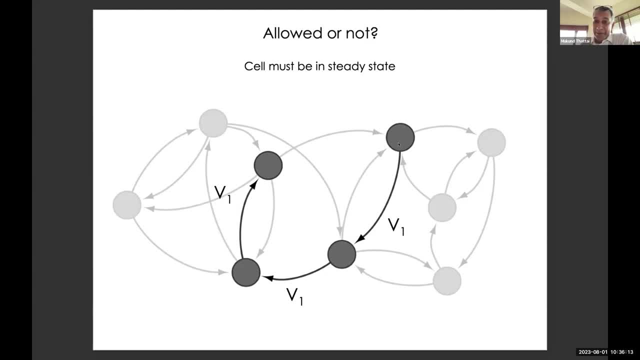 That's the one it's closest to. So, in fact, do this experiment and you don't put inhibitors. these things constantly refuse. yeah, so it is a real problem inside cells. that has see, v1 loves t1, right, we already established that, in which case this vesicle carrying v1 has to go back. you're asking how it fuses here and we'll get. 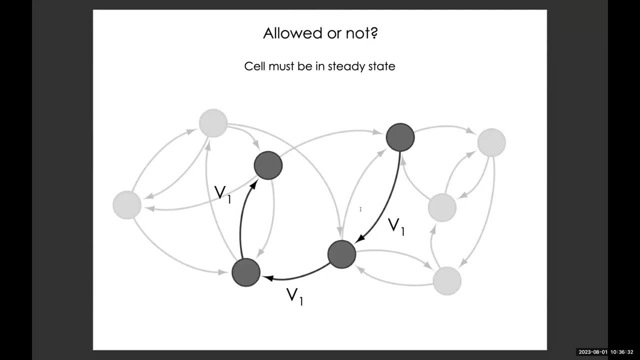 to that in a second. yeah, i, i also. i also had a similar question like: uh, the previous node at the top, uh is even right now the edge going down. um, what is this node, you know? so you guys are getting into it. so the point is that we now have to, if, if we're to make a hypothesis of this, we have to. 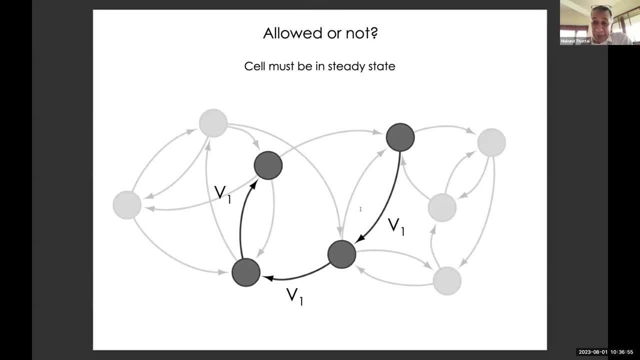 decorate the entire graph. i have to put all the t's, i have to put all the v's, i have to put all the recycling pathways, and then i get a solution right and i'm going to work my way. this is what i'm going to work my way up towards through this talk. so hold your horses, we're going to answer. 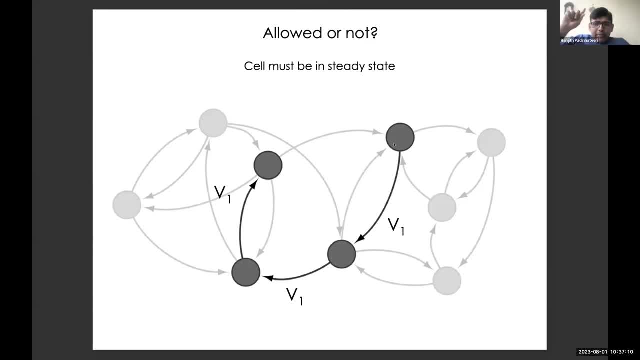 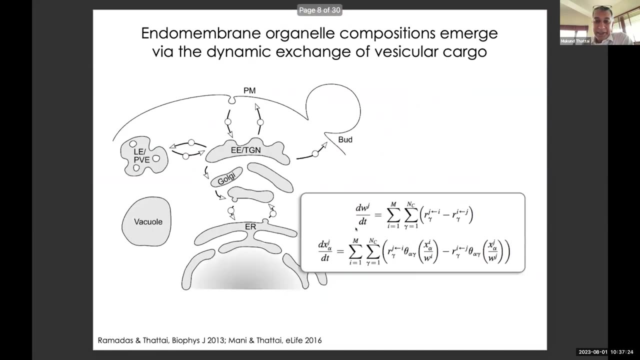 those questions. i also have a question. so when you say steady state, is it steady state in number or flux, or what exactly? it would be both, both. so the fluxes are in. uh, the whole thing is steady. so the composition of each compartment is described by a differential equation of this type. 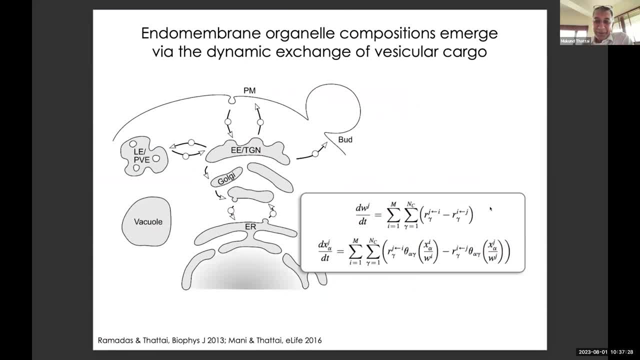 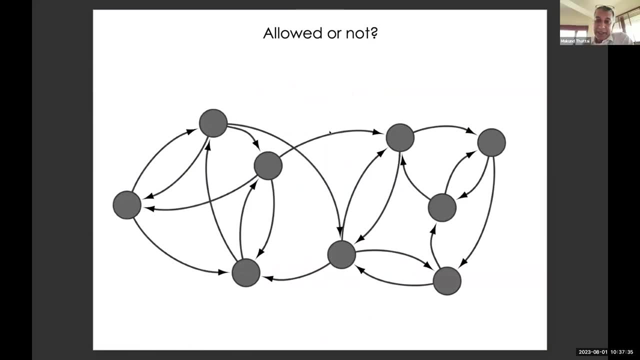 which covers the entire graph. okay, so you should really be thinking of a flux coming and the flux going, but the flux, for example incoming flux of x here, could be balanced by the flux of x here. so the flux of x here could be balanced by the flux of x here. so 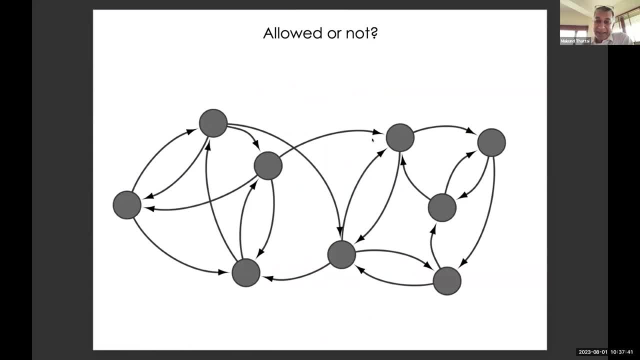 the flux of x here could be balanced by outgoing fluxes and incoming fluxes across the entire set. so locally every compartment has to be balanced, and you again, it's complicated. but uh, i will get to the steady state question too. but this is great. so the point? the point is that if you just start, 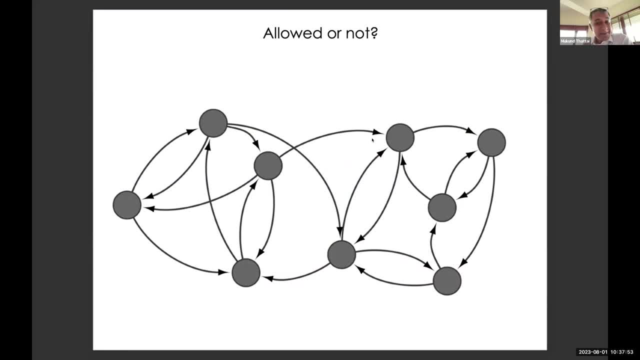 with a cartoon like this, then you realize: well, there's a lot of things that you weren't told, and so you're asking: what exactly are the details about fluxes, steady states, fusion specificities and everything else? and so those demands are what we now need to address with the 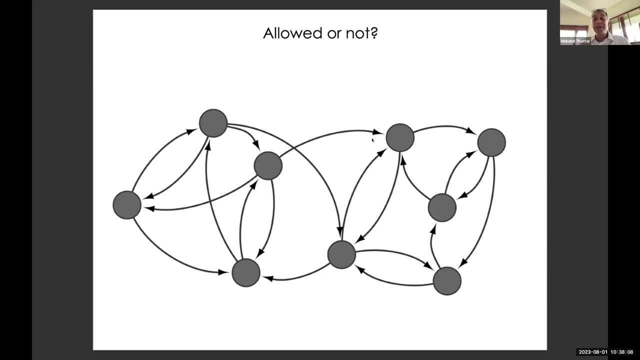 model. one way of saying it is that these cartoons are the ones that are going to be balanced and are not sufficient. if somebody says this is what, i think you should ask for more details. okay, but i'm just focusing on a little mystery. there are many other mysteries, yeah, question. 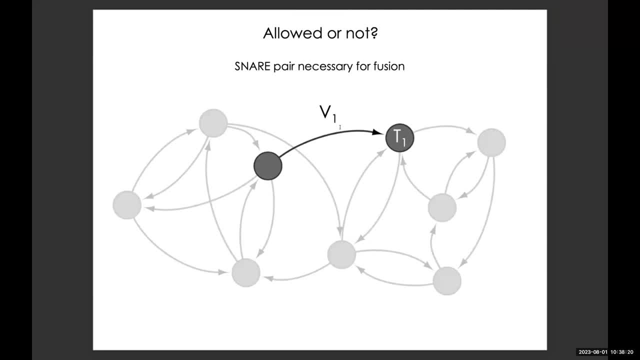 like: uh, two possibly naive, silly questions like: could you have a case where globally it is stable but the local nodes are like dynamic and changing all the time? and yes, you can, and i won't talk about that today. uh, we have done work on that. that's a process called compartmental maturation. 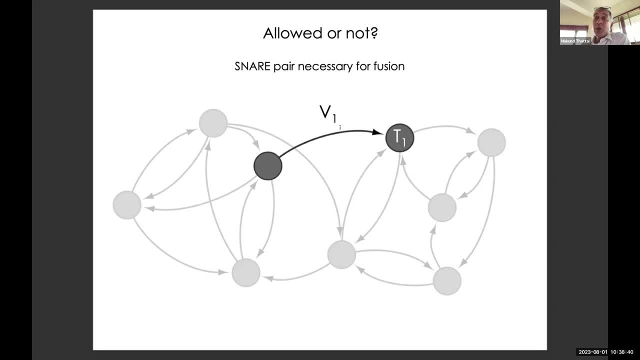 it's uh. now you've moved to a rather more complicated scenario, because the right model framework for that is a, is a markov process where the individual cell actually moves in its state, but the distribution across different cells in a large population of cells remains constant. so 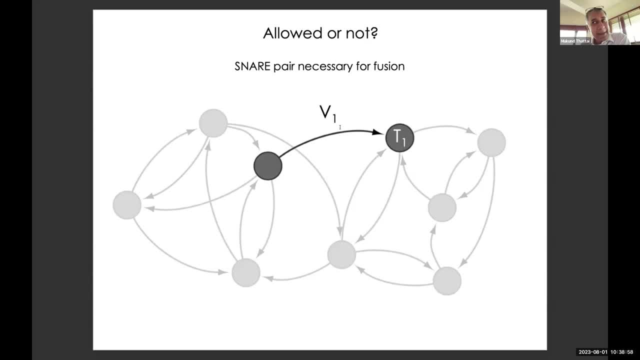 that's a different type of steady state which i'm not going to talk about today. it happens, but it's not universal. the simplest type which i'm talking about today is 90 of what you need to understand. second question: you had two questions. no, and i was just thinking the converse of that right could? 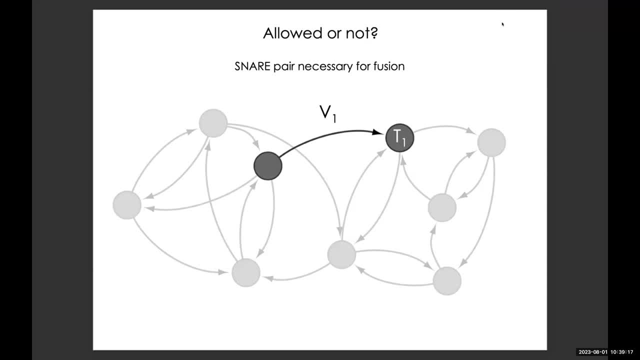 you uh be. could it be the case that locally they are stable, like at a steady state and uh, no changes, but like there is a global flux or dynamism? it is like that because one of the fluxes which i haven't shown, for example the plasma membrane, can 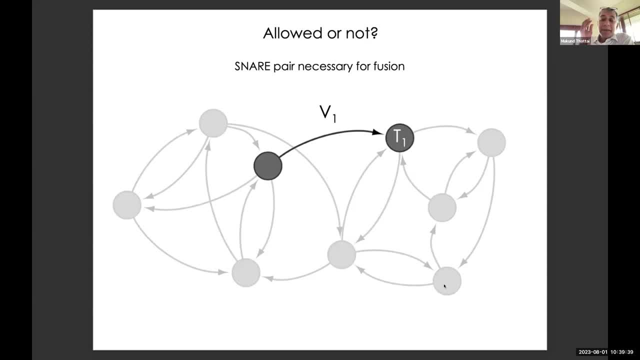 be the source. of course, i take that back. there are fluxes. okay, this is not in steady state because nothing is moving. it's in steady state because everything is moving. so this is the typical example of a dynamic steady state that you see in any out of equilibrium system, although it's a steady state, but it's. 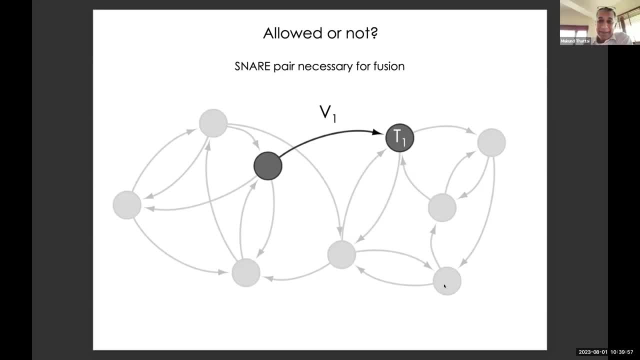 extremely dynamic. yeah, that that's the picture you should have in your head. everything is moving right, but it's the composition kind of they balance, like at each node it balances itself and it's not somehow in the sense you make dynamical systems, models and put in the right 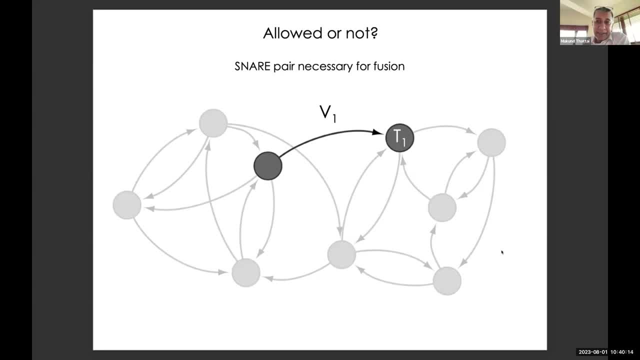 ingredients and they do fall into these patterns. so these attractor states are, you know, fairly common and you can, you can construct the mathematics, the. the issue is not their existence, but to really understand their structure. okay, and and one final question, uh, like i always get attracted to translational questions like: could you, could you make a wild hypothesis that? 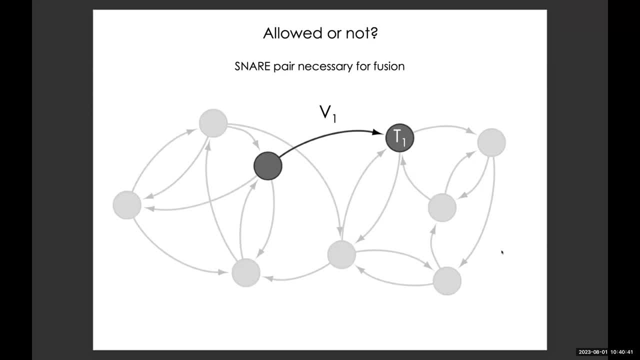 when they fall out of steady state. you know, like maybe the homeostasis or normal undiseased state is when they balance each other out and they're at equilibrium and, like disease state somehow corresponds to unbalance and uh, falling out of equilibrium. yeah, i mean. i mean, this is very new age. 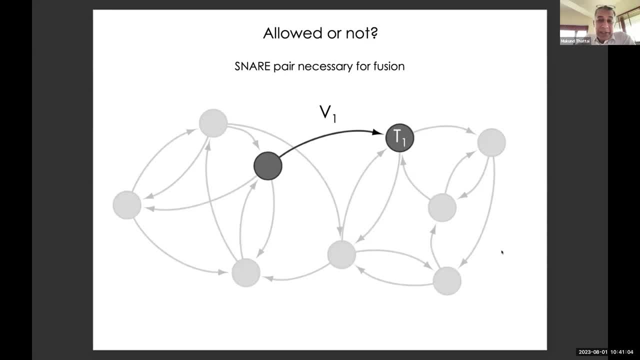 um, it's not like that, because in the natural world, there's no boundary between disease and not disease. if you look at, for example, a marine ecosystem, 100 of the marine microorganisms be infected by viruses and other pathogens. um and so the standard state is what it is i mean. so there are, of course, changes. for example, if you go from one environment to another, you may want to change your traffic pathways. there are of course cases, and very famously, when certain viruses infect eukaryotic cells, they change the pathways in order to actually shut down host protein synthesis and make a lot of virions that go to the cell surface. 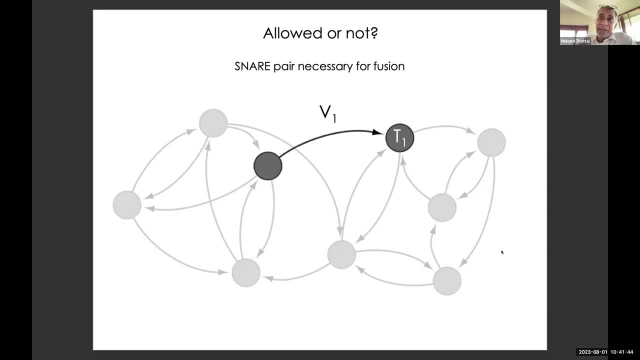 So those do happen, But the connection is not with disease and not disease, It is with different environmental circumstances, one of which could be infection. But actually, this is a question that we're going to start to work on soon- is: how do these pathways get rewired by viruses? 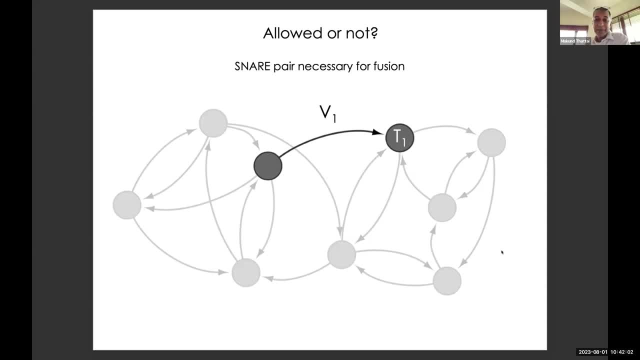 which I find quite fascinating, just as an abstract problem. Okay, so back to details. So there we go. So you are now the setup: V1 loves T1, but V1 has to go back. But if it does go back, 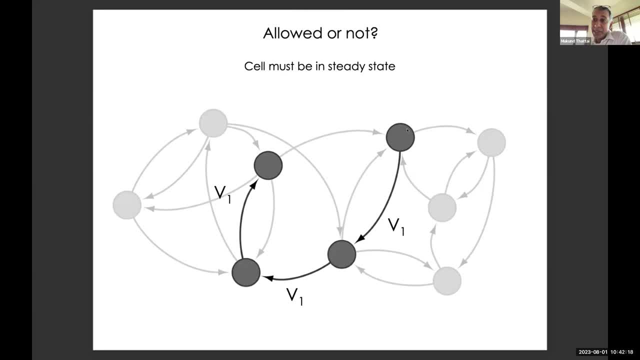 this vesicle will fuse back here. So to prevent that, we're going to pause it. I'm just going to make it up an inhibitor And we're going to say that the inhibitor complexes with V1 to make it inert. So then you don't have a problem. 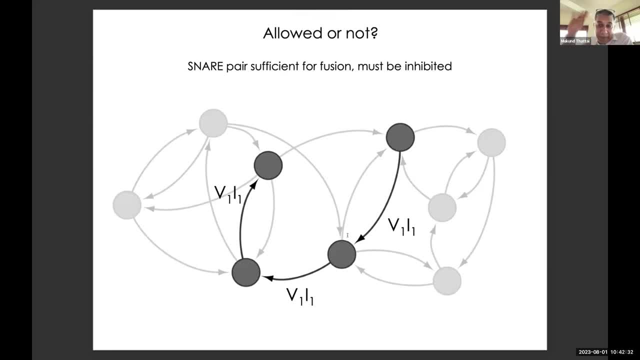 Of course, you also have to have another V-snare, another T-snare here. Those are all happening in the background, okay, But for the moment I've got this V and inhibitor coming up to here, So it's great. 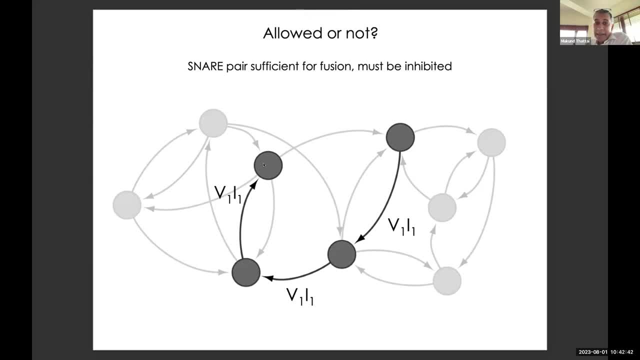 Now I've delivered the V to the starting point And now I can use the V again. But do you see the next problem? The inhibitor has to go back to its source node, which is the target node of V. How does the inhibitor go back? 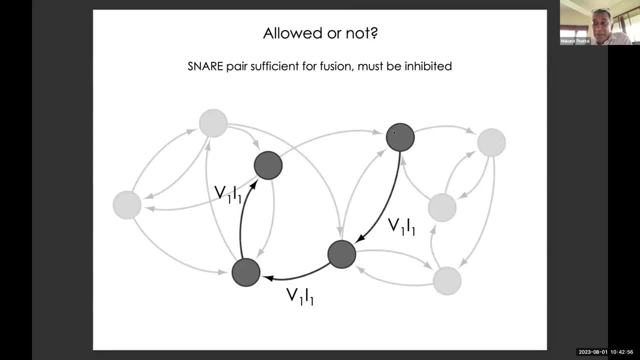 It can't go back on the same vesicle as V, because then it would inhibit V and it couldn't fuse, And so that would you know. you go back to zero, right? So the inhibitor has to go back. It has to go back some other way. 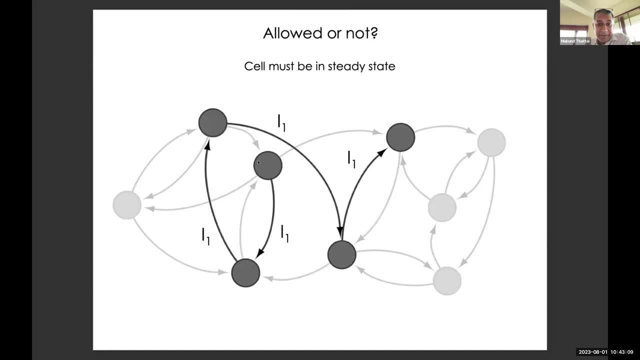 Is that possible? Let's see. Well, here's a crazy path From here. there's, Yes, the inhibitor can go back, And so now we have a full system. Just to explain the fusion of this vesicle to this target. 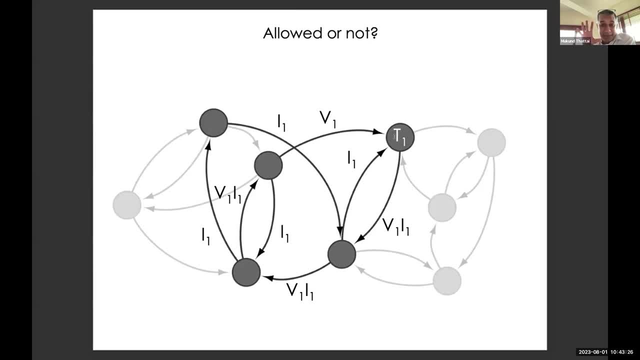 you've now invoked this large subcomponent of the whole cell Right, And now we've got to do this for every vesicle fusion again, and again and again. Let's try another one. Here's a vesicle that contains V2, binds to target T2.. 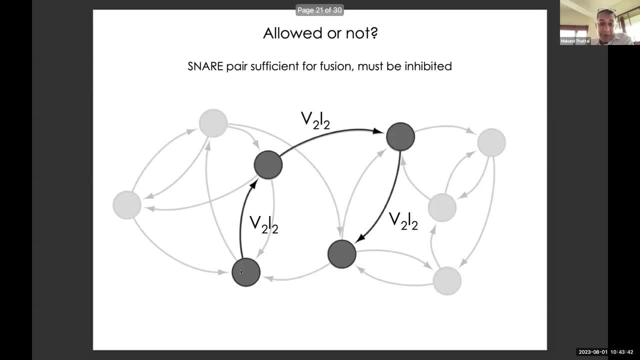 Cool, Okay, now you send the V2 back. Same problem. Why doesn't it refuse? You make an inhibitor- I2, which comes back Great. And now the inhibitor has to come back to the source. Now you're in trouble. 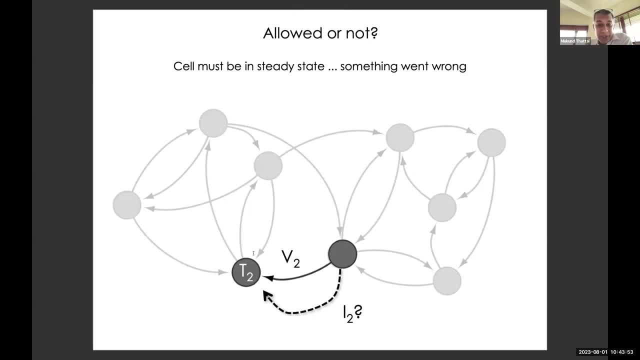 because there is no route from here to here other than this vesicle. This may not have been obvious when you first drew this diagram. Now it suddenly becomes obvious that if this is the diagram that you think is happening inside the cell, and it is this inhibitor, 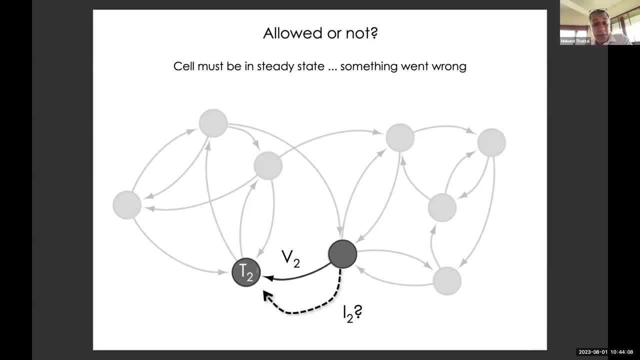 and this is the hypothesis. it can't explain what's going on here And, you see, we have to work quite hard to discover this gap in this model. Yeah, Something went wrong And I could give you this and you could play. 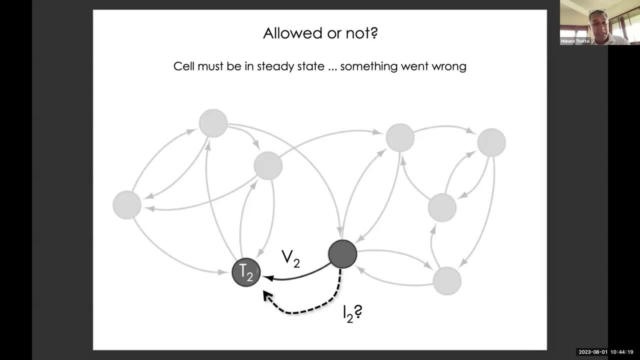 And this is how I first came up with these patterns. right, We played and played and said: could we make it work, Could we make it work, Could we make it work? And sometimes we could and sometimes we couldn't. So does everybody see why this failed? 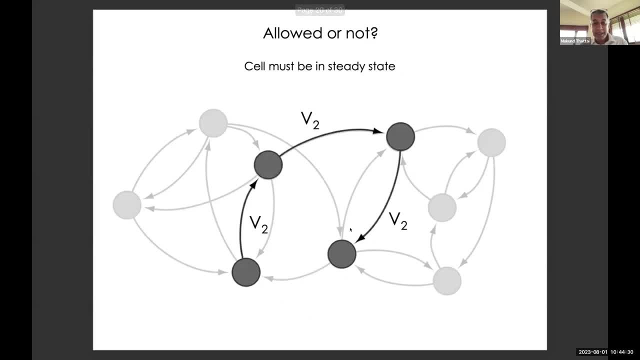 Same game we played, V2.. V2 has to go back, It has to be inhibited, The inhibitor has to come here and, if you notice, there are no arrows that go from this guy back to that guy, Because if I make a cut across this plane, 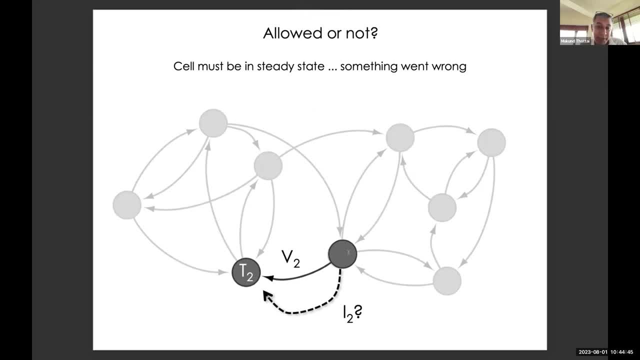 you see that two arrows come back and only one arrow goes forward. So you know there's no way to go from here to here apart from this. Okay, Any questions? So that's neat, right. So we want to now generalize from this little puzzle that we started with. 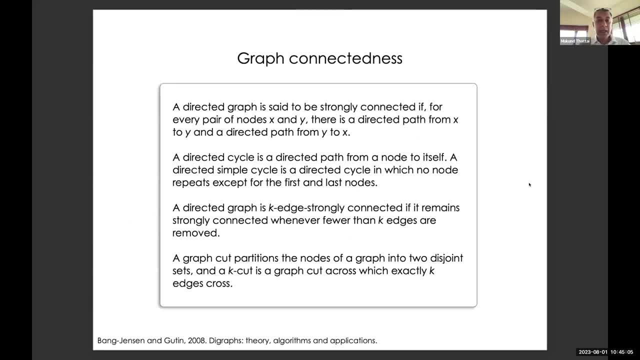 Okay, So for this I'm going to teach you a bit of graph theory, So bear with me, but it is fairly simple. So a directed graph, right? A directed graph has many features. So if the nodes are labeled as X and Y, it's called strongly connected. 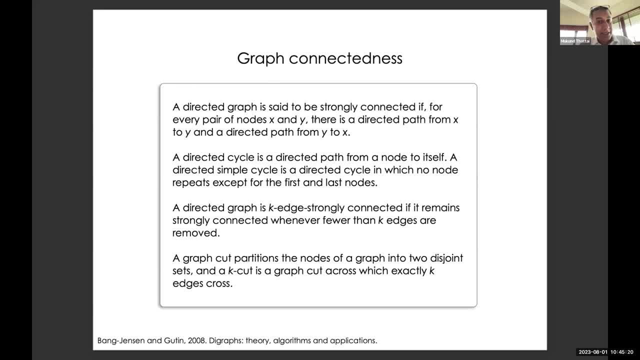 if you can go from anywhere to anywhere else by a directed path, If it's strongly connected, then there are cycles, There are ways to actually go in a cyclic pathway through the whole system, And then there are these two very important features which I'm going to stress on. 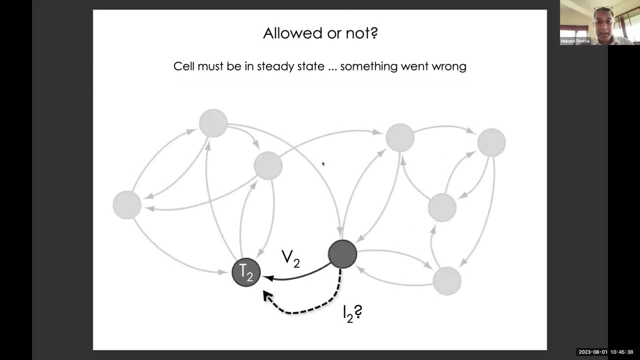 Remember what I said here. I cut, if you can see my cursor. I cut across the midplane here And I noticed that three edges of the graph cross my cut: Two in one direction, one in the other, And if you try and keep on cutting this graph, 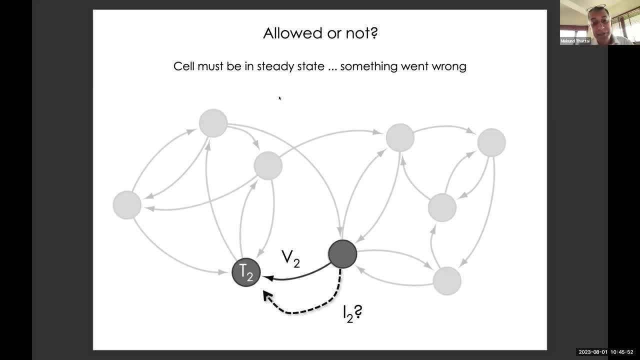 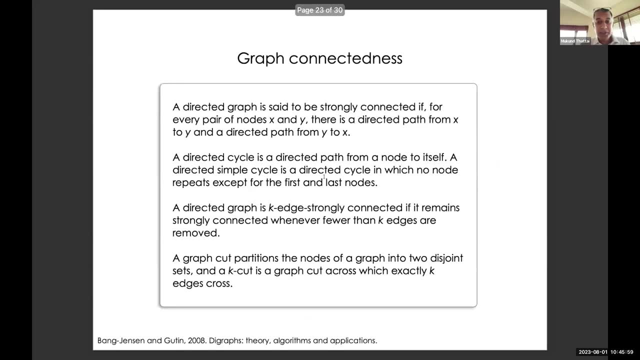 you'll find that every other cut either just doesn't go through the graph or it cuts three or more edges. So by cutting these three edges I can disconnect the graph. So this graph has a connectedness of three, And the more edges a graph has, the more its connectedness tends to be. 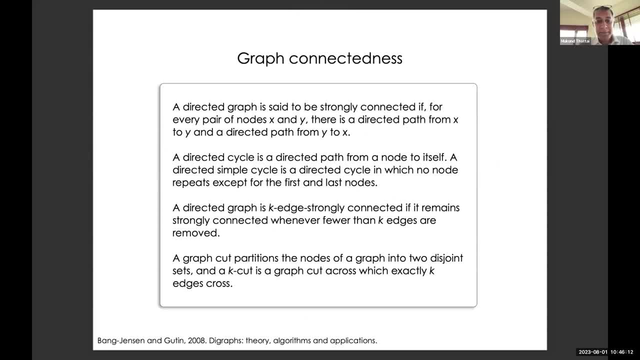 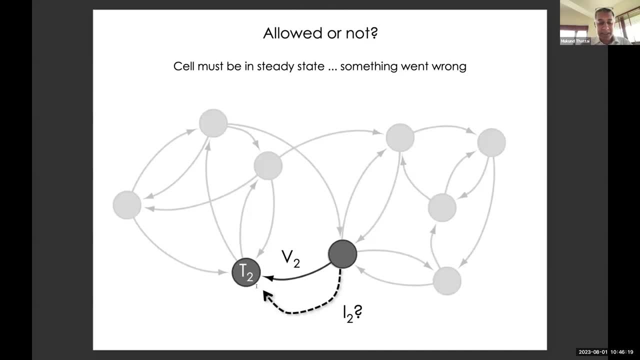 So this turns out to be an important feature. Yeah, Are there any questions about graph connectedness? So the way you find graph connectedness is: you make all possible cuts and you find the cut that has the least number of edges crossing it. 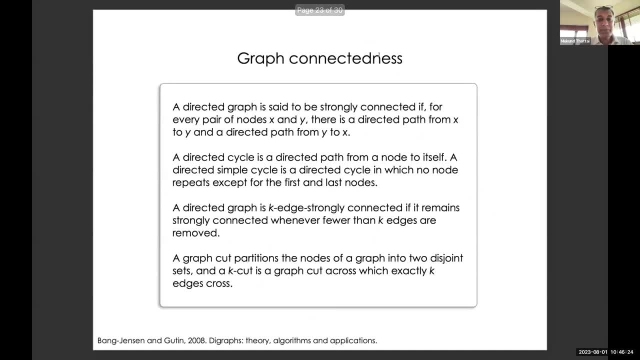 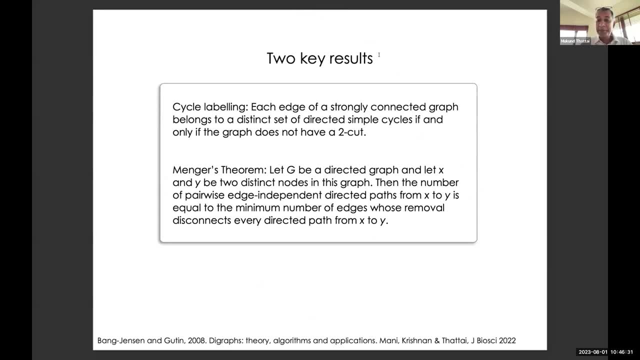 In this case it's three. OK, So there's a little theorem which is from the 19. 70s, called Menger's theorem, And you'll see why it's related to what we're talking about, right. 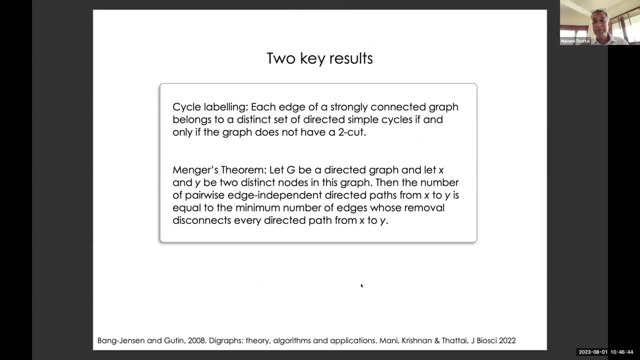 This graph cuts, graph connectedness are all fairly abstract, And this is the theorem that connects all this abstract stuff to a real question you may have, And I'm going to read out this theorem. Let G be a directed graph. Let X and Y be two distinct nodes of this graph. 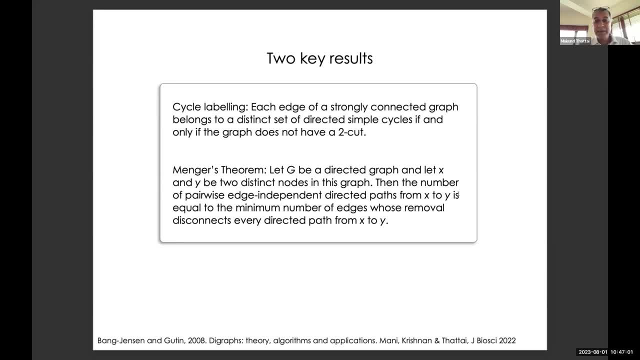 Then the number of pairwise edge independent directed paths from X to Y is equal to the minimum number of edges whose removal disconnects every directed path from edge X to Y. OK, So very complicated statement, But we can unpack it. We're going to pick two nodes, X and Y. 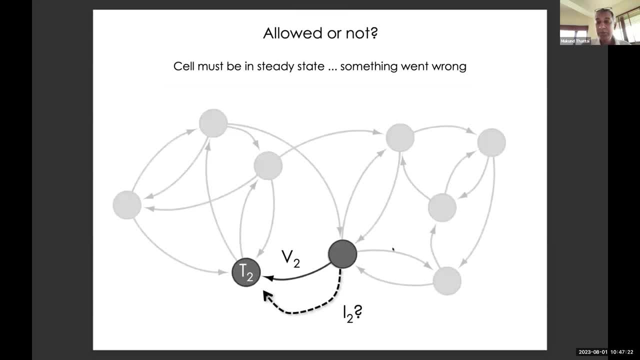 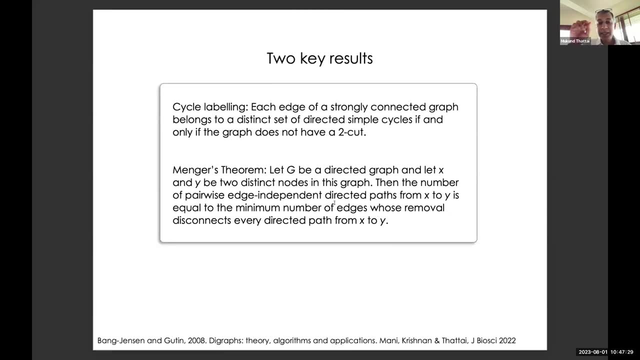 So, for example, this node is X, this node is Y, And what we're going to do is we're going to try and see how many edges you have to remove to disconnect directed paths from X to Y, And this is a very complicated statement. 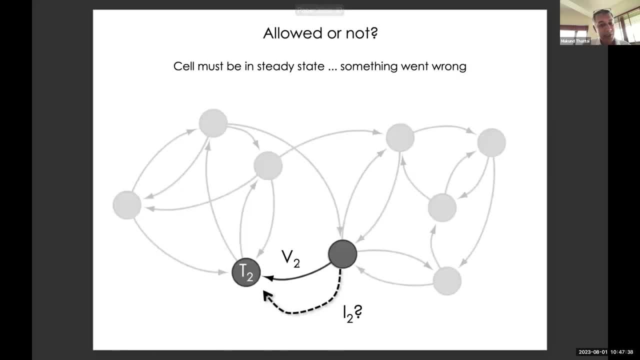 In this case, whoops wrong way around. In this case, you have to remove just one edge to disconnect directed paths from X to Y. In this case, you actually had to connect. take out two edges. right, I'll go back to the original case. 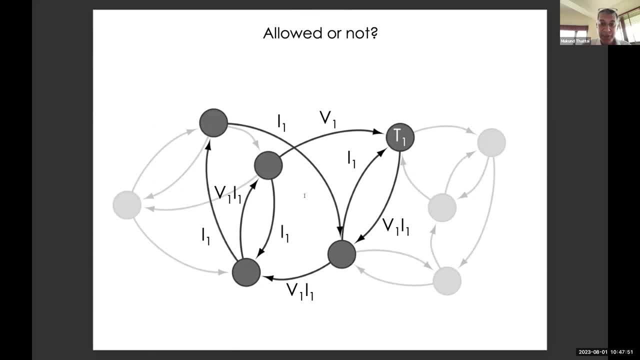 And for if this was X and this was Y, you actually had to take out two edges to remove all directed paths from X to Y. Now here's the thing about Menger's theorem and why it's useful. I know this graph is strongly connected. 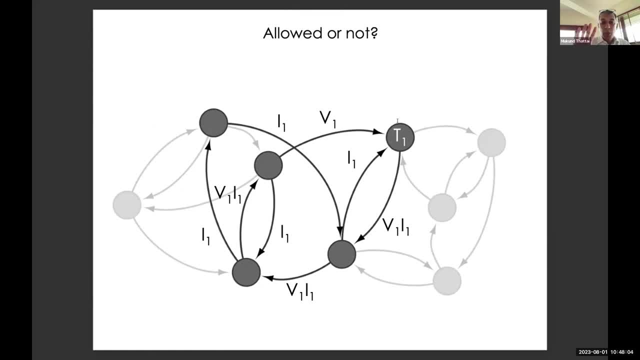 Here is node X, here is node Y, Without even knowing what the paths are to get from here to here. I know that there are two paths that share no edges at all. If I know that, I don't have to know what the paths are. 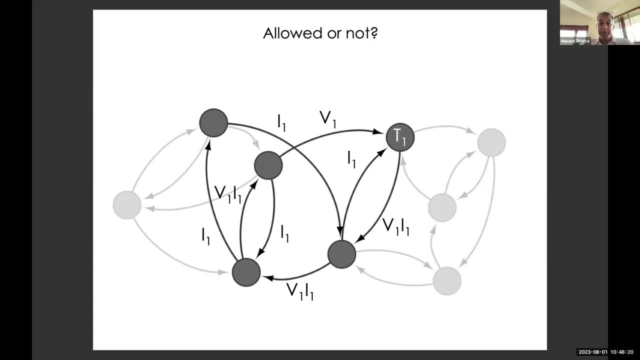 If I know that, then I know I can send I on one of those paths and V on the other, and my job is done. I don't even have to find those paths Right. And that's the real importance of these theorems. 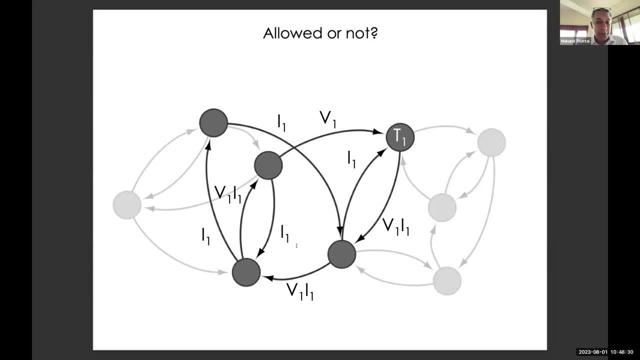 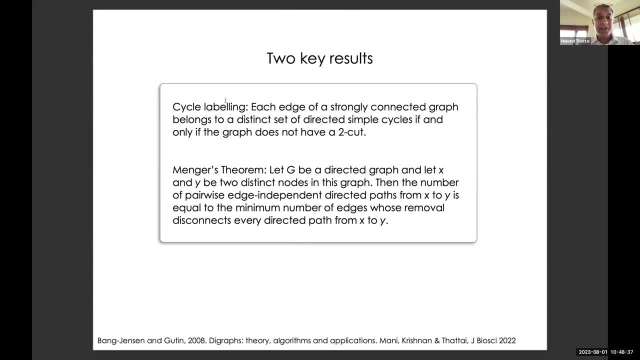 From something simple you can infer something very complicated, So I don't have to play this very complicated game. Okay, There's another theorem which I'll read out. This is actually something we proved. It's not in the literature, as far as I know. 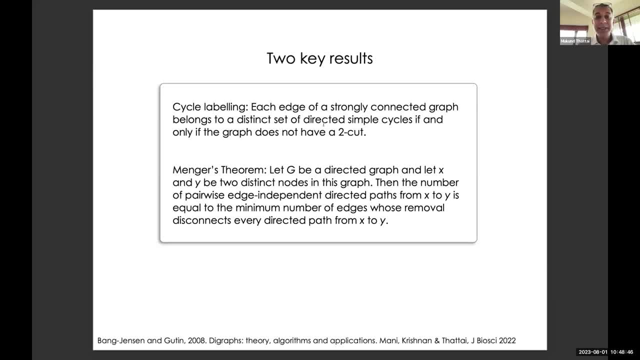 I'll read it out. It'll come back later. Okay, Each edge of a strongly connected graph belongs to a distinct set of cycles. If, and only if, the graph does not have a two-cut. Keep it in mind. I'll come back to it. 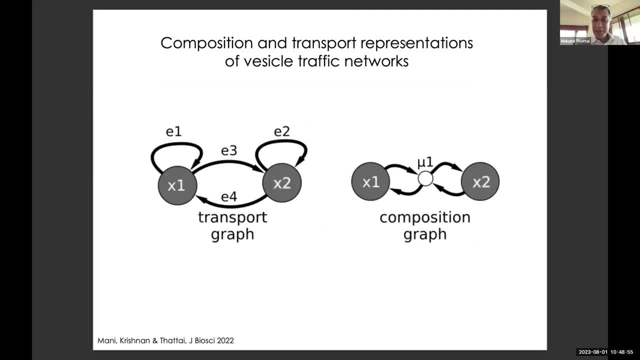 Okay, So I've told you, I've sort of drowned you in cell biology, molecular biology. Now I've given you sort of a textbook's worth of graph theory, Menger's theorem, And now we're going to bring it back together. 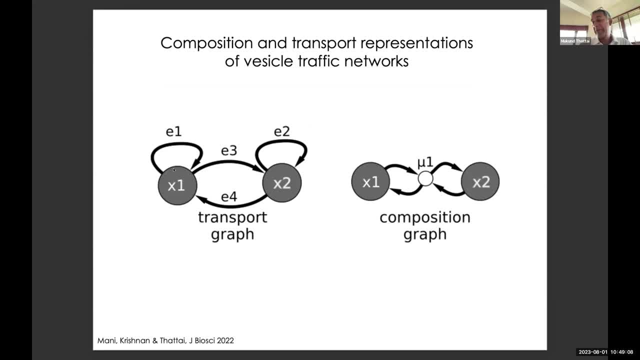 So here again I have my graph which represents the cell. But let's look at something rather simple: two-compartment graph. So here are two compartments. Here are the vesicle edges. Okay, But with one important caveat: the edges represent fluxes. 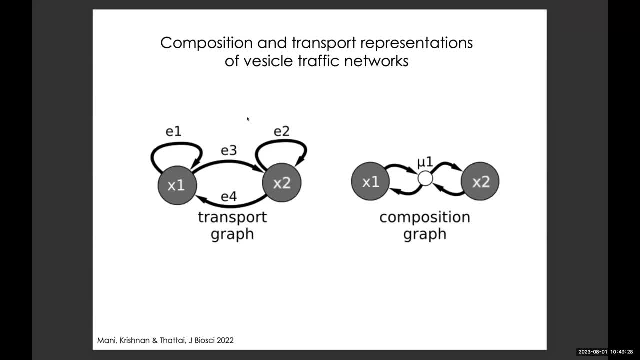 Question: Would it be okay if I interrupt right now, or would you rather I wait? No, please, please interrupt. Okay, We have plenty of time. So if you go back two slides when we were considering the other one, which had yeah, 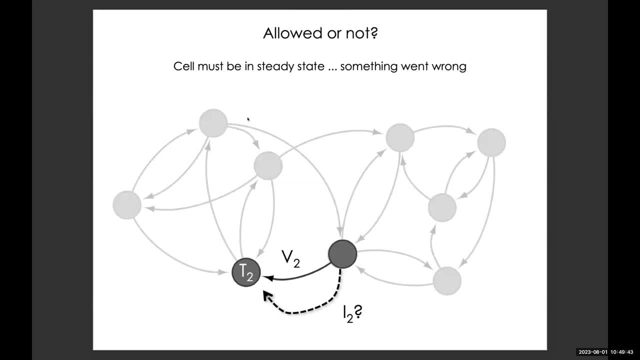 So when we were considering this example where X is V2 and T2 is Y, don't you think this graph is incomplete? I mean, when you said we have to only cut one edge in this case because we haven't taken care of the inhibitor here. 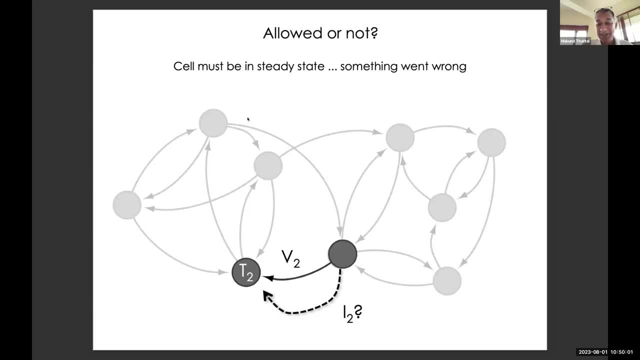 No, no, no, no, no, We indeed have. So this graph is incomplete in the sense- This is the graph you gave me and I'm saying it doesn't work. So in that sense it is incomplete- that the experiments have not yet figured out how the inhibitor goes back. for the whole thing. 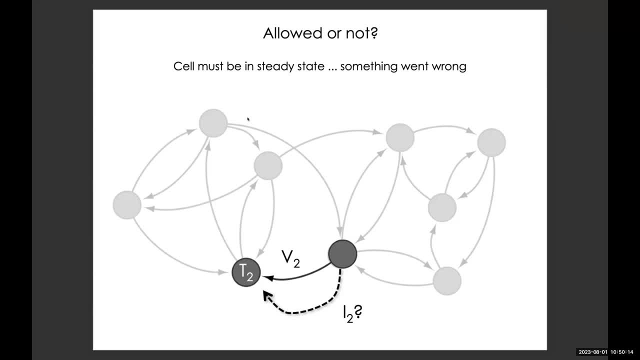 There has to be another way somewhere. Yeah, So are we right in saying that we have to cut only one edge at this point, Because then there would be two edges that we would be cutting. No, no, So the dotted edge doesn't exist. 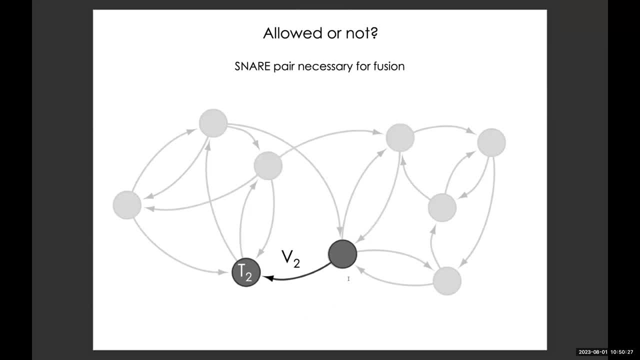 There is no dotted edge, But when we were, I mean I don't get why then the? if we take V1 and T1 as X and Y, we're cutting two edges, Yeah, And that's why you see what happens here. 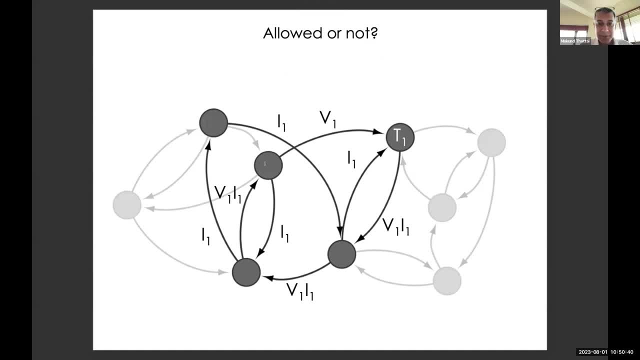 There's a cycle that V follows. I'm going to draw it out with this cursor. There's a rather complicated cycle that I follows There and there, Yeah, Yeah, And the reason that V and I accept the one place where you wanted it can go on different cycles is because of these two edges here, both going from left to right. 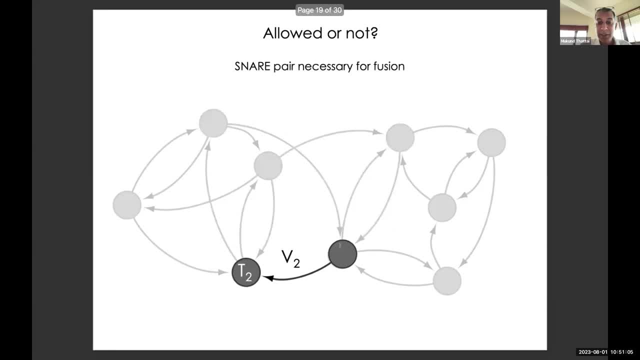 It turns out, if you wanted to play the same game with V2 and I2, there's only one edge going this way. So there's no way at one level. Obviously there's no way to send it on two different paths from this to here. 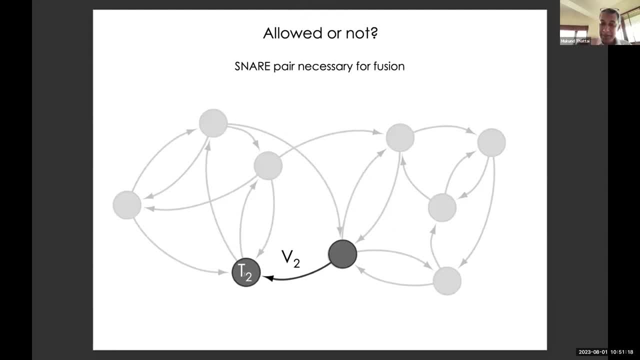 Now what Mengel's theorem says is the other direction. If there are two edges, you can always find a cycle. That turns out to be the hard part of proving that theorem. The easy part is obvious If there's only one way to go from this side to that side, because if I just draw a line across here, there's only one trip, that's going from right to left. 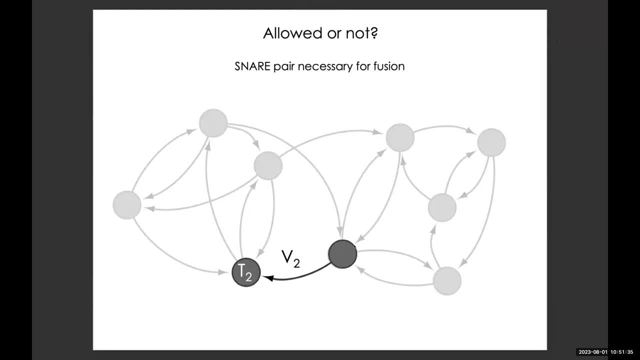 It's on this bus. So if you want to send any molecules from right to left, you better be going on this bus. And yet we know that I2 and V2 cannot go on the same. So that's the contradiction, Right. 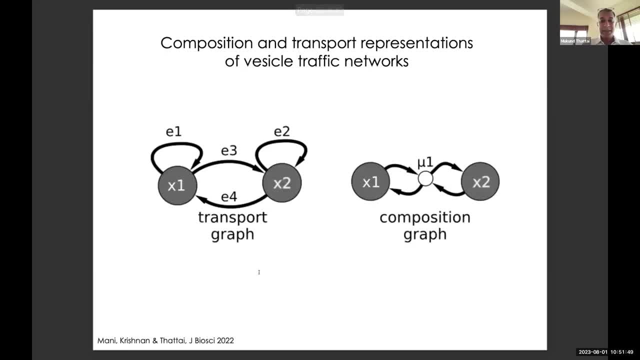 Thank you. Okay. So here we have two kinds of graphs. I'm just showing the fluxes. These fluxes are on edges E1, E2, E3, E4 and two compartments, X1, X2.. Just keep in mind. 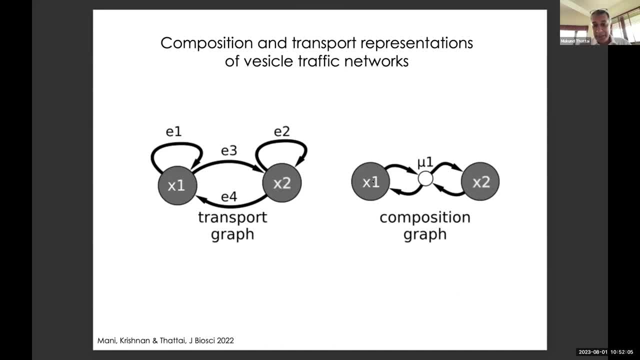 In mind, though, that the same vesicle. it could be, for example, that this compartment makes a vesicle, that compartment makes a vesicle of the same composition, and this vesicle fuses back to both compartments. It's the sort of most degenerate case you can imagine. 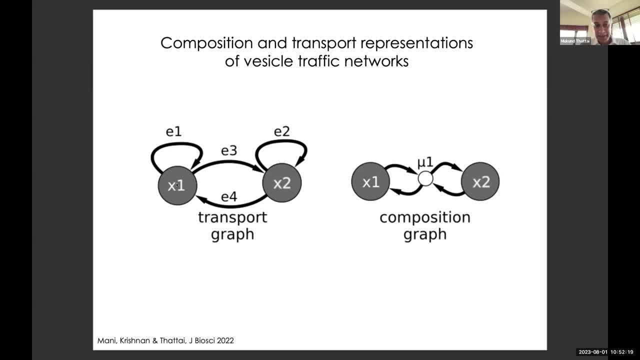 The fluxes from this. there are actually four fluxes: one to one, one to two, two to two and two to one, even though there's only one vesicle type. It's just a detail you may have to keep in mind, but we're going to focus on these transport graphs. 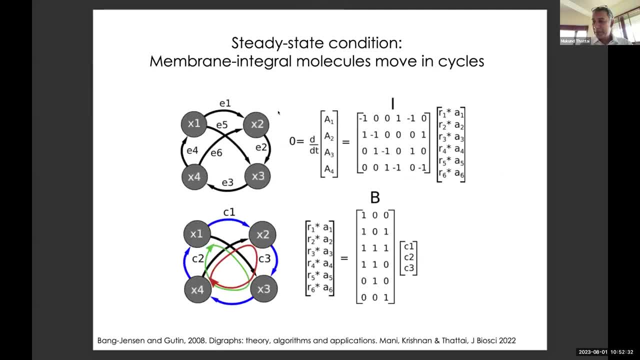 Okay, So this: now you need the tiniest amount of linear algebra to follow what I'm saying, And even if you don't remember it, I'll just remind you how all this works. So it comes back to this issue that Ranjith asked about fluxes. 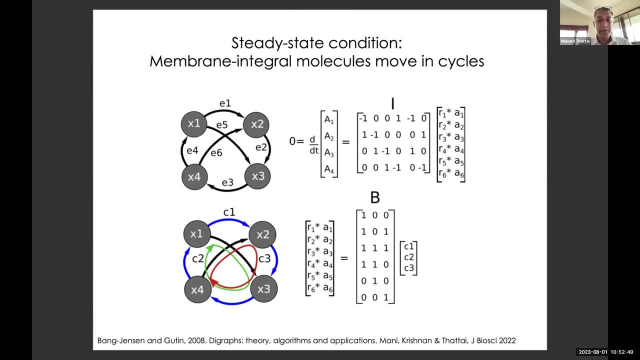 So now I'm going to have a hypothetical cell that has four compartments: X1, X2, X3 and X4. And my hypothetical cell has six edges: E1, E2, E3, E4, E5, E6, just so, and there are no other vesicle edges and there are no other compartments. 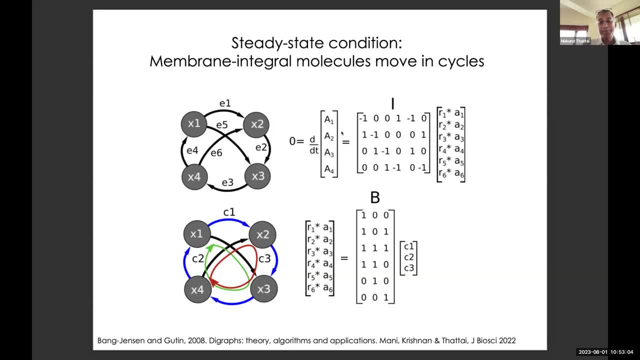 And now I take some molecule A and I say that the amount of A on each of these compartments is called capital A1, capital A2, capital A3, capital A4. And the amount of that A on each of the vesicle edges is little: a1, a2, a3, a4, a5, a6 per vesicle. 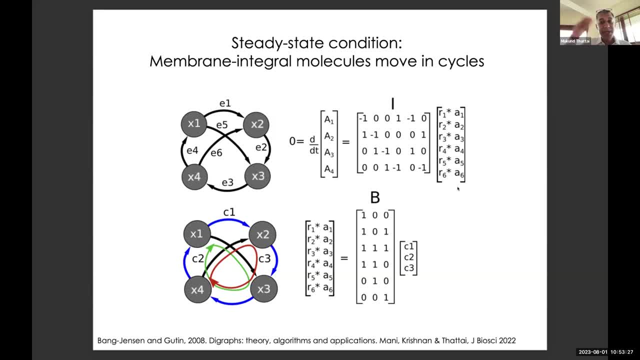 And of course the vesicles move right. So there's a rate, let's say, 10 vesicles per minute crossing each edge. So the total amount of molecule A that crosses on edge one is that rate of vesicle, one times the amount of molecule one molecule A it contains. 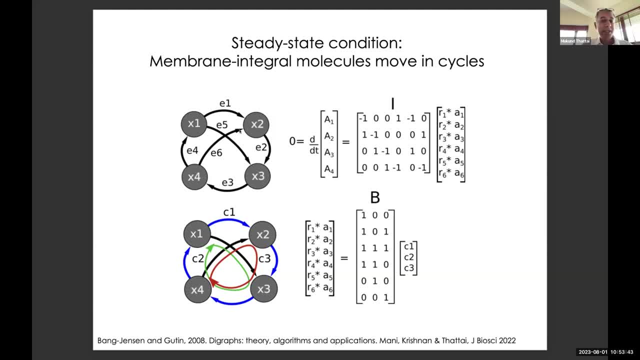 And similarly for all the other rates. So you can write down the steady state equation. This is sort of the first day of linear algebra. You'd write down something like this, And so let me write it down explicitly. DDT of A1, first equation is minus R1 times A1,. 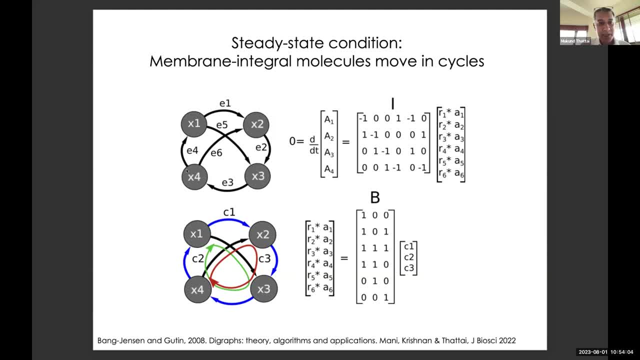 minus R5 times A5, plus R4 times A4.. That's the two outward edges, one inward edge. You see this, Minus on edge one, plus on edge four, minus on edge five. That's the first row. 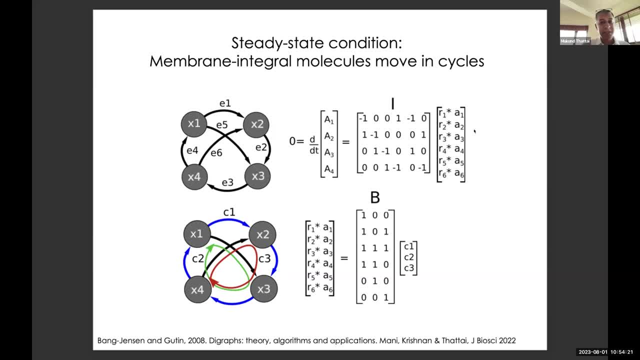 And so you multiply this row by this column to write the first differential equation. Second differential equation: similarly, I'll just go through this explicitly: X2, there are two incoming and one outgoing. One and five are incoming, two is outgoing. 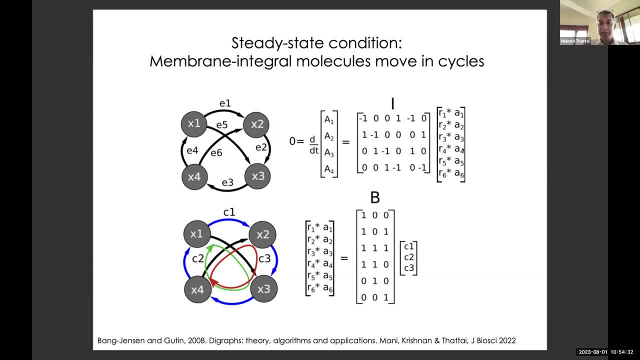 Is that correct? Yes, One. One and five are incoming, two is outgoing. That's the equation. So you write all this down. This is the connectivity matrix of the graph, And so I'm just conveniently writing this as a matrix. 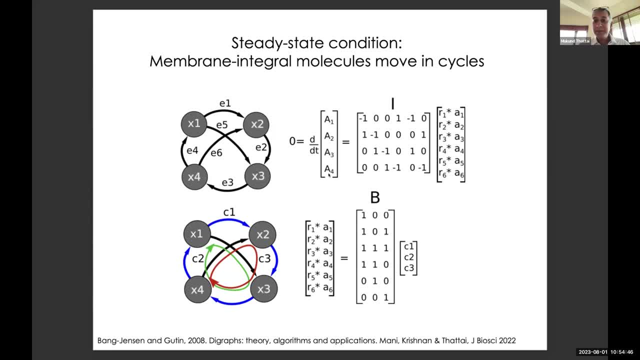 but this is just four differential equations, And this set of equations sets up a condition. It says that if you want me to be in steady state, so the left side has to be equal to zero, I'm assuming- then this matrix multiplication has to go to zero. 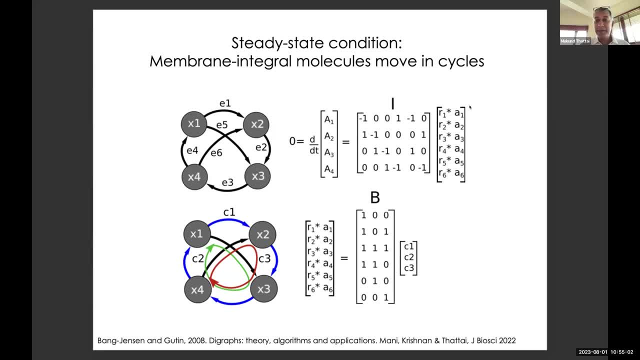 Another way to say this, if you remember linear algebra, is that this six-dimensional vector has to be in the null space of this matrix, the kernel of the matrix. The matrix has to project it to zero. And now you can show that if the matrix represents a strongly connected graph, 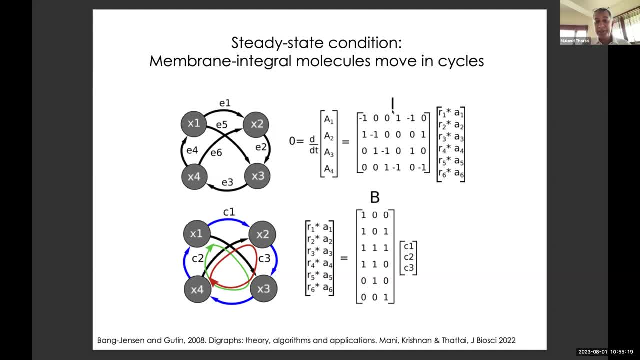 the only way to be in the null space of the matrix. the null space of the matrix. a little trick for those of you who remember your linear algebra: you can solve this problem And there's something that you can use- It's called the rank nullity formula- to figure out that. 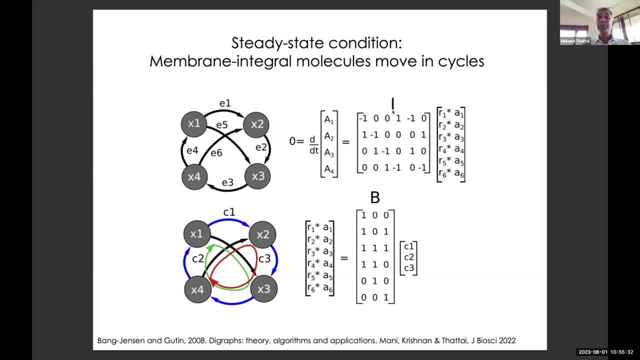 okay, dimensionality of the null space okay, And it's all cool stuff. The only fly in the ointment here is that all these numbers are positive. So this is a slightly more difficult than standard linear algebra, where things can be positive or negative. 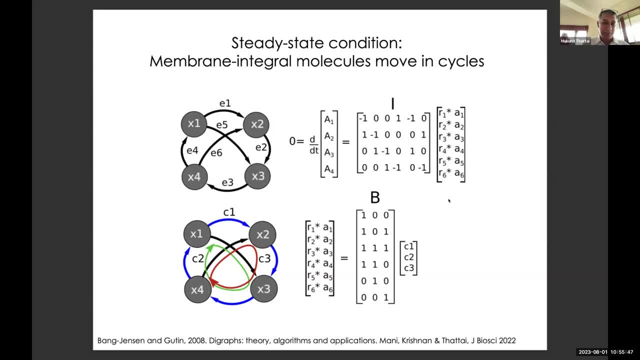 Here. all my rates and concentrations and quantities have to be positive. So if I put that condition, the answer turns out to be very simple and intuitive, and you didn't have to use all this math to believe me. The only way that a single molecule can 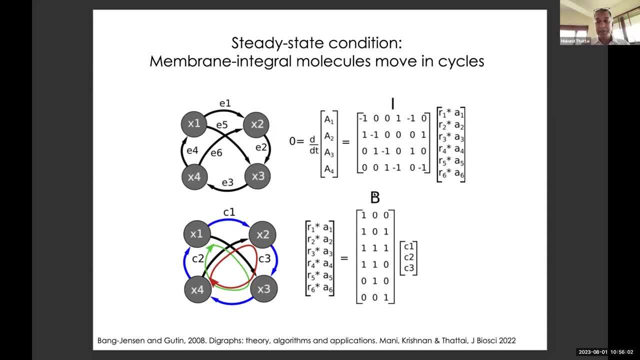 can be in steady state throughout the system is if that molecule moves in cycles, Right. So, for example, it can move on this blue cycle or on this green cycle or on this red cycle and there are no other cycles, Turns out in this system. 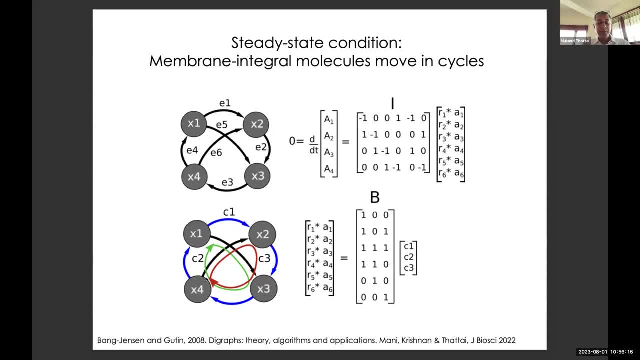 there are only three cycles. There are ways to compute how many cycles there are. So, just to be clear, this molecule will have a flux which is represented by the sum of all the three cycles. So if it was equal amount on the red. 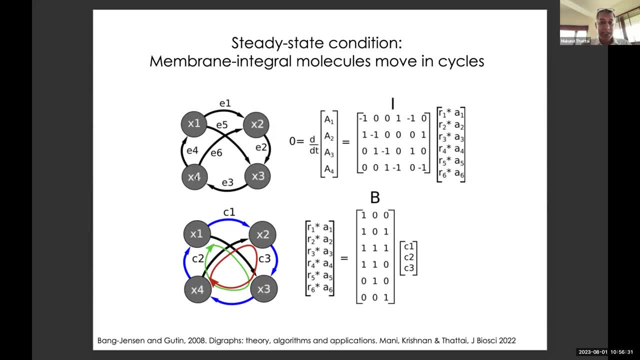 the green and the blue cycle, then three units of it would go across edge three, because all three cycles cross here, but only one unit would cross across edge one. Two units would cross across edge two and two across here, and one each. 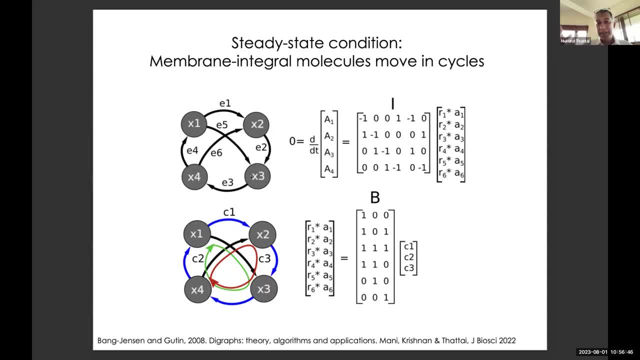 Okay, So you can see the point. For a graph like this to be in steady state, all the molecules have to go in cycles. Any questions about this? It's a very simple statement. Okay, It turns out to be slightly niggly to prove. 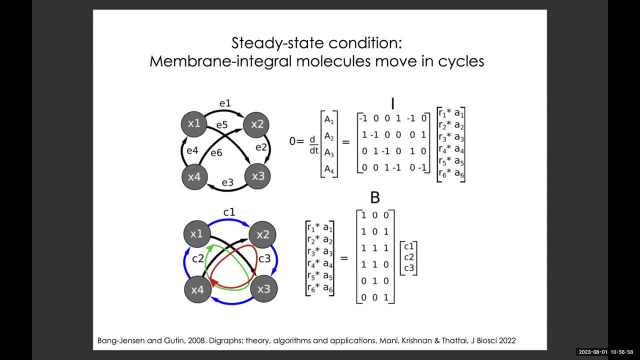 but it's a very simple statement. Any questions? Okay, So a corollary. corollary is that if there are no cycles, we can conclude that that molecule is not in steady state, right? Either it's like being depleted or enriched. 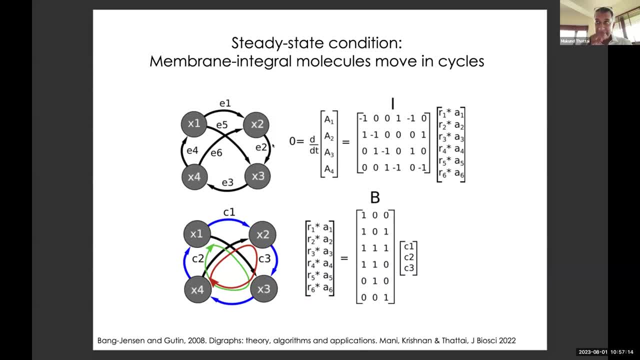 Sure So, and so the more general statement is that you either travel in cycles or you have source sync balance terms that are one-to-one connected or connected in a directed way. That's the most general steady state condition, But in this case, where we're looking at snare proteins, 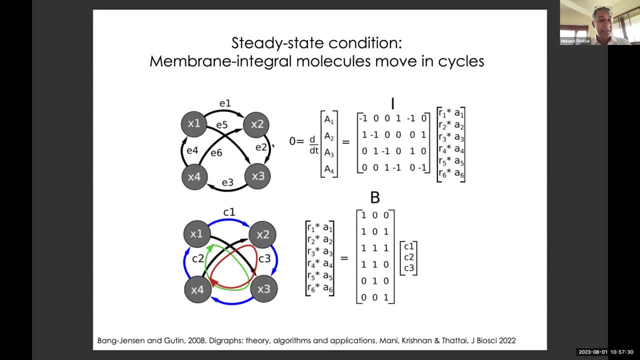 which tend to be created at very low rates and hardly degraded at all. they go around a hundred times before they get degraded. So it's a very good approximation. And the same statement is true for every molecule in this cell. So every molecule in the cell can only move on linear combinations of. 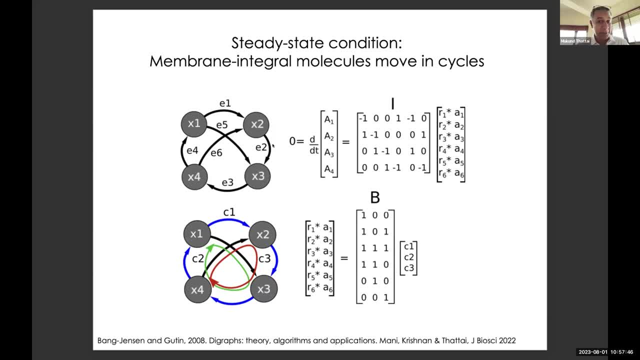 cycles, Okay, And there are thousands of molecules. You may worry where the cycles exist. So it turns out, if your graph is strongly connected, there are cycles, There is a cycle basis for the graph. It's another little theory. Okay, So every molecule can be associated with some linear combination of cycles. 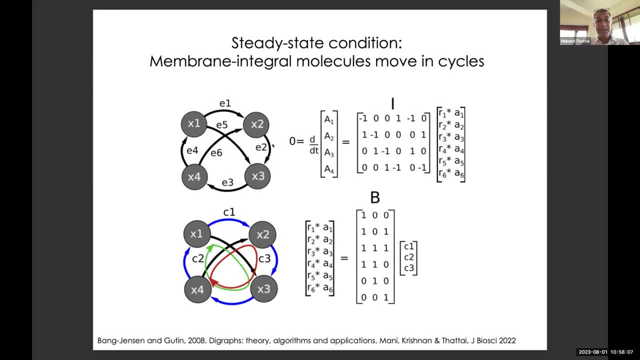 So let me pick three molecules which are as distinct as possible. as possible, Let me take one molecule which is blue in color and only run it on this cycle, And one molecule which is red in color, only run it on this cycle. 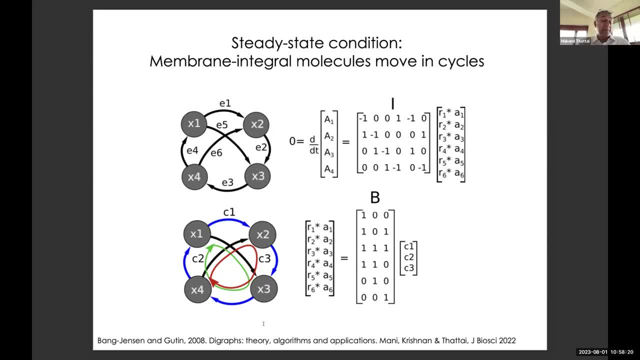 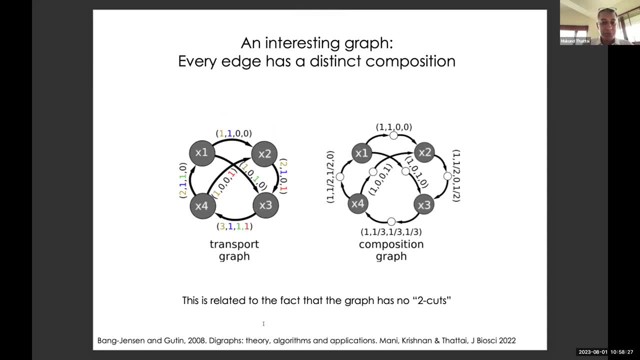 And one molecule which is green in color only run it on that cycle. I'm allowed to do that. I have as many molecules as I want, Okay, And that's the picture I've drawn over here. So I am using a four dimensional vector to represent the composition of each. 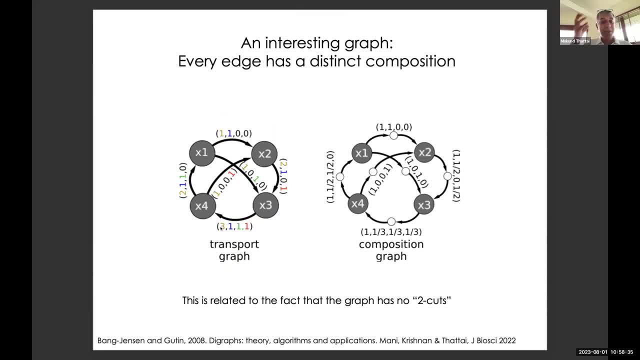 vesicle. The first dimension actually represents how much membrane there is on a vesicle. Okay, So a vesicle needs to be bigger to carry more stuff, So forget that this. the next three represent how much of molecule one, molecule two and molecule. 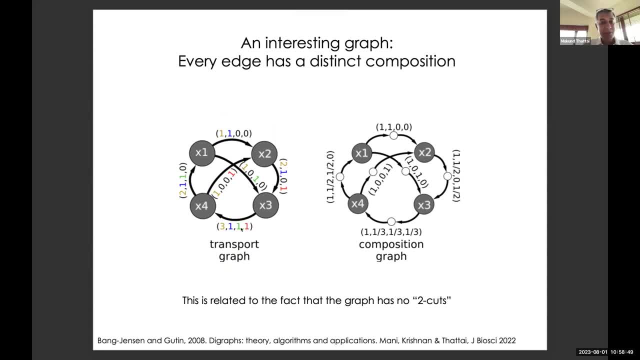 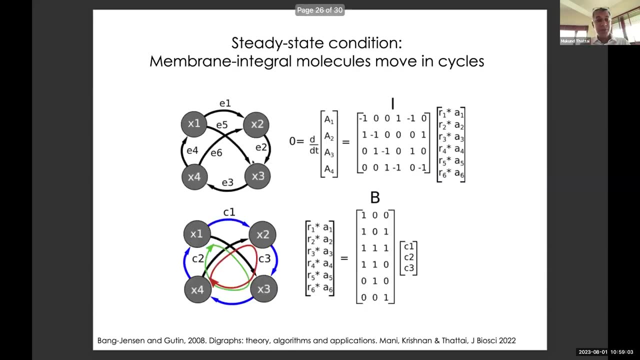 three is carrying. this edge carries all three molecules. that edge carries only one molecule, One. this edge character carries molecules one and two. This one carries- sorry, one and three, one and two, just three and just two. So now I've put on top of what was just a graph. 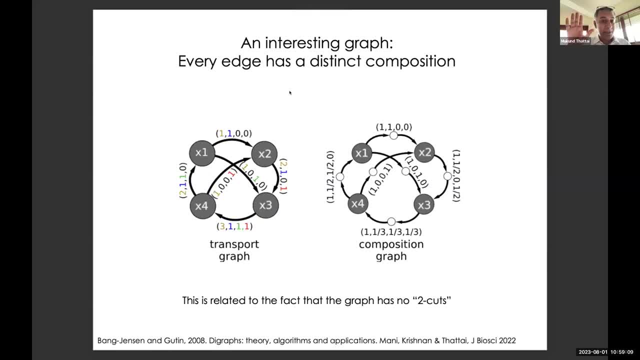 Okay, I've put now vectors of very special time, And these vectors are in the, in the null space of the of the matrix. So you see the beauty of this process, right, You? you take graph theory and suddenly you have the enormous power of. 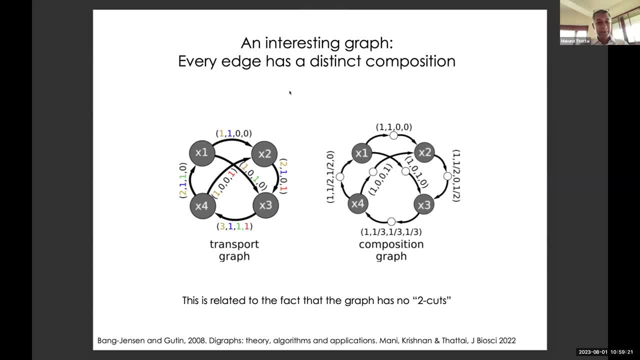 linear algebra to: to save your skin, Okay, Very good. Uh, if I divide the uh, the vesicle, by the membrane size, in some sense to normalize it, I then get the graph on the right, which is actually the vesicular composition of this graph. 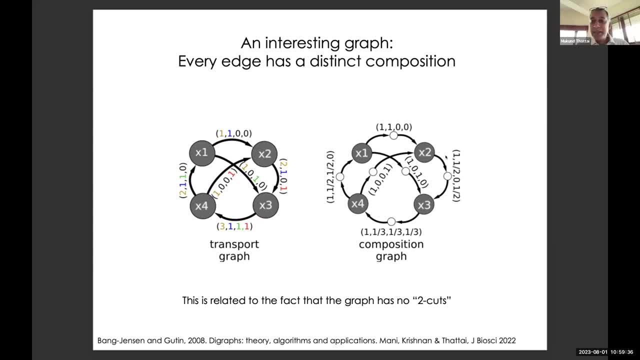 You would not have guessed this upfront, Okay, Uh, that this is the steady state of the system, And so it is sort of fairly complicated. Why is this? half and half, one third, one third, zero and one? it's sort of very. 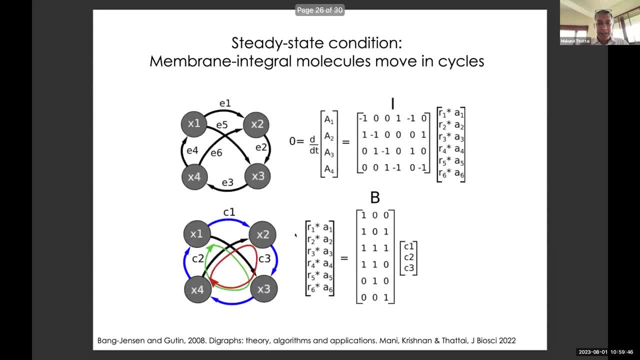 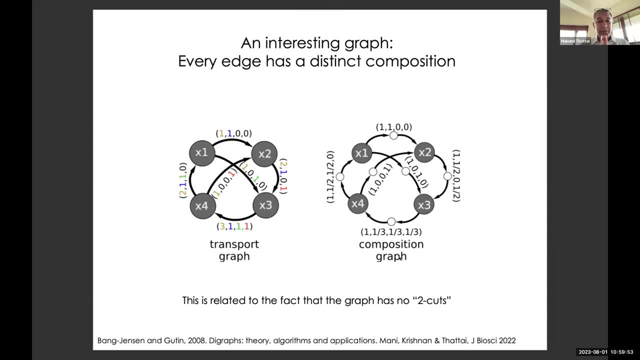 very weird, right? It only becomes natural and obvious if I showed you the cycles, otherwise it's not okay. Now I'm going to bring it back to this. This is all graph theory. I'm bringing it back to the cell biology and bringing it. 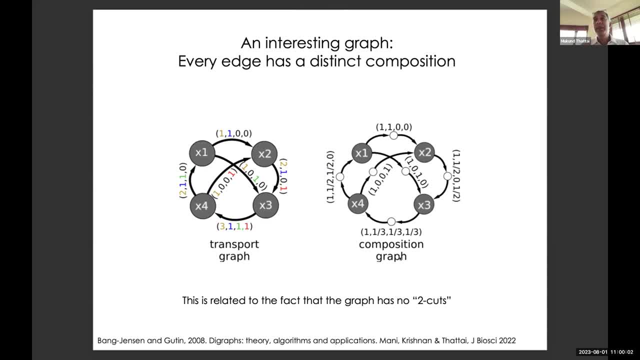 back to the statement I made right at the beginning, which is absolutely true and verified. inside a cell, The properties of a vesicle are determined by its composition. Okay, By assumption, every vesicle here has different properties. This vesicle fuses to this compartment. 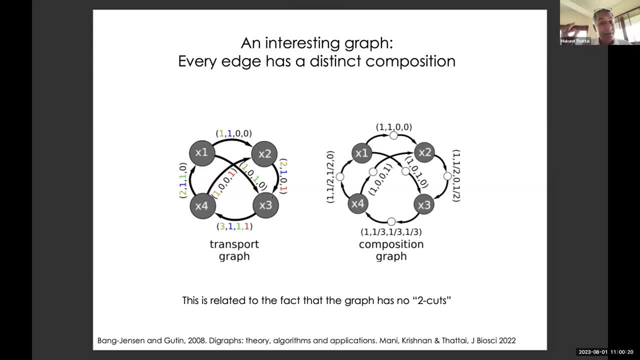 This one fuses to this compartment. This one comes from here and fuses here. They all have different properties. If they all have different properties, they must have different compositions. That's the necessary condition for this whole thing to work out. And if you gaze at this graph, 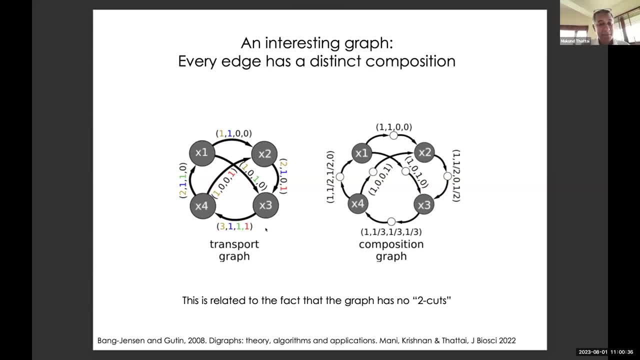 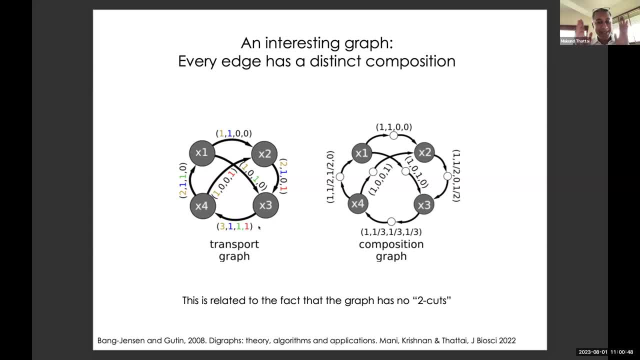 0 and 1: 1, 1.. The six edges have six different binary representations. Okay, And that's neat, because if that's true I can make this whole thing work out. I just say that the molecules are clever enough to know exactly what the full combinatorial composition of the vesicle is. 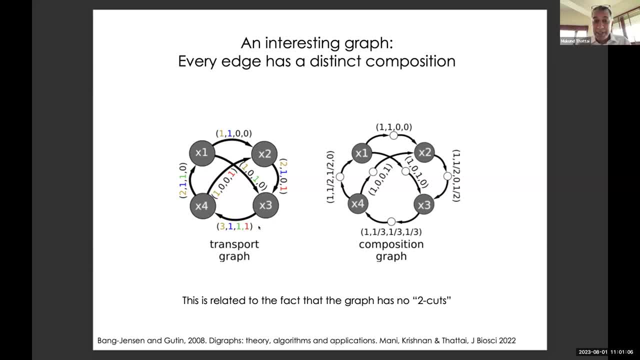 And therefore they can behave differently depending on the composition. The only issue that would have arisen is if two vesicles here ended up having the same composition but behave differently. then we would say we reject this hypothesis. So I've shown you one example of how to do this. 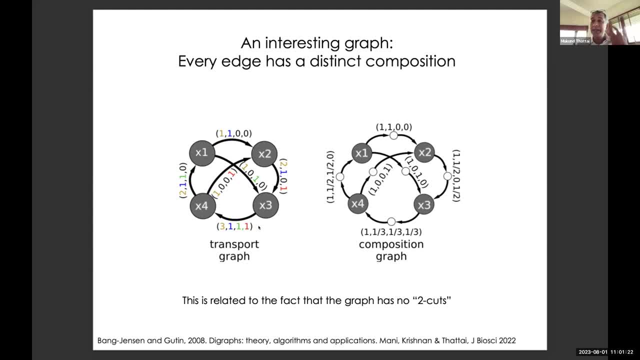 And now the obvious question is: what are the necessary and sufficient conditions to do this? What are all the examples that make this kind of thing work? Okay, so for that, before I get into the more complicated snare business, um, I'm going to tell you what the answer is. 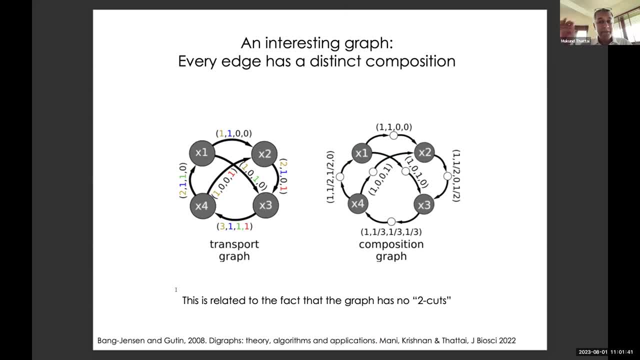 The necessary and sufficient condition for every vesicle on this graph to have a different composition is: the graph has no two cuts. A two cut, remember, is an edge that you cross where always one vesicle is going one way and one is going the other way. 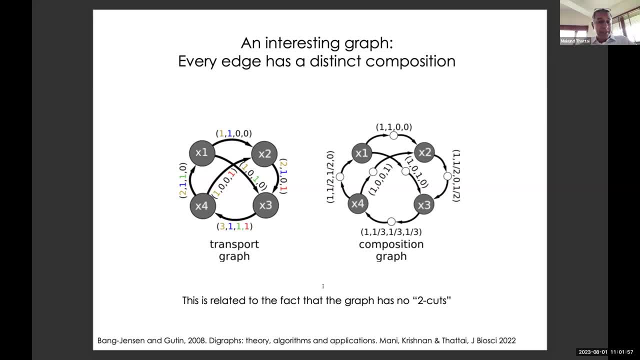 And there are no more edges, because you can remove them, Those two edges, and you disconnect the graph. If the graph had a two cut, for example, if I remove this edge, oh no, that's not, that's not to cut. 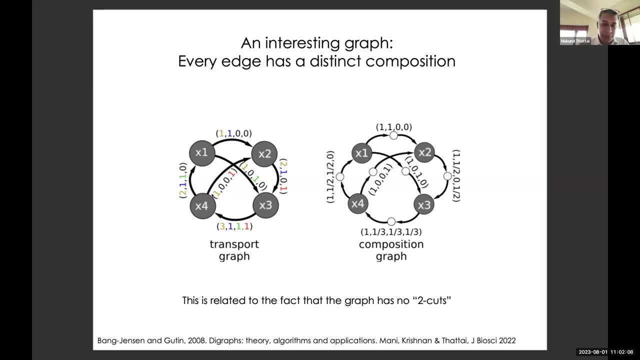 Let me see how to make it to cut here. Uh, okay, that's true, If I remove this uh edge here. no, the graph still has no two cuts. Okay, I think what I have to do is I have to remove this edge. 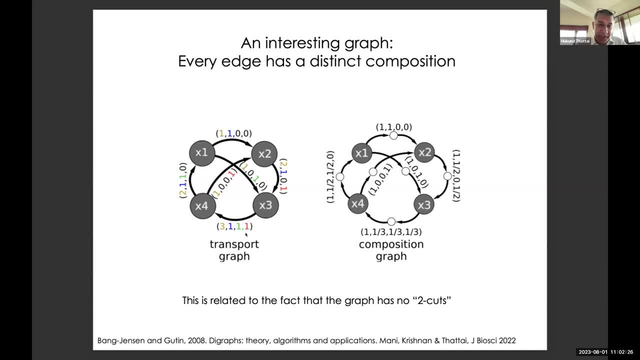 Let me remove this edge, which is the zero, zero one edge. Then you notice that if I make a cut like this, there are only two edges crossing it and that will decouple compartment X- four from the rest of the system. Is that right? 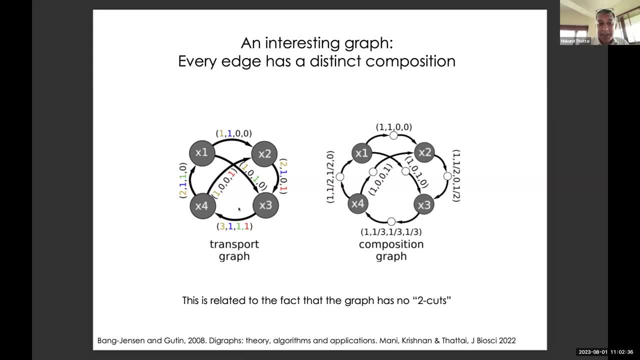 Yeah, Now that system just by the steady state conditions. if you have vesicles coming in here and vesicles going there, obviously the composition of this must be the same as the composition of that to make this compartment in steady state. If they are the same. 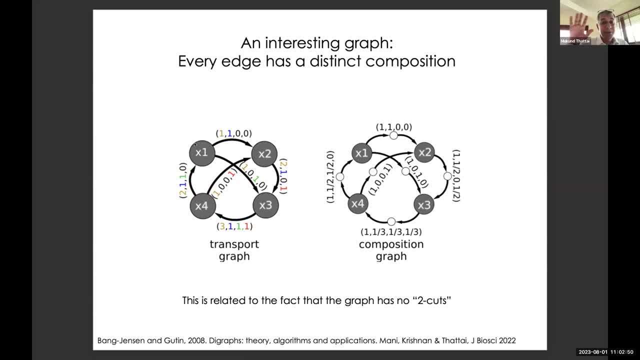 then why is this vesicle behaving from that So obviously? one direction of that theorem is very simple. If it has a two cut, obviously you can't make it work out. That's the same failure we had in the original graph Right. 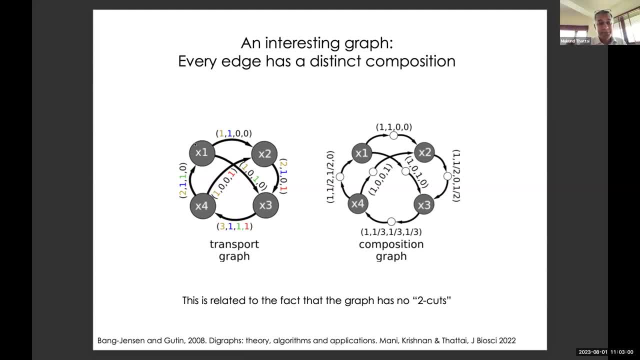 You just can't make every system satisfy these circles. The real difficult part of the theorem, which is the other direction, as usual, is: if it has no two cuts, I can always make it work. It doesn't show you how, but it says the solution exists. and then you have to go and make the solution. 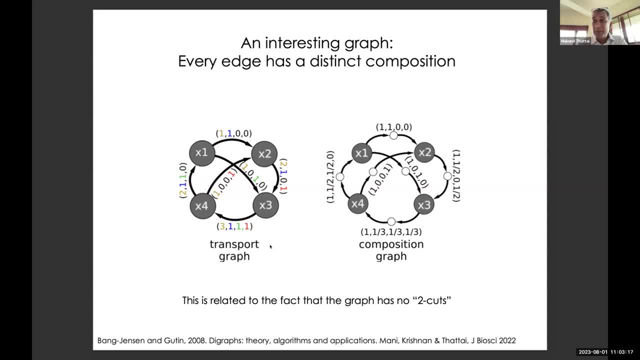 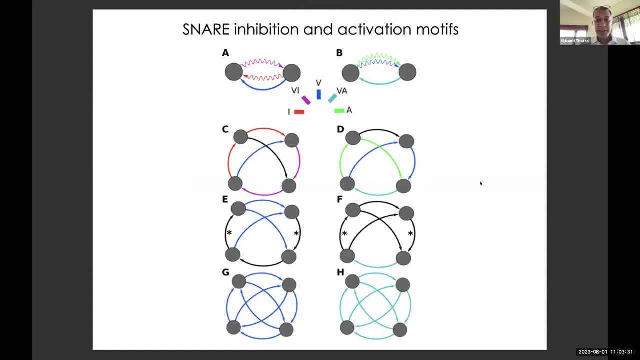 Incidentally, this exact type of result is what you can use to generally solve this wolf, goat and cabbage problem. You can state it in exactly the same way and find very, very similar conditions. Okay, Now, that system which I just talked about is not still close enough to the cell biology. 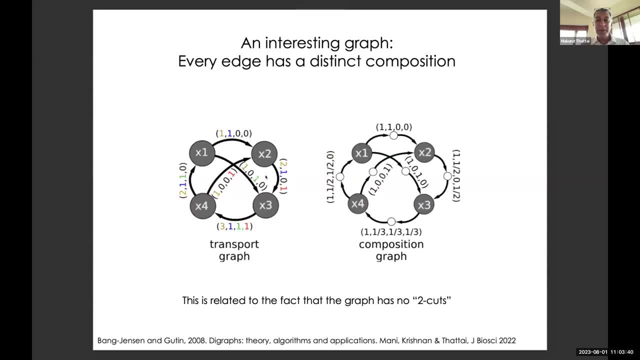 In the system I spoke about here. sure, every vesicle has a distinct composition, but for this to work out, the molecules have to be very clever. They have to be aware of the entire combinatorial composition of the vesicle in order to modulate their own properties. 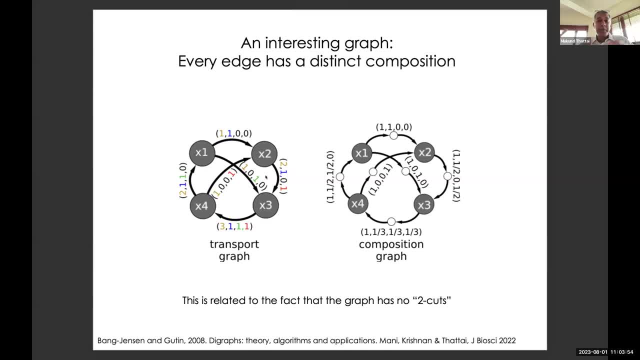 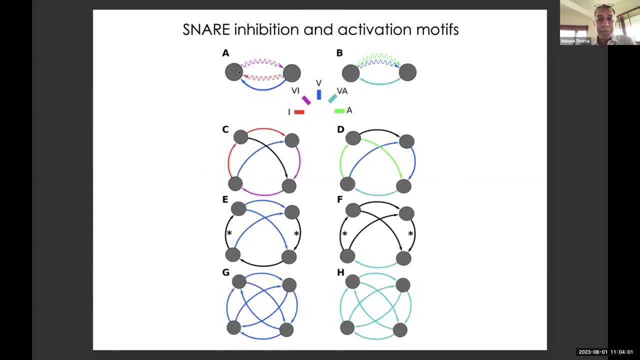 And that maybe is too much to ask for. Molecules typically have one to one partners- Snares, for example. I have that feature. So if you have snares, what's the result? And here's what I'm going to show you. 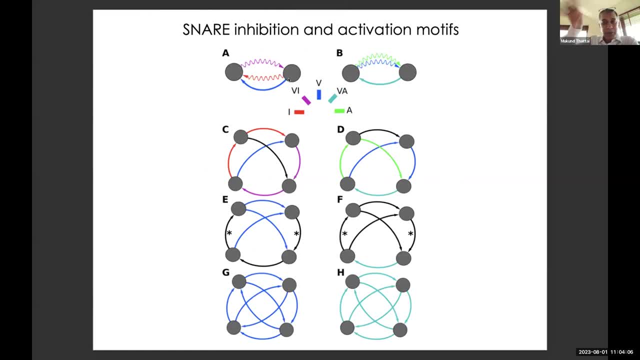 And this relates to the big puzzle that I had possible or impossible, And we went over that puzzle quite a lot. It comes down to a very simple test that you need to do, Okay. So, for example, if I start from the right graph in this case, 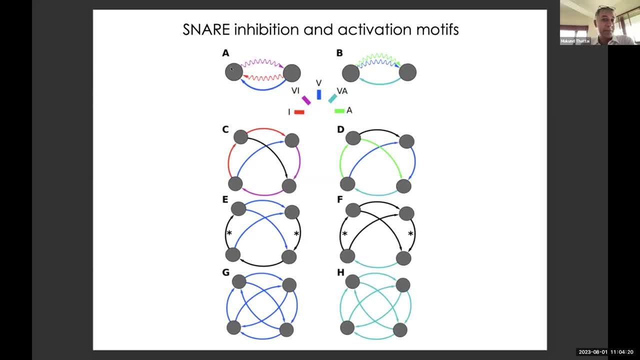 the right node- I'm sorry- and go to the left node on this vesicle and I assume that there's a V-snare that does it And a V-snare with an inhibitor that must travel back somehow through a very long path. 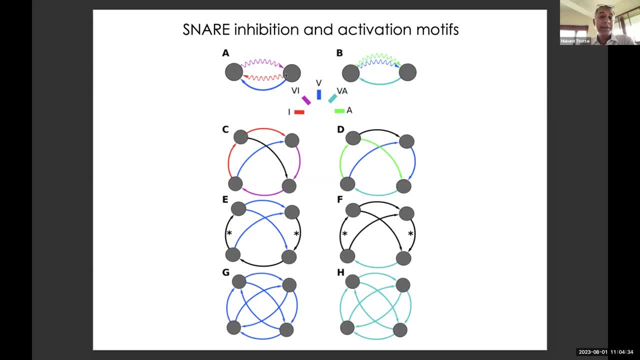 And that's why I've drawn it as a squiggly edge. And the inhibitor is coming back to the original point, to a very long path which I've drawn as another squiggly edge. I don't care about those, They exist throughout the whole set right. 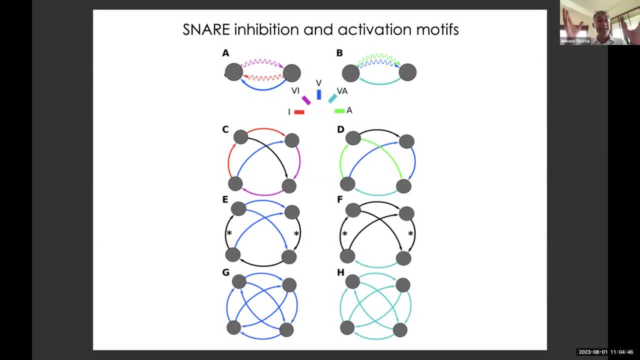 The important thing is to make this work out. It implies those two long paths exist. Okay, So how do I test this? It turns out just like in the previous slide, but I'm not going to prove it over here To test it. 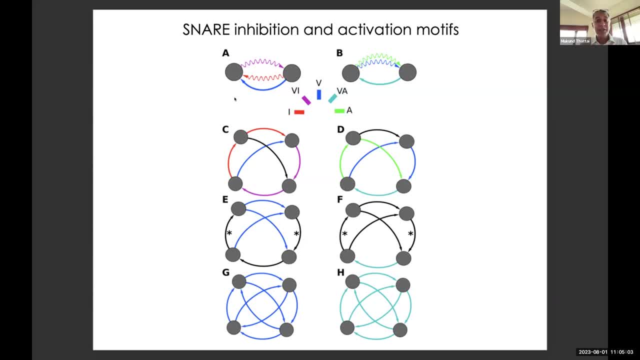 the graph actually has to be. to make it work out, the graph has to be not three connected, but actually four connected. Okay, And the reasons are, you know, a little bit detailed and they don't need too much insight, but let me just finish the story. 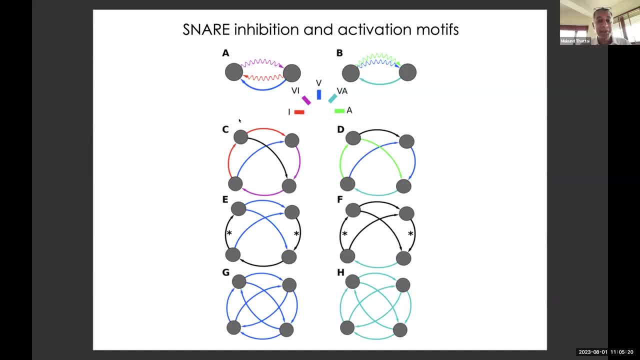 And I'm going to leave some time for questions- Finish the story with this little picture and show you how it can work for the graph that we had in mind. Okay, So, for example, if this is the source node and this is the target node of the blue vesicle, 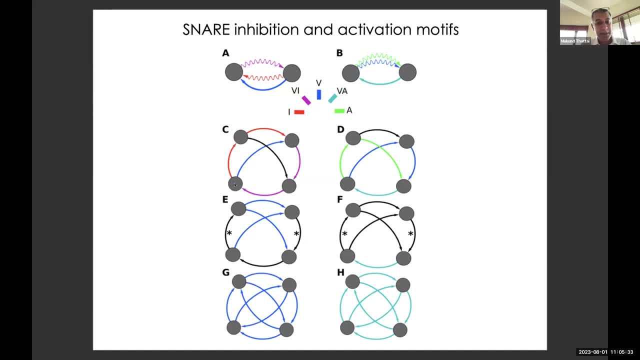 I need the inhibitor and the vesicle and the v-snare to come back on this path And I need just the inhibitor to come on this path. Okay, That's fine, But you have to make that work for every single path, for every v and inhibitor combination. 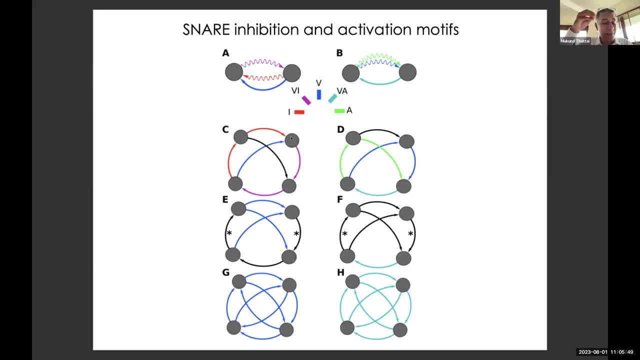 v1 and v2, sorry, v1 and t1 and i1, v2 and t2 and i2, and so on for every edge. I found a way to do it for this edge, but I can't do it for this edge. 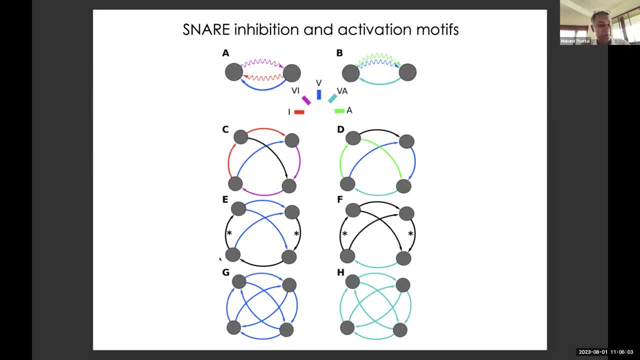 You can just look at it and convince yourself. and I can't do it for this edge. But if I add two more edges to make the graph four connected, not three connected, then I can make this whole thing work. So there's a general theme here. 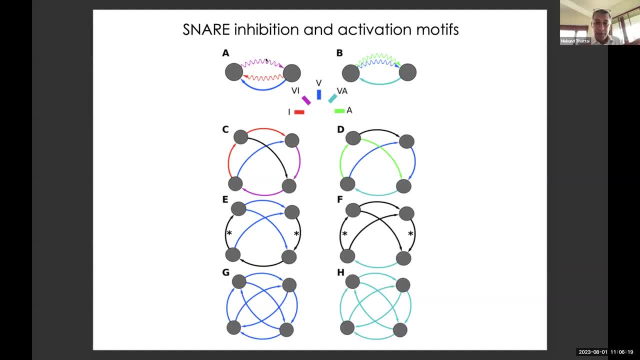 If the molecules are very clever, you can get away with fewer edges. If the molecules are not so clever, you need to make more edges to make sure that there are no clashes. Roughly corresponds to longer solutions in the goat, wolf and cabbage book. 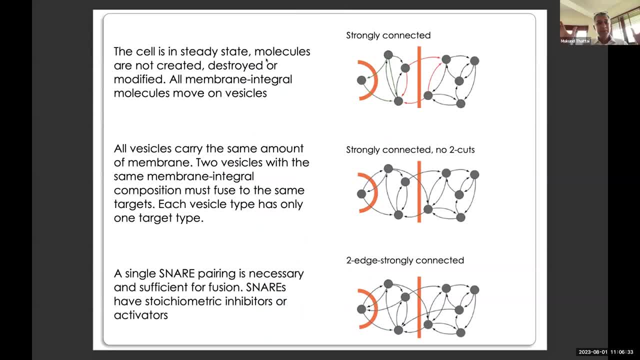 Okay, So here are all the, the full set of results. If my only requirement? the left side are written in essay type form, right, What my requirements are, And on the right side it says what kind of graph can satisfy If the only requirements are that the cell is in steady state. 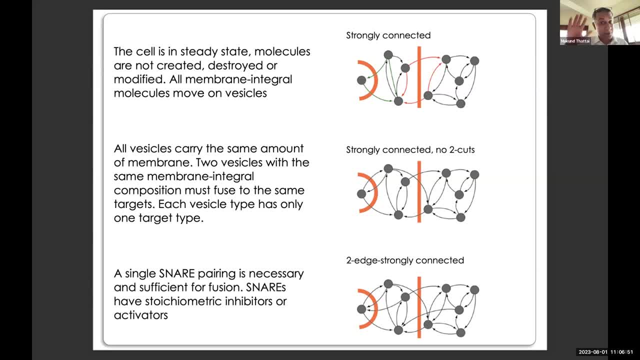 which is a good one. molecules are not created, destroyed or modified, which for snares is true, And all membrane integral molecules move on vesicles, which is a hundred percent true- Then the only requirement is that it's a strongly connected graph. 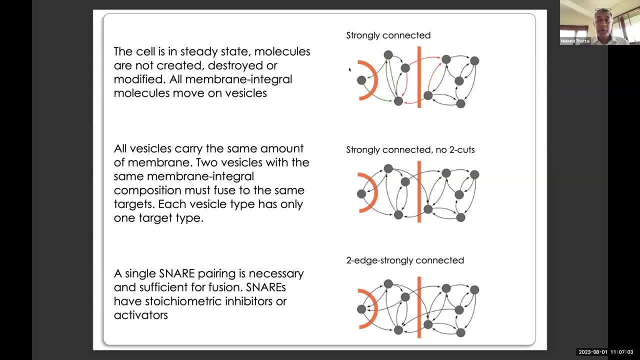 that has a path from everywhere to everywhere. One way to think about that is: you have to have a path from everywhere to everywhere to make sure that membrane doesn't accumulate in one part of the cell, And then this works out nicely. You don't need 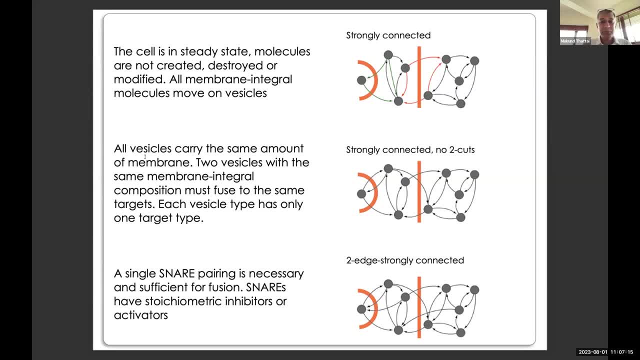 you know, you can have two cuts and so on. It's not a problem. If on top of that you add this property: the two vesicles with the same membrane, integral composition, must fuse to the same targets, which is true, right. 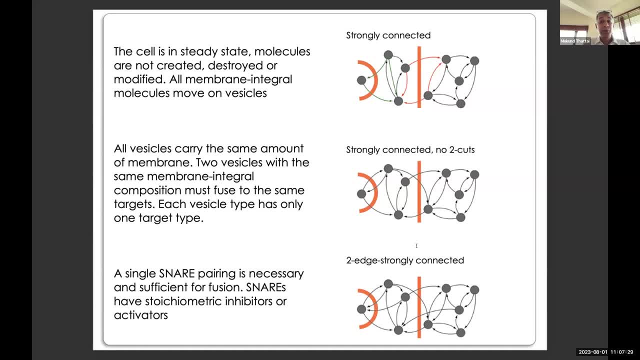 Then strongly connected is not good enough. You also have to have no two cuts, So you have to have another edge to make this work. If on top of that, you say there are snares and snares have inhibitors or activators, 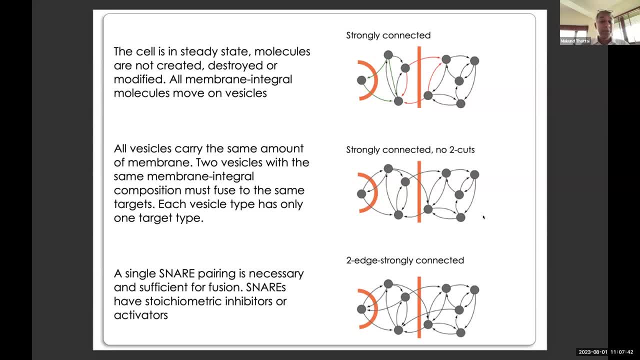 then it turns out that the famous graph we were puzzling around with is not enough, because that has a three cut. You have to have at least another edge here to make a four cut to make it work. And if you go, take a screenshot of what you're seeing here. 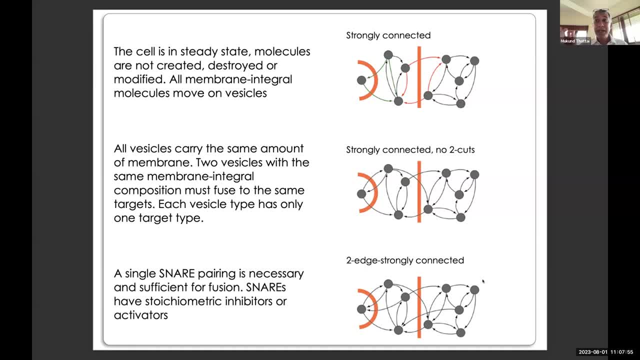 go home, take this little graph and try and work out with a different V-snare, T-snare inhibitor combination for every edge and work out. if you can find paths, I guarantee you will find a solution. I don't know the solution. 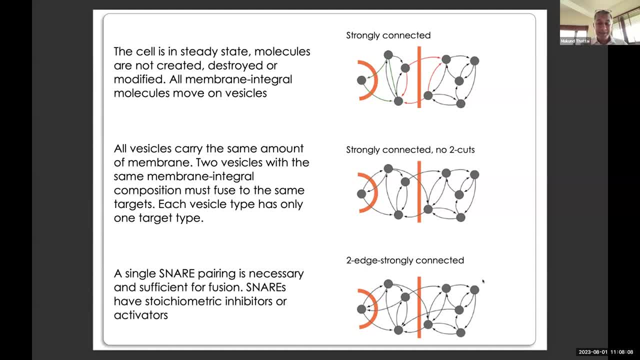 but it exists, because I know this graph has four strong connectings. Okay, so that's. that's my final slide, So I hope the few things I wanted to convey are: first of all, cells are deeply interesting and mysterious and we really don't understand. 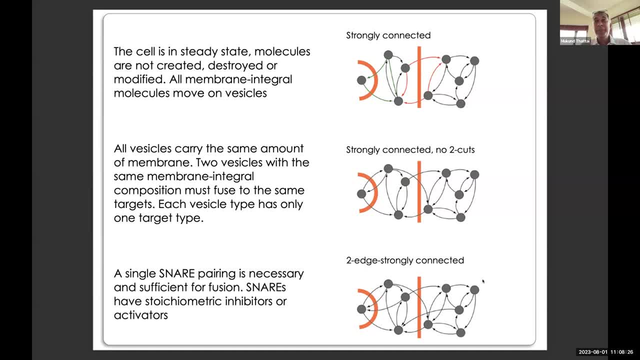 how they work at a global level. We understand a lot about the molecular level. The transport system has some puzzles that are still unresolved about how molecules get recycled, in particular snares. We still don't know the answer. If you abstract this out. 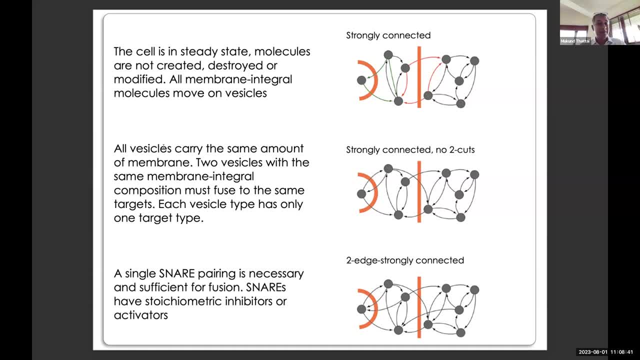 with some very reasonable assumptions. look at this. I haven't made any assumptions about, you know, it's some very general stuff we can all agree on. Then it turns out that it places strong conditions on the graphs that people discover using, say, imaging. 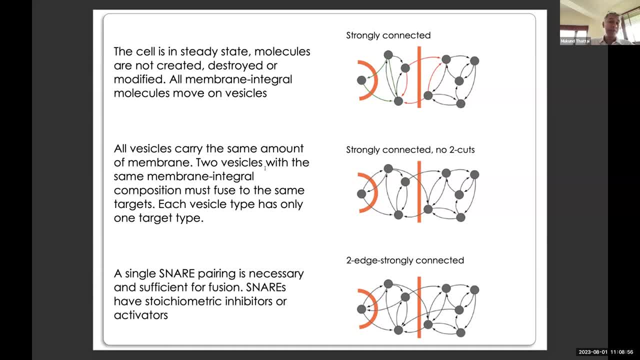 And you can take these assumptions, go back to the imaging and say: you're missing an edge, Please go back and look. and hopefully people can go back and look and they can discover new edges and you can actually tell them where to look, right. 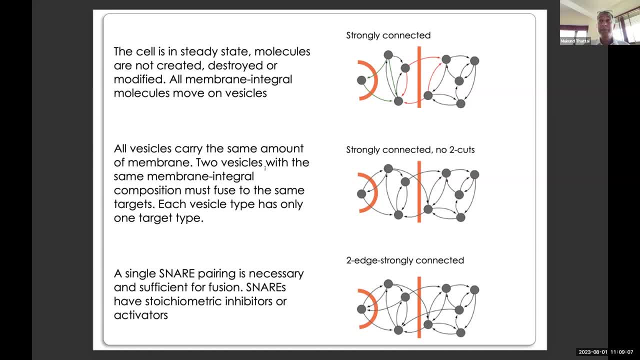 And in this particular case it's very rare, but in this particular case we not only have a model which gives answers, but we actually understand why. because the model behaves exactly as the theorems predict, and the theorems give necessary and sufficient conditions. 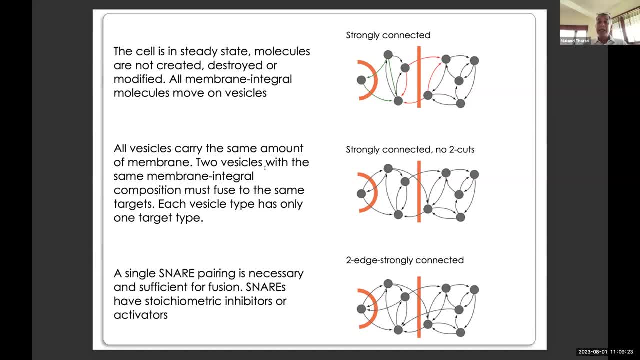 to make everything work out. So once I've just written down the theorems, I don't have to do this back and forth thing where you give me a graph, I give you an answer, You give me another graph, I give you an answer, and so on. 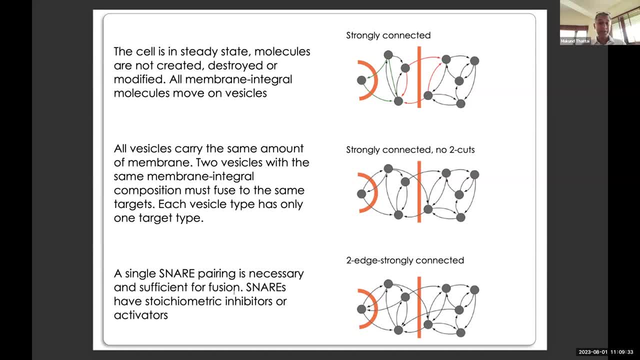 I've given you the full answer for at least these three assumptions. Okay, Now, of course, what do we do next? There are assumptions about coat proteins and how they load cargo. There are assumptions about self edges which we've ignored over here. 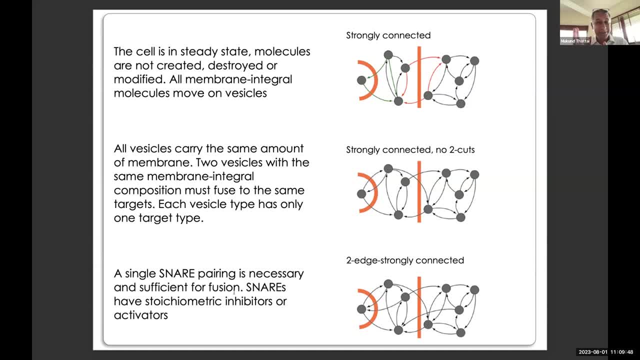 Okay, There are assumptions about the level of specificity- Okay, And then, of course, there's the other broader questions we had about if things are not in steady state, right, So I can scratch out each of these assumptions and make things more and more general. 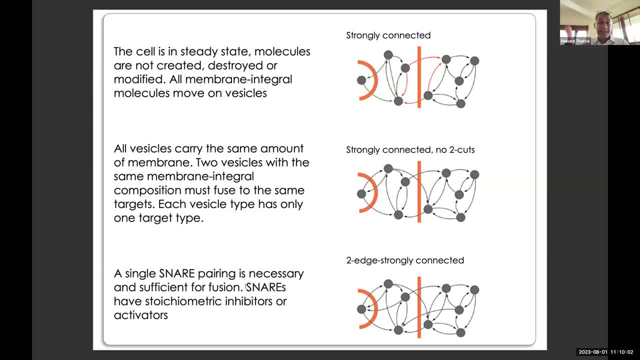 And you can do that and we have done that, But at least here is a nice, satisfying sort of closed solution to the problem, which I found very, you know, a lot of fun. So this is published in Journal of Biosciences. 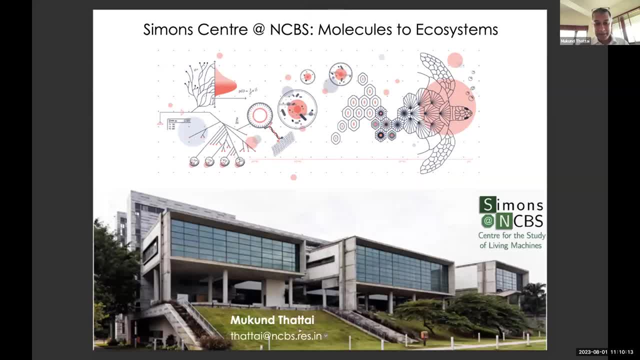 You can go read about it and email me here if you have any questions, and please come visit. We have a lot of fun here at the Simon Center, which is a bunch of physicists and engineers, mathematicians, computer scientists, looking at problems like this. 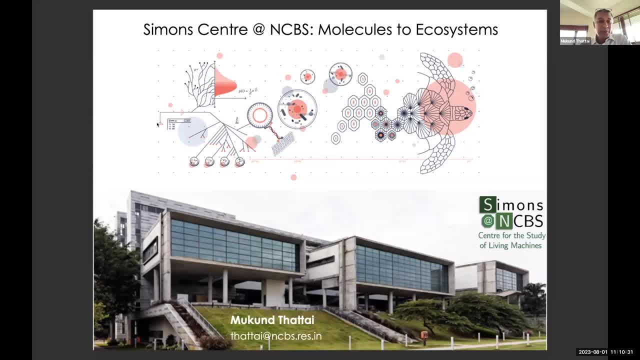 This is a little logo for the Simon Center we commissioned a few years ago. I don't know how many of you are old enough, but on the left you have a logo. turtle Logo is a programming language from long ago- 80s. 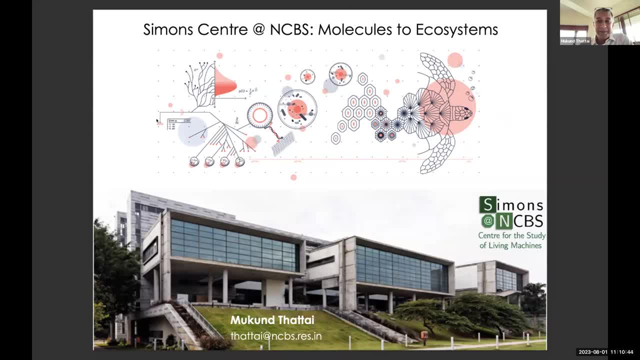 You had a turtle on the screen, You were allowed to tell it forward 30, right, 10 degrees, and so on and so forth, And from that you build a whole picture. So from such microscopic interactions you can build up trajectories. 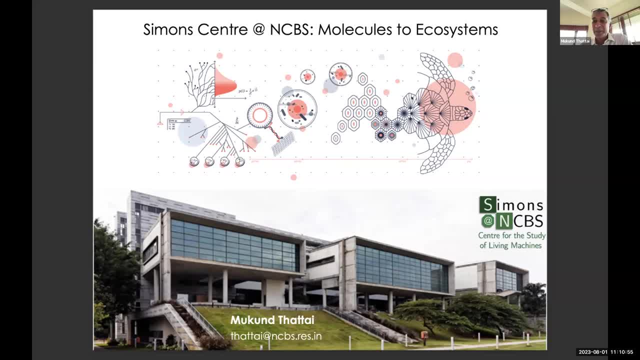 You can work at the scale which I talked about of cells and vesicles, entire cells and tissues and indeed organisms, And you can build up on the right a real turtle or at least a picture of a turtle, And really the goal is to span all these scales. 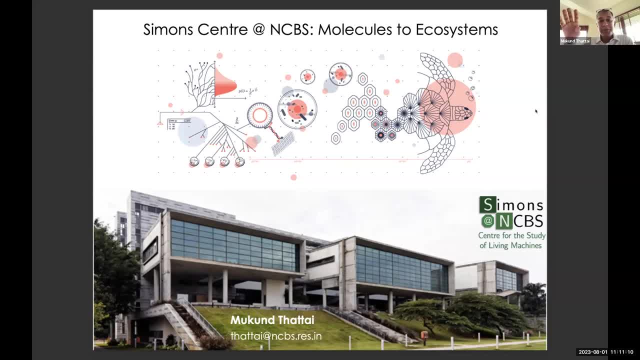 at least be aware of them in any biology problem we deal with, because that's the fun part of biology, right? You've got a couple evolution to molecules and everything. I'll stop. I'll continue sharing in case there are any questions. 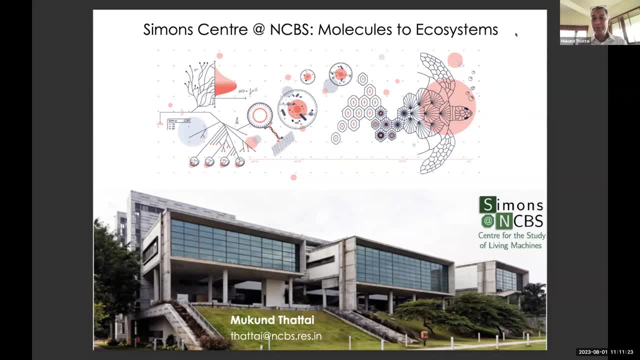 I can go back to that slide, Happy to take questions, And among other questions, we can also talk about broader issues of what distinguishes models from theories and and how to choose problems to work on, and so on. Yeah, there's a question. 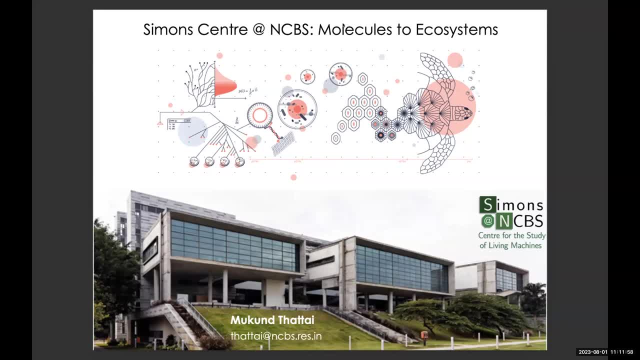 Yes, Kasi Hi Mukund, If you would discuss a little bit about graphs that are static and not really directed, for example, arborization of the blood vessels or, you know, webs you see in biology right. All the information travels through them. 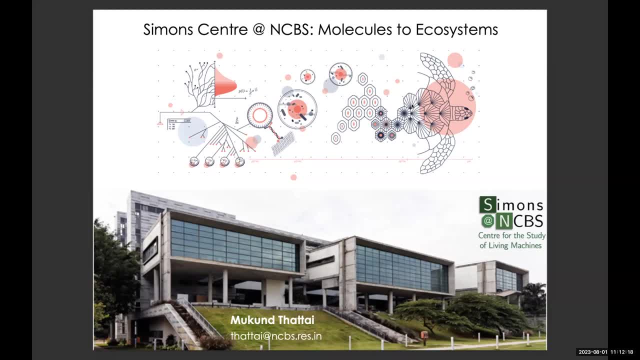 But then their structure is kind of static, And then when they're made, possibly there was some directionality to it. So can we deal those structures in the same manner, Or would Menger's theorem apply for those, Or there is another substitute for that? 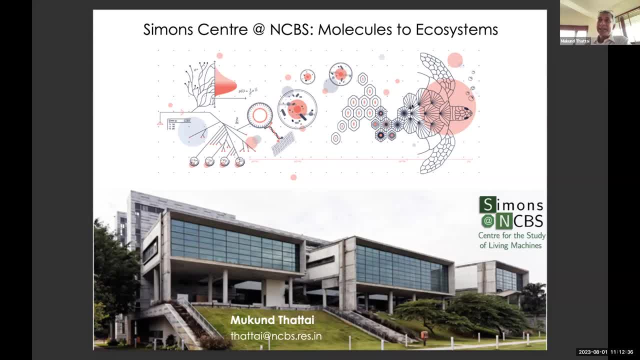 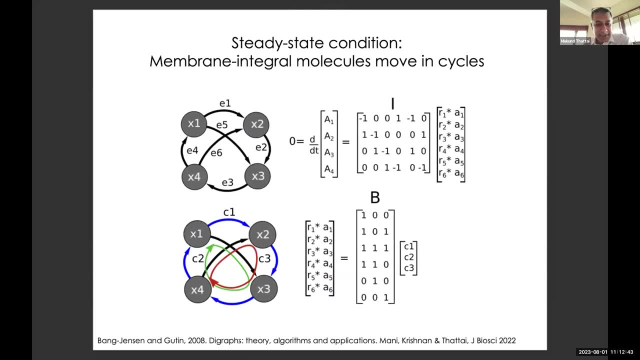 No, no, no. So Menger's theorem doesn't work, So strangely directed graphs are understudied, even in engineering. In fact, this monograph Bang Jensen and Gutin, you can download it for free And it has every result. 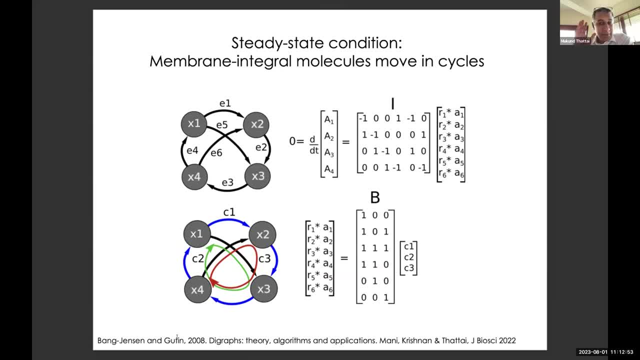 that you want to know about directed graphs Quite recent. as you see, There are no full textbooks on directed graphs. The whole huge amount of work has been done for undirected graphs of the type you bring up Now. there's an interesting question. 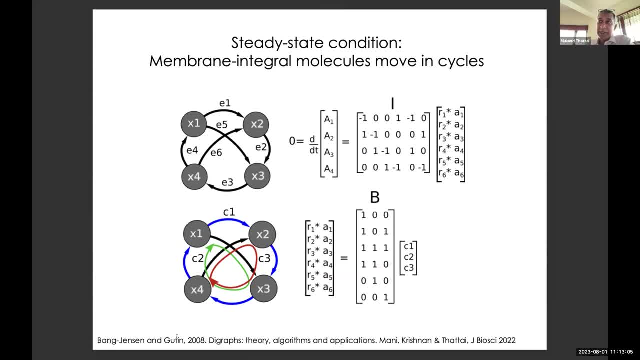 I give you an undirected graph where between node A and B, you have no sense of direction, But globally there may be some sense of asymmetry And you might be able to identify it. And you might be able to identify such a thing. 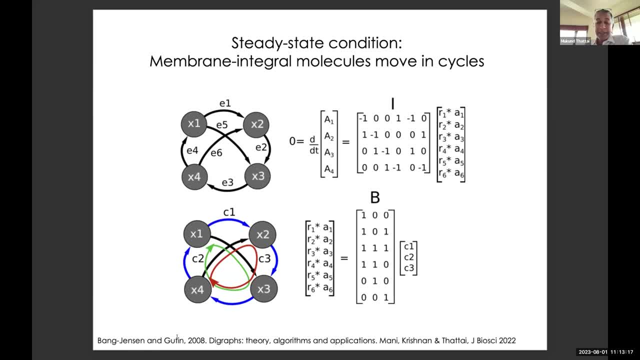 Now, there are techniques for this, And they're not as clean as these theorems, Because if you can't rule out a reverse flow, let's say, of some blood vessel during at least some phase of the pulse or something, you have to have a more sophisticated view. 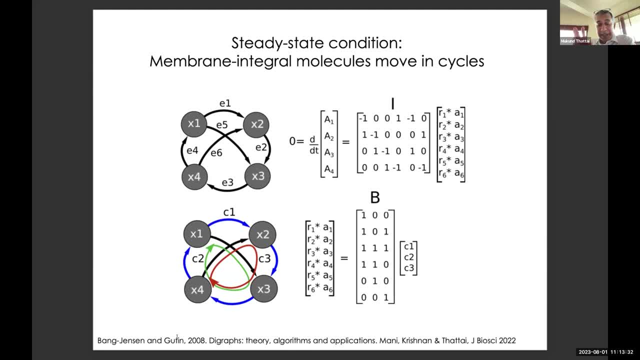 of what the edge means. The other graphs that people tend to forget are undirected Metabolic networks Where, yes, enzymes tend to move, chemical convert, you know, substrate to product, But enzymes are actually reversible And you can convert products to substrates. 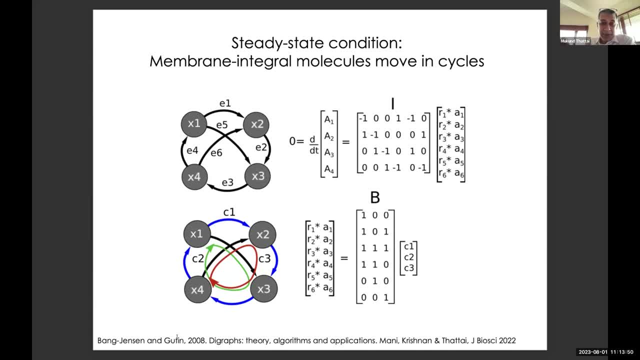 And so under conditions where the product is in excess, or under thermodynamic conditions where certain arrows don't work in the right direction, the thing can flow in completely different directions. So chemical reaction networks and the theory of that, for example, flux balance analysis. 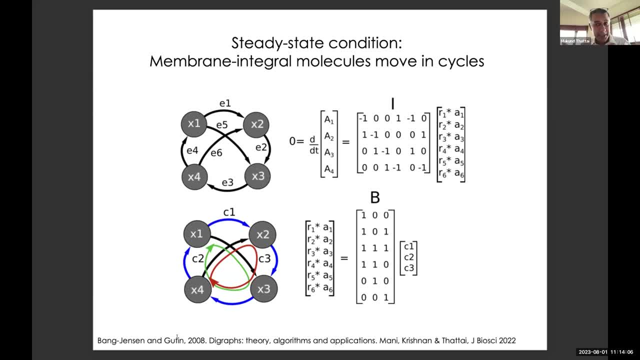 what they do is they convert the undirected graph into a type of fake directed graph where every edge has two directions. You replace an undirected edge with two edges and you treat them separately. You can always pull that off, But if you can pull that off, 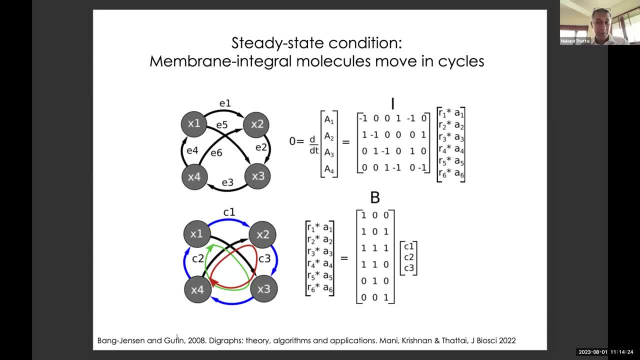 then you can use the theorems that I just mentioned to check if things work out or not. But it's subtle and you know it should be left to the experts. Thanks, So I had one question. I was just wondering. 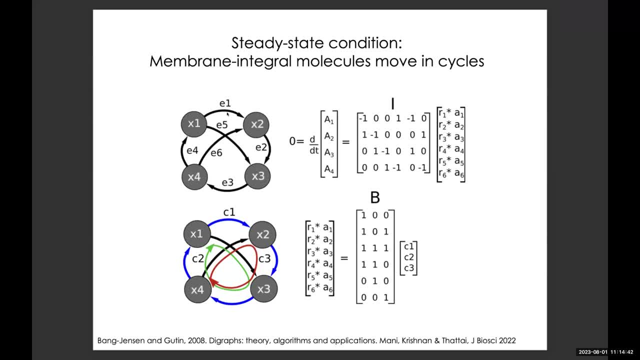 you mentioned that you studied all these results in the context of snare proteins. I was wondering: are there other classes of proteins which might obey these and you can apply these? Yes, So, first of all, here's the way you should think about it. 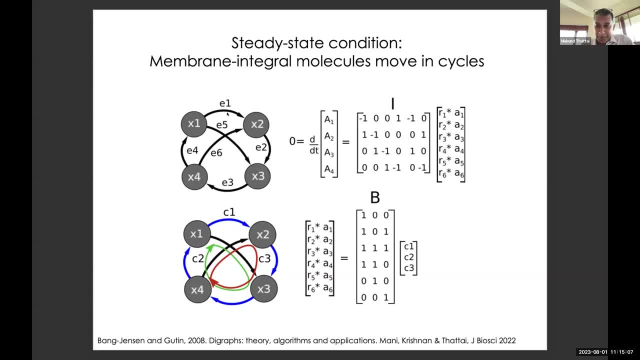 So, just looking at the constraints for snares, here's the number of edges we need. Okay, So you have to ask whether other things obey the same constraints. If they do, you can get away with the same edges. Now you have to ask: 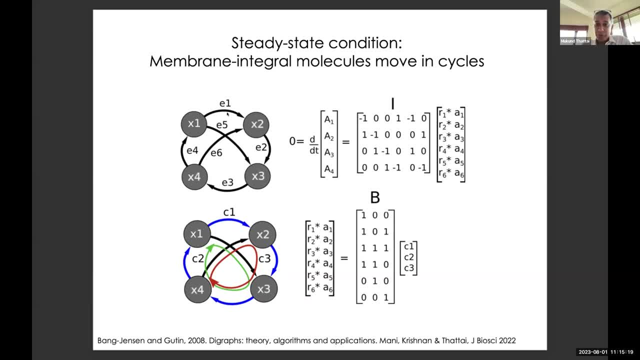 whether other things obey different constraints. Okay, Suppose I only have two coat proteins, then I should ensure that the coat proteins that are being reused in different parts of the cell don't clash with each other. But that's a whole other set of constraints. 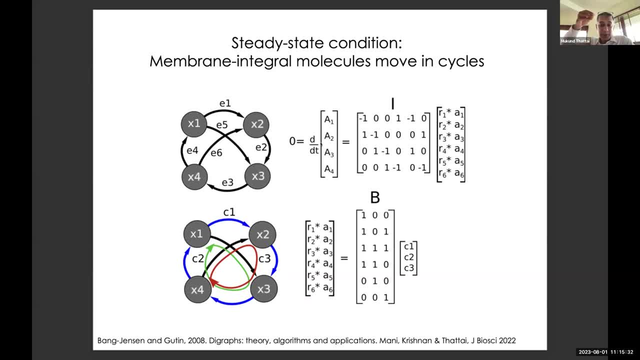 which we have studied, that I'm not bringing up over here, but which will introduce even more edges and compositions and so on. So something that obeys the same as the snare proteins. we've solved for all of them: Snares, lipids. 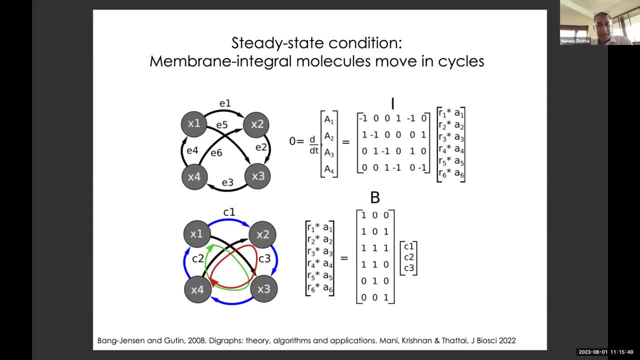 basic things that travel in cycles. The thing we're studying now are the coats, But I think the real constraint is something I haven't mentioned, which is interesting. It's the question of function. What are these graphs good for If they're not good for anything? 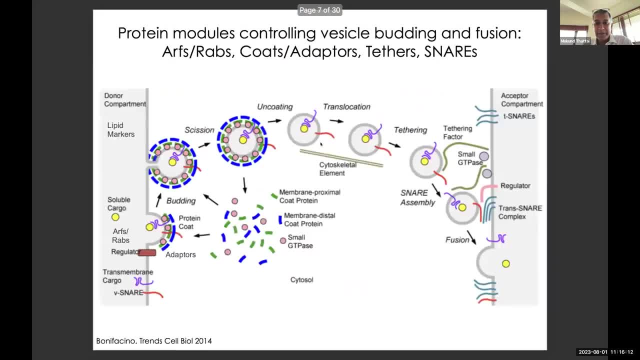 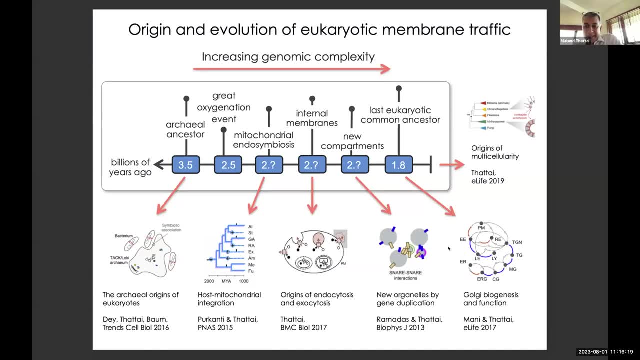 so let me go back to my at the beginning. I have a picture of a graph that is: look at this graph here. That's actually a directed graph where I have other kinds of edges. Okay, here I have. this graph is not in a static, steady state. 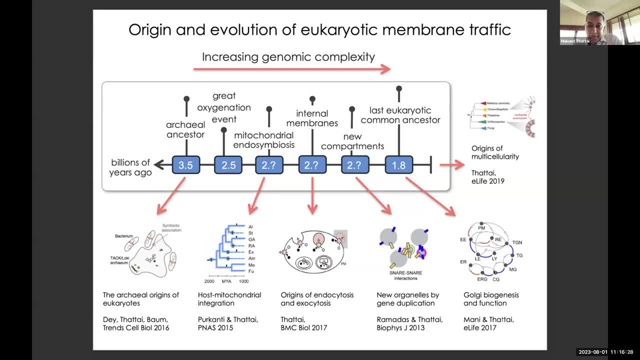 but it's actually in dynamic, steady state where compartments themselves flow from creation to destruction. So these graphs also exist, And this part of this graph is actually the Golgi apparatus, And it turns out that this particular graph, topology of the Golgi apparatus, is very useful. 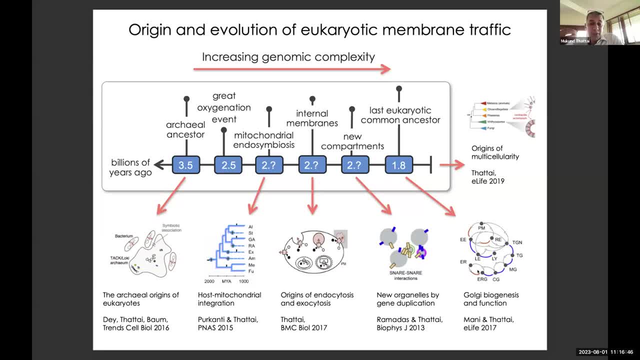 in order for the cell to synthesize complex molecules, to show other cells on the cell surface. It's a very tight connection between the topology of the Golgi and its ability to synthesize complex chemicals. So just making these graphs is not sufficient. It has to be useful for a cell in order to be selected. 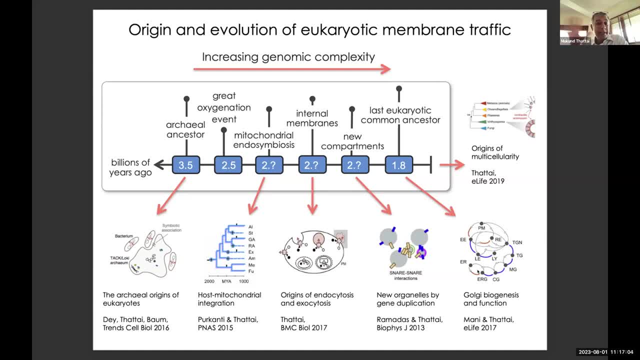 And I think that part people haven't even done experiments to check why certain vesicle particles are useful for a cell. Obviously, this is a technically challenging experiment, So I think it's a huge field of new work that can be done. Actual benchtop evolutionary cell biology. 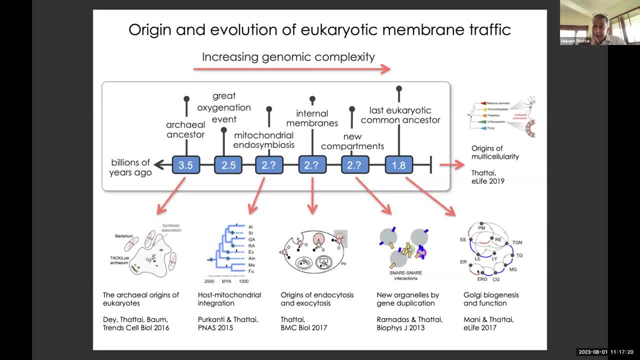 where you put selective pressure and track individual fluxes and see what good it's doing. And I'm going to bring that back home to one aspect of what we've done today. Okay, so why is the graph like that? Well, because the cell needs. 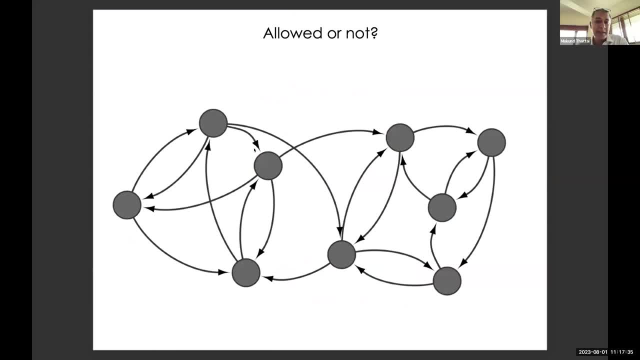 so, for example, why is this graph like this? Well, it turns out the cell needs this cycle to do something cool. It needs it. Okay, that's what the graph is for. Well, what's the rest of the graph? Well, maybe the rest of the graph is there. 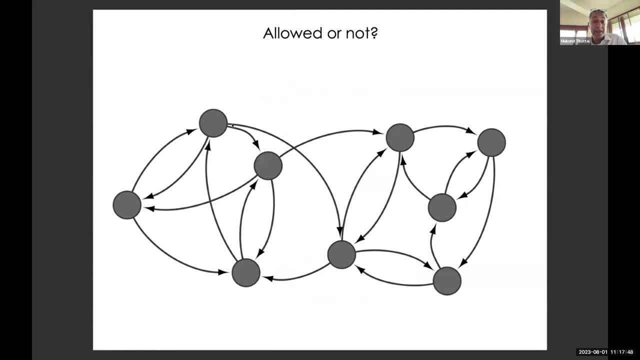 just to make sure the Vs and the Ts snares and all that behave the right way to make this work Right. so there's the underpinning substrate and then there's the functional link. I've only talked about the substrate part. 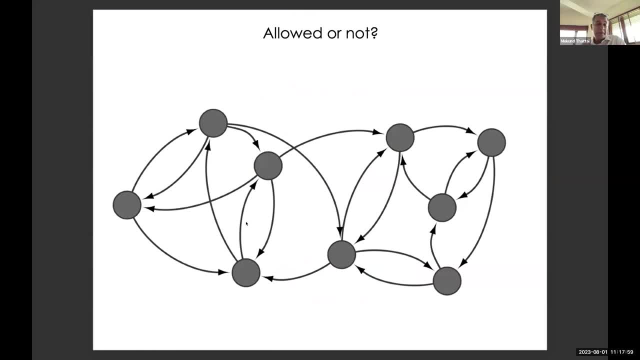 Right. so to separate the basic machinery from the functional machinery, and so on. these are things which people have just started to ask. And it's difficult. Cell biology is difficult for exactly this reason. If I break an edge here and knock out a molecule. 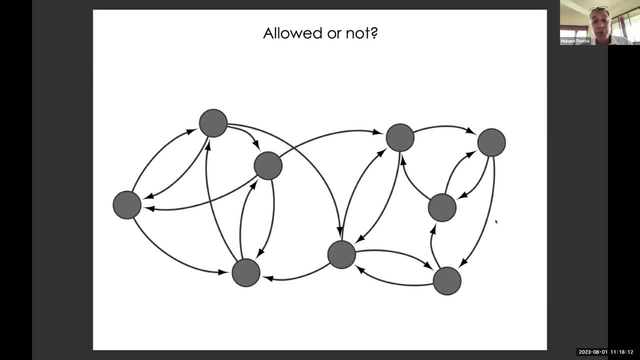 I break an edge here. the consequences happen throughout the cell. They just things start breaking as the fluxes go out of balance, And this is the reason why genetics of vesicle traffic has been so difficult to do. Okay, so I'm not saying that it's an easy thing. 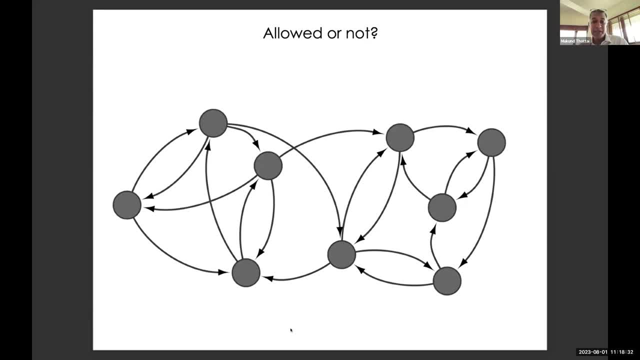 but it is really a thing that we need to. we need to start working on as an experimental subject. There's a question in the chat if one makes these graphs undirected and put some probability for forward and backward parts of the same solution. 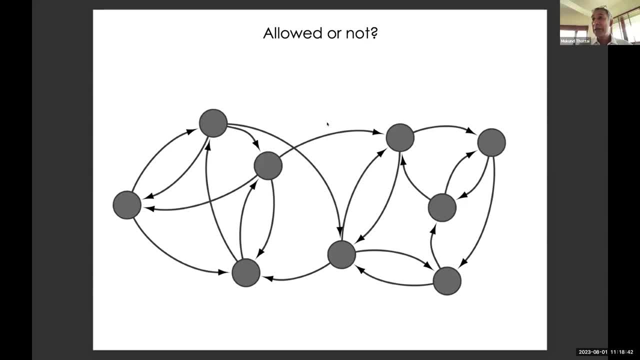 Yeah, so very nice question. So, as I briefly mentioned, there is another representation of the same thing, which are Markov chains. These nodes become states, the edges become transitions, defined by some probability, which are columns of a matrix. Then you get some Markov chain transition. 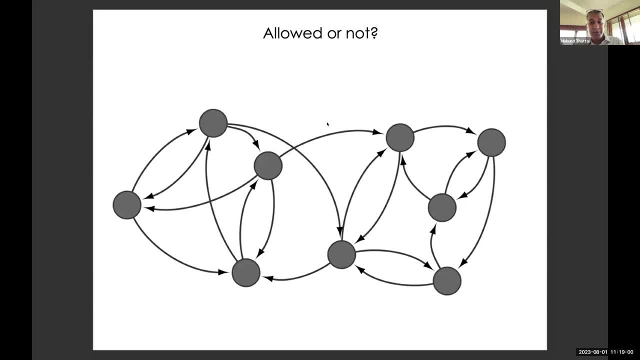 and you get a steady state. And those steady states always exist. So in some sense, if you introduce probabilities, you can always find solutions. The issue with probabilities is function- How do you determine those? How do you determine the solutions? It's just the-. 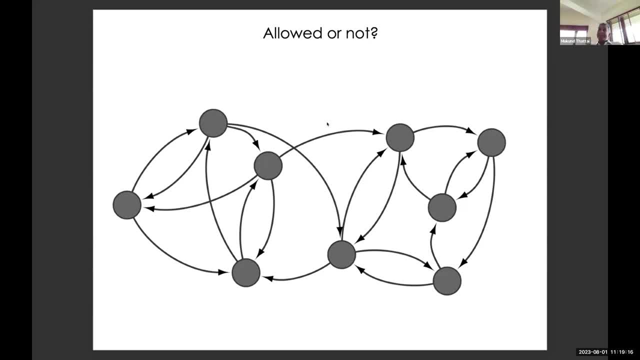 Those probabilities? Oh, how do you-? Experiment? Nobody's done it okay, And my impression is that actually it's a bad approximation, which I was just going to get at, because what you want when you get inside the cell is: 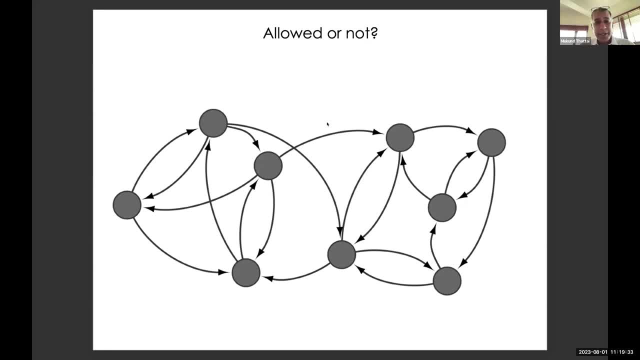 again. think about it as a user of a bus system. right, You get on a bus. you want to make sure it gets to where you want. okay, You're not going to get on a bus with a 50% probability of getting where you want, okay. 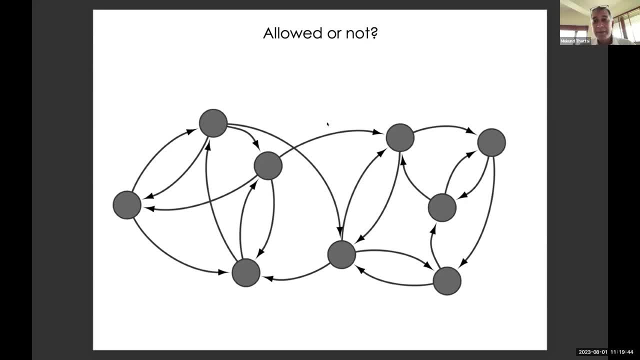 Because then you're stuck and you don't know how to get back. So, inside a cell, I think the probabilities are dominated by certain fluxes which you should think of as approximations. You should think of a pure directed graph as an approximation to a probabilistic graph. 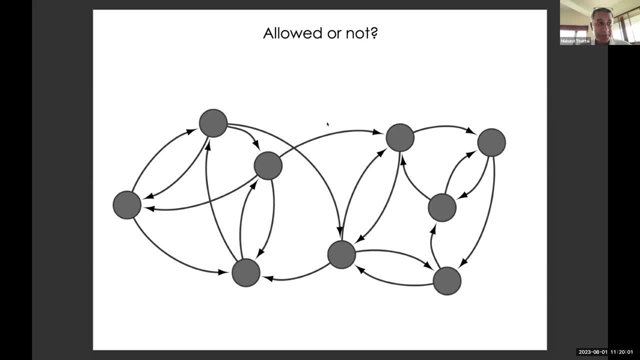 with very high probability of certain fluxes. The rest will then constitute errors. And then you can ask: is this steady state robust to errors? And the answer is yes, because you can make a dynamical system with some low probability of errors and up to some probability of errors. 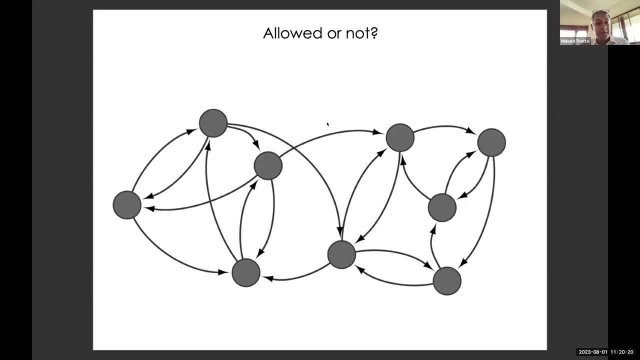 it will still do what you want it to do And, of course, beyond some threshold it'll fall apart catastrophically, and you can make such theories. The problem is that nobody's measured the error rates for individual pathways. It's difficult, but it's worth doing. 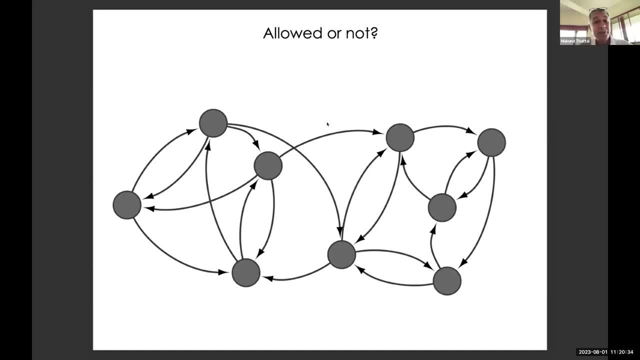 Except for one thing, which is synaptic vesicles, which pretty much don't do anything wrong. So it's not a useful case. More questions: I'm loving the questions. Really, you guys are saying this is all too simple. I want something more complicated. 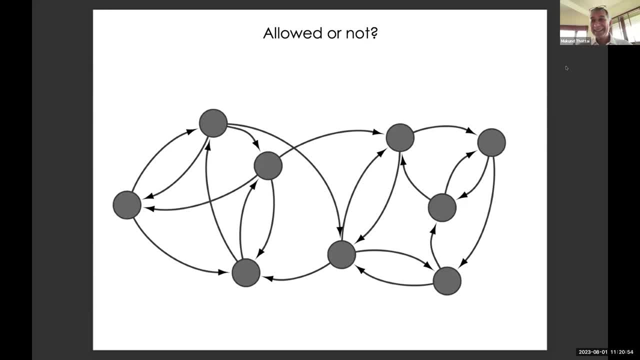 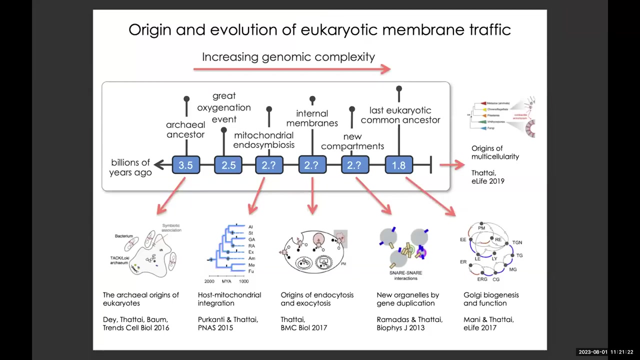 So sure Any questions about the broad issue of what distinguishes theories from models and so on. Or we can ask other questions about cells, And let me go to a page which may have enough stuff to talk about. Participants, don't be shy. 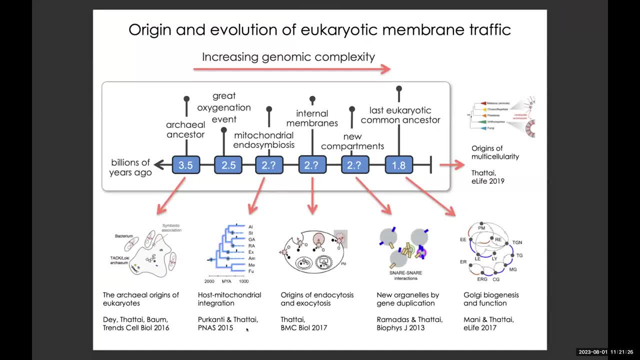 Feel free to ask questions. Yes, You said you can discuss about how to choose a problem. I didn't promise that. I said how to make a model. How to choose a problem is the question if you want to go down a research career. 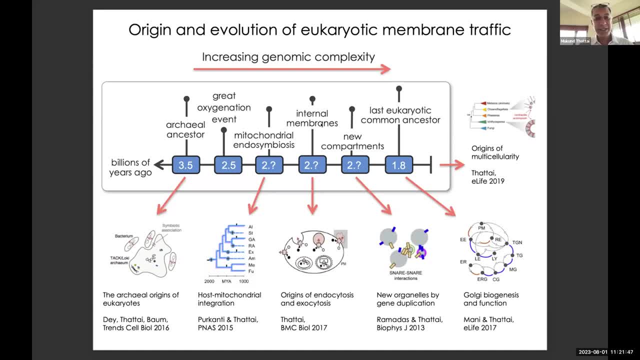 And you learn how to do it by working under somebody as a guide. You see how they choose problems and then you stick out your own directions while you still have some buffer inside your PhD group. And then you take a risk and you choose a problem. 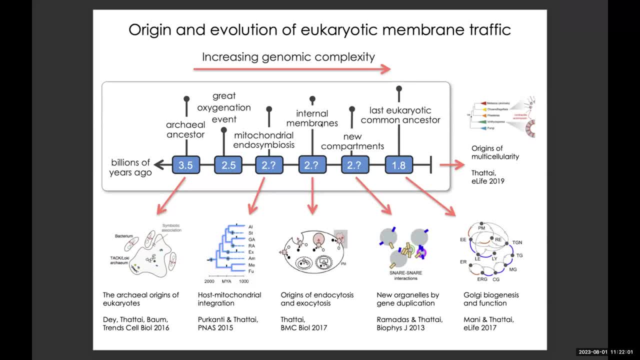 based on some combination of your interests and your skills, But it's not the same. It's not the same. You know the ability. you know this is a question which, I think, may take more than 10 minutes to answer. So what I promised was how to make a model. 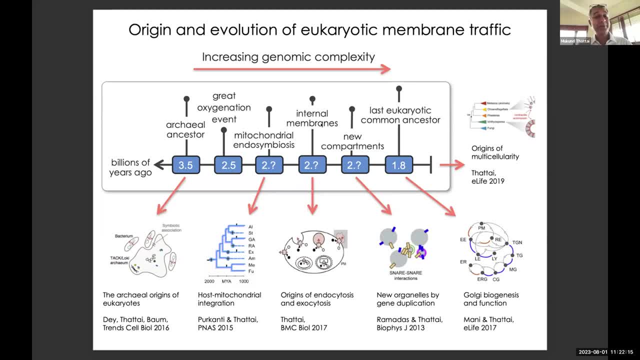 and distinguish that from theory. How to choose a problem. you develop a taste for it over time, But you know, please be adventurous. The only way to try and choose problems is to try and push yourself beyond your limit. fail a little bit. 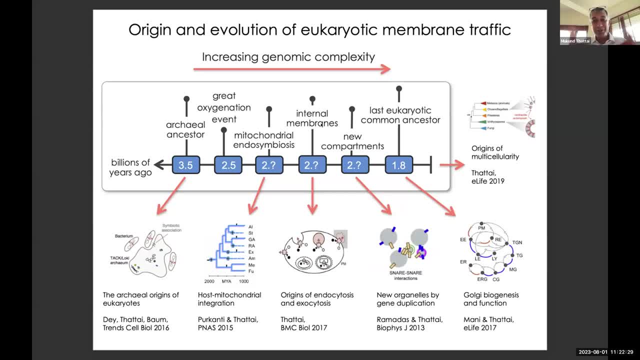 fall back into your comfort zone and then keep trying this. Yeah, It's a generic answer. It's the hardest thing, Mukund, it may help the trainees if you could discuss how to toggle between experiment and theory, Like Oh. 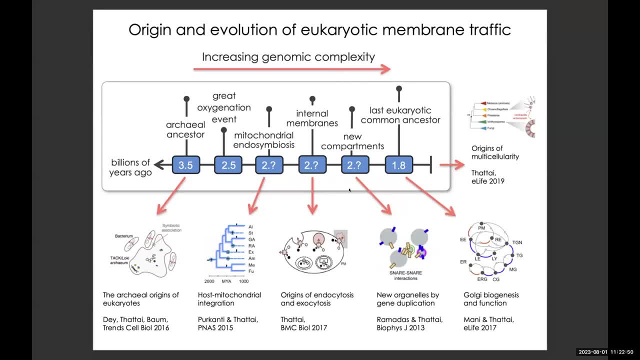 that's a great experiment, Yeah, So it will help the trainees, I guess. Yeah. So actually when I started, I started in physics as a pure theoretical physicist And during my PhD I started doing experiments. I actually cloned. 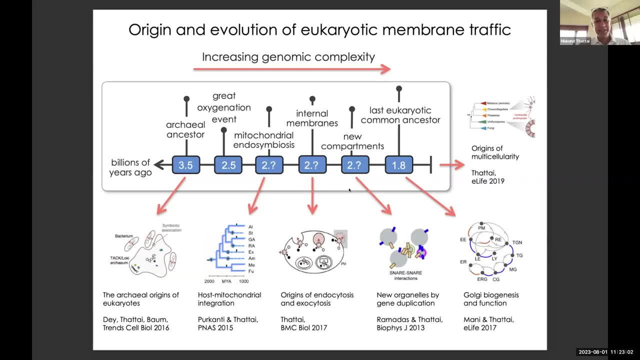 some genomic insertions of genes and measured stochastic gene expression. bacteria did some imaging So I had you know some. I carried out some experiment through the full cycle up to publication And when I started up at NCBS 20 years ago. 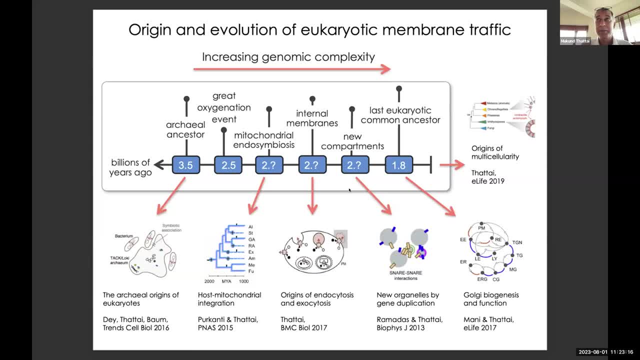 I had an experimental lab And you know we were doing quantitative experiments with bacteria. So I think it's absolutely a must for everybody interested in biology to have literally done experiments with their own hands at some point, And by that I don't mean 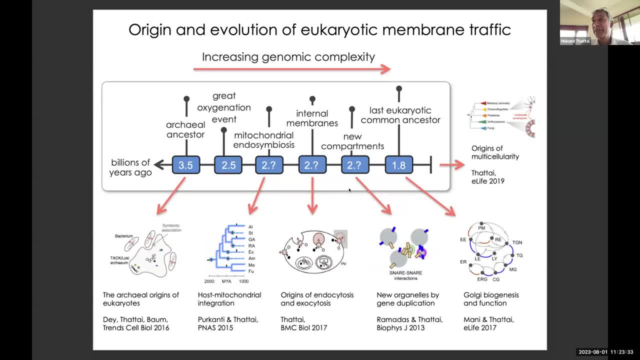 an assay, but a proper experiment, where you design it, you carry it out. it fails, you go back, you do the full cycle. Only after you do that can you have the. You know, if you don't do that, 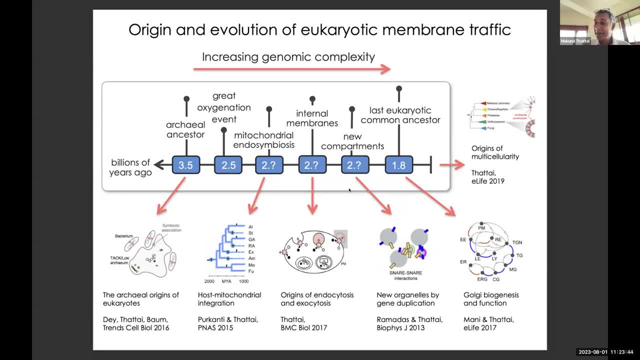 and then you go talk to your experimental colleagues and you're just a theorist. you'll just be saying: why don't you just give me this data And you don't realize that they would also love to have that data? It's technically challenging. 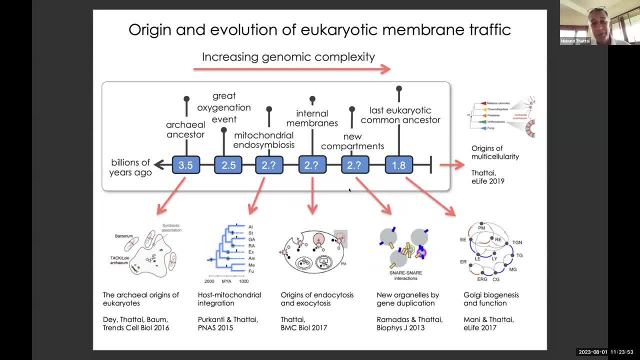 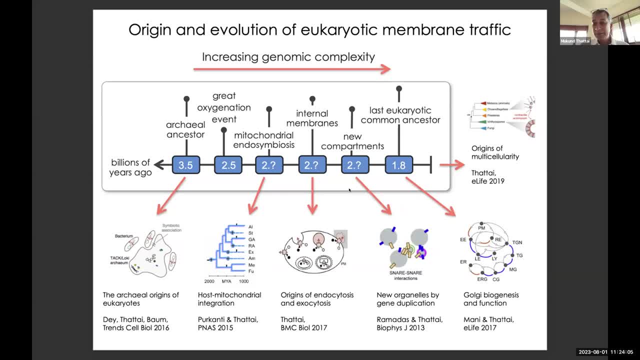 with a way to circumvent various technical hurdles. it's not possible. So first, you know, do experiments, at least sometimes. Secondly, when you work, you never give up that link with experiments. Every model you make and every theory you try and see. 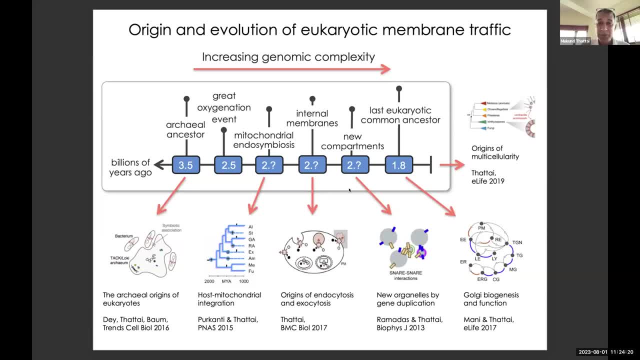 how can it be tested? How can it be tested? How can it be tested? Go and ask people What assumptions are too simplistic. What am I doing wrong? Go and ask people. By people I mean experts, Because they know intuitively. 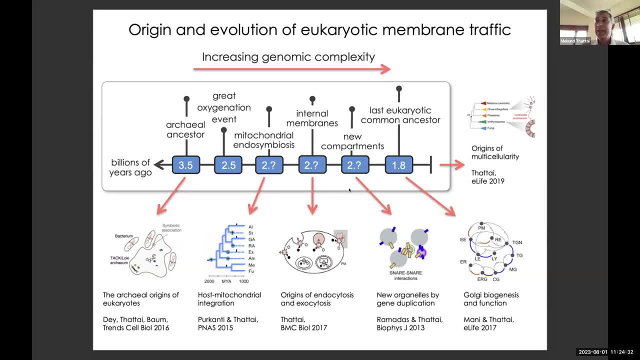 a lot more about how their system behaves than you do, And they may have seen some pattern which they filed away in their minds and they see your model and suddenly they say, ah, this looks like that, and then you can go back in, So that back and forth- 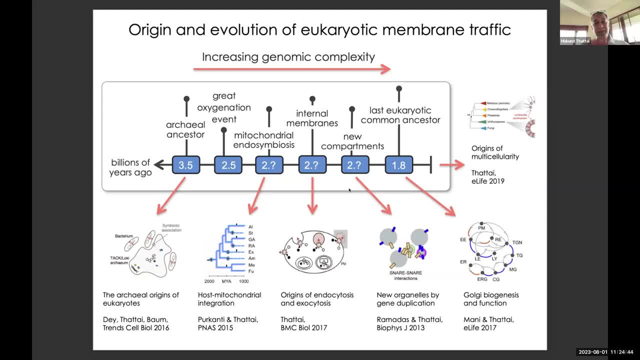 has to be there, So you shouldn't end up in a department where you know it's a cocoon of just modelers and theorists, And this is I'm speaking for cell biology, Of course. bioinformatics is a different field. 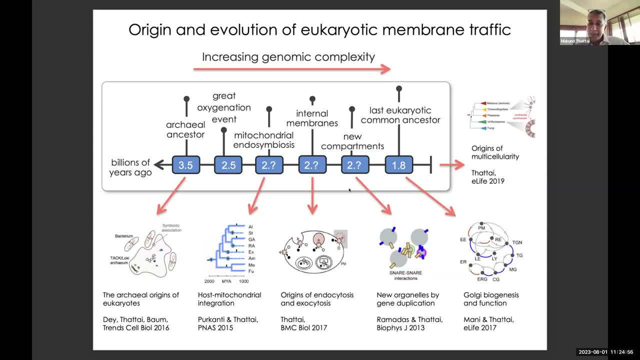 Very mature, where one can deal with purely computational data sets and do purely computational work because the data sets are so well-structured- genomic data, things like that- So that's possible. But if you do that then you shut yourself off from potential new problems. 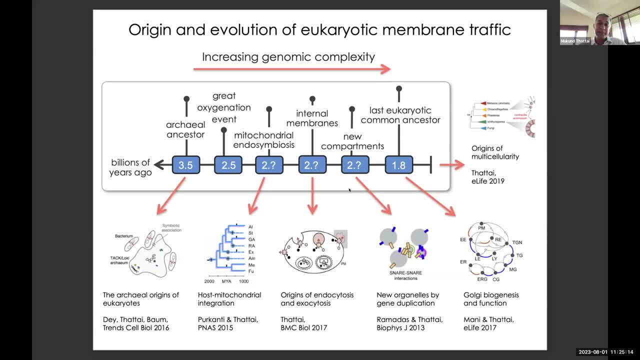 which may come up by somebody introducing a new model organism and a strange new way to measure things. So that connection always has to be there. So for me, I think what's ideal about a place like NCBS is where there's a few of us theory people. 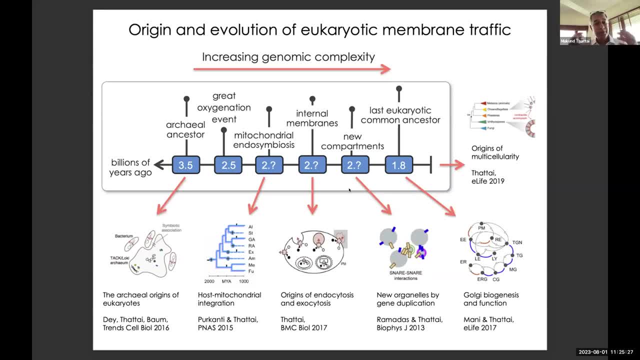 or computational people, but the rest are really people who keep us on our toes. We see new talks, We see new experimental modalities. We really see data. Things don't make sense all the time, And that's the process. So that's the connection. 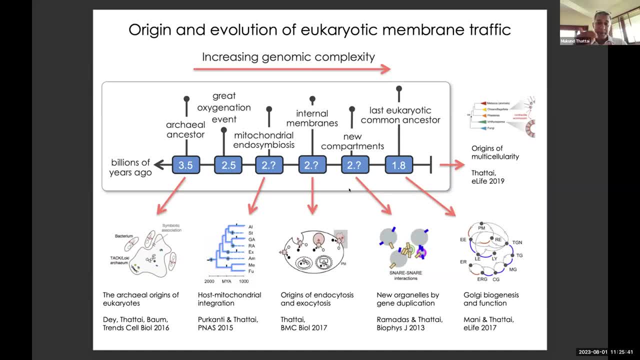 And if you want to start a collaboration, you start by respecting the cell or whatever the actual system, And then you start by respecting the techniques and the people who do the measurements And you slowly try and work your way toward articulating a question. 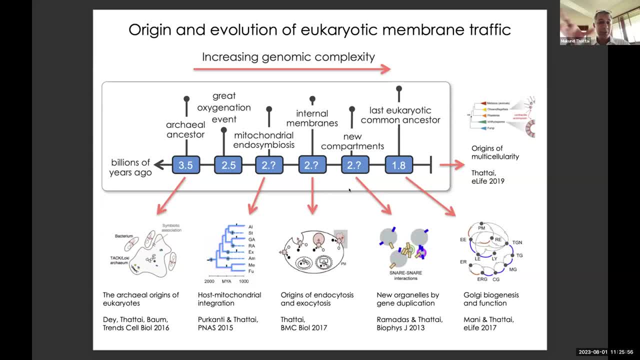 You don't go in and say I have the answer. You go in and say this is very serious And you work backwards from there. My two cents. This has been my experience. Your mileage may differ, but I think it's roughly correct. 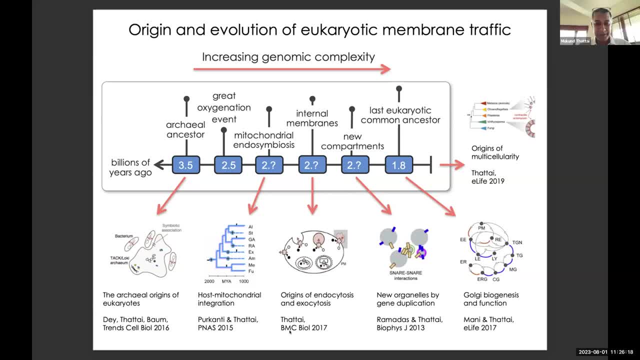 Prasamukhin, there's another question in the chat. Sorry, Let me open that. I'll just read it out. Kaushik, if you want to ask, you can unmute and ask yourself also. I got it. 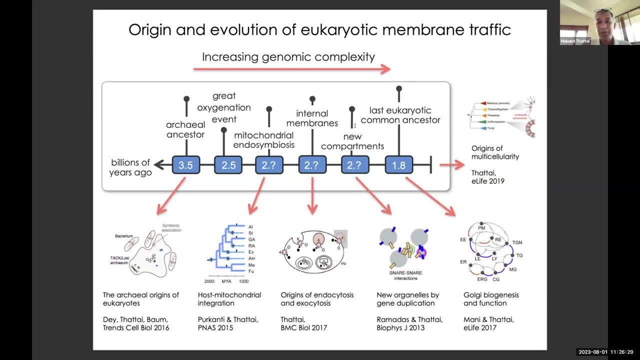 Can V-SNAP proteins be used for another vesicle? That is the case. How is the recycling modeled in the node-edge form? Beautiful question. So it turns out this distinction between T and V-SNAPs is not a molecular distinction. 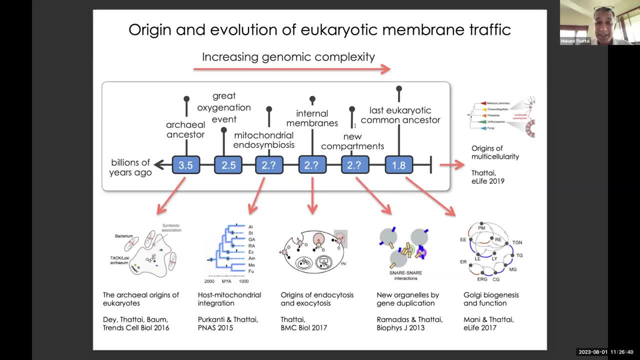 The same SNAP can behave as one on one path and behave as the other on the other path. Then the question becomes: and how does the T-SNAP get to where it needs to go, Which we didn't even address today. but we have some models. 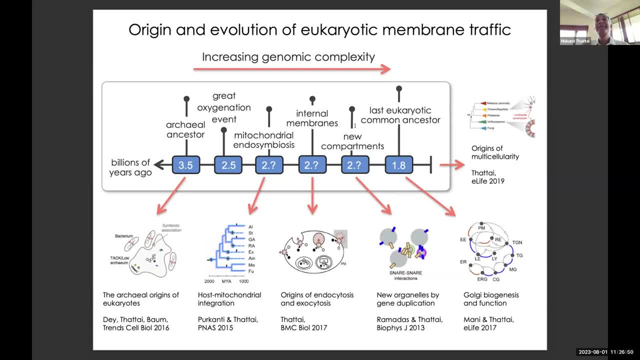 for that And that ends up being a very difficult constraint to satisfy, And fewer than one out of a thousand graphs that you might naively write down can jointly satisfy this V and T-SNAP constraint. So the graphs that are true cells are a very special 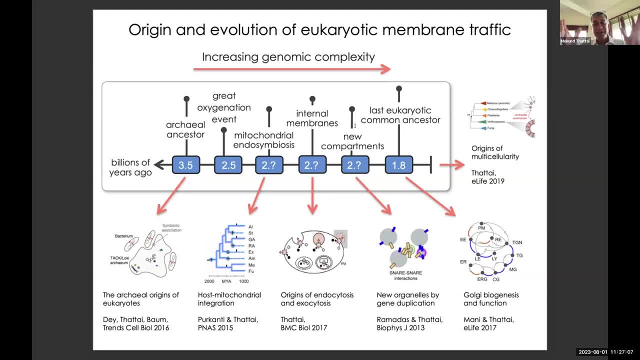 set of graphs out of all the cells I forgot to mention. how did the T-SNAP get to where it's going, Because all SNAPs are starting out in the ER. That's where they're made. How do they get to where they need to go? 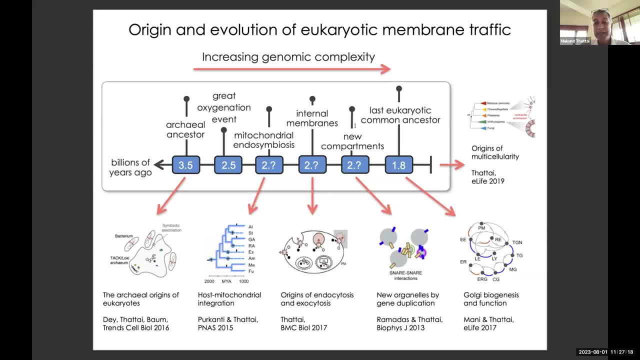 So that's a lovely question. So that's why in the field people tend to not talk about V and T-SNAPs anymore. They talk about the SNAP quadruplet, the four helix bundle, and there are three that are called. 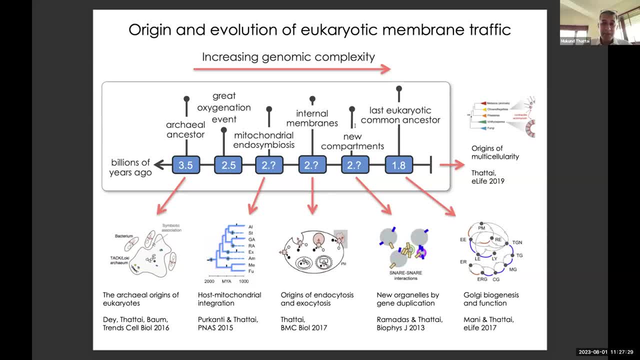 Q-SNAPs and one that's called an R-SNAP because of the amino acids at the midplane. It's very understudied about how T-SNAPs get to where they want to go. Thank you for that question. 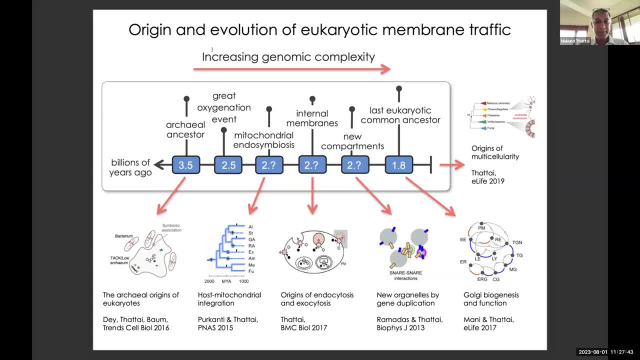 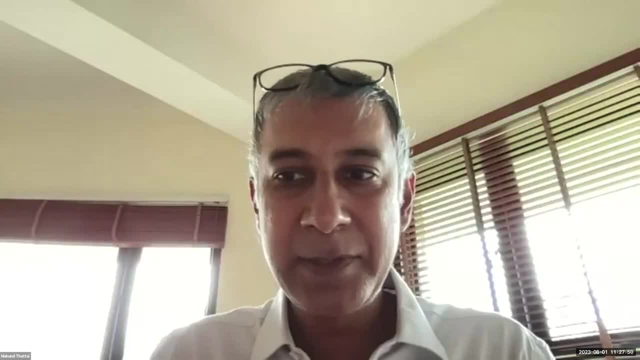 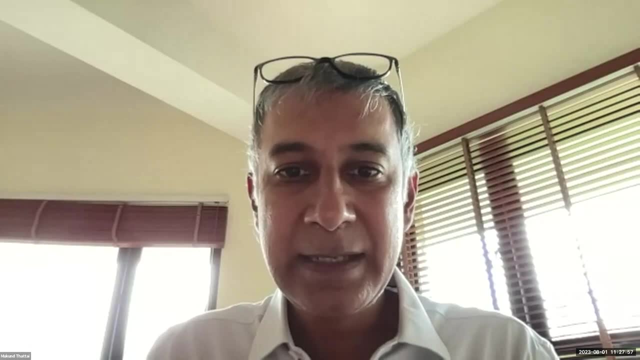 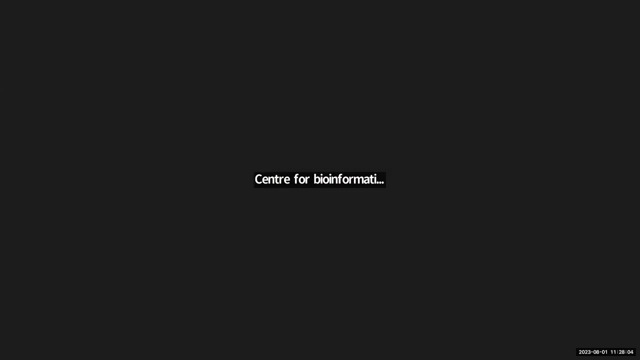 Actually I should have highlighted There's another. Let me just stop sharing here. There is another paper which you may want to look at, which I'm going to, So I'm just going to flash here this paper for you. Feel free to go. 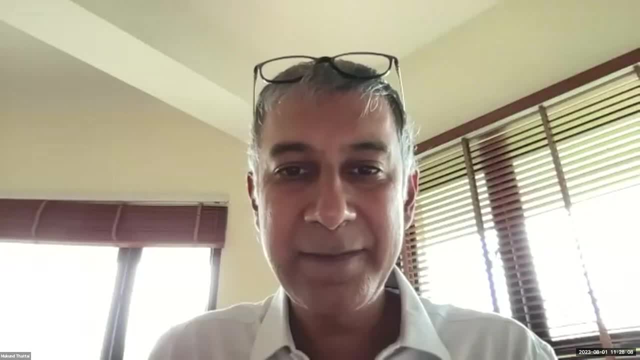 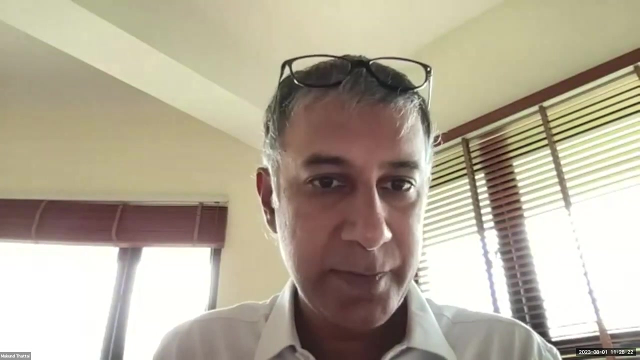 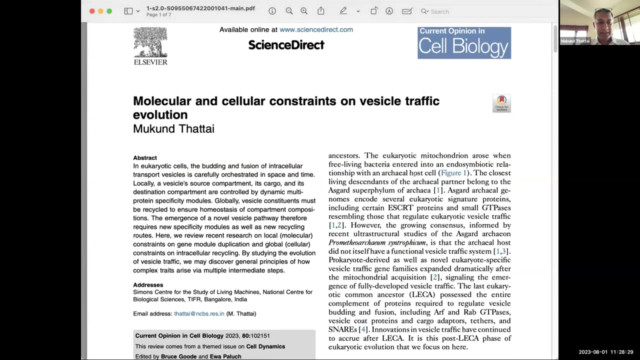 a couple of minutes above limit, sorry, Oh, is that okay? Yeah, fine, Share my screen again. We'll do this. I'm sorry for not including the citation. This is a recent paper, So can you see this paper? 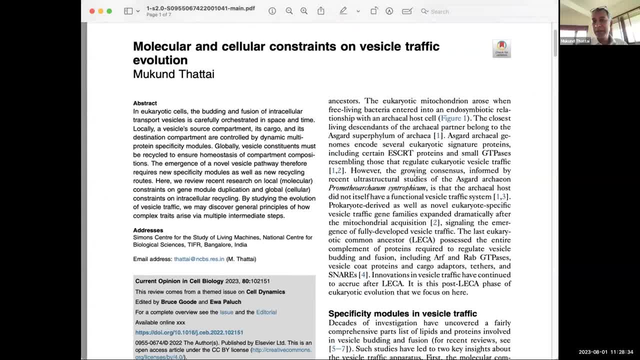 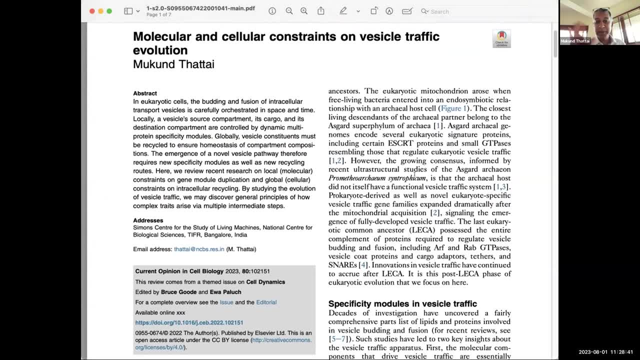 Yes, sir. Okay, Molecular and cellular cancer. So basically all the cell biological evolutionary themes which I touched upon today. this is not a mathematical paper. You'll find the recent references from the last couple of years. I do talk about this idea. 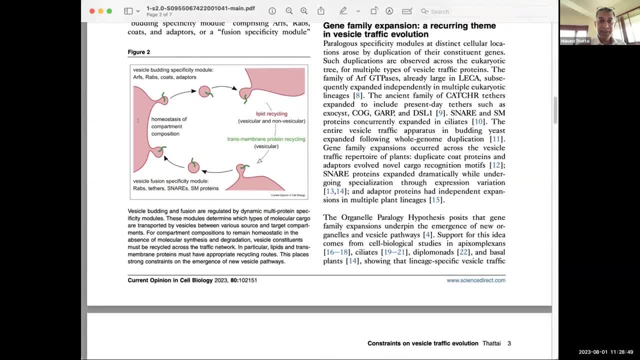 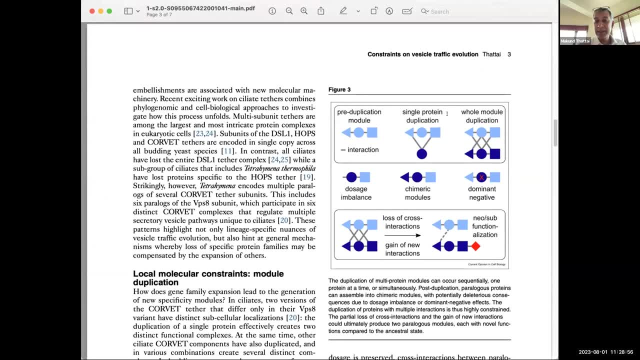 of eukaryotic evolution. I talk about these two things: how you maintain homeostasis, how you do long-distance recycling. I talk about another piece which I didn't bring up today, which is that there's pervasive gene duplication in these systems. 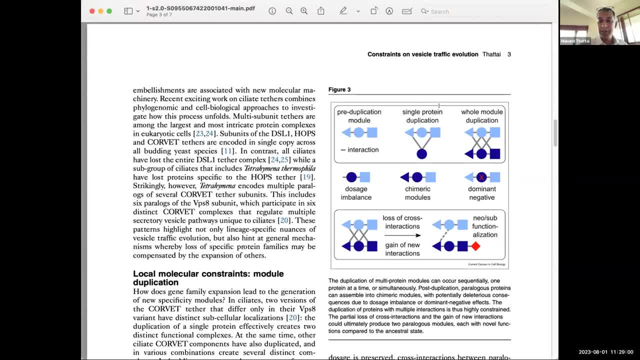 I alluded to it because of all these homologies. So how do duplicate genes actually arise and find new function inside the system? And then a few other cell biological tidbits. So it's an up-to-date reference sheet. A lot of nice papers here. 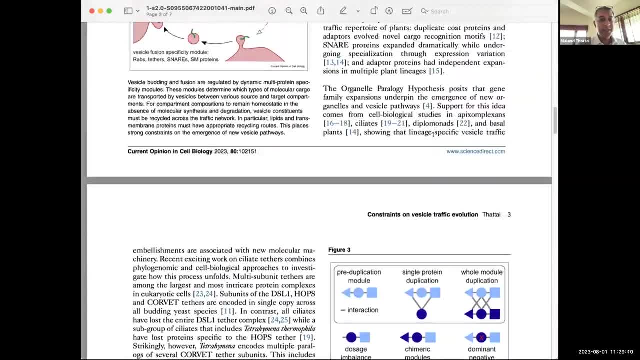 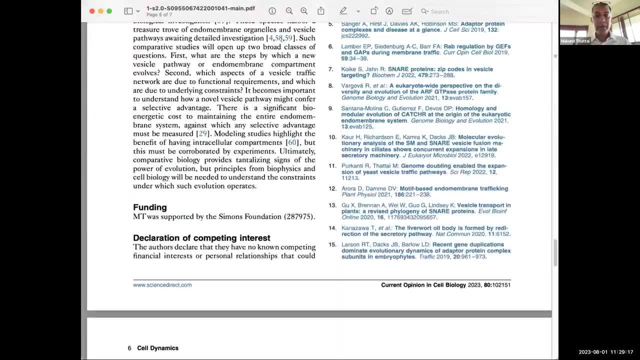 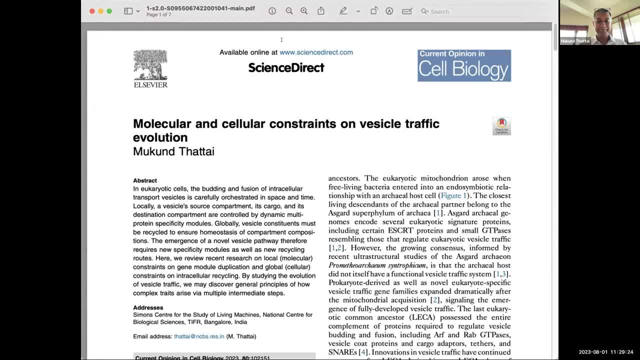 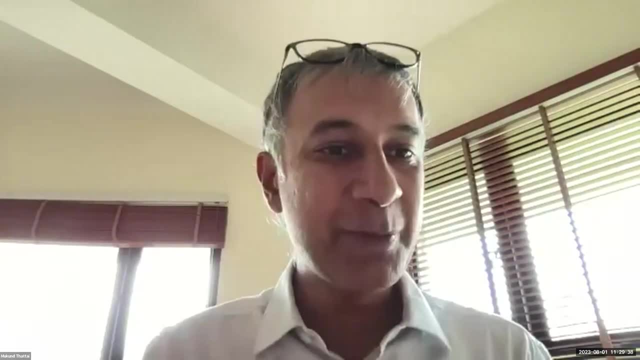 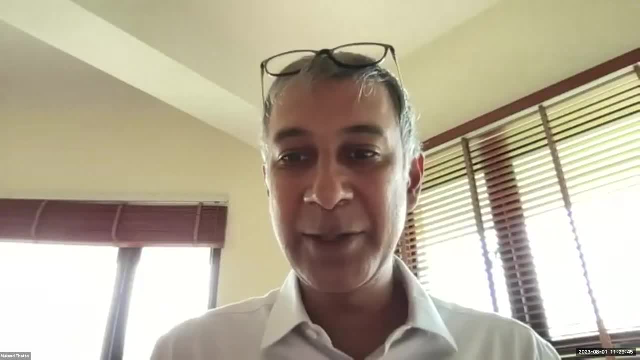 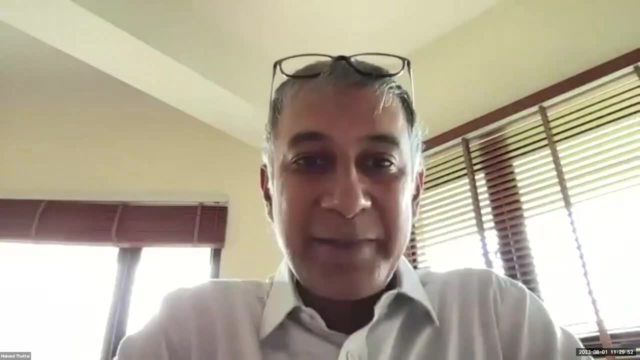 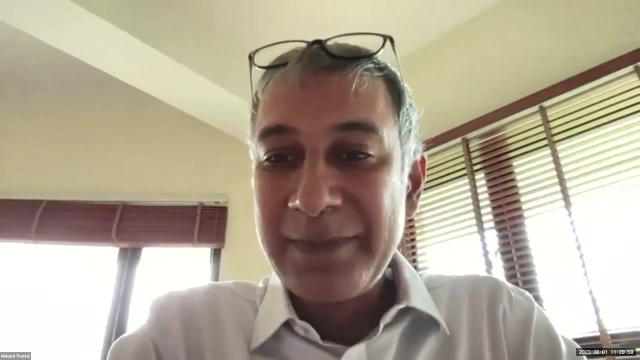 So, but I really love the questions. I think you guys are well on your way to becoming excellent computational cell biologists. Sure, If you ever want to work on any of this stuff, i'm happy to to get involved. um and and again, thanks for the the opportunity. 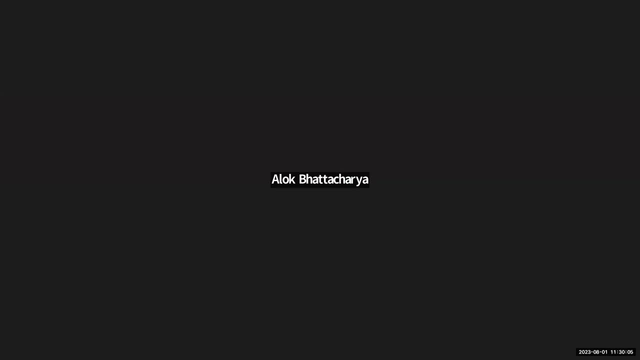 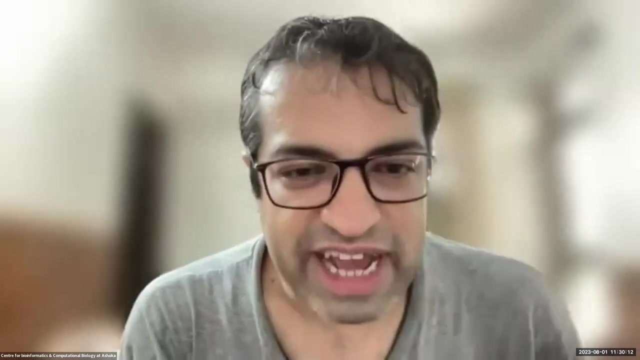 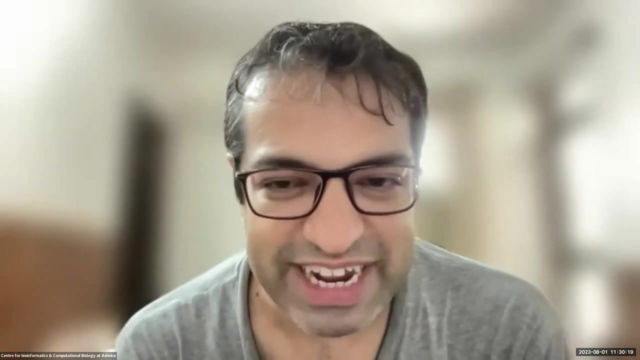 thank you, mukul, thanks, thanks a lot thanks for being here. yeah, what a wonderful talk, thank you. thank you, professor mukun, for an excellent talk and a very intricate look at uh vesicles and trafficking and trying to understand the math and physics behind them. so 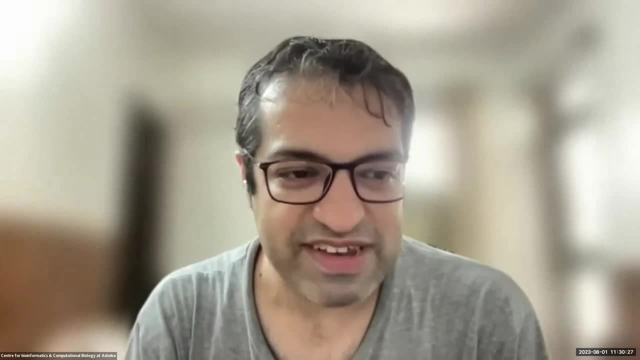 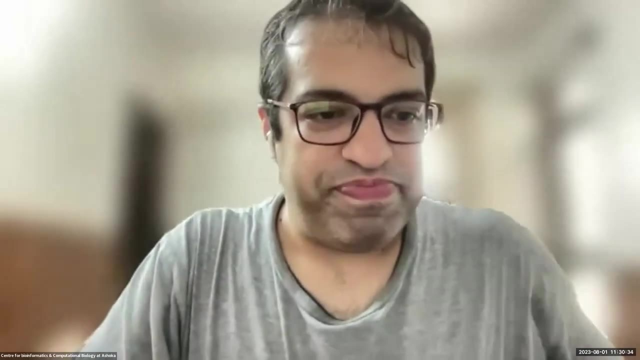 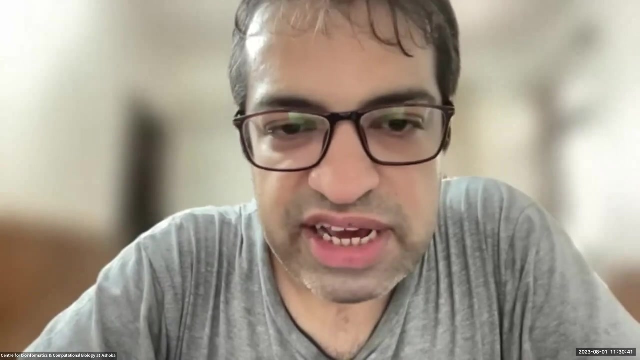 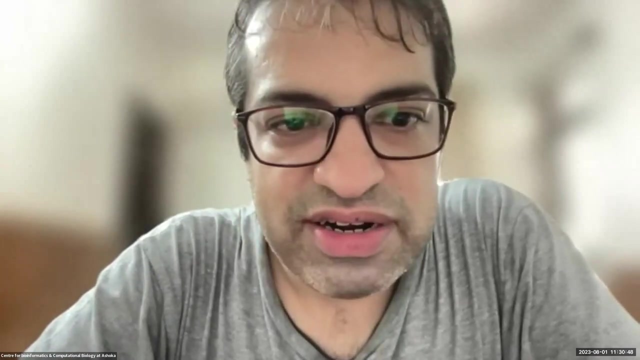 uh, thank you once again and look forward to the next edition. yep, hopefully in person, i'd love to visit. okay, bye, thank you. so, participants: uh, the next talk is by professor amitaba nandi of iit bombay, at 11: 45. we can take a quick uh 10, 12 minute break and see you at around 11: 40, 11, 45, thank you. 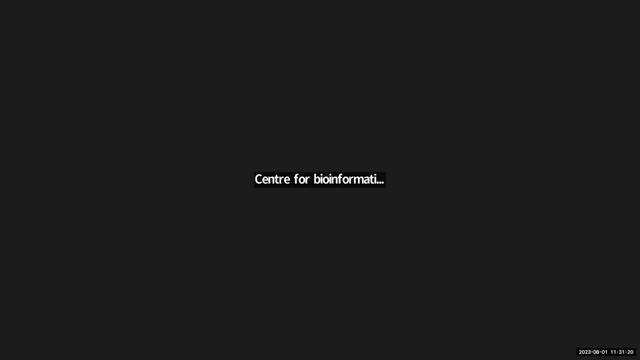 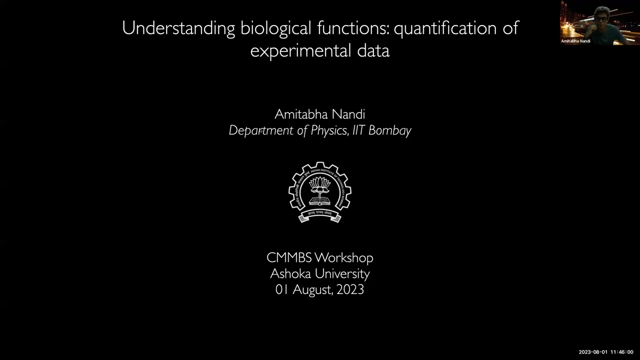 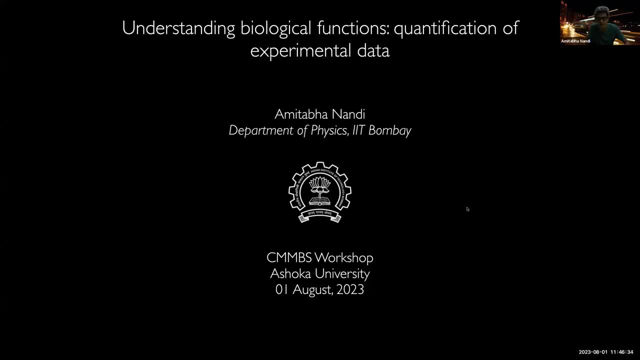 you are putting a biological system, which can be a cell or a tissue, and you, using a microscopy technique, you can track some vesicles or organelles or proteins inside the cell, or you can track several cells, their location, their, their spatial position and how they move with time. so basically, i'm talking about some kind of a spatio-temporal data. 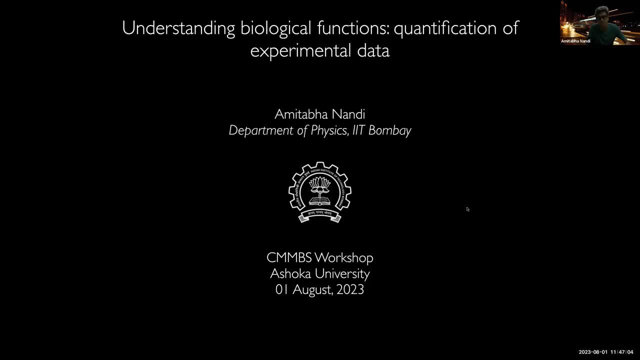 And you can basically get this kind of a time result information through the fluorescence. And now the question is, given this experimental data, how one would quantify this data so that you can get some understanding of the underlying physical processes which drives this kind of movement. 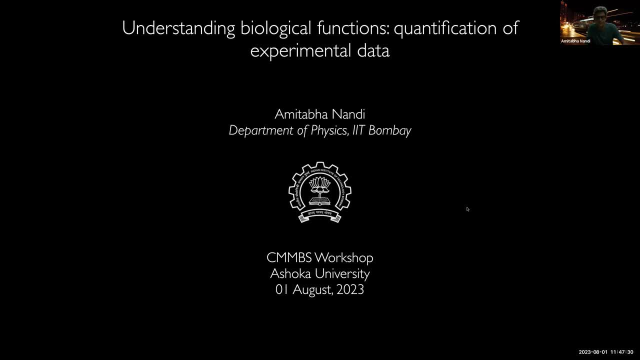 And so that is number one. And number two is: can you use some of this quantified information from the experimental data to build up a theoretical model such that when you have this model based on this quantified experimental information, you can try to regenerate some of this? 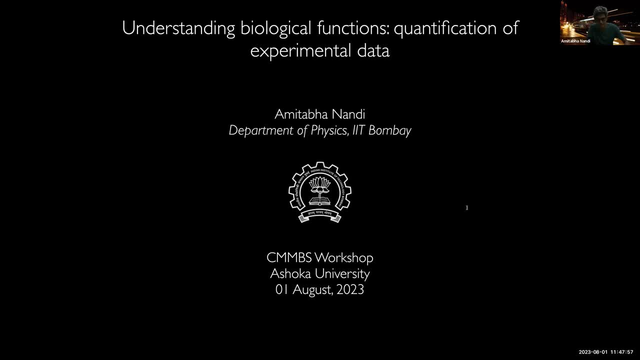 like what you have seen in experiments and then make a comparison. And finally- so this is number two- like building up a theoretical model. And number three is whether, using this combination of experimental data analysis and theoretical model, can you have some understanding? 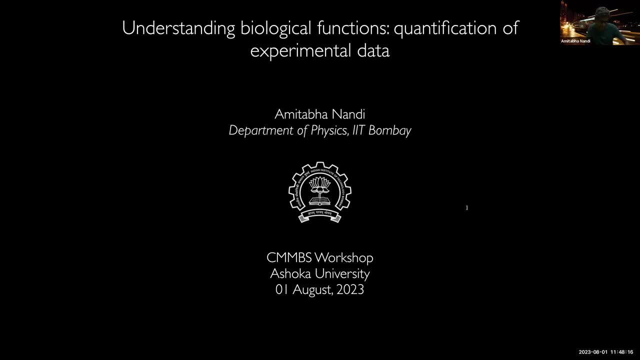 of the biological function, And here by biological function I would say that it is a little bit exaggerated, in the sense that what I mean by biological function is function at the level of whatever movements you see like. what are the outcomes at the level of individual cells or tissue? 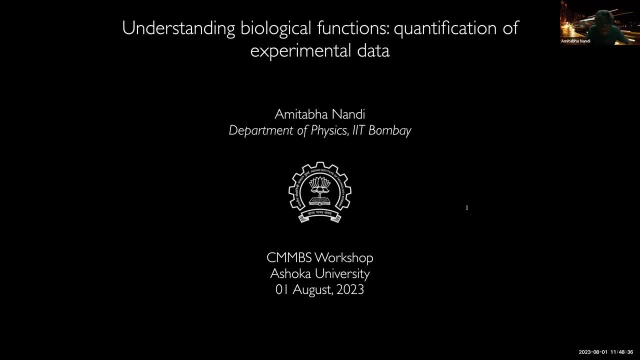 not like a much more higher complexity. So I hope I would be able to explain this idea. So I will go rather slow because this is a workshop, So it is OK, And I will try to discuss this issue or this problem through two representative examples. 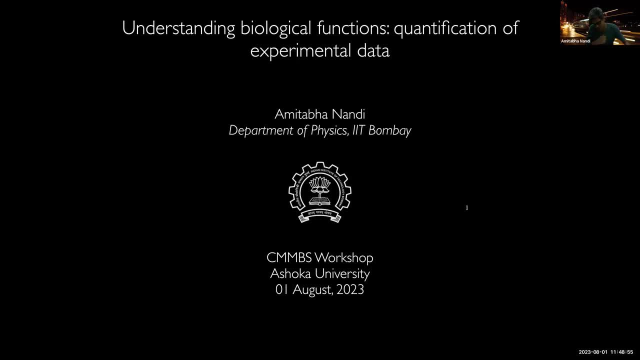 But I will mainly focus on the first example And if time permits, I will go to the second example. So please stop me If you have any questions. it's OK if I cannot finish it, So and we can take questions in between. 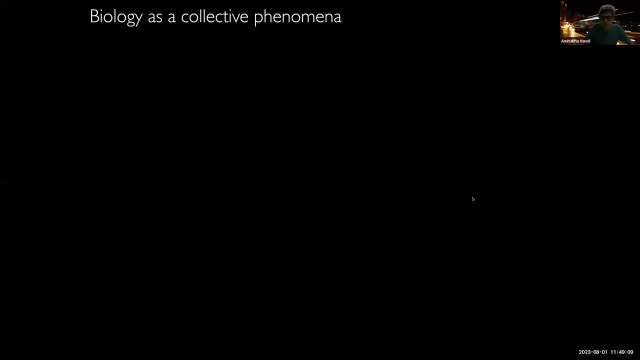 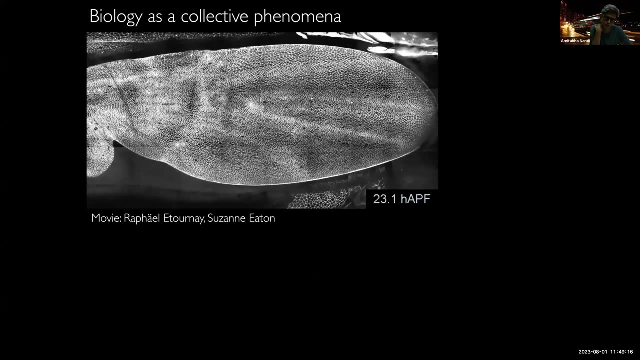 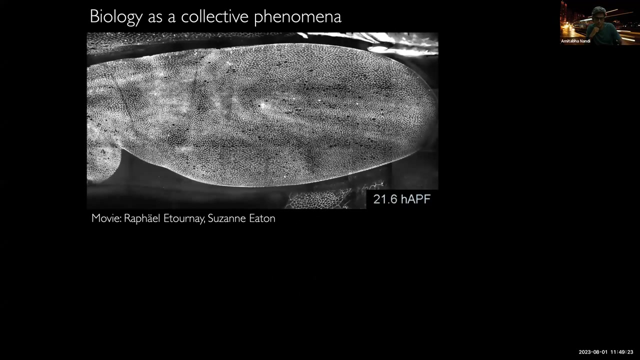 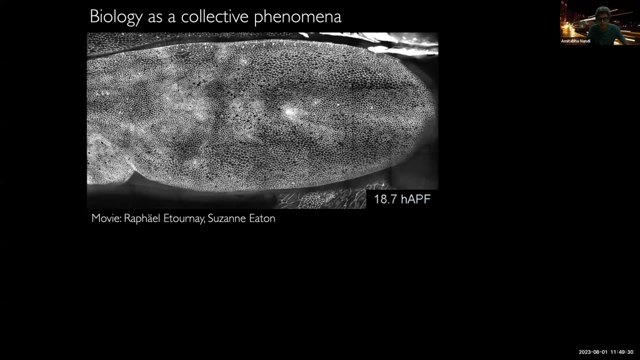 OK, So I wanted to give you an overall motivation of what we are interested as physicists, So I usually show this slide or this movie all the time. So this is a movie from experiments And what you see here Is the wing of a fruit fly at the early developmental stage. 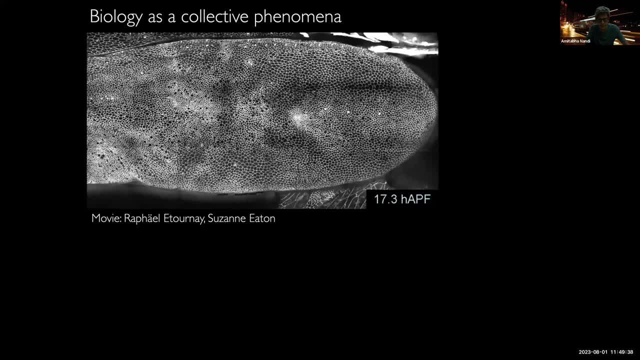 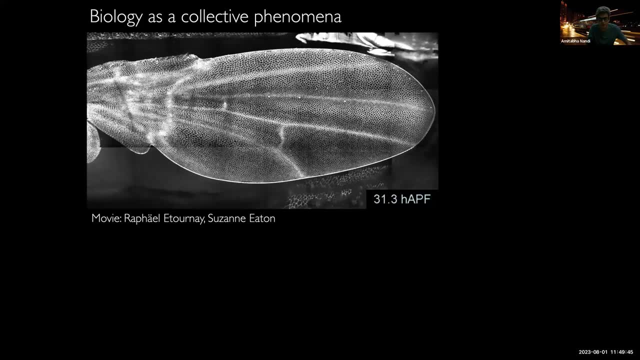 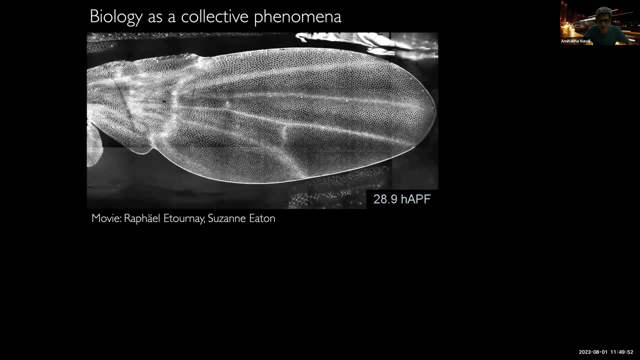 at 16 hours, after the PPRM formation, And what you are seeing is how this wing shape evolves over time, over a very long time, over a span of 16 hours, And what you see here are these polygon-like structures, which are the individual cells, because some proteins at the boundary of it Over this very long span of time, And what you see is a nice pattern emerging. You can see the wings And you see collective cellular flows from the right to the left And everybody can see the movie right. So the movie is looping OK. So the question is, if we think, if we could have zoomed inside a single cell, we will see the dynamics of a lot of proteins and organelles and things like that which are responsible, which are essential for the functioning of a single cell. However, if we look at many such cells, it is because of the interaction between these cells. we see that there is emergence of new physics. We see these emergence of shapes, And this is something which, as physicists, we are interested in how a collection of entities, when you put interaction between them, how they lead to emergence of new physics. So the question is how one can understand biology as a collective phenomena, And what in our group we are interested is to study some of these properties. 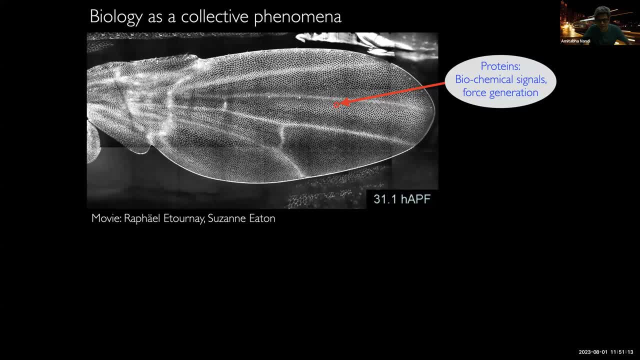 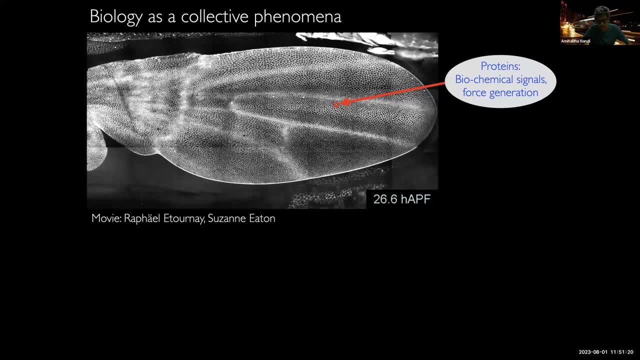 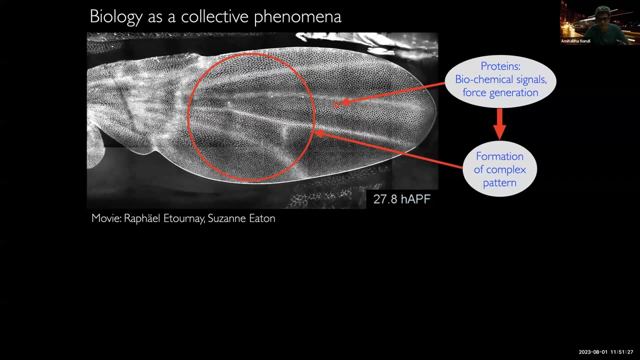 using theoretical methods from statistical mechanics and nonlinear dynamics. So this was kind of an overview. So let me come to the problem, or the problem which I wanted to discuss, And it might be a good idea to give some kind of an overall plan. So if you think of that, as I started with, 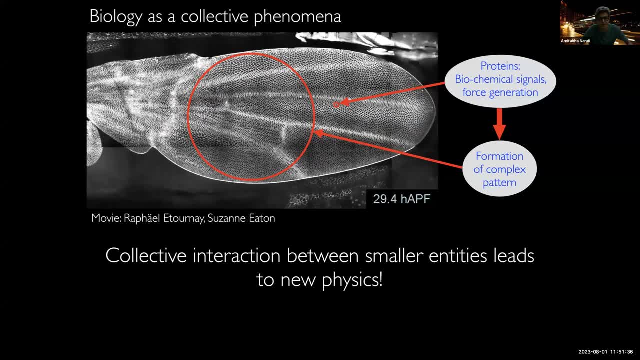 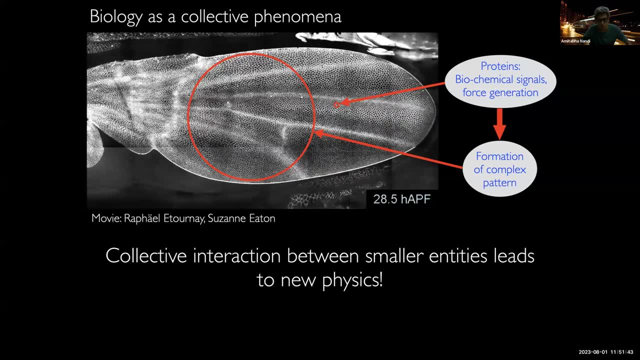 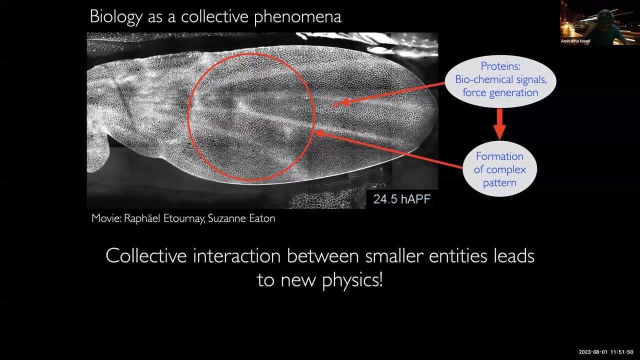 that, as an experimentalist, you have some experimental data. Now the question is how you can quantify these experimental data and use this quantified information to build up a model, but which can explain what you see in the experiment. But you don't want to stop there, in the sense. 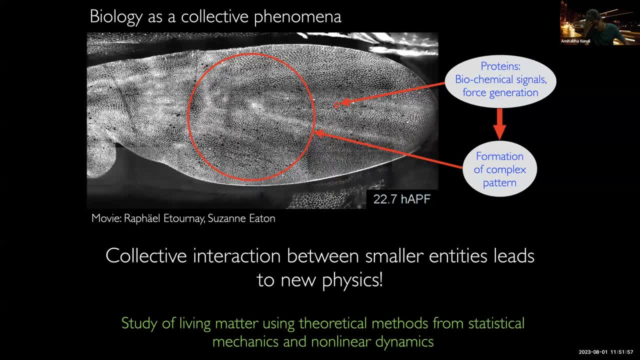 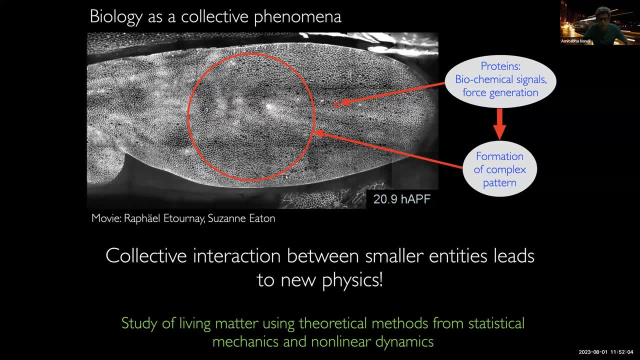 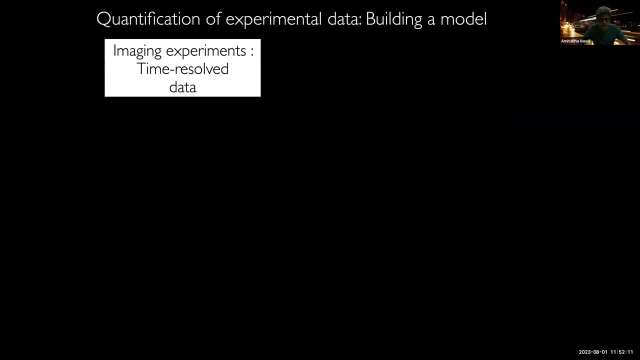 that you also want to now use this model. model because to test some hypothesis you can tweak the parameters, change something and see if it leads to some new predictions, And the idea is if some of those predictions can be tested back in the experiments. 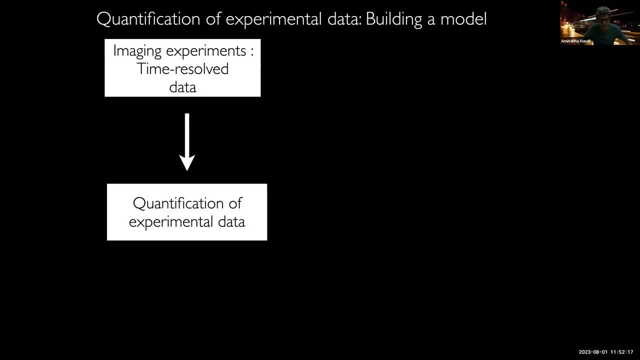 So this is one part. The second part is: whatever model you can build up based on this quantification of experimental data. you want to ask the question that if you can actually identify this model as a subset of a more general theoretical framework which can be identified, 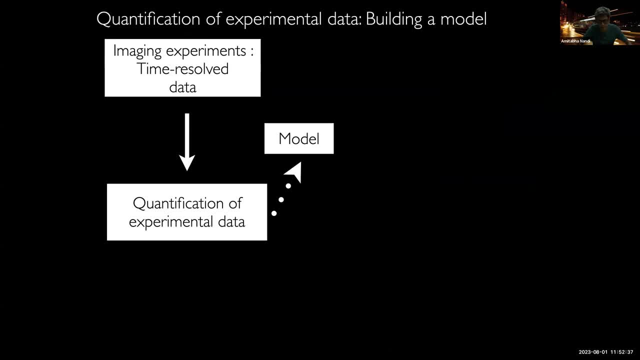 and applied to a large class of similar systems. So this is the main idea And we will try to study this through these two representative examples. The first one is kinetochore capture in fission yeast, which is an essential part of cell division. 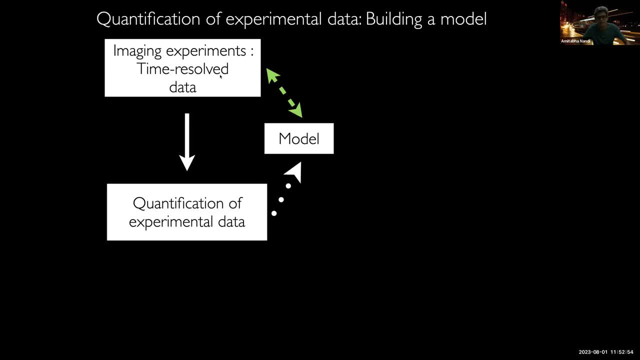 And the second one is looking at axonal transport in C adenine. OK, So before I come or describe this problem, let me go a step forward and try to see what happens during mitotic cell division. So what you see is again an experimental movie. 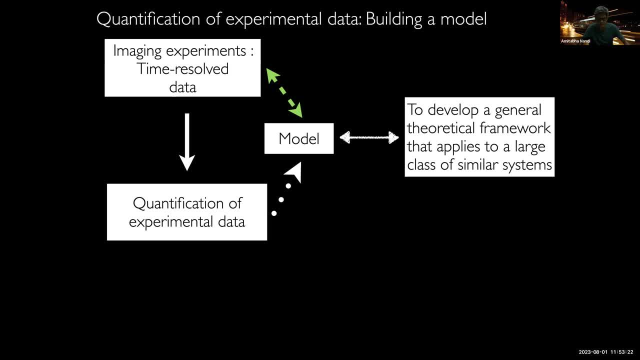 So this green structure here are made up of microdivules, And this is called the spindle, And these magenta-colored objects actually are the chromosomes. So one important function of a living cell is to distribute genetic material, or chromosomes, identically to the two daughter cells. 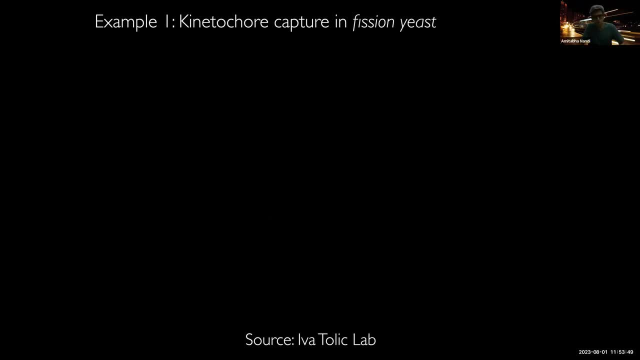 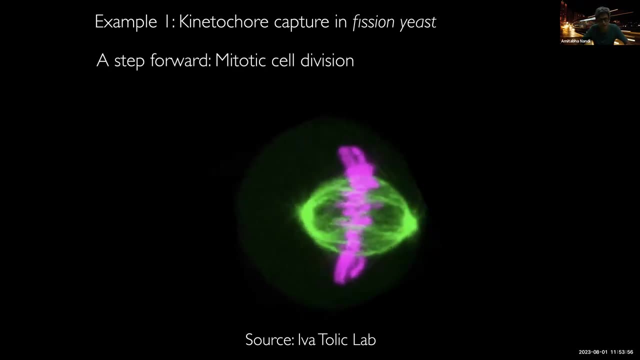 And the mother cell does this by forming this nice spindle structure which is made up of microtubules, cross-linking proteins And other motor proteins. And then these chromosomes are aligned along the equatorial plane of this spindle. And once this has been aligned, this spindle actually. 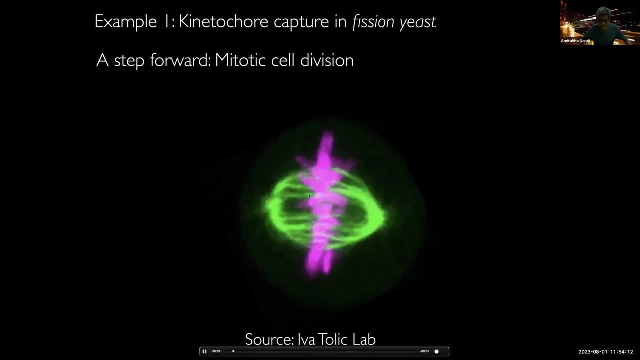 pulls apart, stretches, as you can see, and divides these chromosomes into the sister chromatids And then the cell divides And this material is identically distributed in the two daughter cells. And this whole study of spindle morphogenesis. it's a very exciting field. 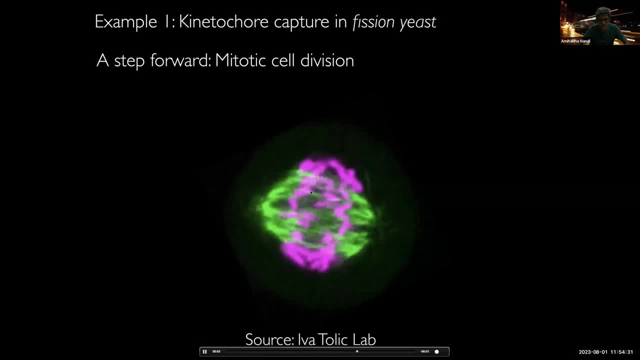 Now, what we are going to discuss today is not how this mechanism of spindle morphogenesis takes place, but a step backward, Namely the following: that, once this spindle is formed, if we look at a cartoon of the spindle, what we have, 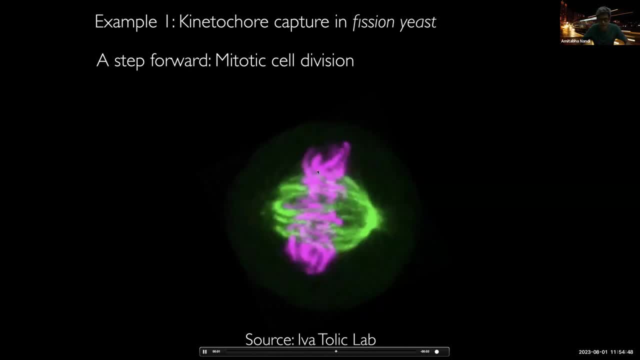 are these microtubules, which has formed this nice bridge-like structure, And these two objects are the spindle-pole bodies from which these microtubules nucleate, And these are the chromosomes. And these chromosomes has these small dots on their body. 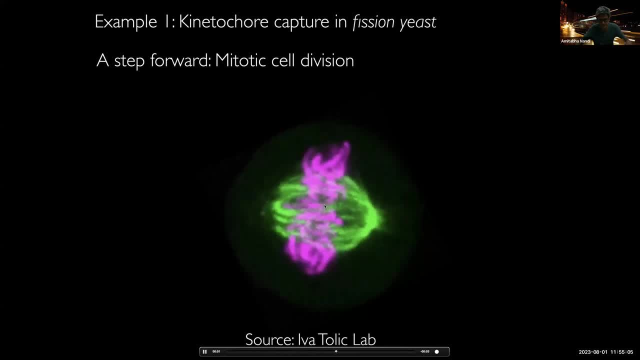 These are protein complexes which are called kinetopores. Now, one essential part that this cell divides is that it forms this spindle in right time in time- comparable or less than the cell division time- so that it can divide in a realistic time. 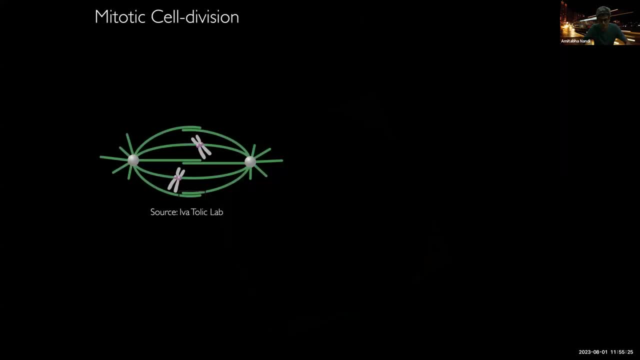 Now the question is: before the spindle forms, there is another important step, And which is the following. So I have explained these different components. So, before this spindle, this structure is formed, one important part is these microtubules. 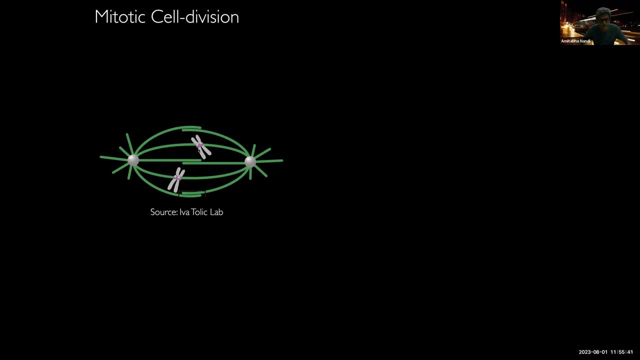 which grows out of this spindle-pole body. They capture these chromosomes which are floating in the bulk, And the question is how these microtubules capture this kinetopore- And this is oops, sorry, And this is a very important question in cell biology. 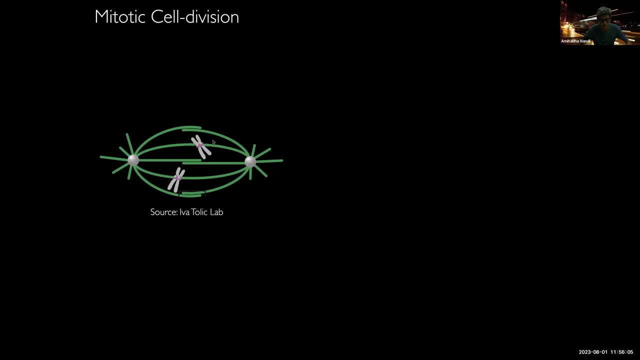 So, depending on the kind of the cell, the mechanism by which this capture of chromosome to the microtubule happens can vary. But there are some like Common methods which are predominant in many cells, And one of them I'm first going to describe. 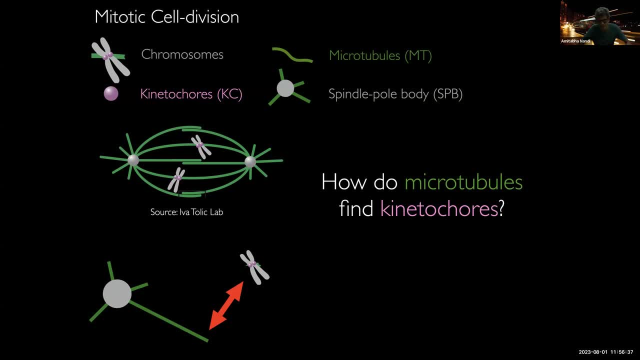 And that is this, something called dynamic instability-based search and capture. So what is this? So you can see this cartoon, So you have this spindle-pole body And there are many microtubules which are growing out of this spindle-pole body. 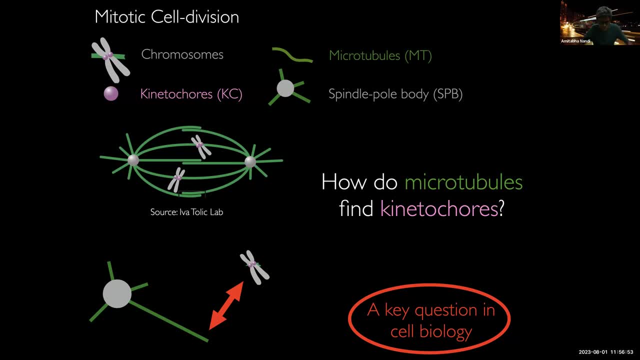 And these microtubules are dynamically unstable, So they can grow And they can go to a state where they start shrinking And using this. so basically, what they can do is they can randomly grow and shrink in some direction, And you think that this kinetopore is also 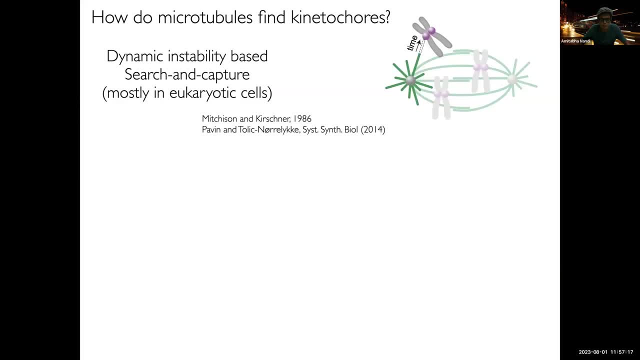 like moving in the bulk cytoplasm And whenever this microtubule comes within the close proximity of this chromosome, it attaches to this kinetopore OK, And a capture event has happened And one can actually write down a model. 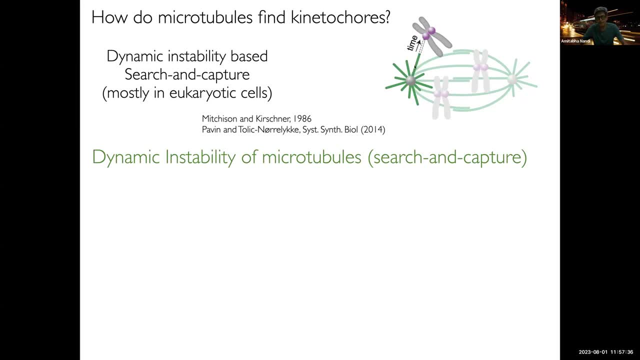 for this dynamic instability of microtubules. So this has been very well studied And this goes back early back in 1993.. So you can think that when the microtubule is in the growth state it can keep on growing with a growth rate v plus. 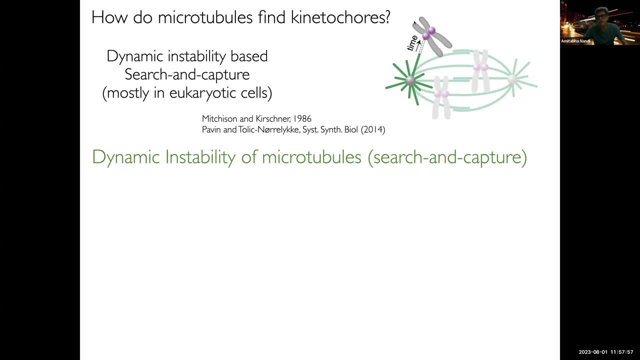 And then it can Switch to a shrink state from the growth state with a rate f plus minus, And once it is in the shrink state it can shrink with the rate v minus And again it can go back from the shrink state to a growth state with this frequency: f minus plus. 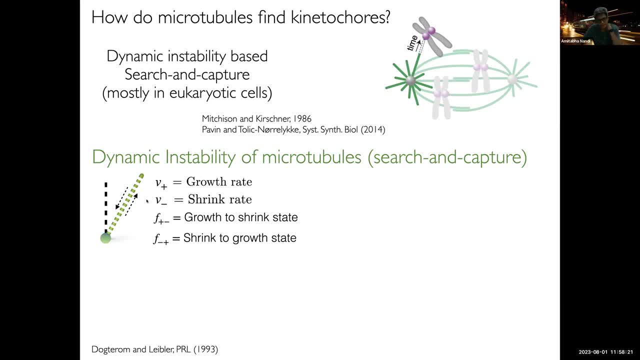 So this is a very minimal model And one can, using these known parameters, perform a computation, A simulation of these dynamics, of this microtubule growing and shrinking, And it can look something like this, the simplest one, where what will happen is you have a microtubule growing. 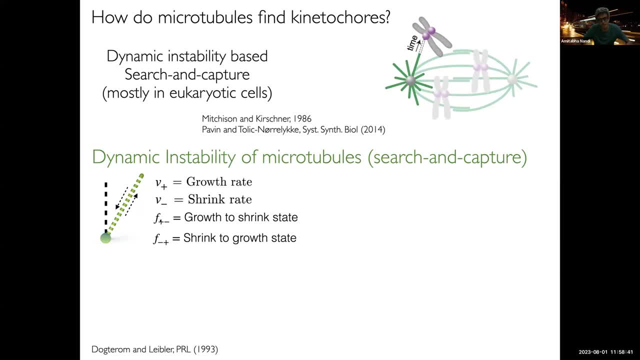 When it switches to a shrink state, it shrinks all the way And then, once it has shrink all the way to this nucleating point, it again starts growing, but in a new direction. And that is again grows. And because this is a stochastic process, this length of growth, 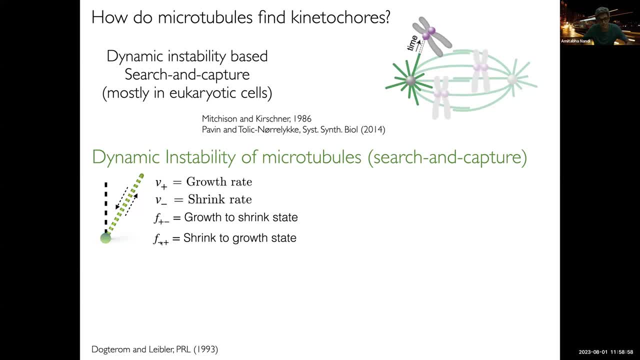 can Be different And this is as I said. this is the simplest model. I am allowing the shrinkage to happen until it reaches the spindle pull body. One could have had something like a rescue rate where it can recover to a growth state sometime in between. 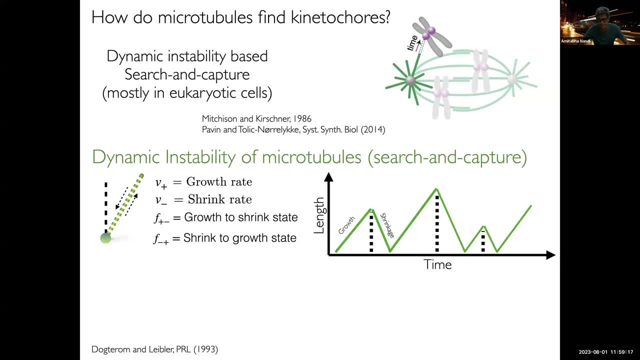 And one can study these computationally, generate the length trajectory like the length of a. I think there is a question. Yeah, please go ahead. You can switch on your mic and ask me the question. I cannot hear anything actually. 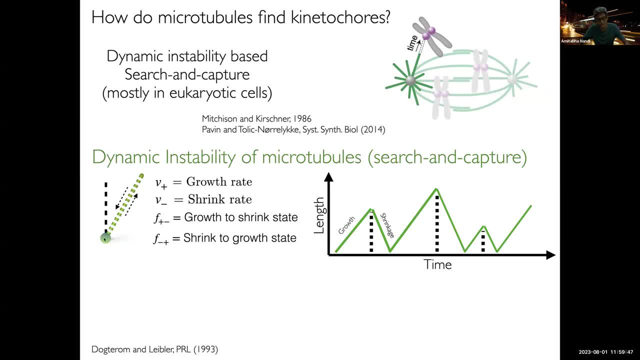 So maybe just some. any is there a question? If there is, please either speak it out or type it out. If you can't speak, OK, then if there is no question at this moment I can continue, But if somebody types, you can tell me the question. 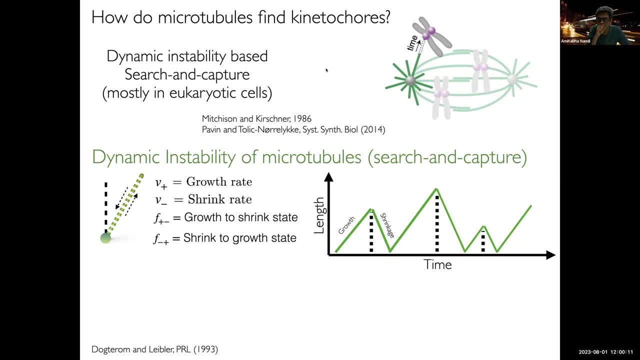 We'll do so. yeah, OK, OK, So, yeah. so this is something which has been well studied, And one can use this information and perform Monte Carlo simulation- kinetic Monte Carlo simulation. This is also known as the Gillespie simulation. 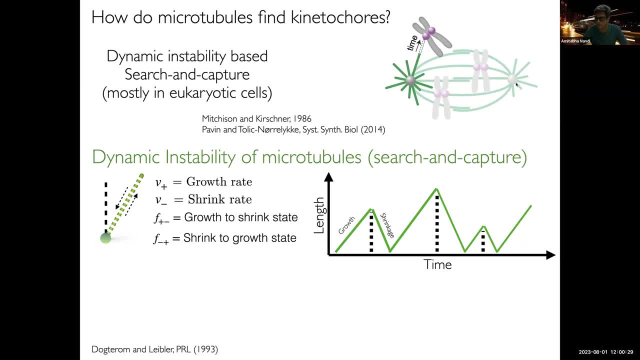 which might be already well known to many of you. One can also write down an analytical formula for the time evolution of the probabilities of these microtubules, either in the growth state, which is called p plus, or in the shrinkage state, which 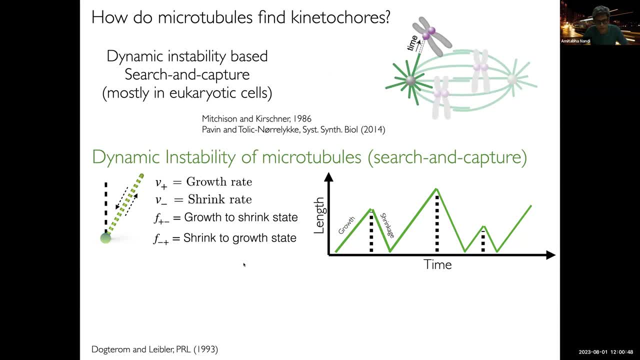 is p minus, And you can see that when it is in the growth state, it grows with this rate b plus. When it is in the shrinkage state, which is p minus, shrink state, it shrinks with the rate b minus and this gives rise to some kind of an advection term. 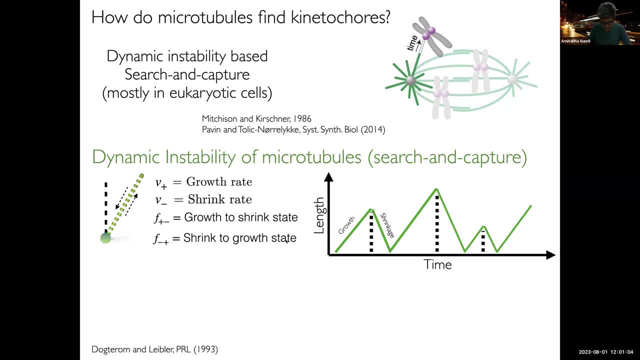 or which is like the first term on the right hand side in both the equations and the third term. and the second term in the first equation is the rate of switching to a shrink state, which comes with a minus, and the gain term, which is because of switch to the growth state from the shrink state. 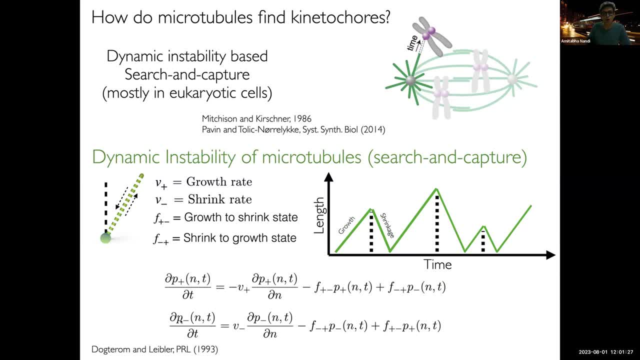 and similarly these two. the last two terms comes in the second equation with opposite sign, as expected. so one can also study this: if time evolution of this length of the microtubule through these equations for the time evolution of the probabilities in either the growth state or 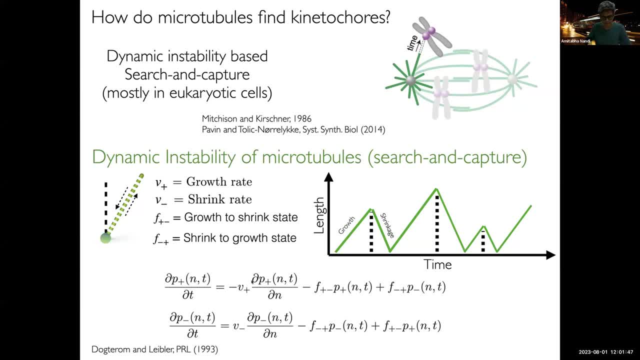 the shrink state, So I will not spend time on this. so this is typically a mechanism of microtubule growth and shrinkage which has been dominantly seen in many eukaryotic cells, and the idea is like you have many such microtubules growing. when one of them comes in close proximity of this chromosome they attach. 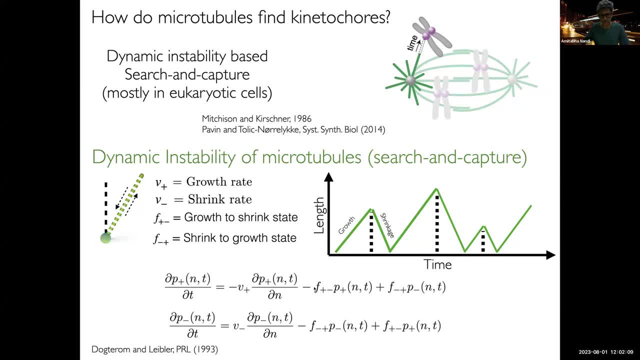 to these protein complexes which are called the kinetochore, and then the capture has happened and then one can go to the next stage. So right now we are interested only in this capture process. Okay, I think there is a question. I had a quick question, So is it like kind of exploring different ones before? 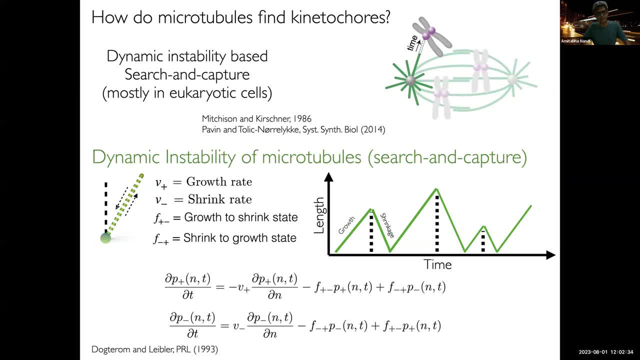 capturing a particular one, like does it like, come close to one, then maybe decide not to bond to it, and then, like, go and explore another one and then decide to attach to them. Yeah, so I think it's a good question. I think it's a good question. I think it's a good question. 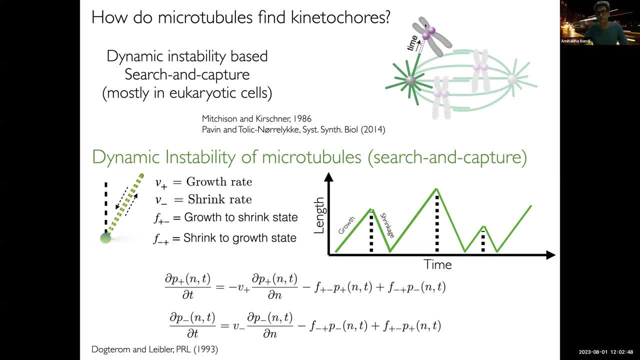 So the thing is, those are more complicated processes. Yes, there can be different, complicated processes, like actually, like the, really the mechanism of how this microtubule, once it is at very close proximity, it binds to the kinetochore. Right now we are not interested. 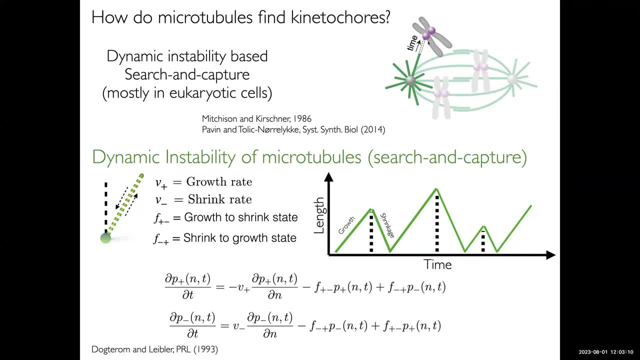 with those fast time scale processes or those details. So we are assuming, within this framework, that whenever they come within like a very close proximity, there is a instantaneous capture and the time scale over this over which this capture happens, it is much faster than the other time. 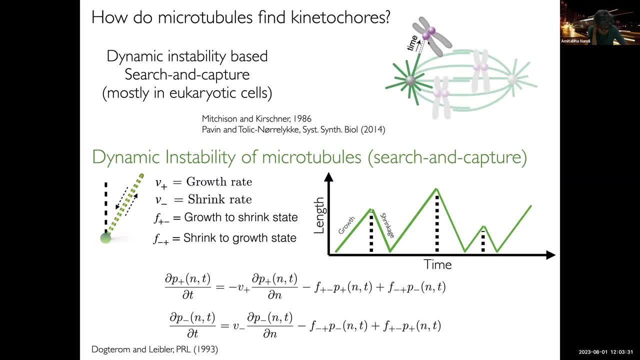 scales, namely the time scales over which you see this growth and shrinkage, or the time scale over which this chromosome is diffusing out in the bulk cytoplasm. But you are right that there can be more complex processes like I mean, how, what is exactly the mechanism of how it binds to the kinetochore? 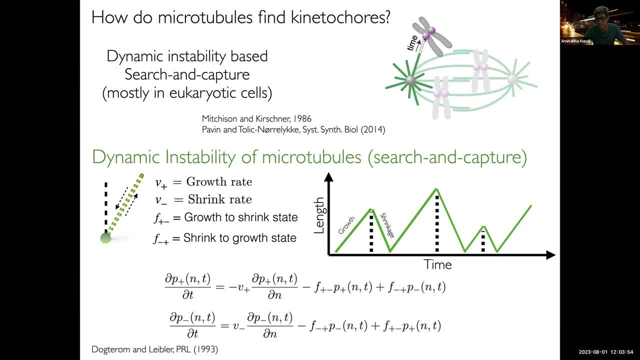 But at this moment we will neglect those really fast time scale processes. So, thank you. Does that address your question? Yes, yes, Thank you, Okay, okay, So so, so this is this is like a well-known model, and and just 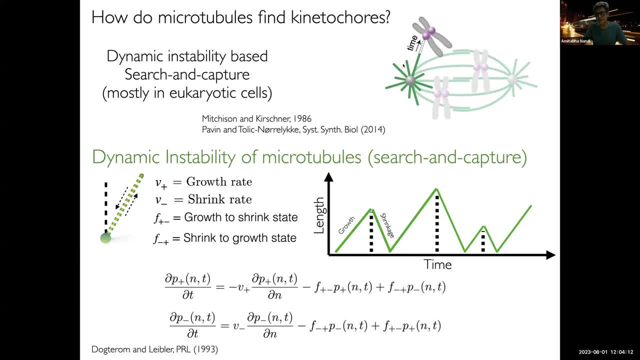 to remind you. so typically in eukaryotic cells like where this kind of mechanism is predominant, there are a lot of microtubules which are growing out of a kind of- sorry, my bad- so growing out of a spindle body. this new nucleating site Now recently- or not that recent- way back in 2013,. 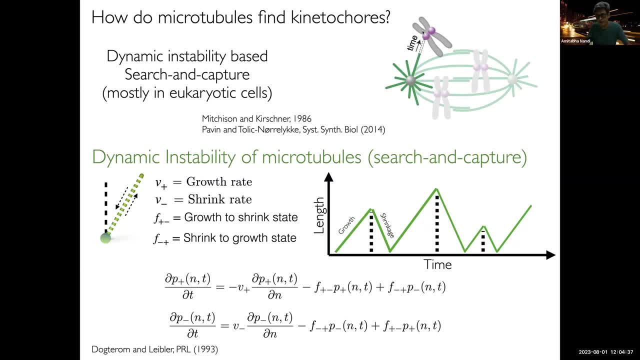 this question was asked in the context of a simpler organism, namely fission yeast. that how does this capture happens in fission yeast. So first let me give you what is the nature of dynamics of this microtubule in fission yeast. 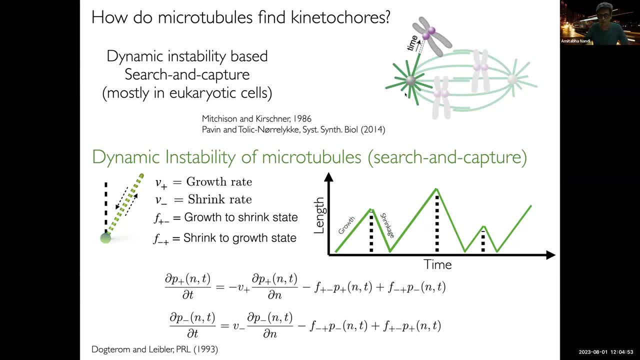 So in fission yeast the length of a microtubule coming out of a spindle body. it has this following dynamics: It first grows and then it is stuck at a pause state where the length of the microtubule doesn't change, and then it can shrink after some time And typically. 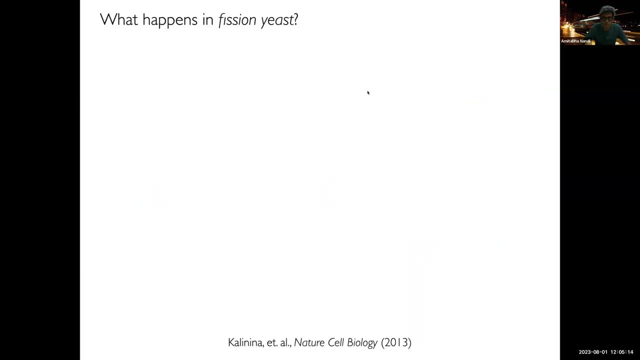 on a, the state over which this migratory wheel does not change. its length is rather very long. so where this length is not like it is like a fixed, it's like a stiff rod, And what happens? it was seen in experiments that during this state it does some kind of. so basically, this rod, 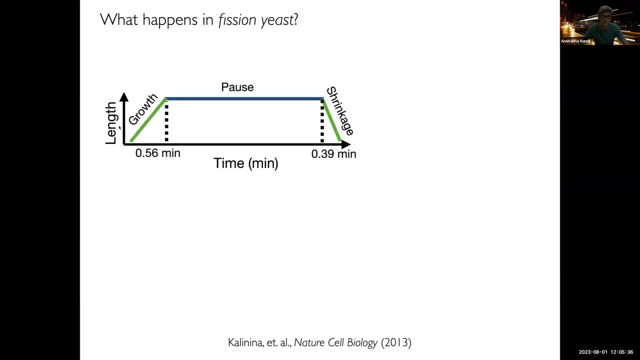 you can think it is a stiff rod. it does not have any kind of like. it is not like a polymer which can bend. so because the length is small, you can approximate it as like some stiff rod and it is like pivoted at this spindle pull body and being pivoted at the spindle pull body it is making. 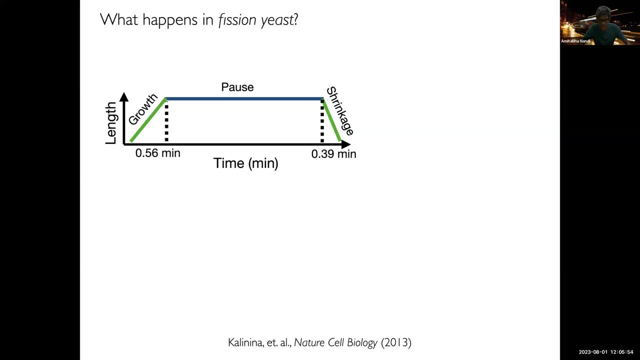 some kind of a physical movement And for the moment, let's say that we don't know what is the nature of the movement. So the question is: what is exactly like the kind of motion it is doing And it was seen in experiments. so this is from a real experiment, and if one, 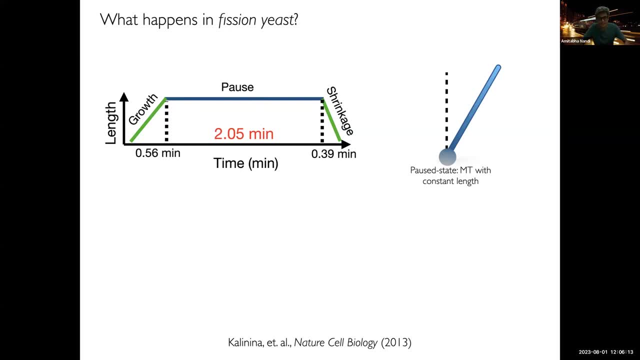 observes carefully. so this whole thing, if you see the cursor, this is the spindle pull body and this movie is looping. so this object, it is a projection, so sometimes you don't see the rod properly. but this rod is doing some kind of a motion which, if you follow the snapshots from 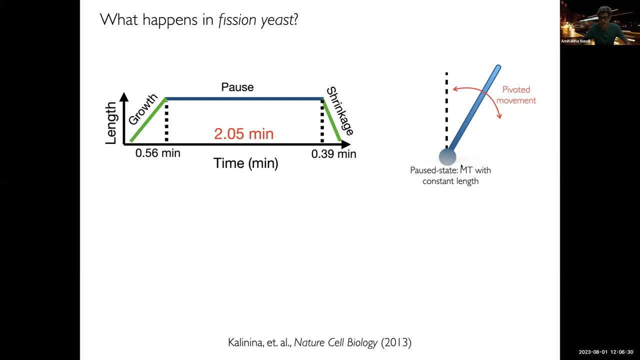 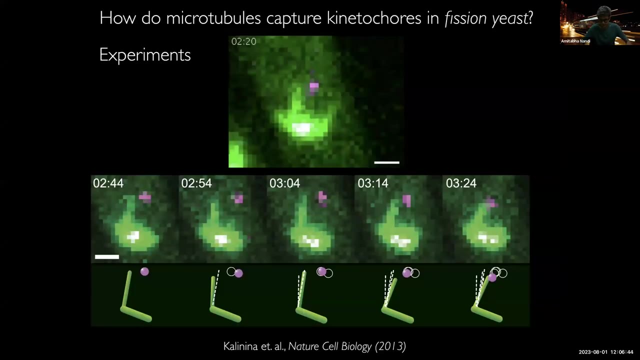 the movie you can see and try to build up a schematic. So there are these slight movements being pivoted at this end and the chromosome, or actually you don't see the other part of the chromosome, you see only the kinetochore, which is this magenta. 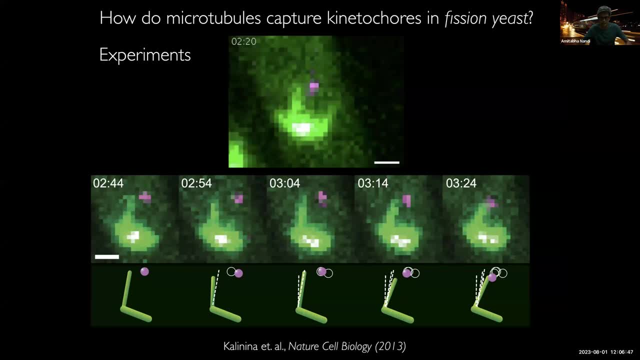 thing. This thing is also moving a little bit and one can see that if you draw a line, it is with respect to some axis, it is making some kind of a pivoted motion and whenever it comes in close proximity, this kinetochore is immediately captured. and once this kinetochore is captured, 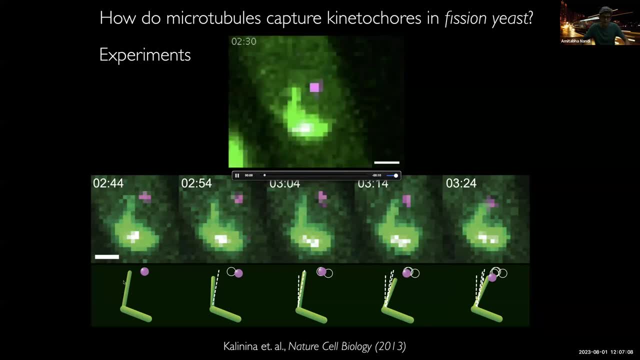 it is like really pulled very fast by that. So now the question is, as I have said in the first slide, that given this experiment, can we quantify the nature of this motion of the microtubule and also the kinetochore? 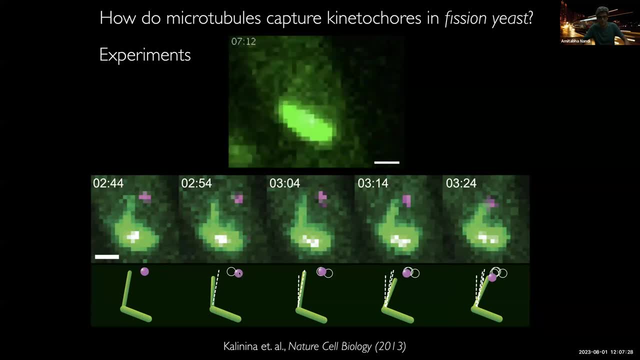 And this is the question, and we will try to do that. So first, before doing that, let me digress a little bit and give like a quick overview of how we can quantify motion in a very complex and complex environment. So let's start with something simple. So let's start with something like: 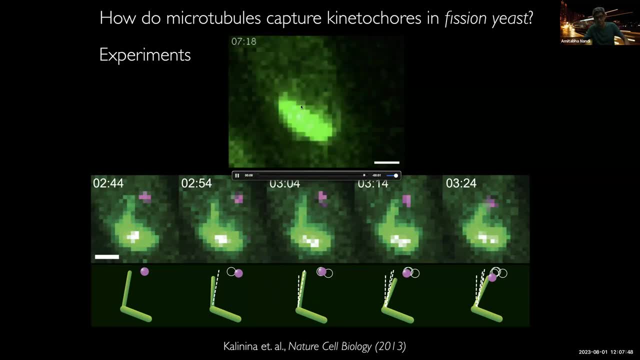 diffusion, pure diffusion in a viscous medium. So you have some particle, which is the yellow particle, and you have a background fluid which is composed of these small dots. Now the fluid is in equilibrium at some temperature T and it is getting bombarded by. 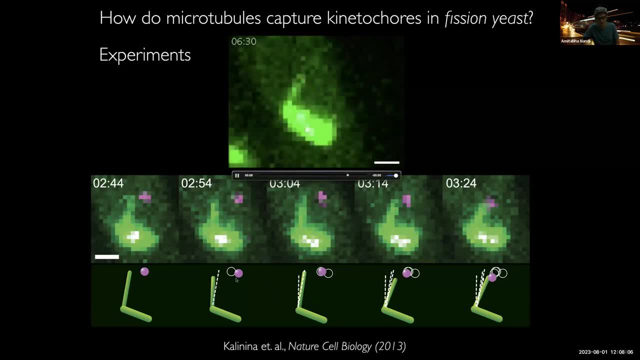 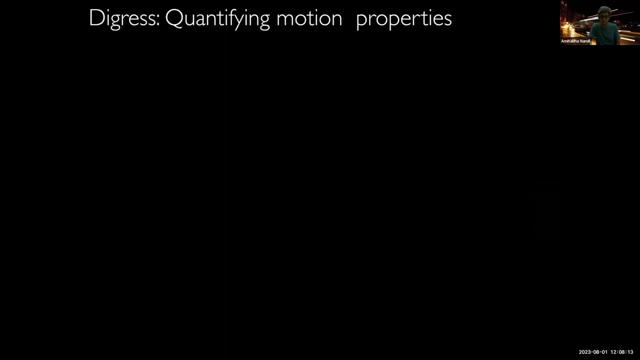 this and the bead and this yellow particle is getting bombarded by this fluid. So this is a very complex particle and it performs some kind of a random zigzag motion. So this problem has been studied very well many years back and one can write down the 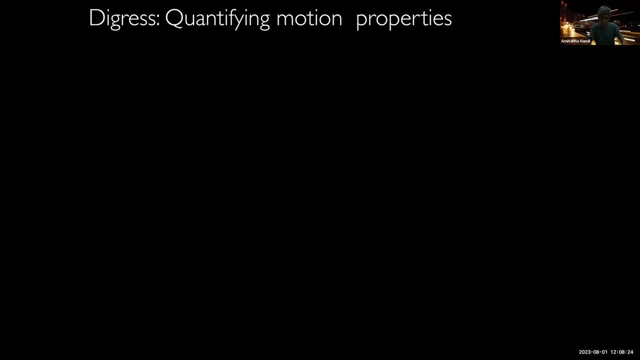 equation of motion of this particle. And what you see here is this equation of motion of the particle. There is an acceleration term, which is the first term, and then there is a friction term. It is like a frictional force because every time it gets bombarded by these fluid molecules, 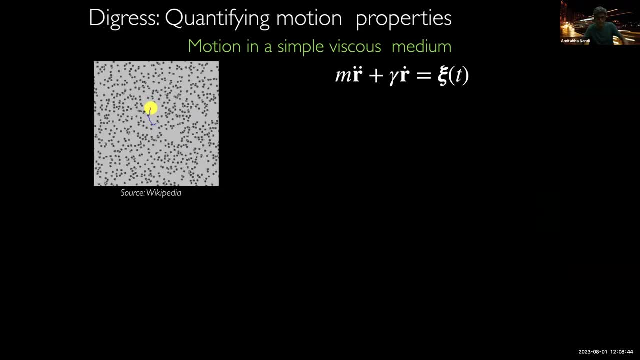 it feels the drag. and that is the second term. And the term on the right-hand side of this equation are these random kicks which this yellow particle experiences due to the fluid molecules at every instant. And these random kicks have certain property which is given by this equation. 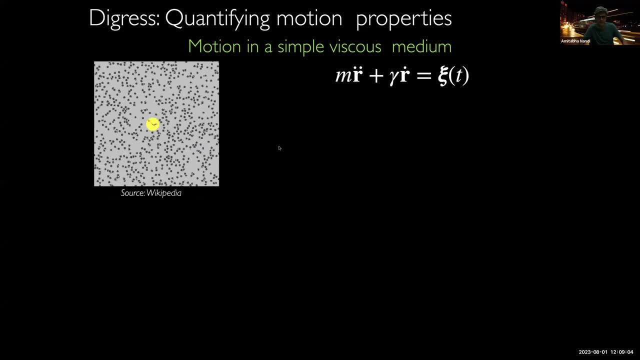 Basically they are called like: these are random forces, which has a mean zero. if you average, it is zero, and they are delta correlated. Now, as I have said that, we will consider that this background fluid is very viscous, which is typically the case for fluids inside a cell. 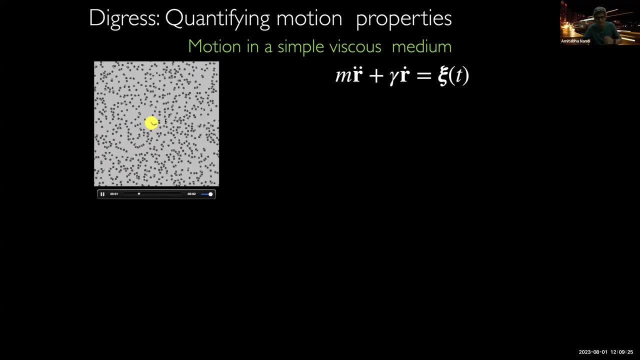 So if it is viscous, then we can drop the first term And this motion will be something called overdamped, and in that case this equation simplifies further and one can calculate something called a mean square displacement, which is this quantity: 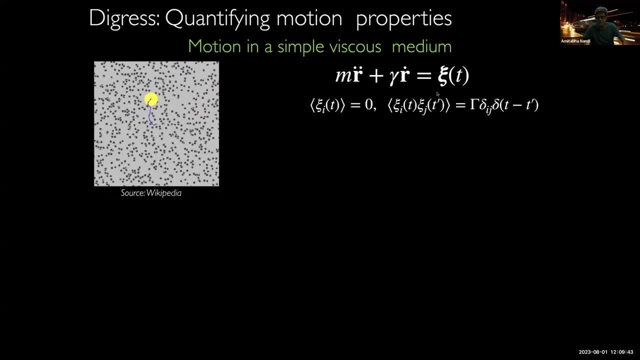 basically the square of the displacement of this particle, averaged over various trajectories or averaged over time. And what we see from this formula- I'm not going to the details of this formula- what we see is this average or this mean square. displacement is proportional to the time. 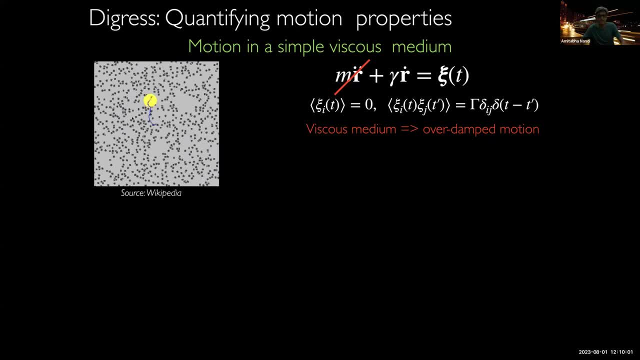 elapsed, It is linearly proportional to the time. Now. this is for simple diffusion in a viscous medium. When we have a more complex medium, this formula will be modified where it will be. this mean square displacement will be proportional to this time to the power sum exponent alpha. 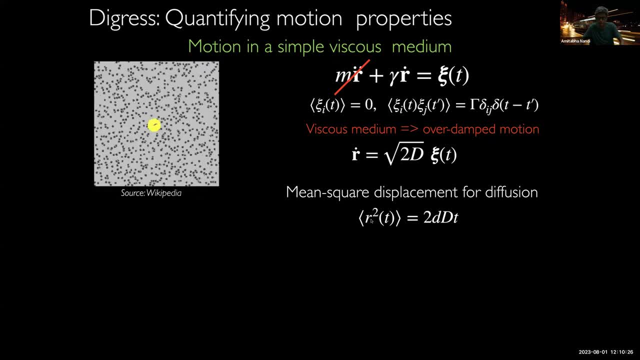 and this exponent will be one for free diffusion, as we saw in the previous example, And it can have a variety of different values. for example, if this particle is moving with a constant velocity, it is going to have an impact at any given distance, So we will have different. 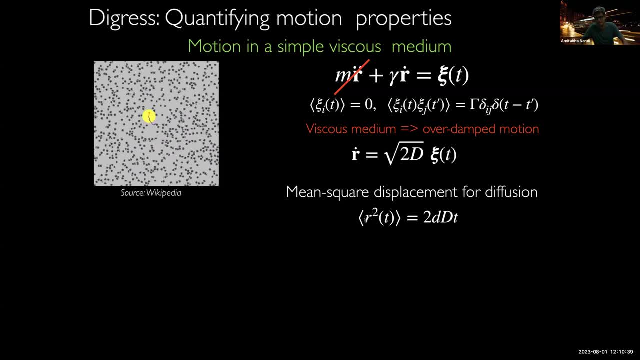 different values. For example, if this particle is moving with a constant velocity, it will will have an exponent 2.. If this medium is very crowded, it is bumping into obstacles, then this exponent will be less than 1.. If it is like a medium where sometimes it 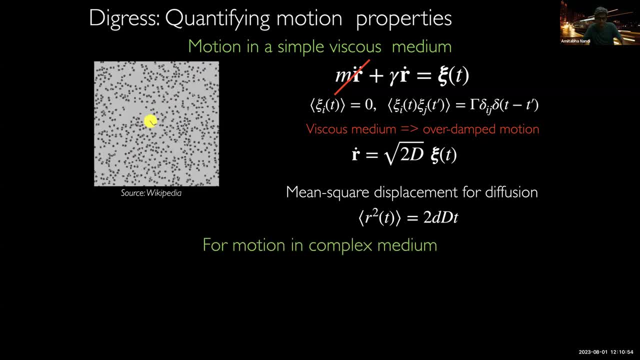 moves with some velocity, sometimes it bumps into obstacles and sometimes it diffuses. it can be something in between 1 and 2.. So it can be a range of values depending on the background medium, And here is the important part. So if I am able to calculate this quantity, 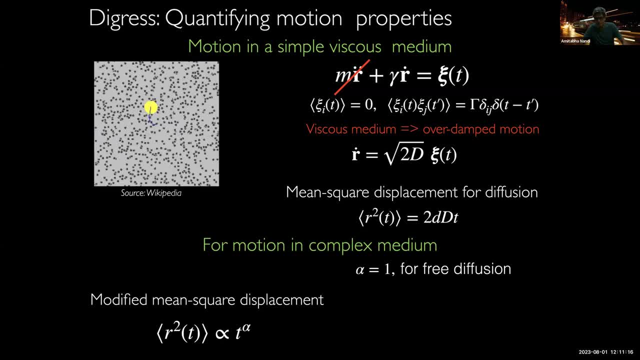 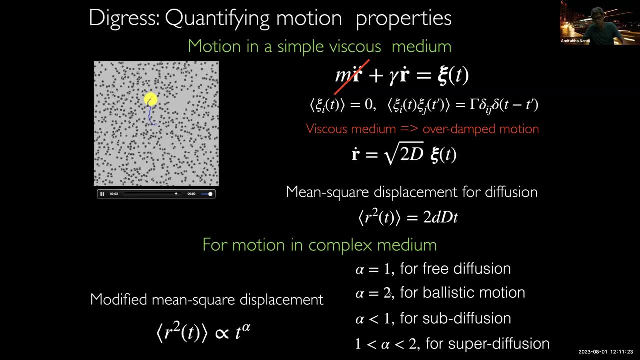 from experimental data, by measuring, by looking at the variation with time of this quantity and what is the value of this alpha, I can tell something about what is the nature of this medium And that can help us in building up a model. So this is the main idea. 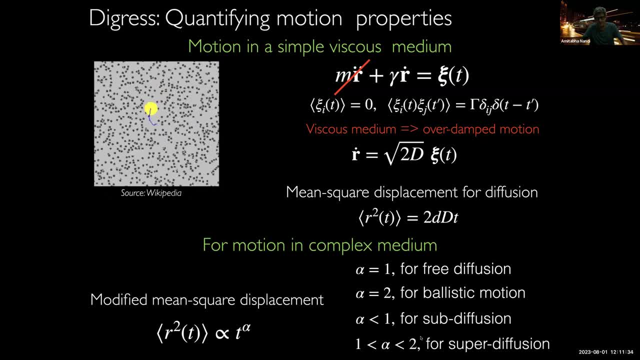 So what we'll try to do is we will try to calculate this quantity for this microtubule doing a pivoting motion and this kinetochore diffusing field. Let us see. So what we can do is we have this microtubule. 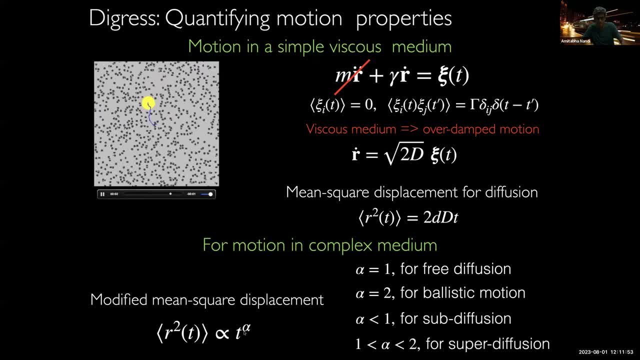 We can choose an axis and measure the angle theta with respect to the axis and measure that angle theta as a function of time. And once we have measured this angle theta, we can calculate that Square of that theta over various trajectories and plot it as a function of time. 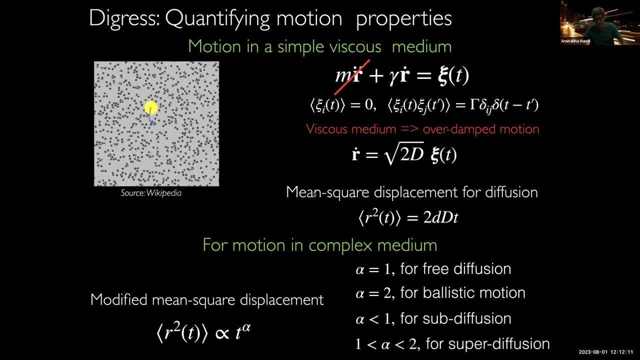 And if we plot that as a function of time- this is what has been plotted here- These dots with error verse and you see that it actually you can fit a straight line, which means that it grows linearly with time. So it tells you that this rod or this microtubule, 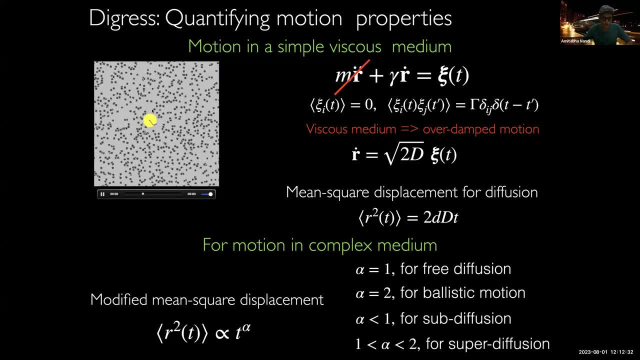 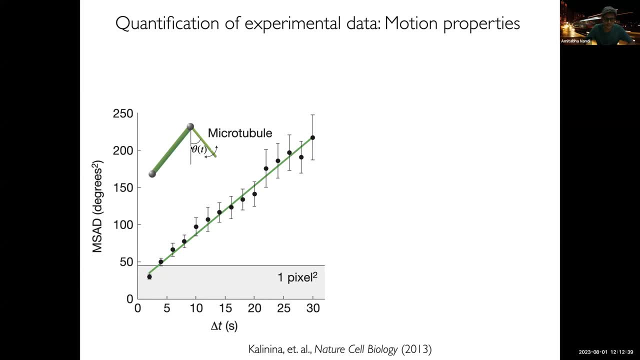 with a constant length. it is getting bombarded by the background fluid molecules And it is performing some kind of a rotational diffusion. It is rotational diffusion because the other end of the microtubule cannot detach from the spindle pull body. It is always attached there. 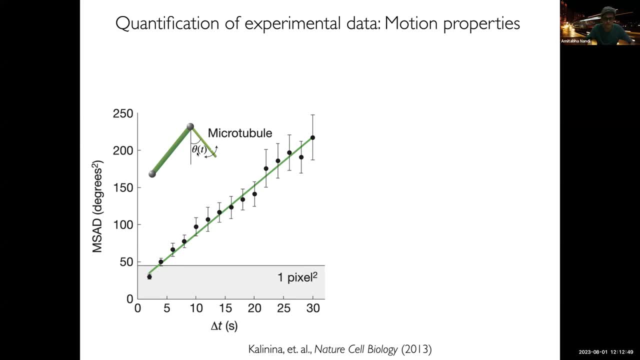 And this rod is getting kicked by these fluid molecules and being hinged at one end it is doing a random motion. So basically, from this information, if you fit a straight line to this data, which fits very nicely, The slope of this feed will give you the diffusion coefficient. 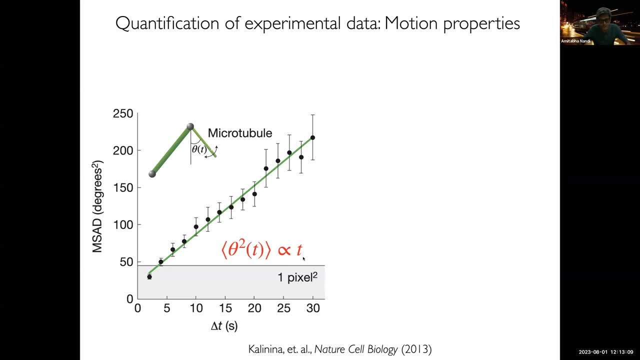 or rotational diffusion coefficient. So this is something which you can extract from experiment. Good, What about the kinetochore, or the chromosome which is diffusing freely? What we can do for that is, we can look at that fluorescent point and mark the position at every time and record the position. 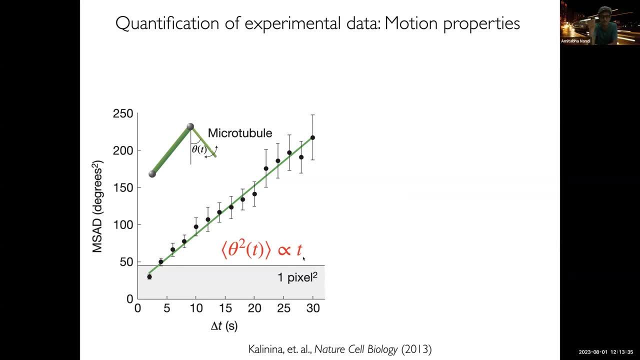 And that will be some r of t. And then we calculate again the r square averaged over different trajectories and plot it as a function of this time elapsed. And here also we see that if we try to fit this data, of course at large times there are some variabilities. 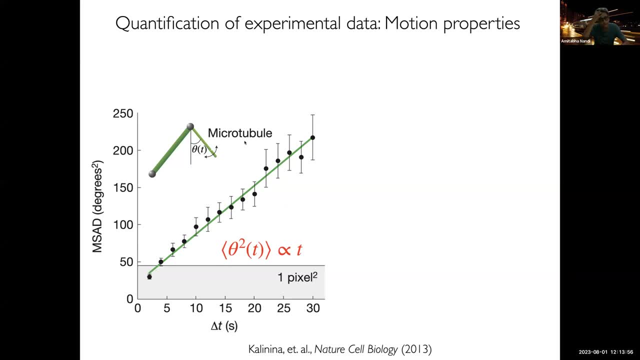 There are some fluctuations in the data But still we can fit this data with a nice straight line which tells us That this kinetochore is also diffusing freely within the bulk fluid. And if I calculate the slope of this fitted straight line, 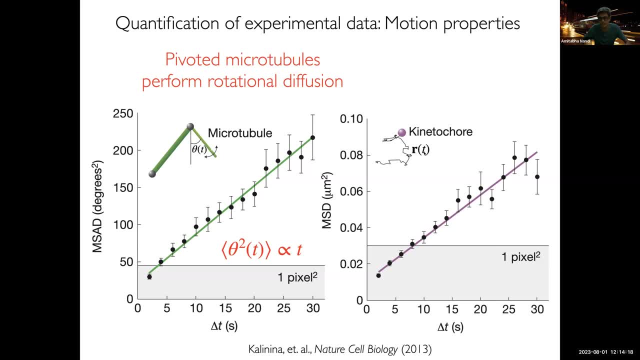 that will tell us what is the diffusion coefficient of the data. So I have got two pieces of information from the experiment That the microtubules are doing a rotational diffusion. The kinetochores are doing A free diffusion within the bulk space. 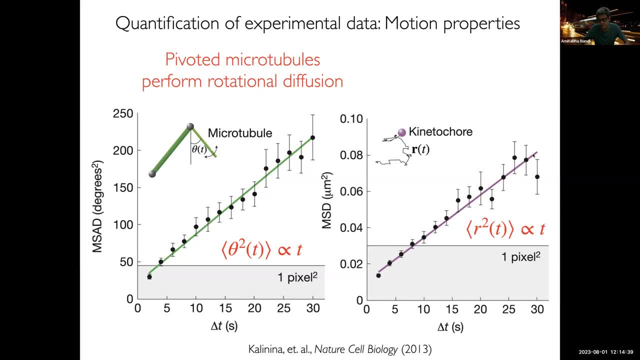 which means that whenever they come within a close proximity, there will be a capture. So basically, using this information, I can try to build up a model And let us see how we can do, But before that we also need to look at some statistics. 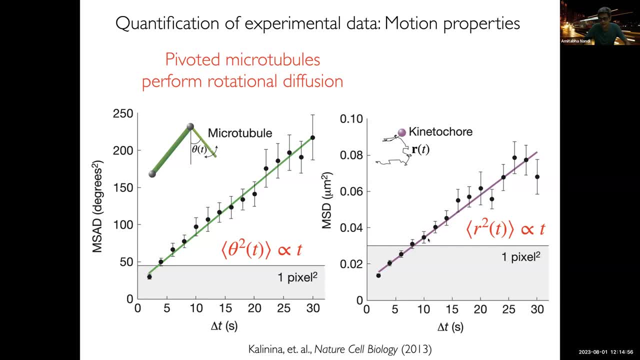 What is relevant statistics here? Relevant statistics is that suppose we look at So many cells and look at this capture process in many cells And we ask the question That what is the fraction of lost kinetochores And this fraction of lost kinetochores? 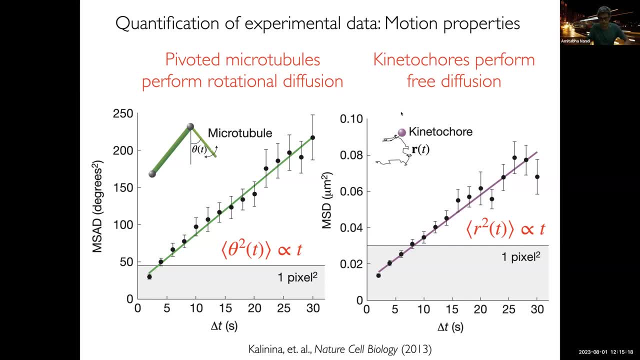 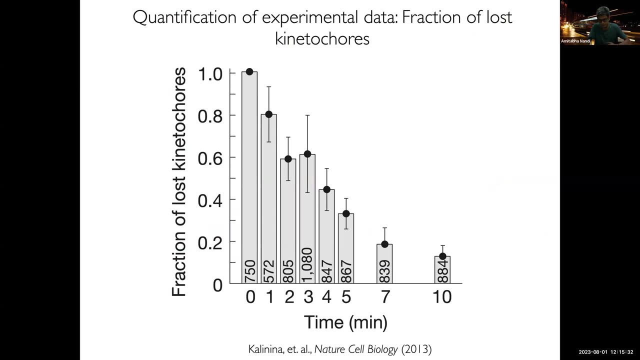 So these dots are the average values of the fraction over time. We see that this fraction is decreasing over time. Now I should clearly explain this quantity. So this is a very crucial quantity which you get from experiments, And let me explain it a little more carefully. 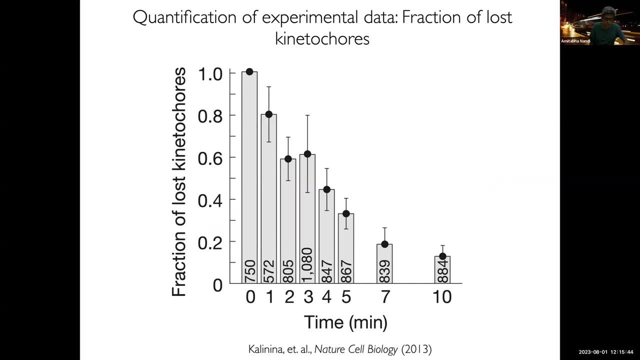 What is this quantity? fraction of the lost kinetochores. So suppose I have each of these spheres which is the nuclei of each cell. So in fission is the capture happens inside the nucleus, So Each of these sphere represents- it's the cartoon- for one cell nucleus. 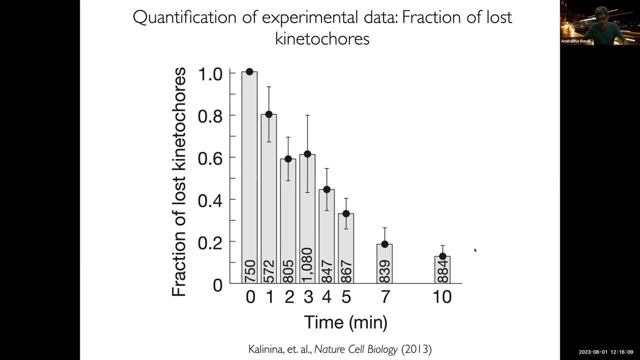 And each of these dot is a kinetochore which is diffusing freely, And each rod, this green rod, is a microtubule. There can be multiple microtubules, But I am showing just one microtubule, which 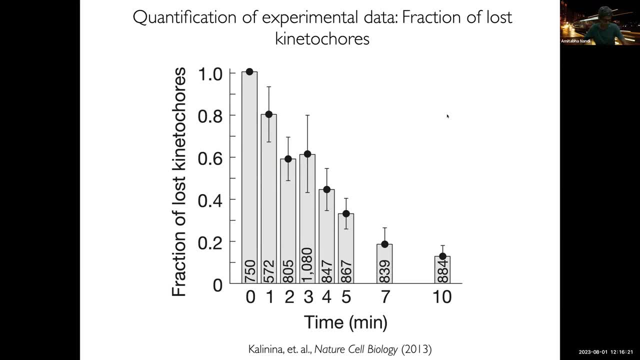 is performing a rotational diffusion, which we just saw from the analysis. Now suppose we are looking at an assay where I have, like n cells, I can look over time. I can look over time together, like in this case, 16.. 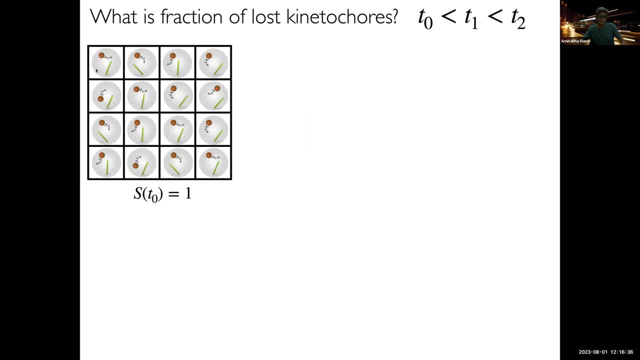 So at the beginning. so I have marked three different times: T0, T1, and T2.. T0 is the starting time where I start doing the experiment, T1 is the later time And T2 is, say, the final time. 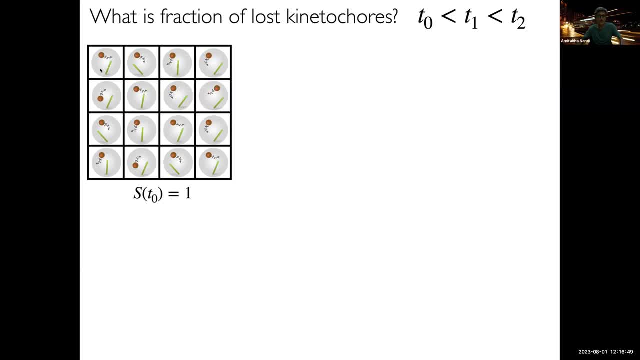 So at the earlier time when the experiment has started, none of the kinetochores are captured by any of these microtubules, because you have just started the experiment So you can say that how many kinetochores have survived? 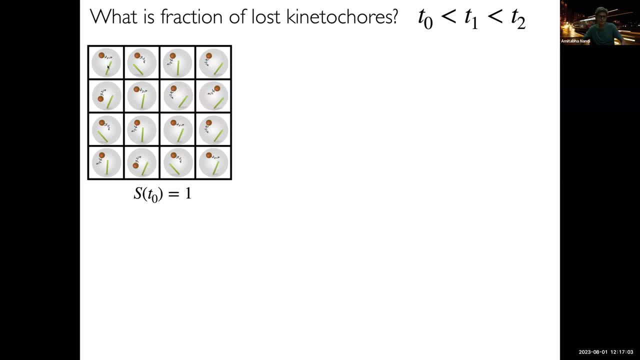 They have not got captured by the microtubule. And in that case it is one, because out of the 16 cells, all of them have survived. OK Say, in the next time, instant T1,. you see that out of the 16, some of them has got captured. 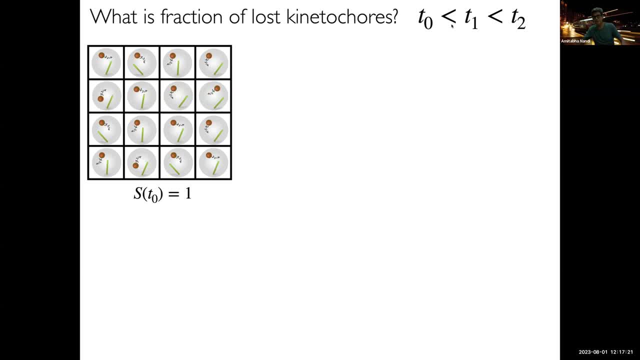 So you can see which are the ones which has got captured, So you can see the cursor right. I cannot see, I cannot. I mean it might be good if somebody like I mean you can ask me, Ask me questions in between, like if you have any doubts. 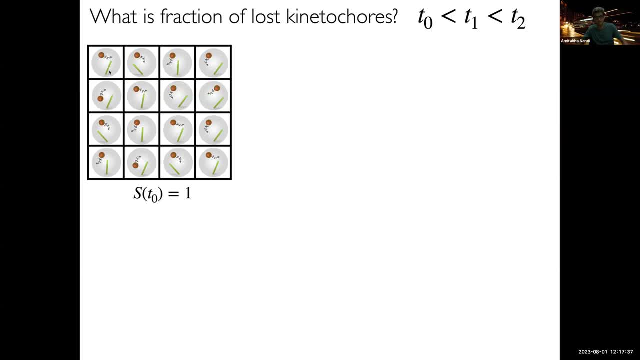 So yeah. so in the second one you can see that out of those 16, some of them have got captured: this one, this one, this one and this one. So out of 16, 4 has got captured, which means 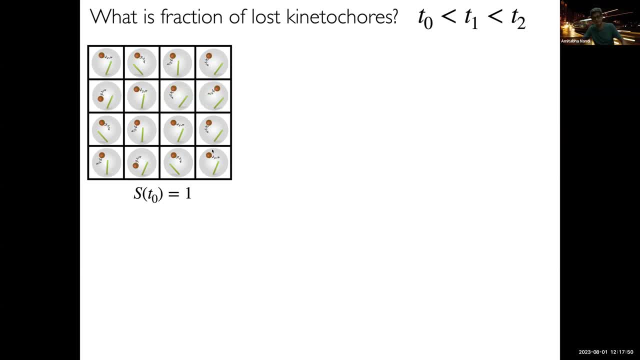 the remaining 12 has survived. So if I take the ratio, I can see that the fraction which has survived is 75% or 0.75.. Now, as time progresses, more of these kinetochores in the different cells will start getting captured. 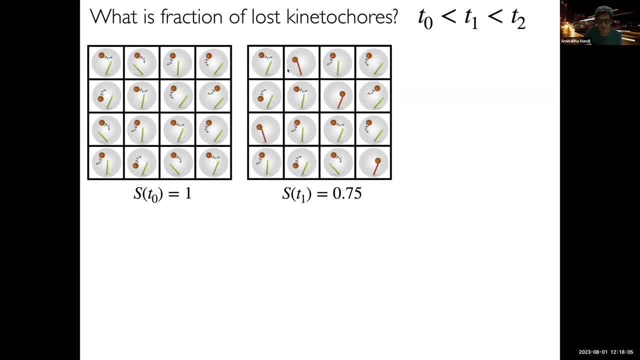 So if I go at a much later time T2, I see that like 12 of them has got captured. So now the fraction which is surviving is 25%. So this is what has been plotted in this experimental, from this experiment. 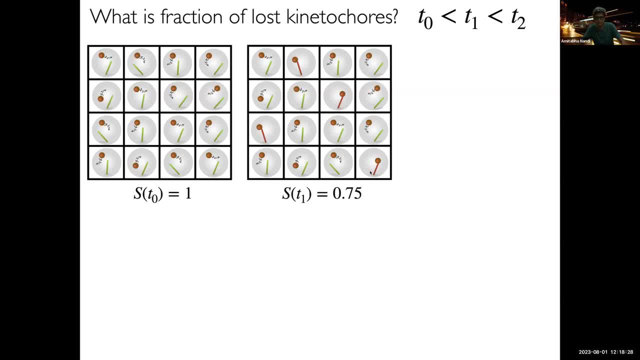 So this fraction of lost kinetochores is basically the fraction, The fraction of cells in which the capture has not happened, And in the stochastic processes literature this quantity is called the survival probability, And I will come to this in a few later slides. 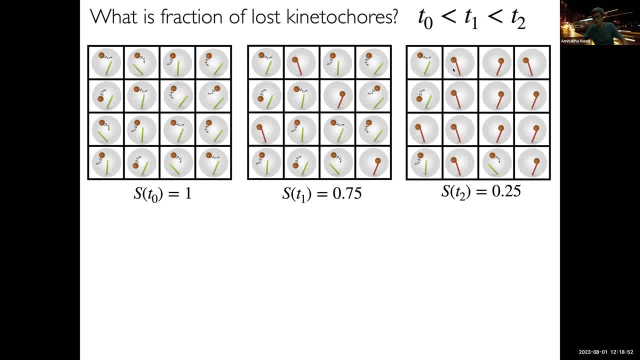 and explain this thing a little more in details. So now I have these nice statistics which tells you that If I look at an ensemble of these cells, this is typically the survival probability, Because each of them is a stochastic event. I can only talk about these capture processes. 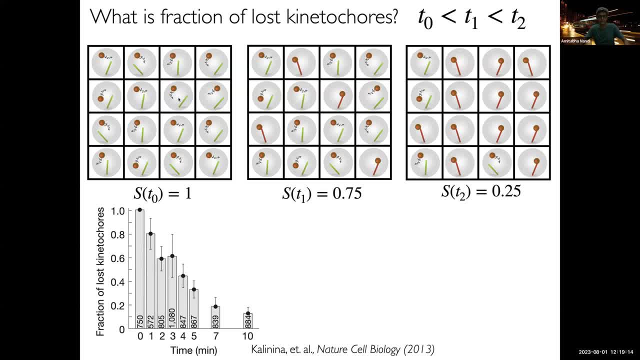 in a probabilistic sense. So that's why I need to plot this probability distribution. So now I have got three quantities: This survival probability, this information about the rotational diffusion of the microtubules and the free diffusion of the kinetochores. 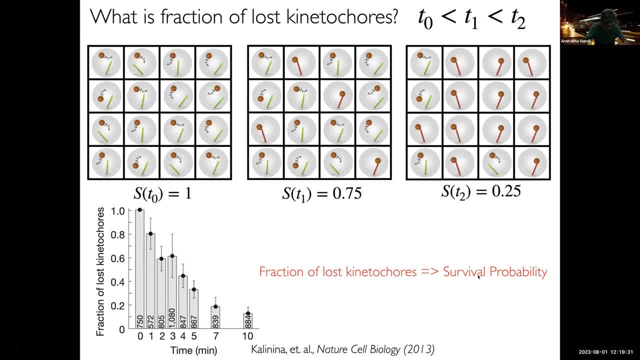 So now let us Try to build the model And let's see what we get. So again, what are the inputs from the experimental data analysis? So this is a fission cell. If I zoom in inside the nucleus I see the rod is doing a pivoted rotational diffusion. 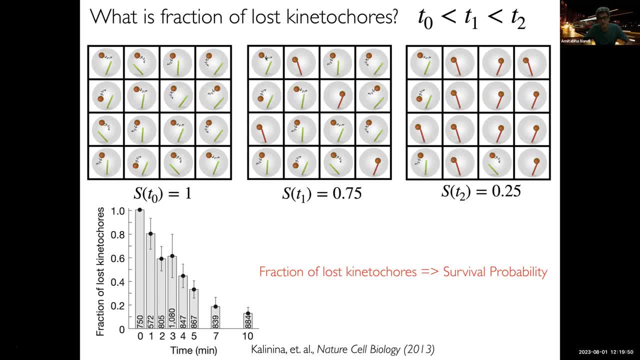 The kinetochore is diffusing And which means that I should somehow be able to write down the equation of motion of the rod And I should be able to write down the equation of motion for This free diffusion of this kinetochore. 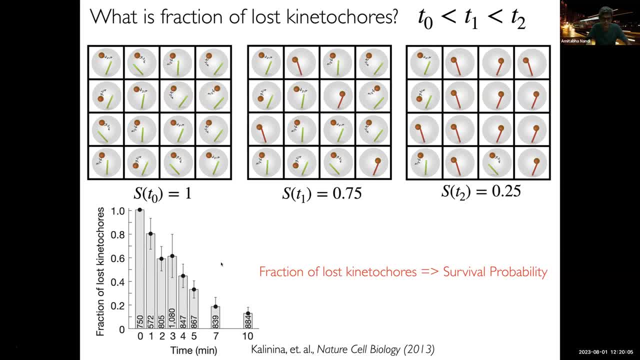 And all these things are happening inside the sphere of some fixed radius, which means I also need to put them inside the sphere, which means there should be a boundary condition. They cannot escape the sphere. And once I have this model based on this information, 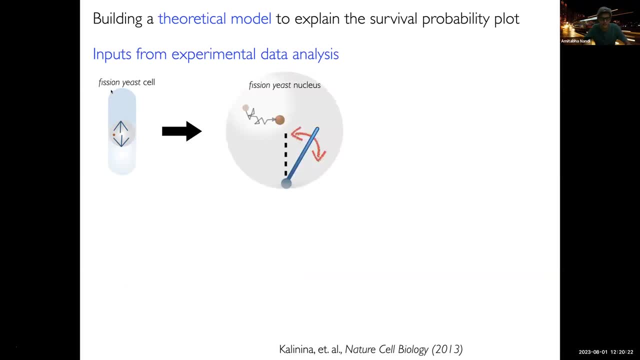 I should take this model, run this model for n different cells exactly in the experiment, And I should try to generate or recreate this survival probability which I have seen in the experiment. So let us do that. Basically, I should combine this information in the two red boxes. 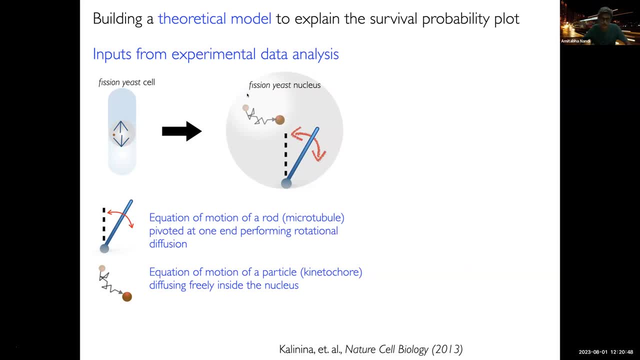 and try to explain this plot in the blue box. So are there any questions so far? If yes, I can take this question and then go ahead. OK, I think there is one question. You can unmute yourself and ask me the question. 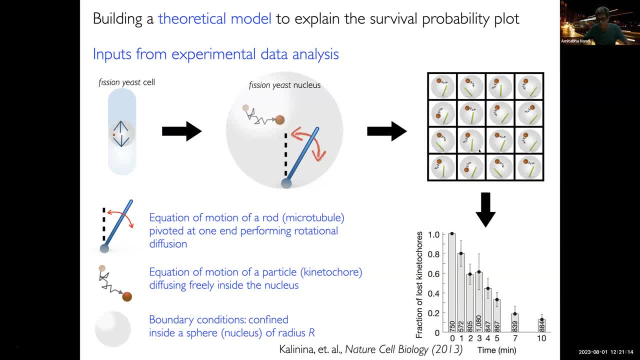 Kasturi. Yeah, So I was wondering, when we took away the viscosity from the equation and considered no contribution from there, is this still applicable, Or rather, what should we do? So let's assume that the cell is in the state where the viscosity of the cell may change, and that may be. 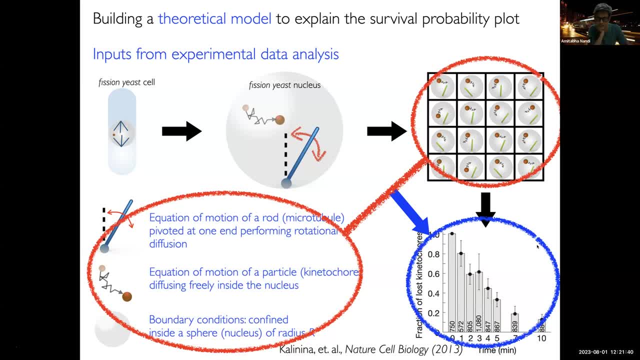 say a disease state or a developmental state, right? So we reconsider everything or add that factor back in, or we have to measure, I guess, the viscosity in those different situations. And that is a probable scenario, I think, in some of the cellular states. 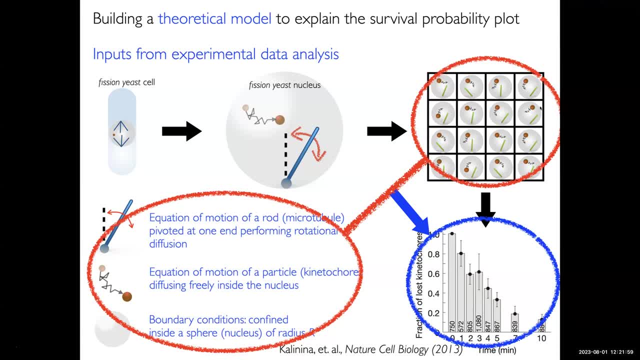 But I don't know ballpark, you don't care. so what's the approach here? okay, let me try to understand the question. so so, first of all, here, what we are doing is we are going towards the limit where the fluid is more viscous. we are not taking away the viscosity. so basically we are saying that. i mean, if i try, 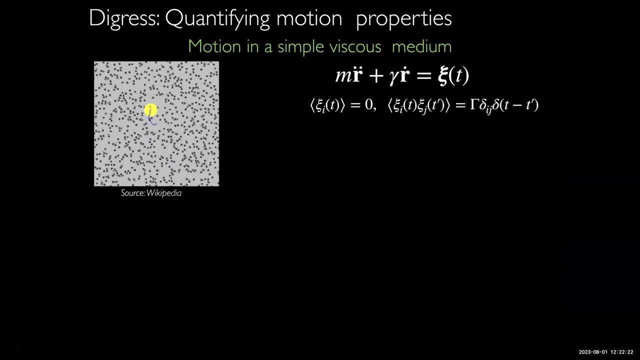 to give an example. so say, initially it was in a fluid which is like water. now it is in a fluid which is like, say, glycerol, which is more viscous. and when we put this bead in a more viscous fluid which is typically like the kind of environment inside cell, this particle cannot accelerate. so 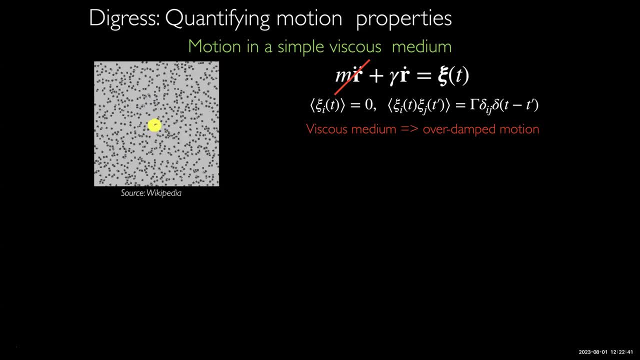 you can drop this term now. whatever is the viscosity, based on that viscosity one can estimate the diffusion coefficient. for example, if we know like there will be a wide range of protein molecules inside cell, and given you know like the, the protein size, distribution and other parameters, and if we know the viscosity, one can calculate. 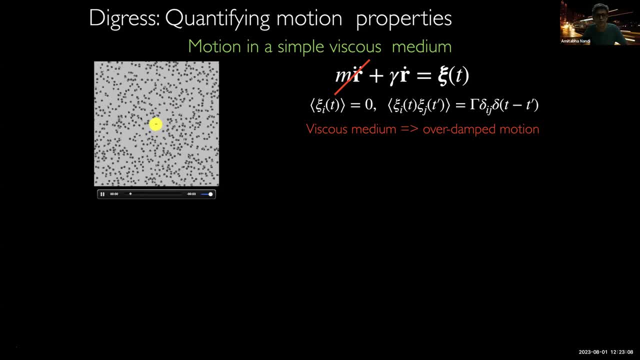 for those proteins, the diffusion coefficient for a given scenario. now if, for example, the viscosity in a given situation, say in a disease state, suddenly increases compared to the normal viscous conditions, then one has to somehow use that as an input in the models, because the when you see, like from this equation, when we write down the simplified equation, 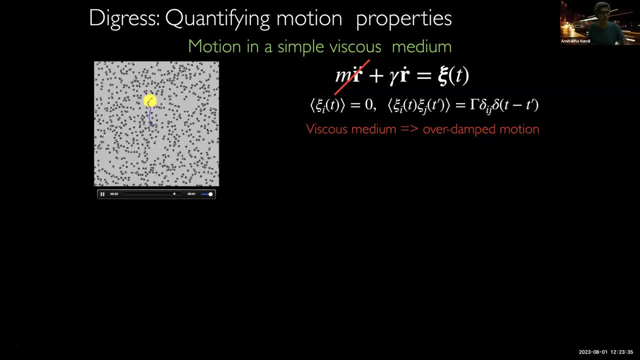 for a viscous medium, i have this quantity d. now, d is a function of the viscosity of the medium. so, as for your questions, the viscosity increases, that should be reflected in the value of d. okay, now if the viscosity is a time dependent quantity, that is like a more complicated scenario. 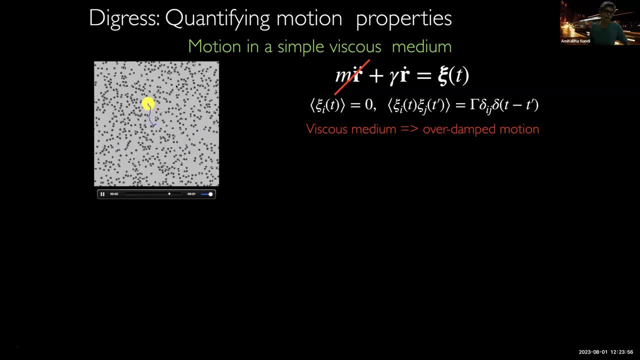 so then that has to be also captured. uh, by a change in d i would say right, so using that it can be also predicted. i guess, if viscosity changes, if d changes right, what would be the scenario correct? and then that could be tested in a, in a, say, disease state or in a situation where viscosity apparently changes. 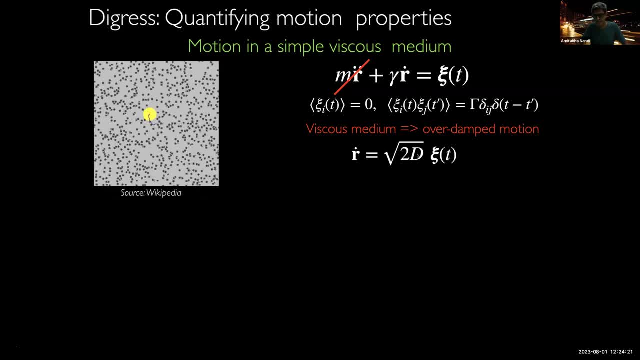 yeah, for example, i mean one thing you can see clearly. for example, if you calculate this quantity, so suppose the d has changed. okay, so suppose you you do this experiment, you record the, uh, the. you measure the position of a particle over time at two different times, at an early time, when, say, the viscosity was something. 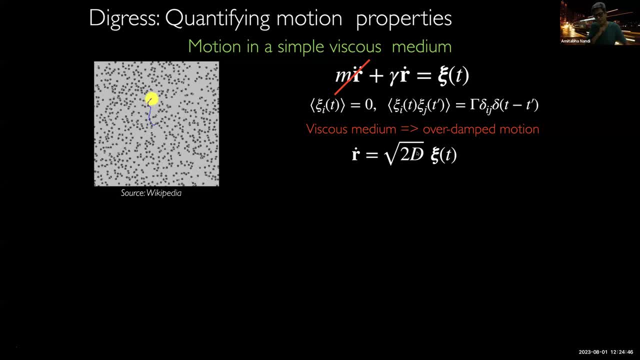 and at a much later time, when the viscosity has changed. okay, now, assuming that there are no crowding, which i was talking about, like there can be more complications, like assuming that this is really like a simple scenario, where it is like a simple viscous fluid, you, 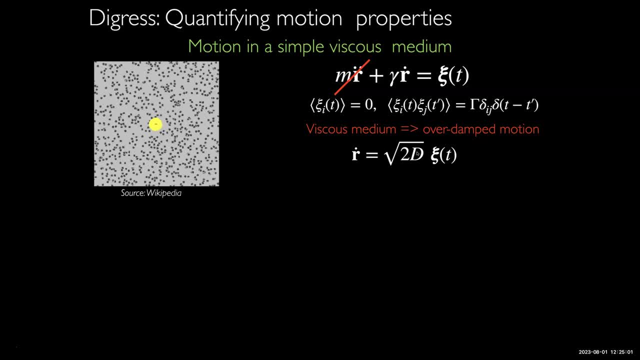 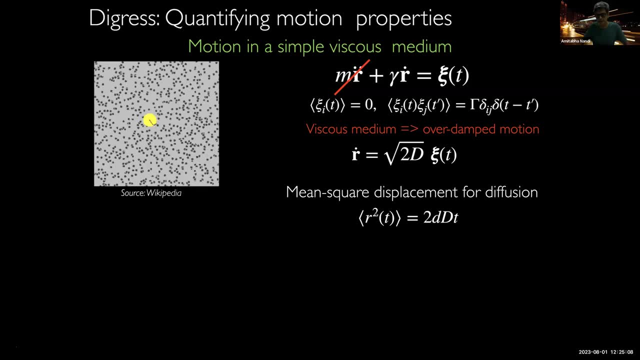 can see from this formula. so i didn't explain the formula. so this small d is the dimensionality of your problem. so if you are making this measurement in 2d, this d will be 2.. if you can record the trajectory position in 3d, in three dimensions, this d will be 3.. so for 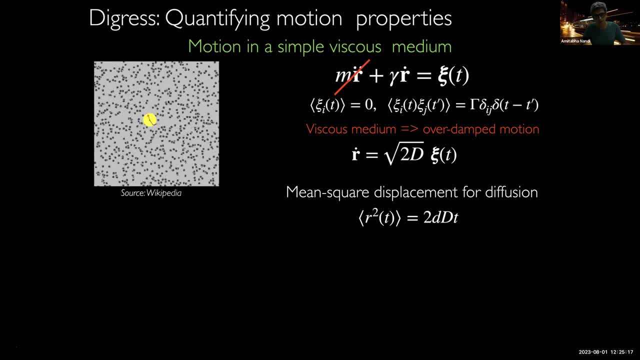 the moment. let's assume that you are making this recording in two dimensions, you put it under microscope. now, if your viscosity has changed- and it is still changing- then you can see that if it is still a simple fluid, then this slope, this d value, will change, and that you can find out by fitting the experimental mean square displacement by this formula. 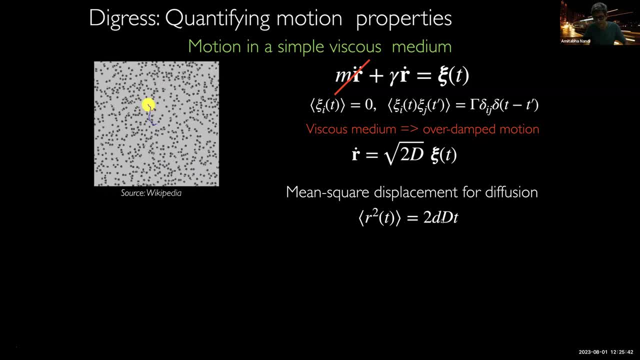 thank you, okay, uh, there is another question, i guess. yeah, hi, devinder, please, hello, hello, sir, so, um, so i would like to know that when, uh, from the fixed point, there are number of models that can be used to calculate the velocity of the velocity of the velocity of 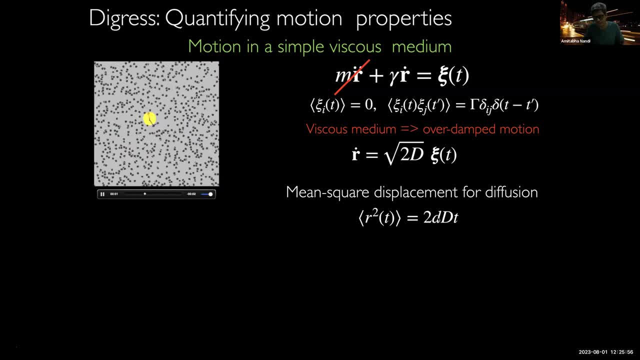 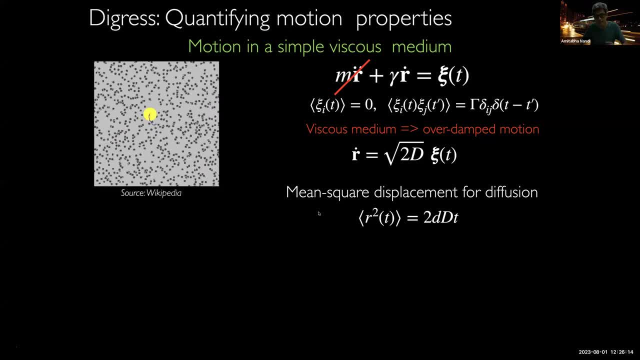 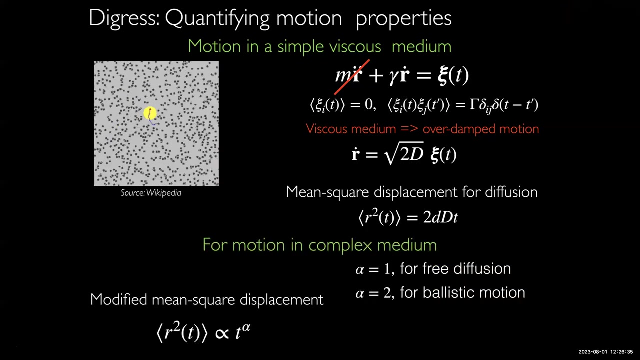 so, for example, these micro tables cannot come very close to each other, so there will be some kind of excluded volume interaction. that is one thing. uh, now, Now, in this scenario, there is no preference for, within this framework, what we see experimentally and what we try to model. we don't have any preference of any particular microtubule trying 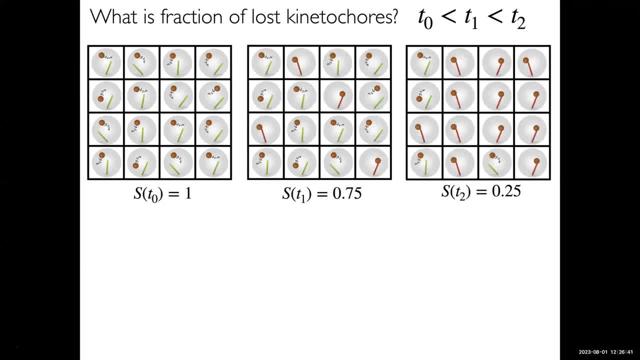 to find, like looking for a particular chromosome, kinetochore or so. So basically what we are saying is like if you have, like N microtubules, the kinetochore movement is completely independent of the microtubules, it is independently diffusing. 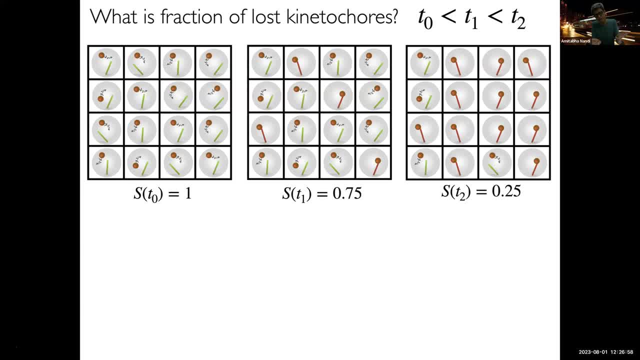 and any one of those microtubules. when they come in close proximity, there will be a capture. But there are other organisms where they use more complicated forms of this search strategy. So, for example, I forgot the organism. is it in Xenopus egg? 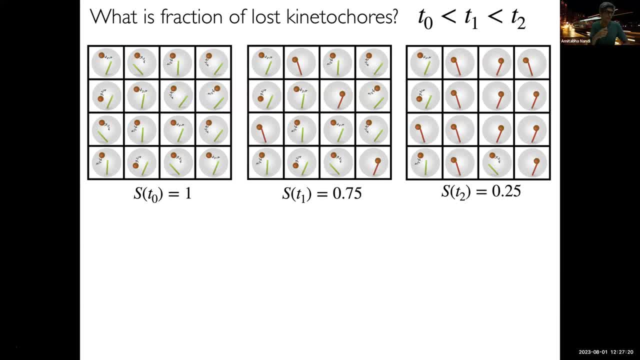 So what happens there? So there is a chemical gradient around the kinetochore, So this is a gradient of something called RAND-GDP and this chemical. actually, whenever the microtubule senses that chemical, its growth state is stabilized. So it is in a preferentially more growth state than shrinkage state, which means that there 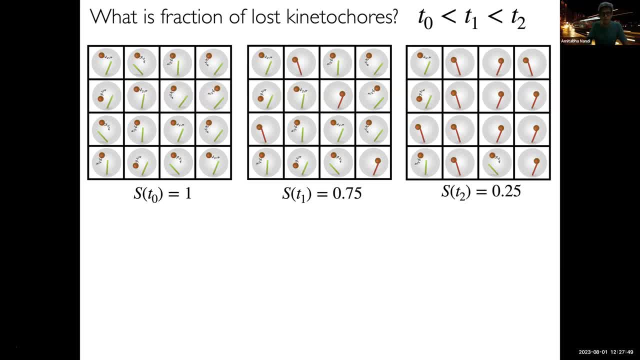 is a chemical gradient around the kinetochore. When the microtubules come in close proximity, the growth is stabilized. When the microtubule starts sensing the gradient, it will bias its growth more towards that kinetochore. 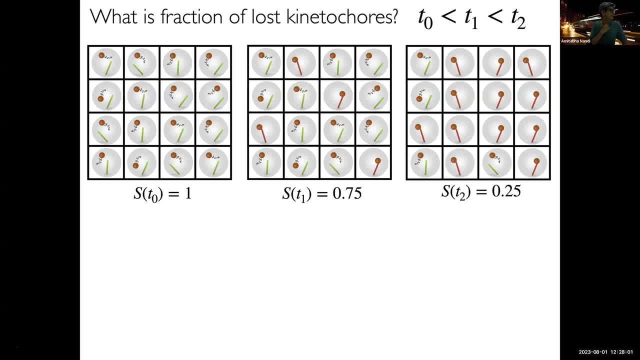 And then this actually enhances the speed of capture. But in this case we don't have- at least in fissionists we don't have- any evidence of such kind of a biased capture process. Okay, And also these microtubules. each microtubule is going to have one or two microtubules. 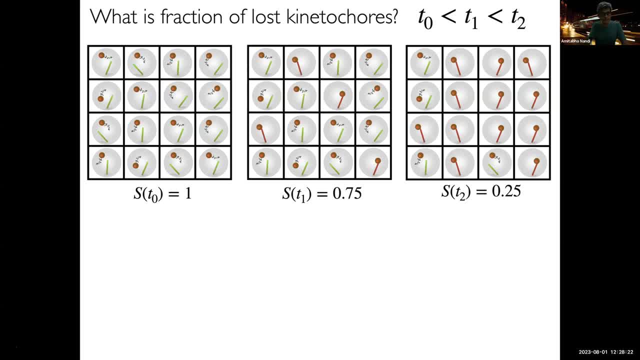 Okay, So they capture one chromosome. Once they capture the kinetochore, then it's not like that: chromosome one, chromosome two, three- so many chromosomes are there on the single microtubule. So how that one microtubule per chromosome? what actually is indication for that? 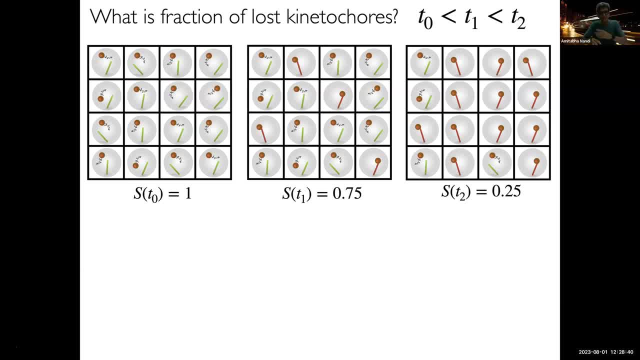 How microtubules get to know that. okay, now the work is done and there is no more search and capture thing. Yeah, this is a very good question. I don't have a very clear answer to like the question. I don't have a very clear answer to like the question. 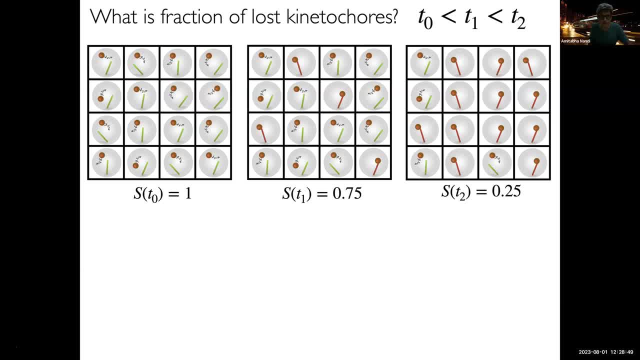 I don't have a very clear answer to like the question. Okay, So I don't have a very clear answer to like because there are multiple chromosomes and all these captures are happening simultaneously, right? So like, once one chromosome is captured, like how the next stage of processes start and 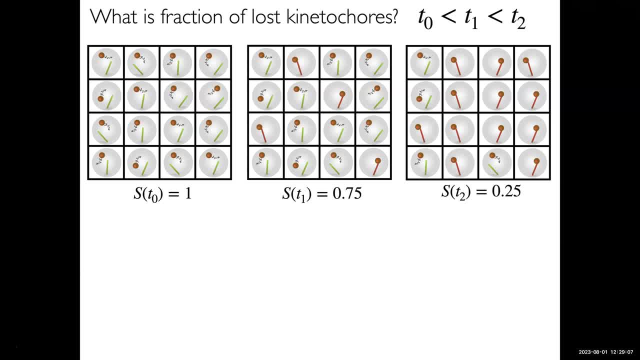 like how, whether, like whether one should actually in the model simulate all the chromosomes and the microtubules together, Or like numbers, Okay, Okay, Okay, Okay. So one is that there are a number of like if there are N microtubules and M chromosomes. 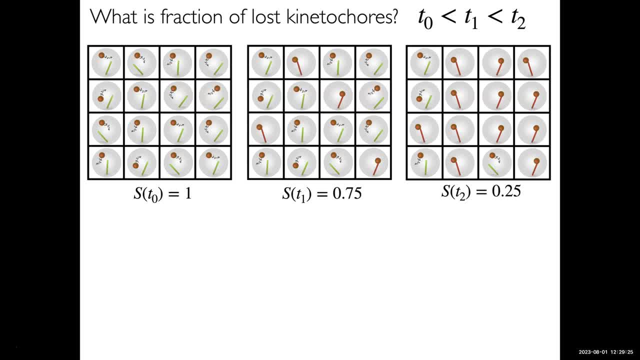 whether we should do like some, like a lesser number of microtubules per chromosome. So this is an interesting question And so the detailed mechanism of, once the capture has happened, what happens, how they are positioned and how they are brought in the spindle. 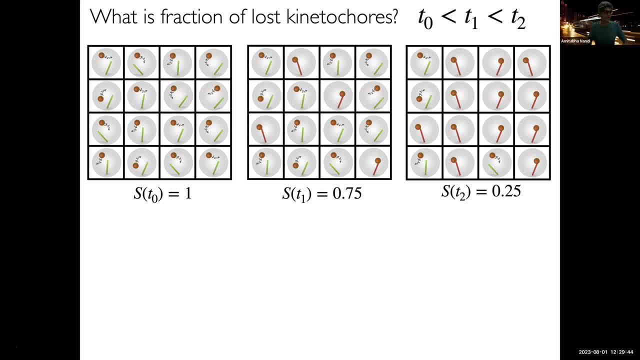 I don't know much of this. So what we are trying to do here at this level of the model, So I know, in fissionists I think there is of the order of three chromosomes in total And like there are typically three to five microtubules per chromosome, you can think of 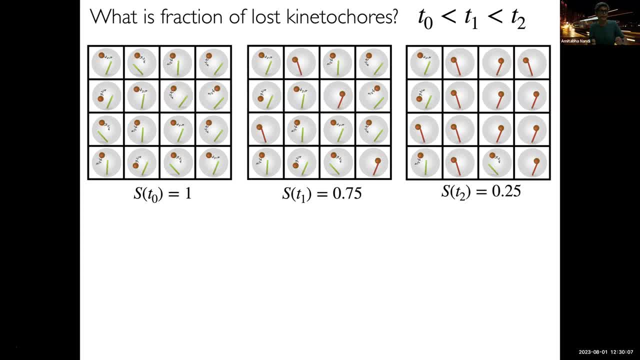 And that is what in this simple model scenario we are trying to model. We are saying that: OK, so I will just worry about, like how, if there are three or five microtubules, how they are competing against each other to capture a single chromosome. 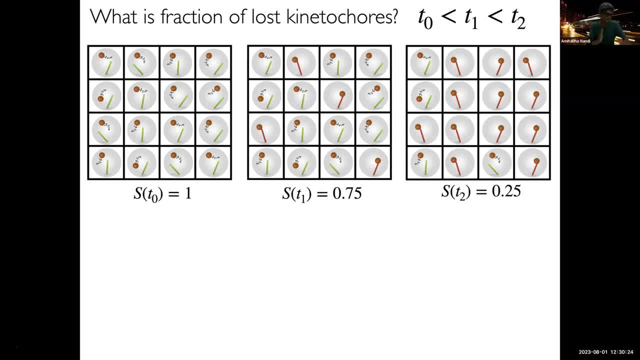 So does that address your question? Yes, So the actual process is, yes, more complicated. That is true, Thank you, OK. OK, OK, good, So I can go ahead. Yeah, So now I will try to build up the model and let us try to do that. 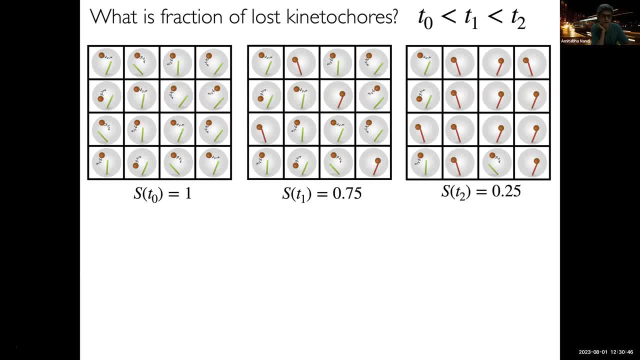 So the first thing, the model for the microtubule. it has this following equation: So I won't have much time to actually go to the details of this equation, But what I can do is I can explain So again. So what you have is: so we are modeling this rod. 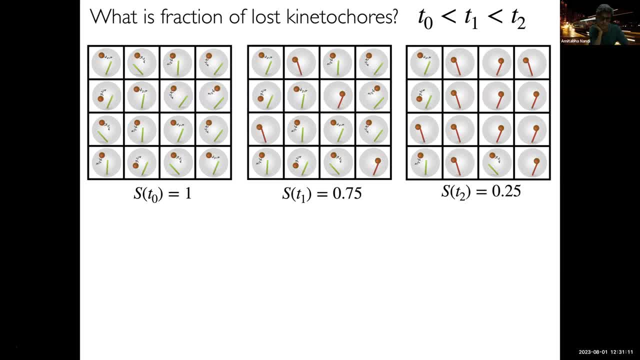 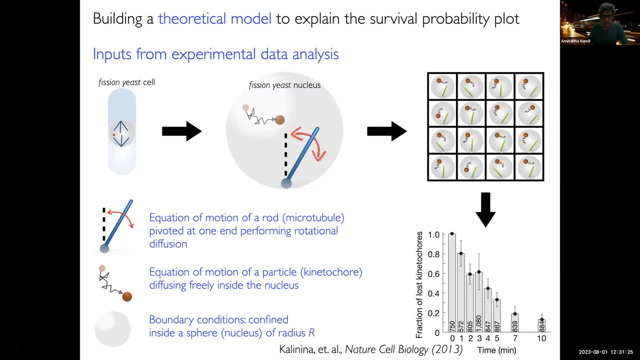 pivoted here, of constant length, doing this rotational diffusion motion. And we consider at the level of this model, we consider this rod in 3D, which means you can think that you have a rod hinged at one end And the tip of the rod is tracing, moving on the surface of a sphere. 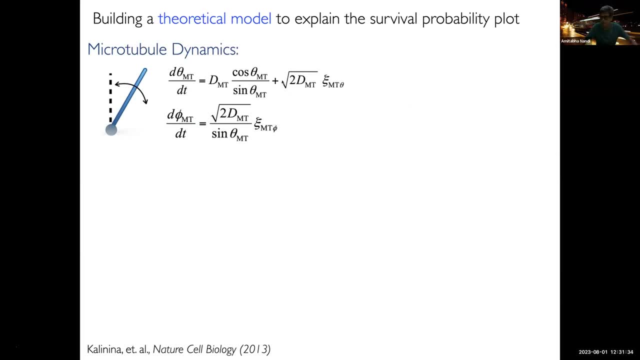 So, since it is in 3D, if you go from Cartesian coordinates to spherical polar coordinates, you can see that the radius of the rod is fixed. So you can see that the radius of the rod is fixed. So you can see that the radius of the rod is fixed. 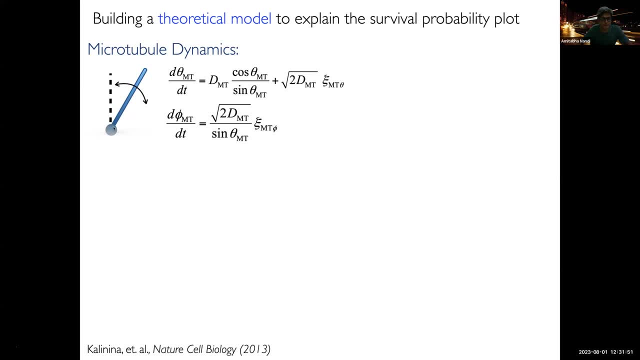 But because the radius is fixed, because the length of the rod is fixed, you need two variables to completely characterize the motion of the rod. One is this angle, theta, Another is this angle, phi. So this is like the polar angle, which is the angle traced out on a plane. 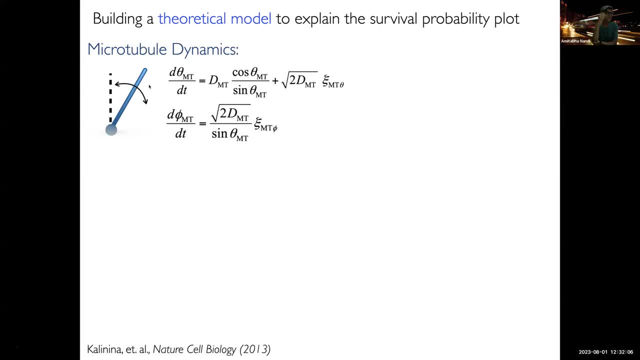 And this theta is the azimuthal angle And what we have written down here is the equation of motion of these two angles and the phi angle. And you can see that because it is a rotational diffusion motion, as we saw in case of simple diffusion in free space, there was a noise term. 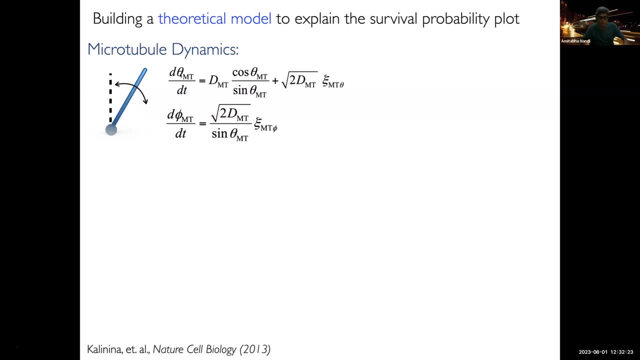 There was a random kick Here also. there is a random kick with a prefactor which has this diffusion coefficient of the microtubule And unfortunately, there is some more complicated term in the front, which is this nonlinear term, which is the cosine of this angle. 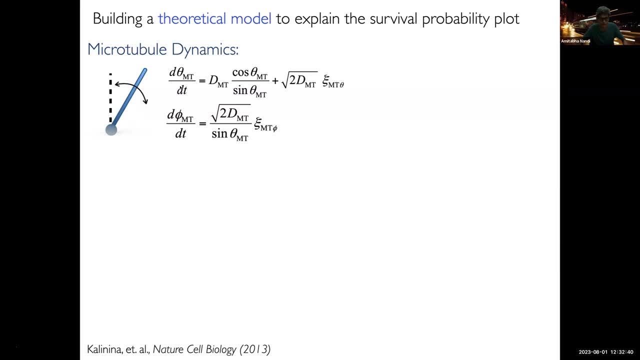 divided by the sine of this angle And the second equation. And the second equation. It also has a noise term, but a nonlinear term which is like the inverse of sine of this. Now, one can systematically derive this set of equations by considering a point diffusing on the surface of a sphere. 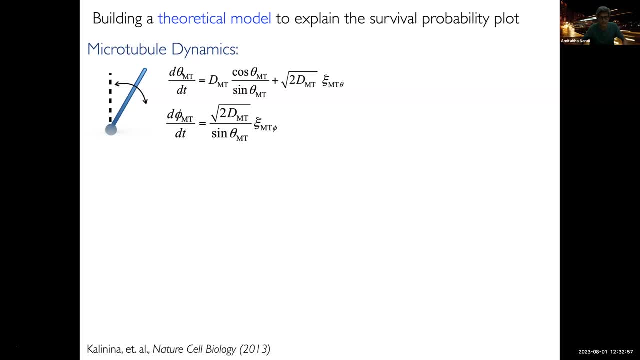 in Cartesian coordinates and doing a coordinate transformation from Cartesian coordinates to spherical polar coordinates, And one would get this equation which we did while we derived this equation. This is a consistent equation, So there are more details in this model, For example, this diffusion coefficient of the microtubule. 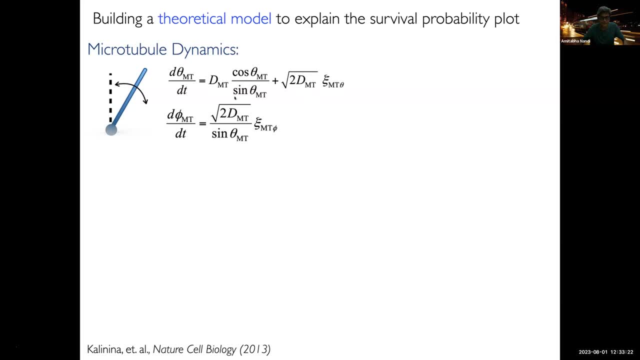 So this we estimate from the experimental fields which I have shown a few slides back. However, this one can show that for a rod pivoted at one end, this diffusion coefficient has a dependence on the length of the microtubule. It has a very sensitive dependence on the length of the microtubule. 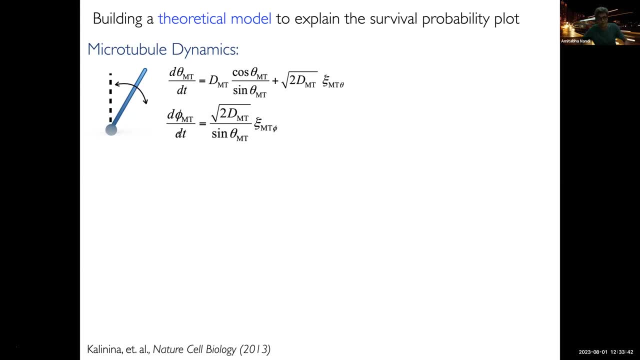 It has a very sensitive dependence on the length of the microtubule. It goes as one over L cube, cube of the length. So you can see that if this length starts growing, this rotational diffusion will become much slower. So this is the details of this equation, for the rod pivoted at this end. 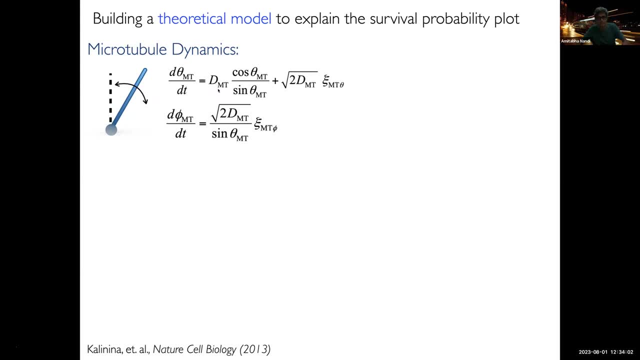 The equation of motion for the kinetochore is rather easy. It is basically exactly the way we wrote down the equation for a diffusive particle in a viscous medium, where it is like a highly viscous fluid and it is moving freely within that fluid. 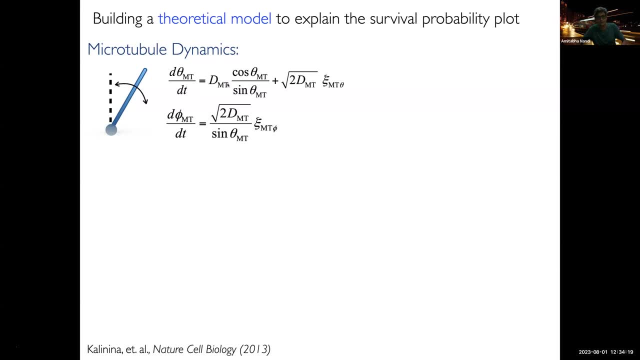 And this is the equation of motion. So at every instant it is getting some random kicks, which is given by this xi of t on the right hand side. Now, of course, we have to put the boundary condition and we know from experiment what is the typical size of a nucleus. 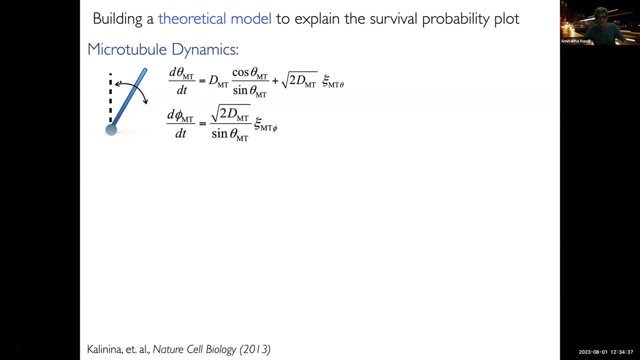 It is three microns, which means that if we put this boundary, this rod cannot go out all the way. So when it reaches this extent, it will feel a physical barrier and its motion is bounded by the actual bound of the nucleus. And all this, like this kinetochore, is also diffusing within this. 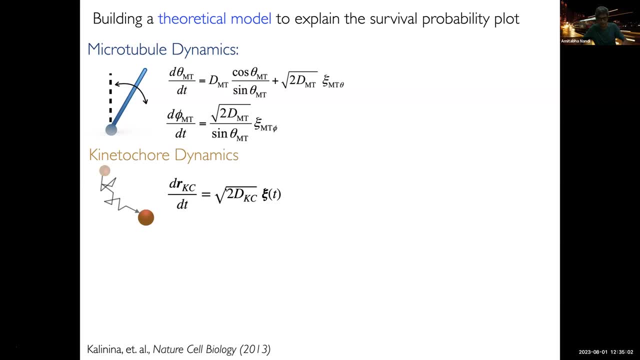 so it cannot leave this whole sphere, And what we can do is we can take these two equations, put this boundary condition and perform a simulation of this set of equations And of course, now we can simulate for n such nucleus and keep on tracking, like over time. 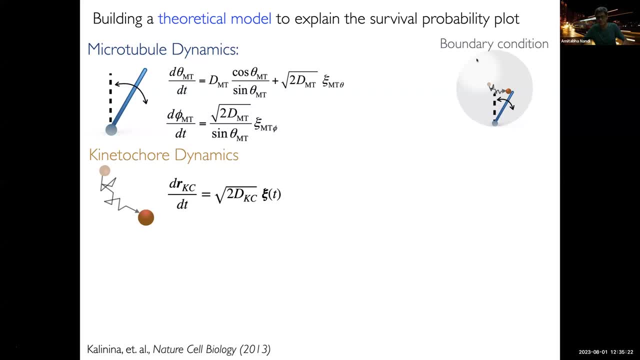 when there is a capture of a chromosome by this microdivision. And if we do that, we can now exactly calculate the fraction of lost kinetochores from our model. And I wanted to tell you one thing. So, in this model, what are the parameters? 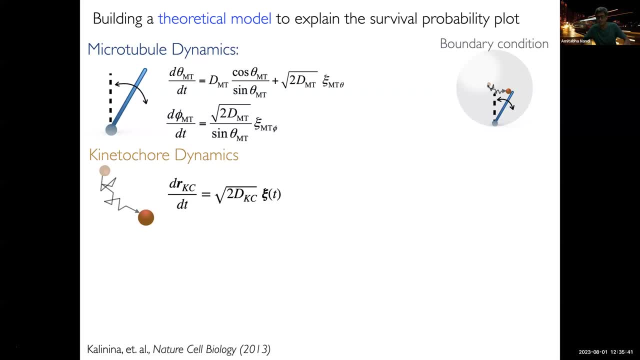 The parameters are this: d, which we measure from experiment. the diffusion coefficient of the kinetochore, which is also measured from the experiment, from the fits of the mean square displacement. the size of this sphere, which is known. the average length of the microtubule. 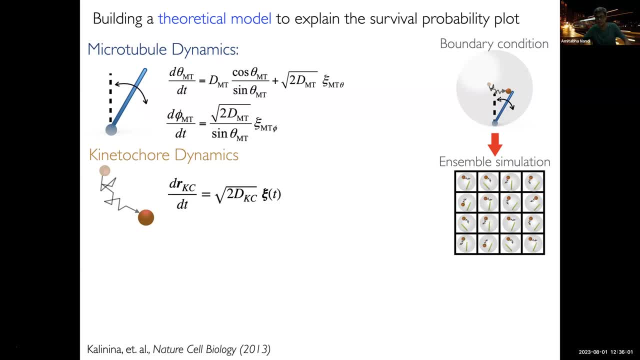 which is also known from experiment. So while running the simulation, there is no fit parameter except for the number of microtubules which we are varying, Because if we just have one microtubule we get this curve which we see does not agree very well. 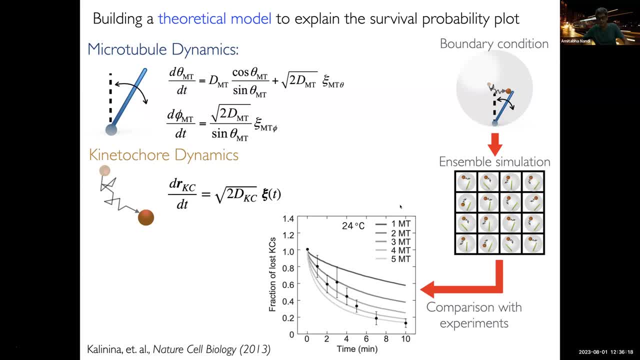 with the experimental data. But as we keep on increasing the number of microtubules, we see that when we have of the order of three to five microtubules, we get a very good agreement, And this is also consistent with the observation. 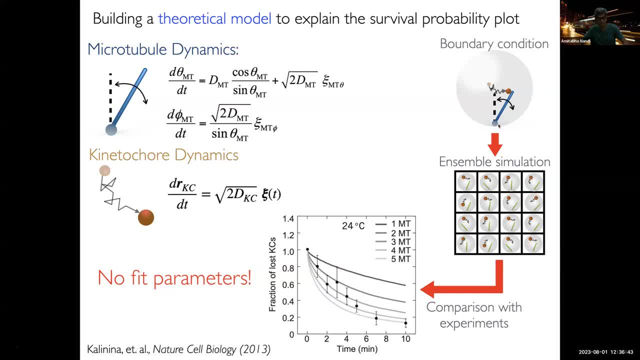 in experiment which is known that for fission is the number of microtubules which are growing from a spindle body is roughly of this number. There are not many microtubules, unlike in eukaryotic other eukaryotic cells where you have like. 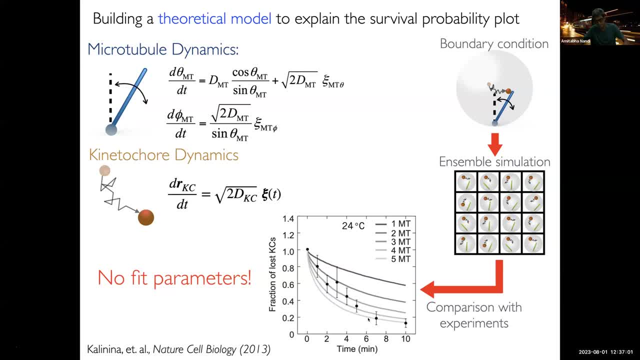 of the order of hundreds of microtubules. So this: first of all, we have a very good agreement of between the model and the experiment And it gives roughly a good ballpark number of the number of microtubules which we get out of the simulation. 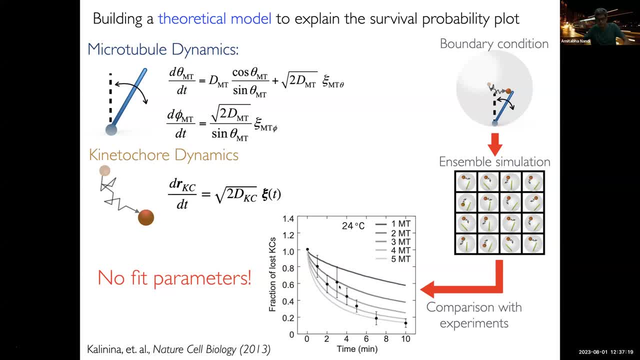 So this is what we have reached so far that we started with some experiment. We analyze the data. based on the analysis, We use them as input to construct data. We use them as input to construct this model and try to make a comparison with the statistics from the experiment. 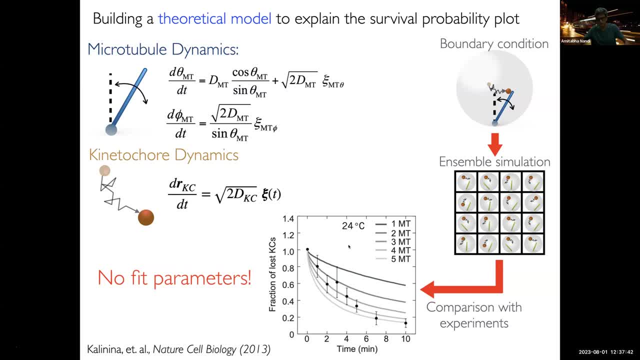 And we got some. we got some agreement. Now the thing is we have to. we should not stop here. ideally We should now, because we have a model where we have a very nice set of equations which you can see, So we can actually play around. 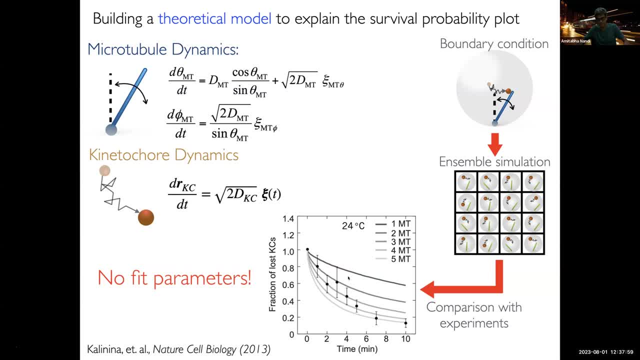 with these different quantities and ask various questions. Okay, So this, that will be the next part, that can we like do something more than just proposing a model for this very specific set of experiments which is in fissionist, Okay, I mean. 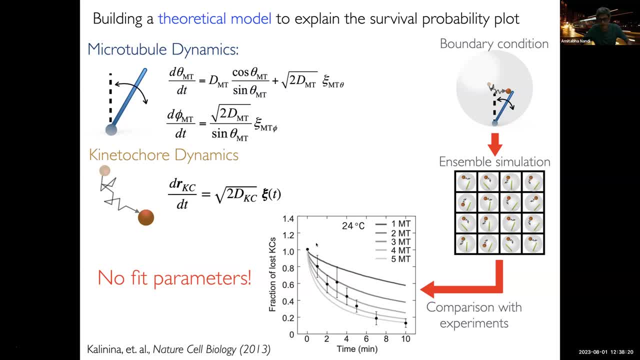 can we, can we go beyond fissionist, Or can we say something more about fissionists Or, in general, more about this kind of capture processes in general? So let us try to do that. So the question is, what else can we learn from the model? 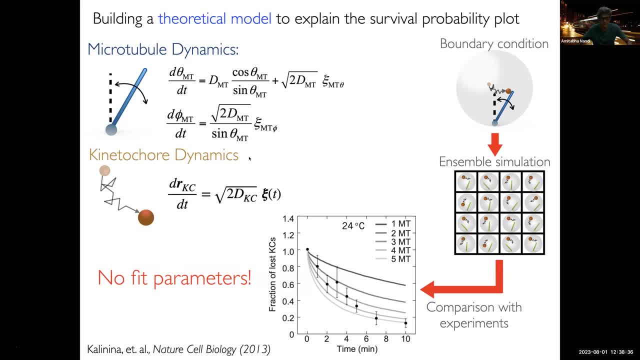 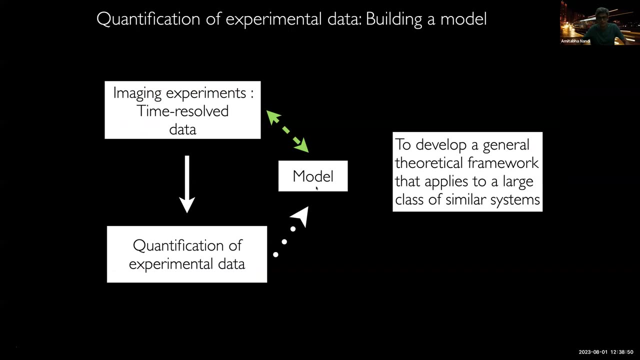 And another interesting thing is this model can be mapped to a very important problem which, in stochastic process, which physicists have been interested for a while, And it is an extension of those class of models And that I will try to explain here. 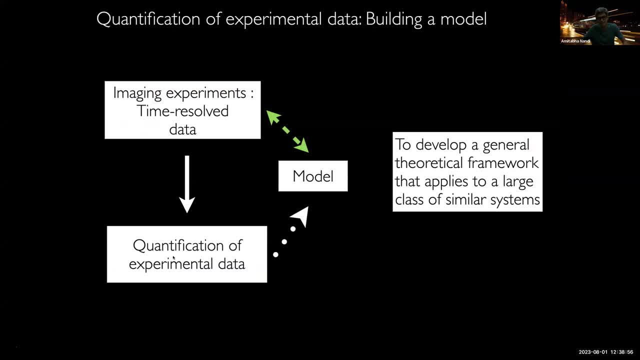 I will like try to give a general framework of the theory on which this like, like which this model, is a part of. So I need to digress a little bit and introduce something called a first passage process. And what is the first passage process? 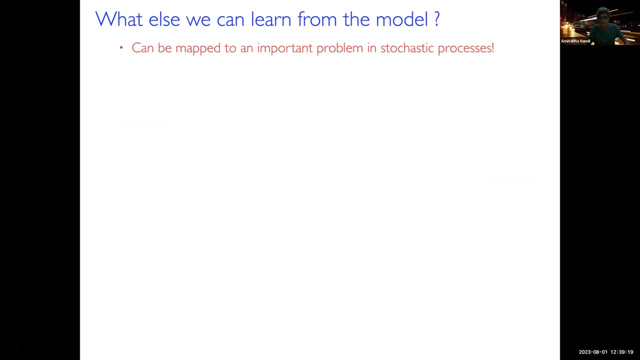 So the idea is the following: So suppose you are recording some random variable, some X, as a function of time, And you ask that when this variable reaches a threshold value for the first time- And why first time? Because this variable is a random variable. 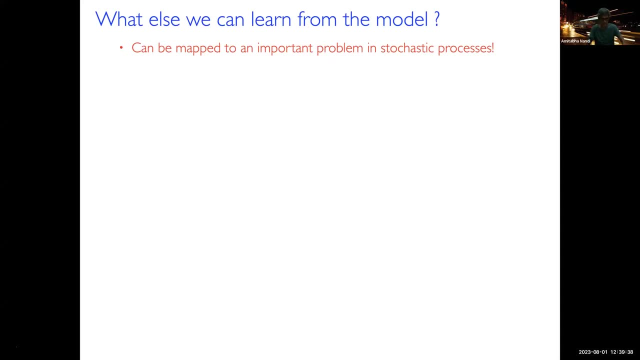 So every time you start experiment where you start tracking this variable, the time taken by this variable to reach that threshold will be different. Okay, So basically what you can do is: and this variable can be anything. In our case it was basically: 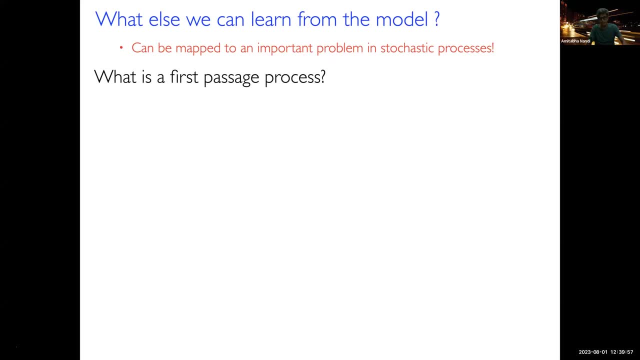 say the position of a particle. So it's a particle that is reaching some target. It could be some chemical like concentration, like a protein number trying to reach the threshold, such that once that threshold value of the protein is reached, some other chemical processes start. 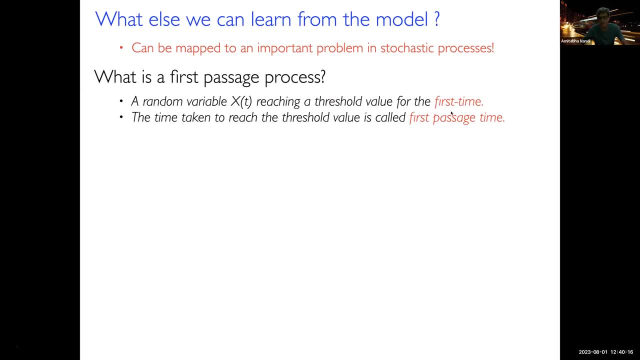 So it is very important that it reaches a threshold And you see that every time you do the experiment what time it is taken to reach that threshold. It can be some stock market index also, which is a stochastic variable, So it has to be. 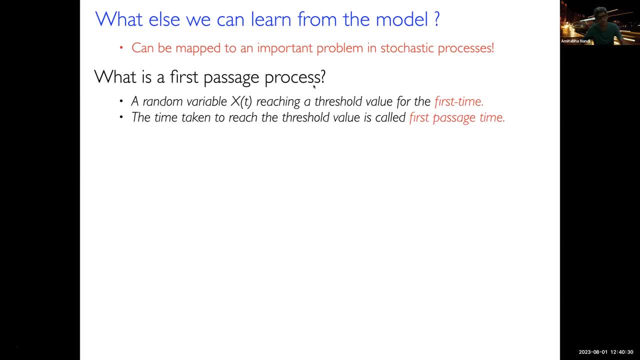 it has to be a stochastic variable. It can. it's time. evolution cannot be determined in states, So now you have this variable. So what a simple example is. you have a random walker, and the random walker cannot control its trajectory. It does a completely zigzag motion. 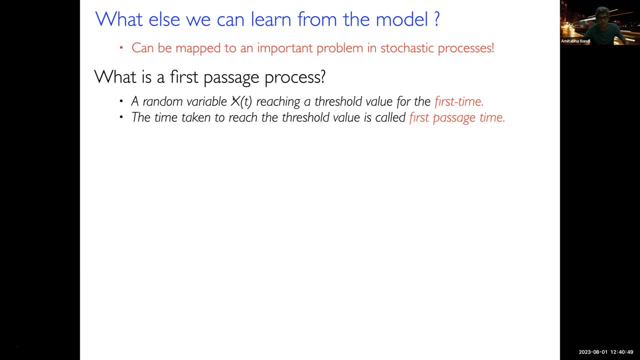 like the particle in a viscous medium And you ask the question that when does it hit the lamppost for the first time? So if you do this experiment with this random walker n times, every time you will record a different time And with this set of times, 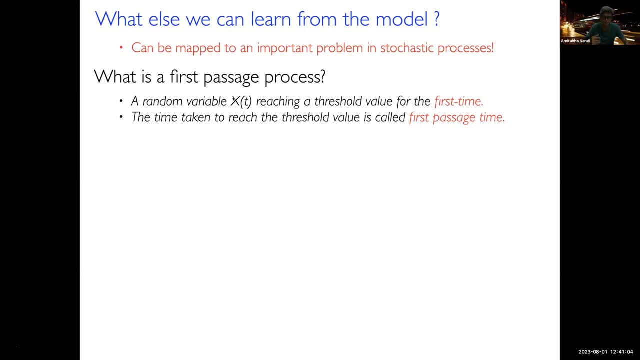 what you can do is you can plot the distribution or the histogram of this time, And that distribution is called the first passage probability density. And this first passage probability density is related to something which I introduced in the previous slides called the survival probability, in a way that the first passage probability distribution 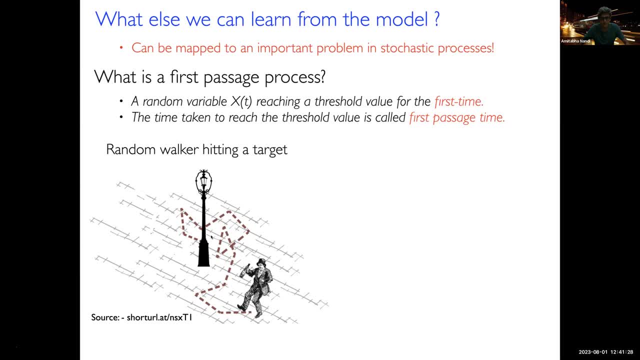 is nothing but the derivative of the survival probability with a negative sign. The negative sign because as time progresses, the survival probability decreases, The chances of surviving becomes lesser and lesser. So if you ask this question, that in between a time instant, t and t plus delta t, 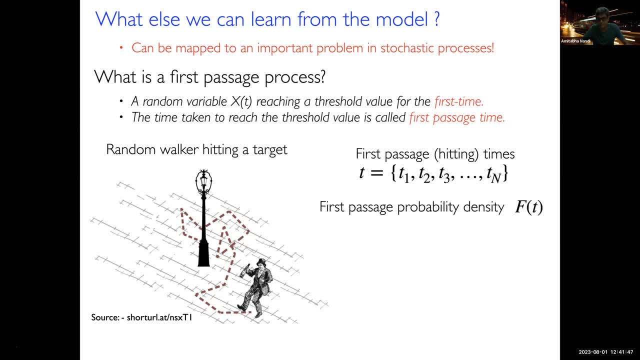 what is the probability that it will get captured? It is ft, dt, And that is the difference of s at t plus delta, t minus s at t, And if you do first order Taylor expansion, you'll get this formula. So it is a very simple relationship. 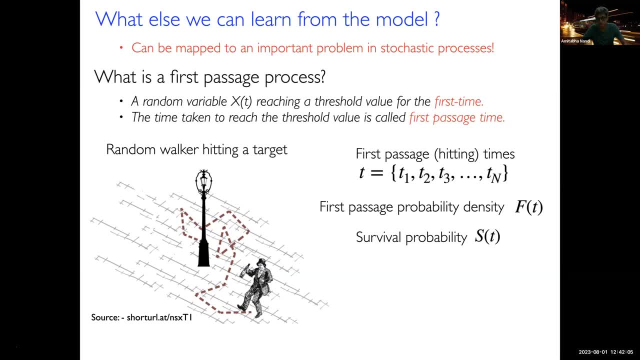 between this first passage distribution and the survival probability. Now this class of problems has a wide applicability in natural sciences in various fields, And again I am digressing a little bit So you can think of again revisiting this Brownian motion problem that now I 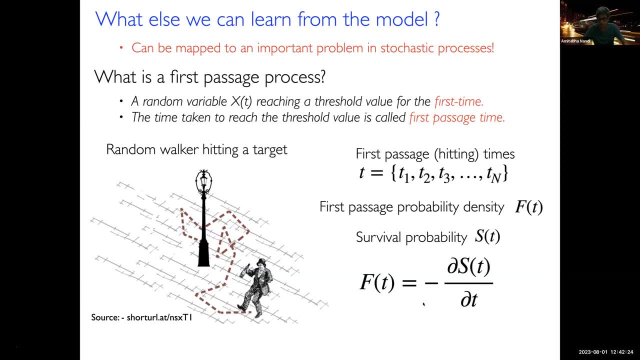 put a flag which is a target. It is a fixed target And you ask the question That every time this particle starts, what is the time taken to reach the target? Now, although this movie is looping, so every time, I had started with doing this experiment. 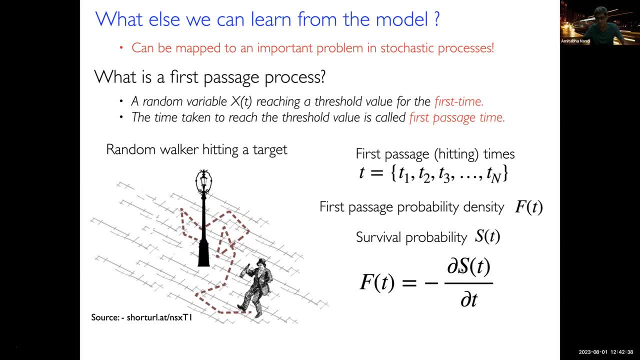 the times taken will be different. So what I can do is I can record the time and calculate the first passage distribution. In this case, I know the equation of motion of this particle And if I know the diffusion coefficient I can run a simulation. 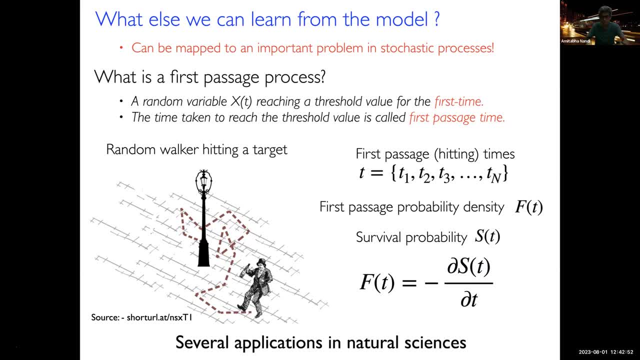 And I can again get the distribution. There are other techniques also which I'm not going to go into the details, that you can write down the time evolution equation for the position of this particle. You ask the question: what is the position? 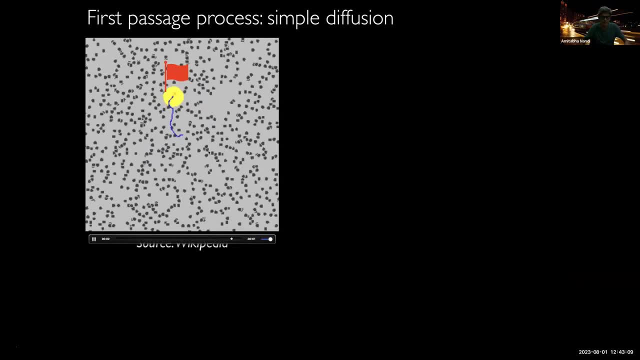 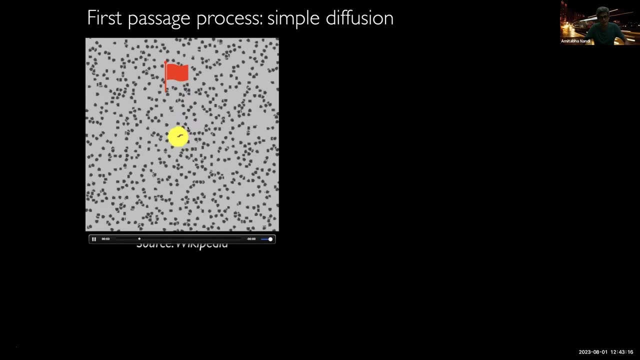 of the particle at some time t, given that it started from some initial condition, initial position x0 at time 0. And from this equation you can write down this equation, which is the diffusion equation, And you can calculate the survival probability. 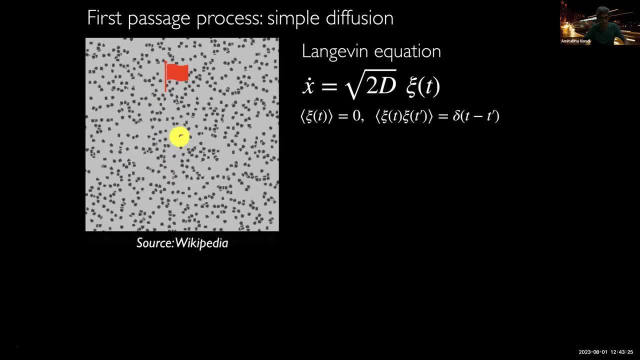 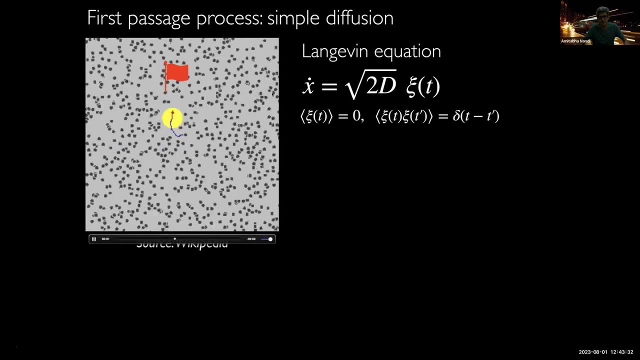 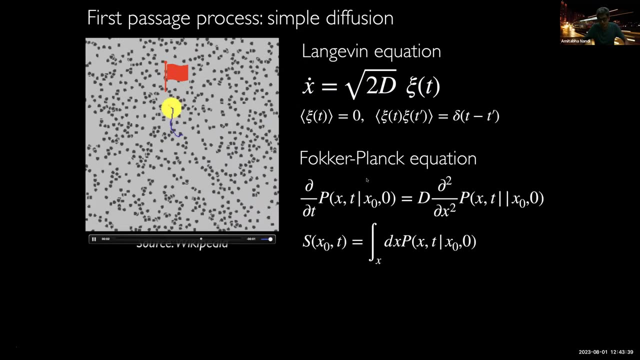 by integrating this probability Distribution And you can from this calculate the first passage distribution. And again, there is another way to directly calculate this probability of survival. I'm not going to get into these details, But the point is this is a very simple example. 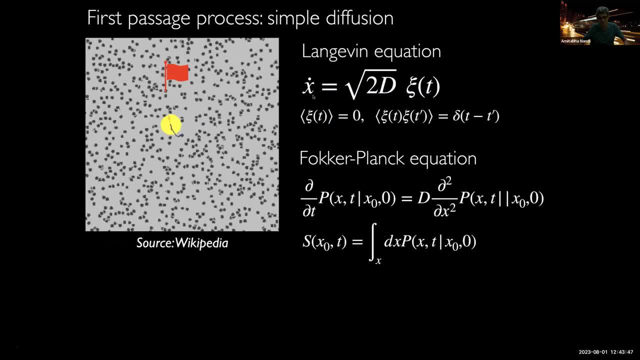 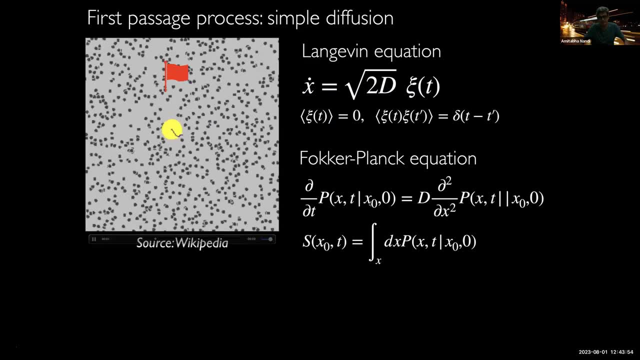 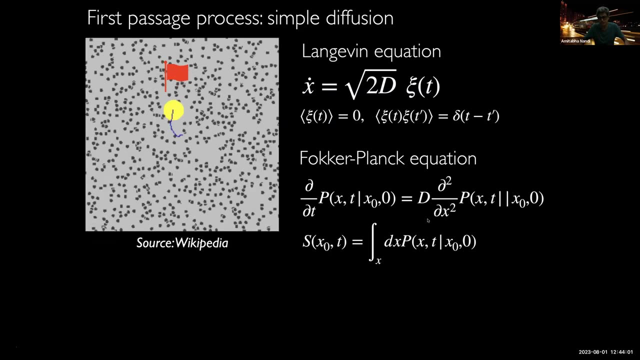 Now, if I try to add some complexity in this problem of the random walker, say I say that I have this random walker. Now I can find this random walker in a box, which means in the previous case this random walker could have a possibility. 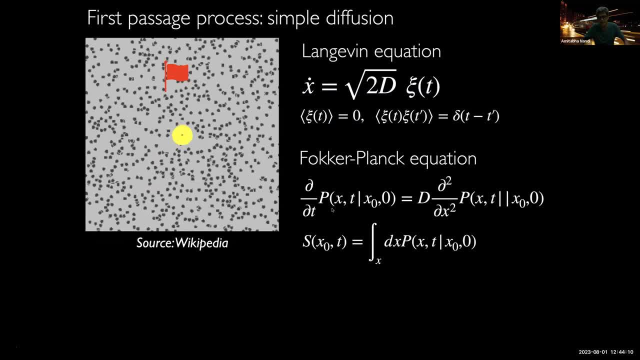 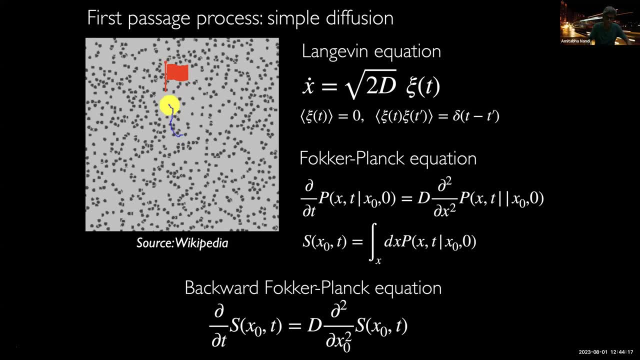 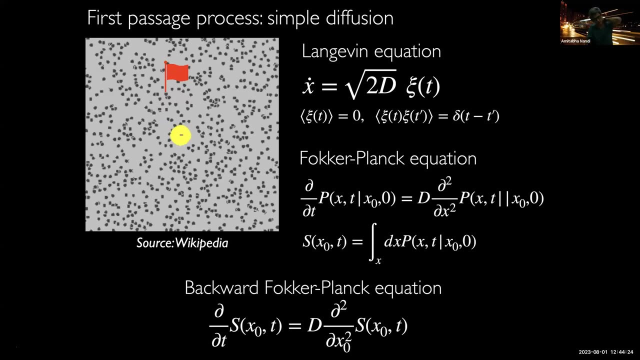 to escape to infinity, But once I put a box, it can never escape to infinity, So the mean time to reach this target will always be finite. OK, I can add. And now this problem can be solved exactly with this target being fixed. 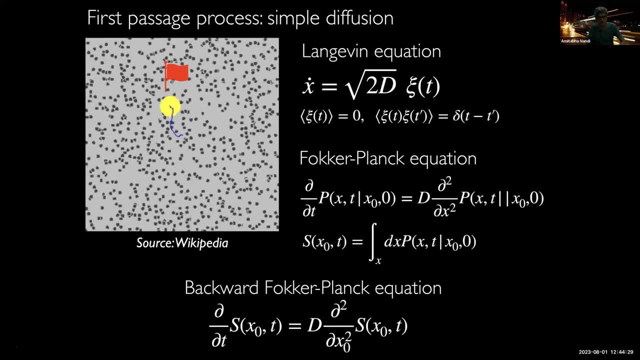 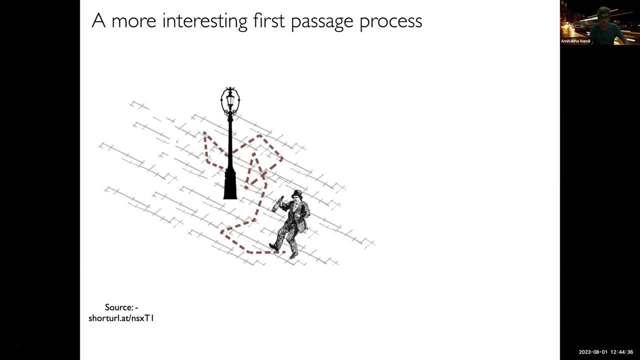 with whatever boundary conditions, I can use analytical techniques to exactly solve this problem. I can add an additional complexity where I say that, OK, there are more random walkers. Instead of one random walker, there are n random walkers. Everybody is trying to reach that target. 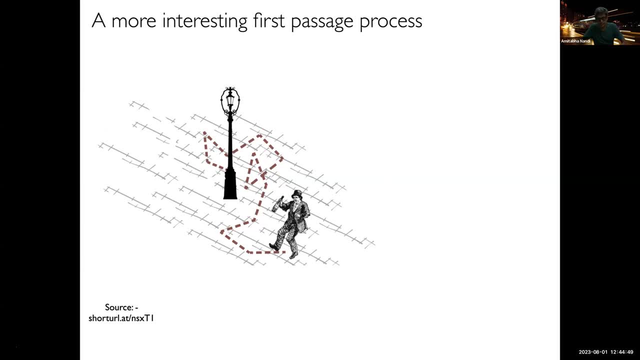 And I will just consider the situation where one random walker reaches this chromosome, this target, And the process is over. And even that problem is simple because this is a static target And if we assume that these random walkers are independent of each other, I can solve it as 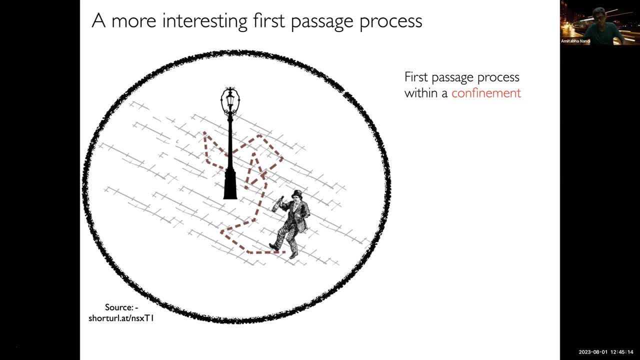 and I can factor out this independence. I can use this independence of the random walkers and factor out the problem, And that can also be analytically solved. However, if I now make this target also move around in this complicated problem where I have n random walkers, 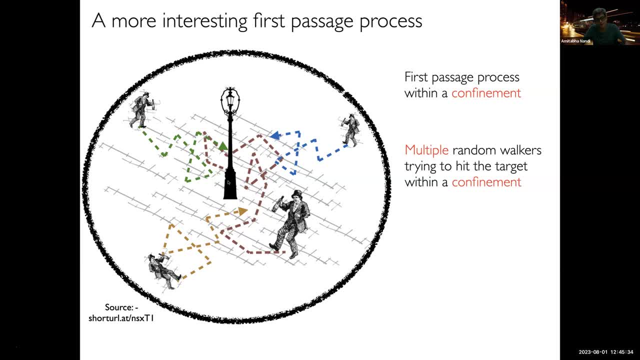 and this target moving around, then this problem becomes very complicated And one cannot use pen and paper to solve this problem And one has to use some kind of a computational method to solve this. I think there is a question. Yeah, Please go ahead. 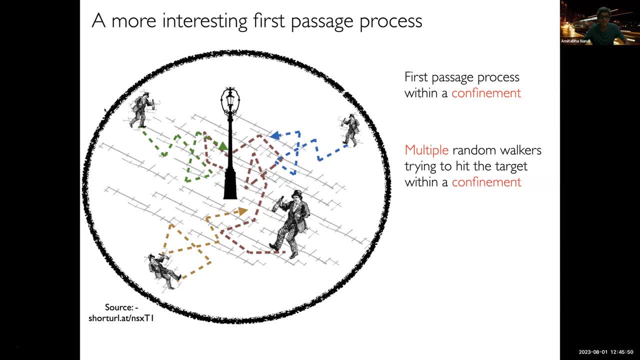 Also I should have a track. Yes, I had a quick question. So if the target is also moving, the intuitive sense I get is that maybe we cannot find a converging solution. Can you guarantee that there is a solution? Could it, in the worst possible case? 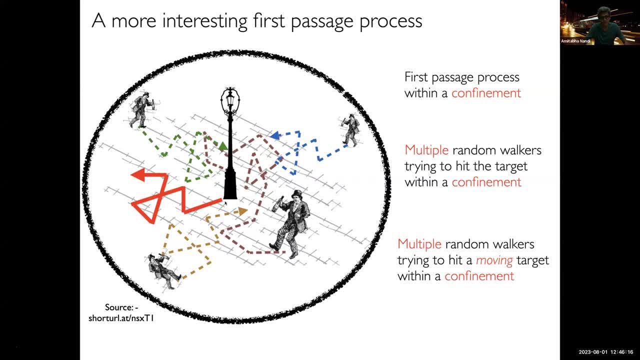 they will never reach the target, Because I'm assuming that the target is also moving randomly And the random walker are also moving randomly, So could they evade each other forever? They can escape each other forever. In this case, no, because you have an external boundary. 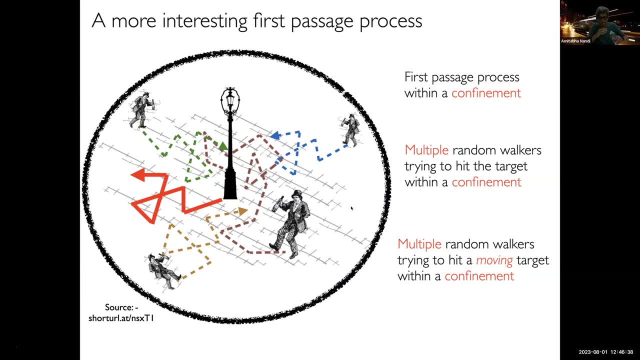 So this boundary will never allow this target to escape forever. So you think of this because these are not very smart walkers, They are just diffusing randomly. So because of this confinement, both of them are moving randomly, So this capture, on average, will always. 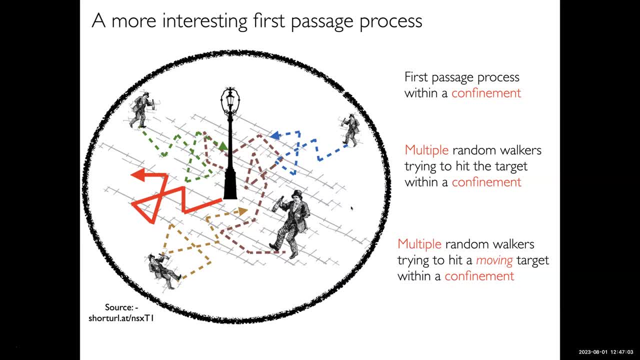 happen in finite time And actually what you have asked is a very important component and question in this study- that if there was no boundary, even with the static walker, this could have once in a while this walker could have escaped to infinity. 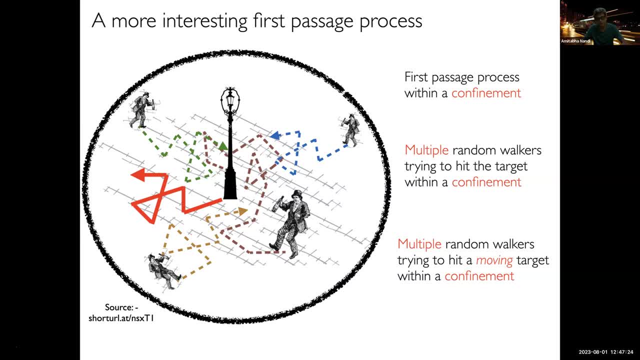 which means that if I compute an average time depending on the dimensionality of the system or the complexity of system, it can be infinite, But if we have a finite bound on this problem, this is never going to happen. It will always get captured. 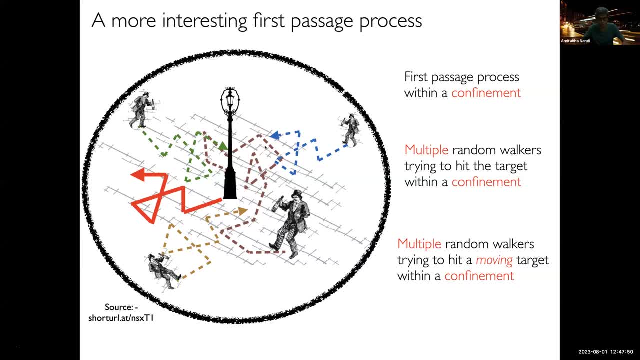 And can one write a closed form expression for the average time it takes if the target is also moving and the walkers are also moving? No, So that is the problem. And that is also a very good question because, as I was telling, I didn't give you the details. 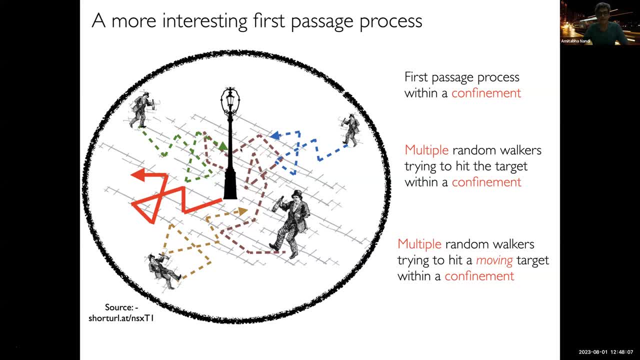 So let us try to see. So, if I have this problem, I have a target and I have this thing: no boundary, a single target is fixed. In this case, I can solve any of those equations which I showed in the previous slide. 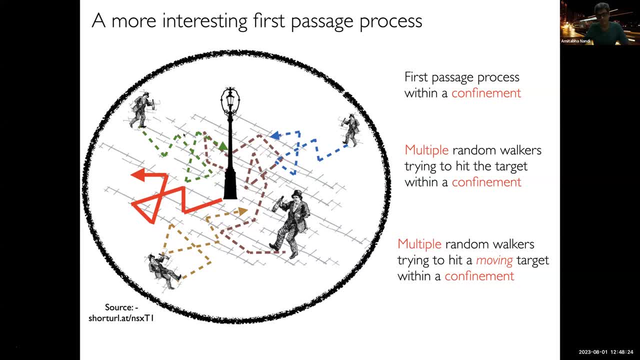 in a semi-infinite boundary and I can calculate the survival probability. and the survival probability has a power law solution. The moment I put this boundary, this survival probability will have some dependence on time, with an exponential cutoff Means what I mean by that. 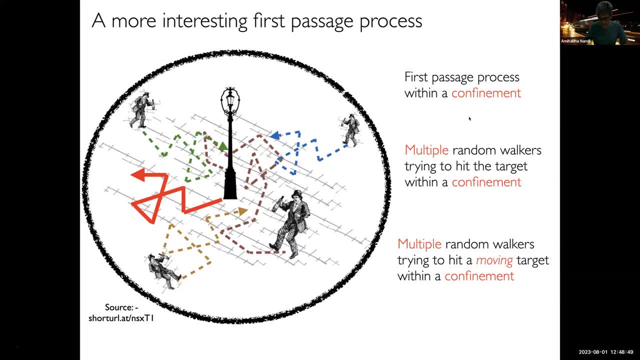 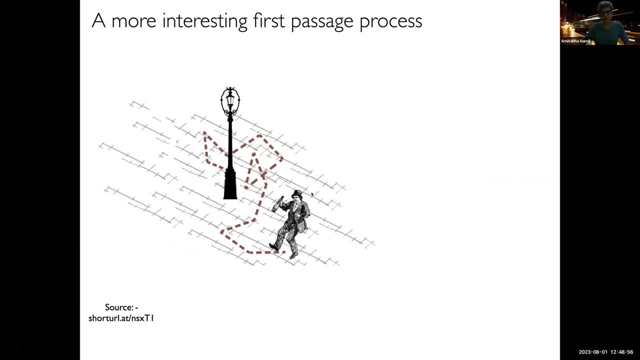 the survival probability at large times will be something like an e to the power exponential of minus t by tau, which means that the survival probability will always, like everything, will always get captured because of the boundary with a fixed target, And there also you can calculate the mean time. 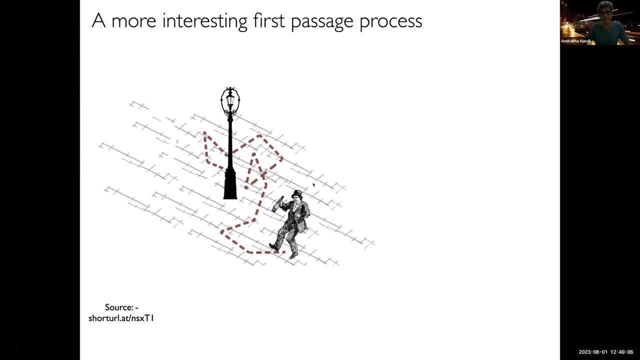 and you can have an exact closed form solution for the survival probability. Now, when you have this second problem, you have n walkers. Now I am assuming, since I can solve the problem for one walker with a fixed target in a closed confinement. 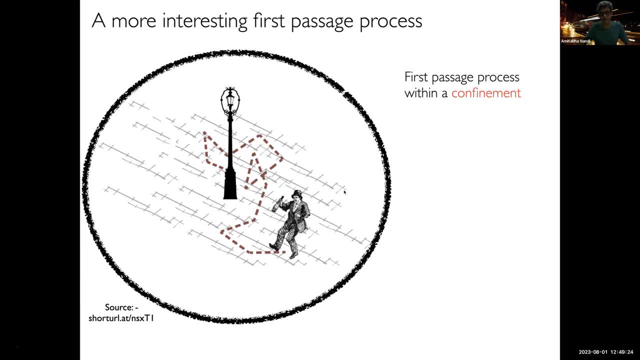 for n walkers which are independent of each other. I can say that I know the solution for n walkers. it will be whatever the solution for the one walker to the power n because they factor out, because they are independent of each other, If they are not independent of each other. 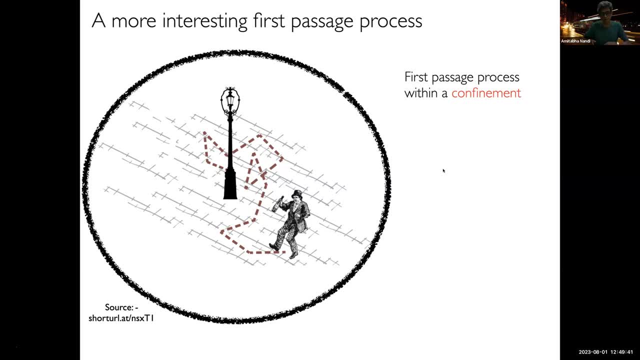 if there is an interaction between the walkers, then the problem is more complicated, you cannot solve. But if you assume that these walkers don't see each other- they can cross each other- then this problem is still solvable. The moment you put movement of this lamp. 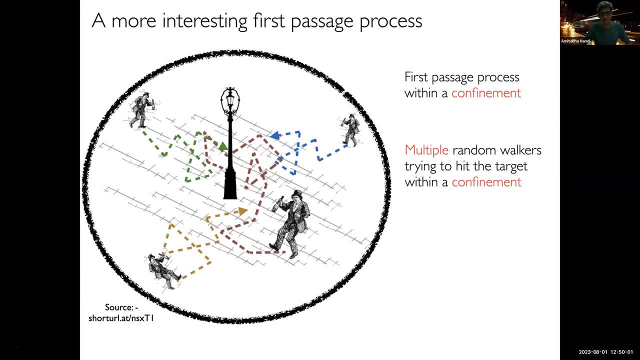 this target, then you cannot have a closed form solution. All you have to do is you can have a closed form solution in a simple case of one walker and one target moving, but not for n walkers. So that is a very simple case. 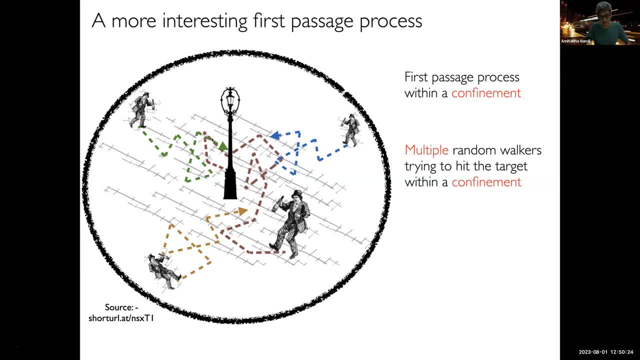 where you can get a closed form solution, But otherwise this you have to solve using computational methods. Thank you, Okay, And this is very important, because now you can see when I have designed this problem. this has been designed as a physics problem. 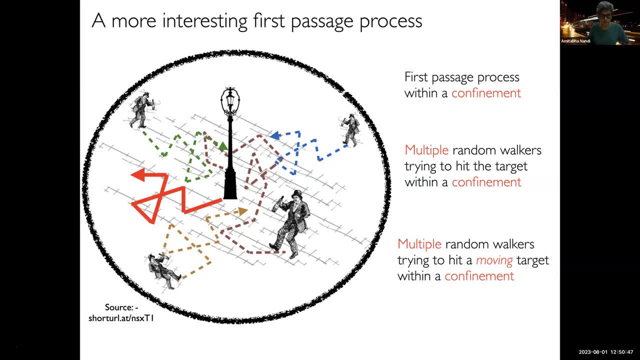 And the physics community or the stochastic processes community had been interested in the problem and there has been several papers in the study of this problem. without the confinement, The moment you put confinement, it becomes very complicated and you can clearly see that with this, this simple picture. 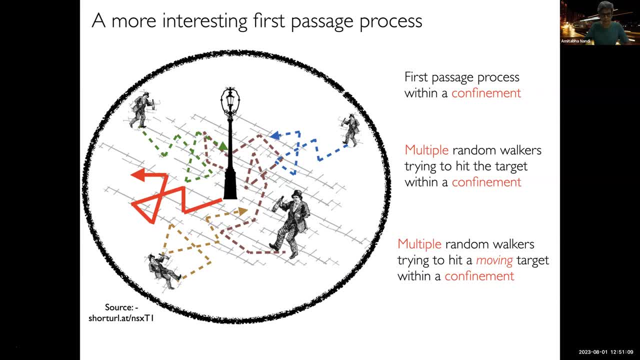 now you can relate to another problem, Right, And this is nothing but our problem, which of course has a more complicated like picture where you have rods diffusing and kinetochore, but roughly in spirit it is exactly the same problem. 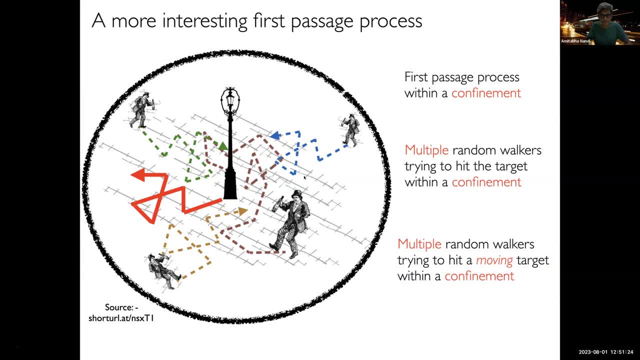 You have this random motion of the microtubule, random motion of the kinetochore, everything happening under confinement. So this is the kinetochore is the target, These things are the walkers, They have a more constrained motion. 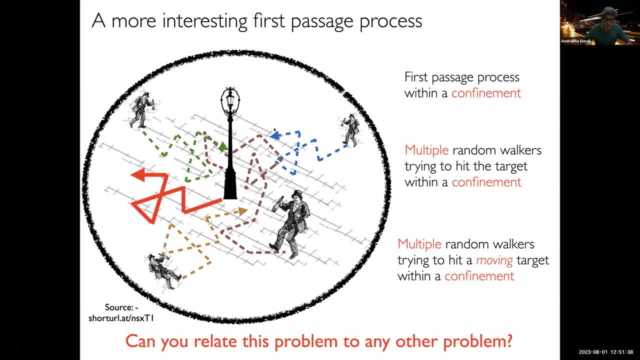 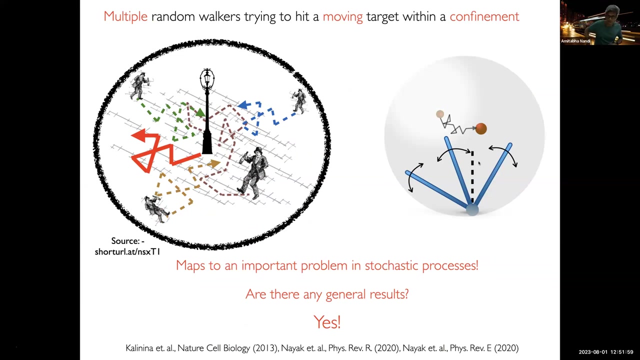 And what we have found is that, because of this mapping, some of the general results which we see in this case, in the left-hand side case, is also seen in this more complicated biophysical problem, And these were results which were discussed in some of these papers we wrote in 2020.. 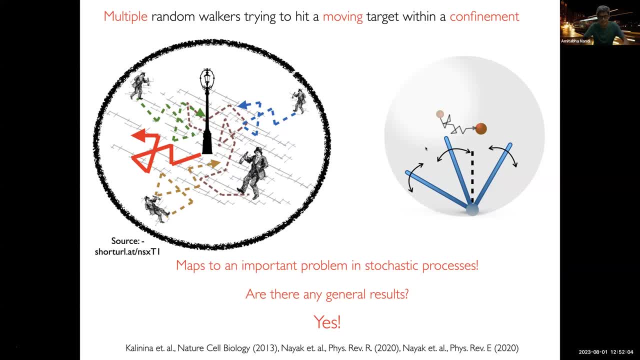 I will not go into these details And so this was a general extension. The other direction you can ask is recall in one of the early slide when we introduced the problem of search and capture, or capture of kinetochore in fissionists. 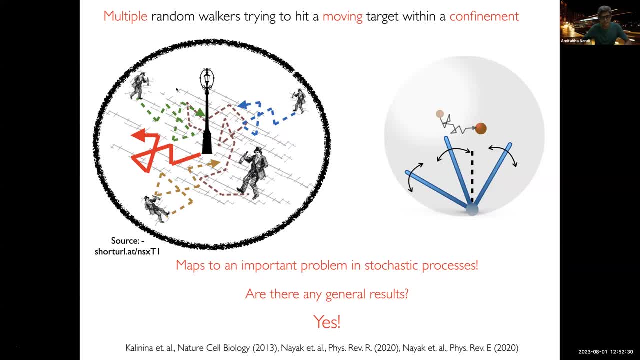 we discussed that in eukaryotic cells the capture happens in a different way. They don't do the microtubules don't do a rotational diffusion. There are many microtubules and each of these microtubule is dynamically unstable. 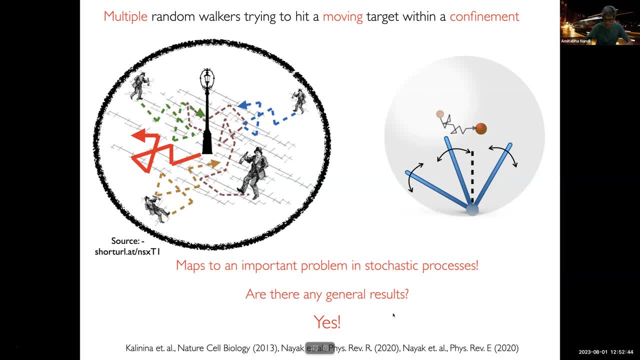 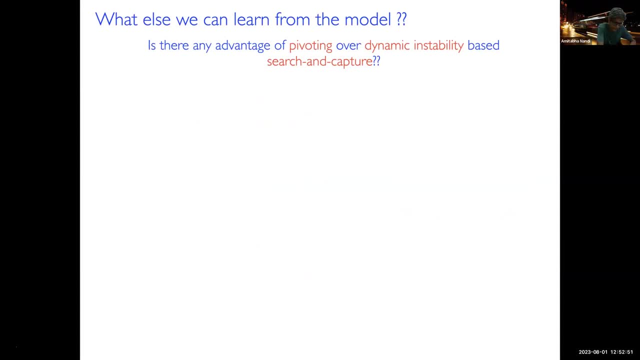 They are doing: dynamic instability along a given direction: growth and shrinkage, And that leads to capture. So now, with this model, and because we know also the model of dynamic instability, we can create a hypothetical model, a toy model, where we use the parameters for fissionists. 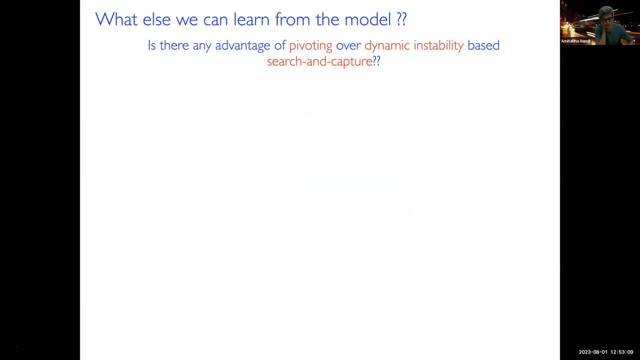 and ask this question: that in fissionists, why fissionists is not linked, using dynamic instability based search and capture, And instead it is using like a mechanism where the rods can do rotational diffusion. I mean it could have done a dynamic instability also. 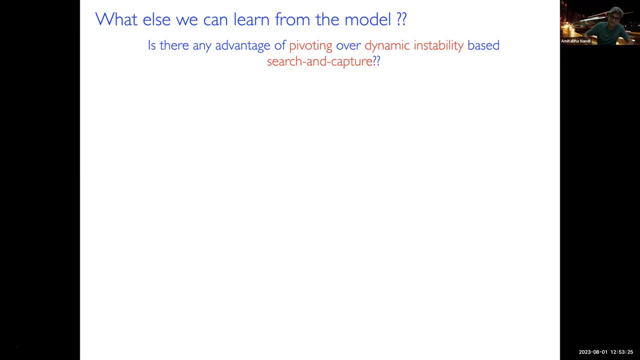 like the other organisms, And why this is not happening. Is there anything we can find out by comparing these two? So the question we can ask is whether to pivot or not to pivot in the context of fissionists, Why fissionists is pivoting. 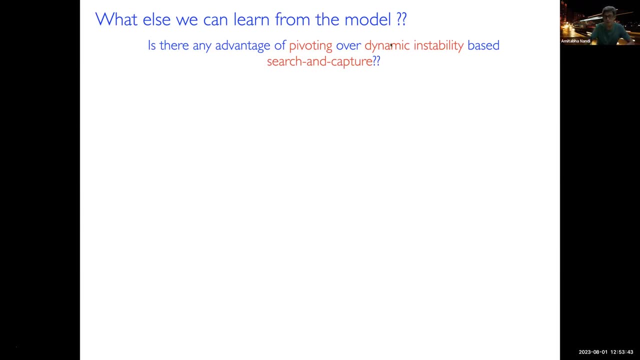 So this is kind of a hypothetical question And basically at the level of model we can compare these two scenarios. We compare a model where we do dynamic instability and compare a model we do rotational diffusion and vary the number of microtubules and see, we compare the time efficiency. 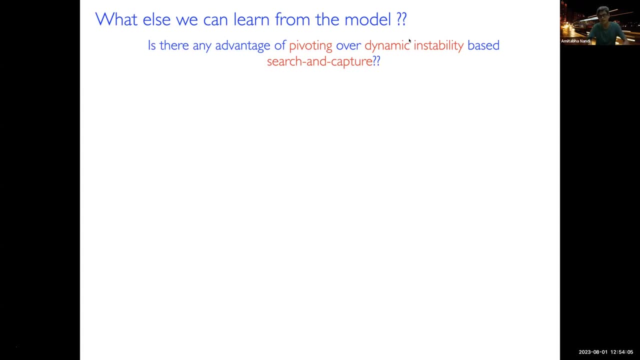 Which one happens faster? So yeah, so I wanted to discuss the second model. So this, actually this study is quite involved and it will go into much details. So I can continue on this problem, or rather go to a different example, But let me first give you, like the key result. 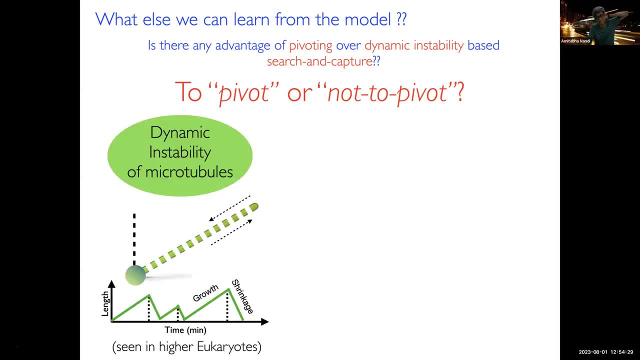 So what we found that with this comparison, that we found some like from the physics perspective or the stochastic process perspective, from the perspective of getting some general understanding, what we found that- and it is a very crucial understanding, what we gathered during the study, that if you are looking at a capture process, 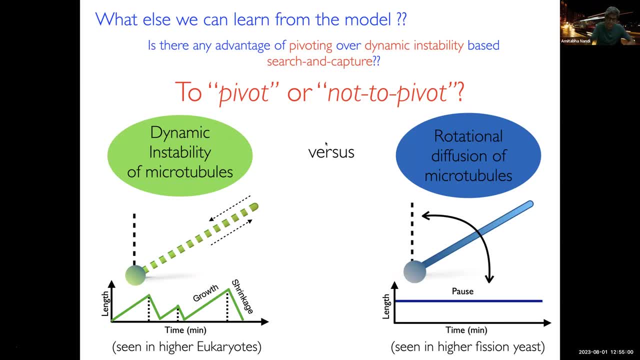 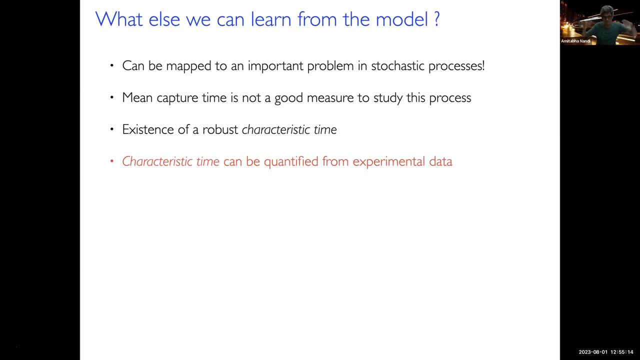 or stochastic capture process inside confinement. one should not- I mean one should- take the mean capture time with a pinch of salt. So because this mean any kind of average behavior could be a little misleading And that is introduced because of a very compact 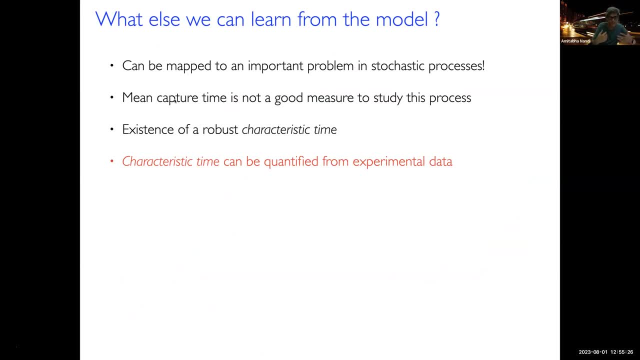 because of confinement, So I'm not going into these details, but if somebody is interested, I can go and show you what I mean by this. So this was an observation. And then the question is: so, typically, when we do some experiment or some study, 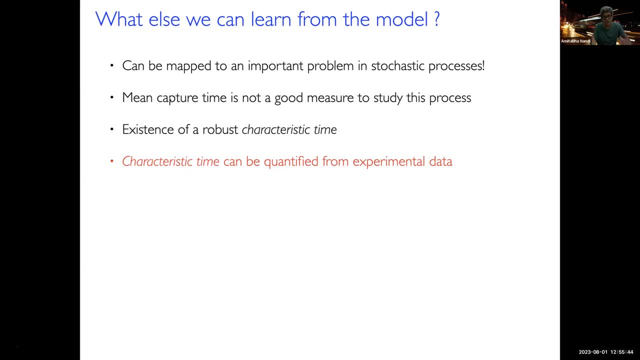 of some stochastic time evolution. typically, what we do is we calculate the average the second moment, and so. So it is very standard to calculate a mean. Now, if we cannot calculate a mean, what should we calculate? And what we found was: 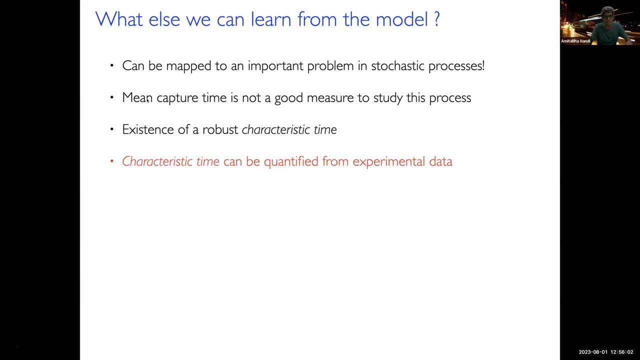 in these problems with confinement, there is an additional time scale which is very robust to any other variation, And this is called the characteristic time scale. Again, I'm not right now going into the details And this characteristic time. we can also 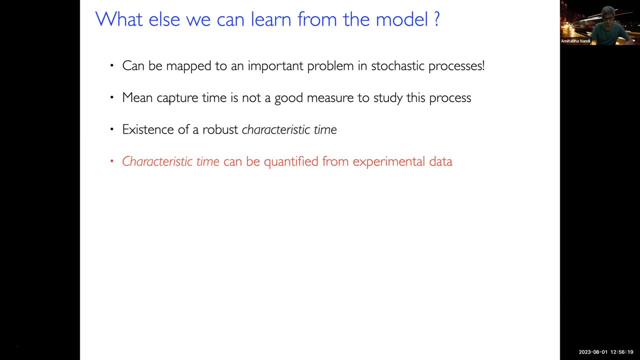 use something called extreme value statistics and quantify it from experimental data. Okay, so this is a very important and robust quantity. And what we found by running this, by running this comparison between these two different models? it gave a prediction that if you have less number of microtubules, 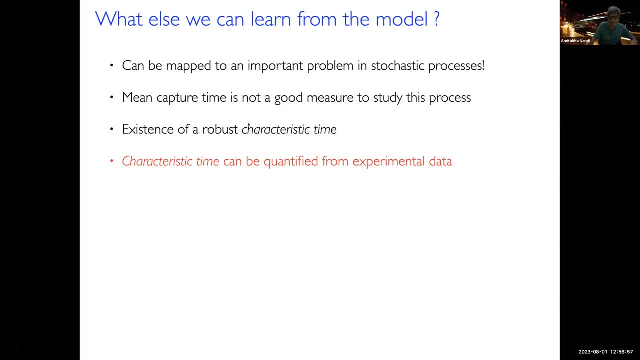 competing for, like trying to find a target, a moving target, then rotational diffusion is more efficient. If you have, if you can grow many microtubules, if you have, like a large number of microtubules which can like, 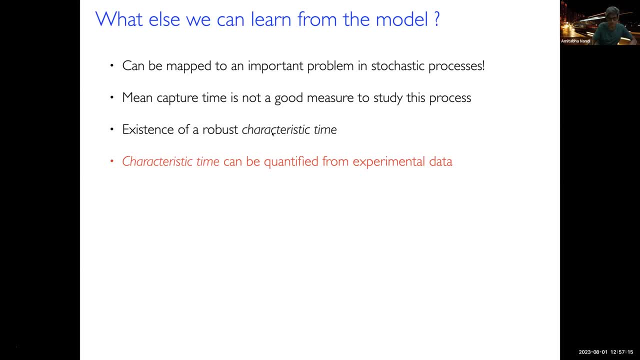 you have an like a larger source of tubulin, then it seems this search and capture, or dynamic instability based search and capture is more efficient. And this is somewhat interesting because in FissionEast we have noticed that the number of microtubules 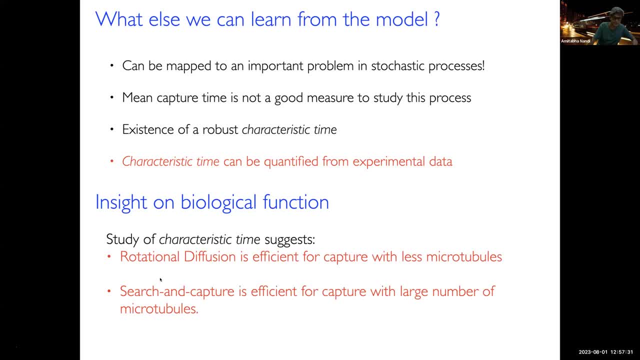 growing out of a spindle ball body is quite less. where we found. this was the dominant mechanism, Whereas this search and capture like which is observed in higher order eukaryotic cells. there, the number of microtubules is like: 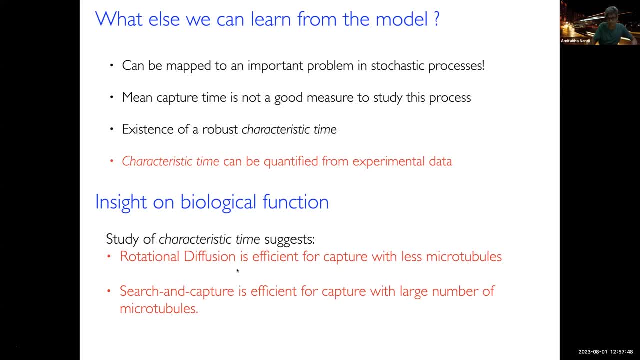 very large compared to FissionEast. So this, this actually gave us some idea or some hypothesis about the biological function, And this is so, so, so. so this was roughly the problem which I wanted to tell you or give you an overview. 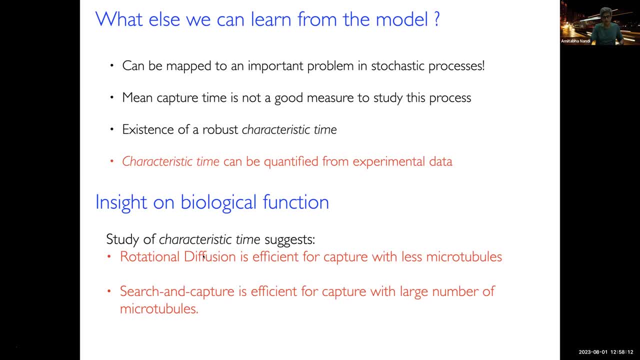 of how you can use the combination of experimental data, analysis and modeling to get insight about like the biological processes that is happening inside, like at the level of cells or tissues. I don't know how much time do I have? Do I have sufficient time? 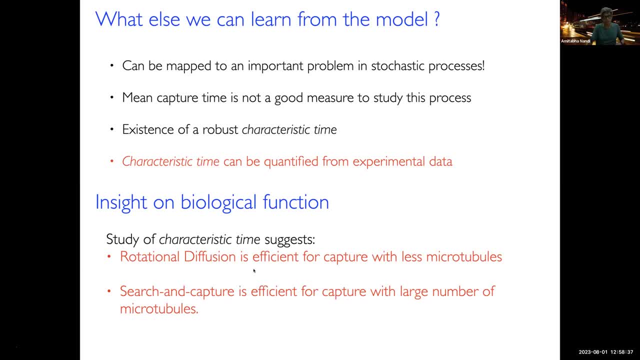 Also. the thing is I have skipped a lot of details here And I can also continue and go into the further details of this problem or discuss briefly about another problem where we can take a similar approach. So I don't know. So if somebody has any questions, 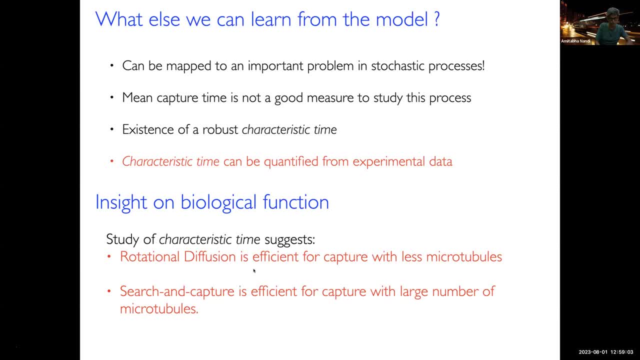 I can take some questions, like for the moment, take a pause and like address the question. Professor Amitabha, the scheduled time is still 1.15, but maybe we can go till 1.20 or so And so. 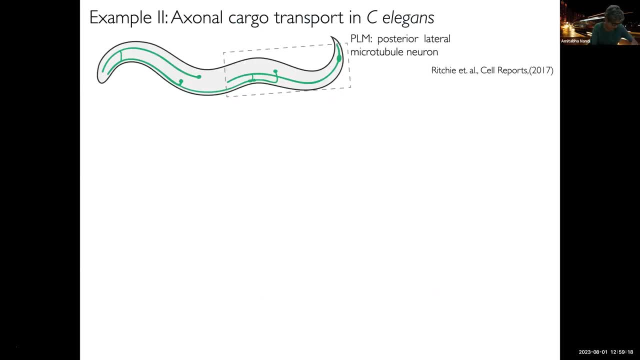 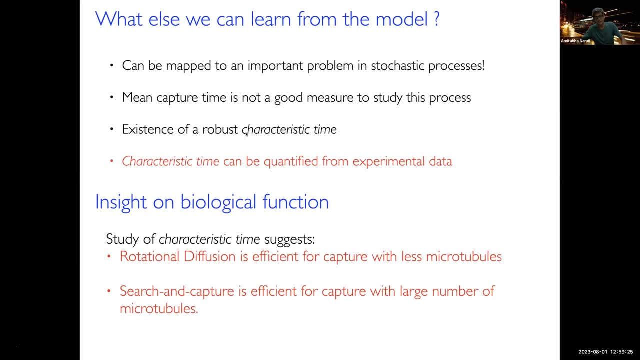 I personally would say we can look at another problem. so that gives us more variety. But I leave it up to you to make the final call. Okay, Okay, Sounds good. So then we can discuss the other problem. So are there any questions? so far, 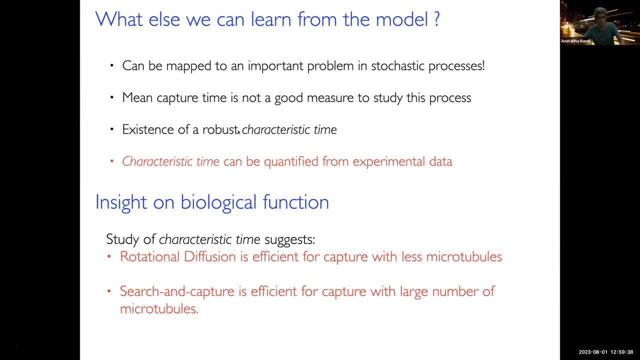 on whatever we discussed until now. Hello Hi, Yeah, Yeah. So I wanted to ask, like while doing the simulation, so to apply the boundary condition as in the confinement, like in the simulation? how do we do it Like? 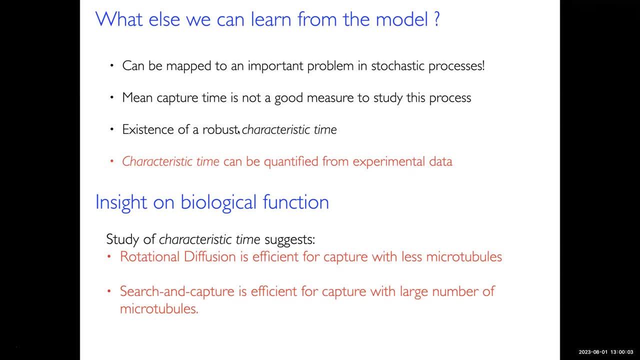 do we put some potential like, some bouncing potential or something like that? Yeah, Yeah, It is something like that, Like, but it is like a very like hard potential, So you can think of something like a reflecting boundary condition at the boundary. 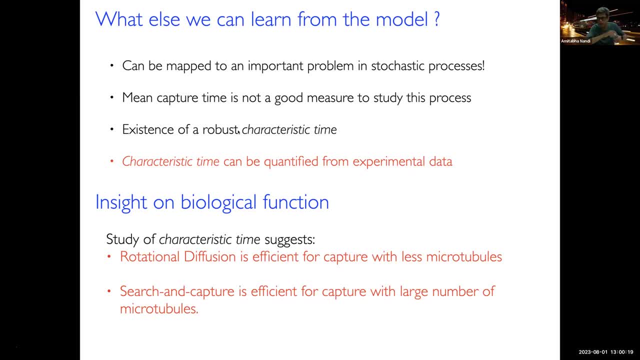 But I mean, we exactly don't know how the microtubule in reality will interact with the nuclear envelope. So if we know, those can be taken into consideration. but for the for the sake, at the level of this simple model, 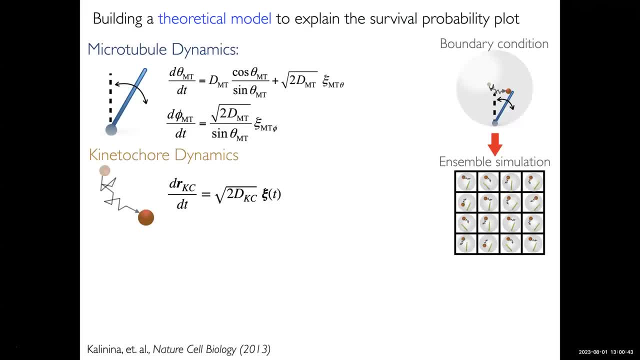 we just it is a hard wall, So whenever it it hits the wall, it feels it gets reflected back. Okay, Thank you very much. Another thing is like this: the characteristic time that we're talking about like from: 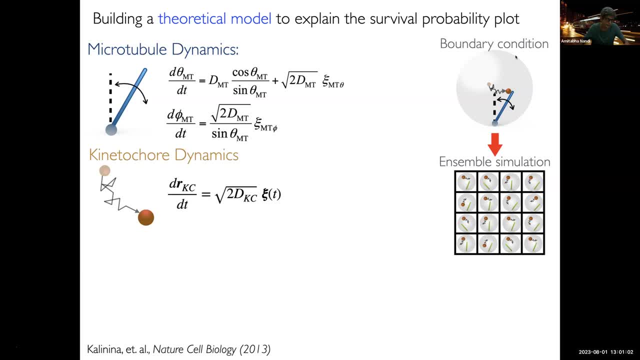 from what physical quantity are we seeing the? the characteristic time? Yes, Yes, This characteristic time. sorry, this characteristic time. I have to spend at least five minutes to tell you what is this characteristic time, So maybe I can digress. 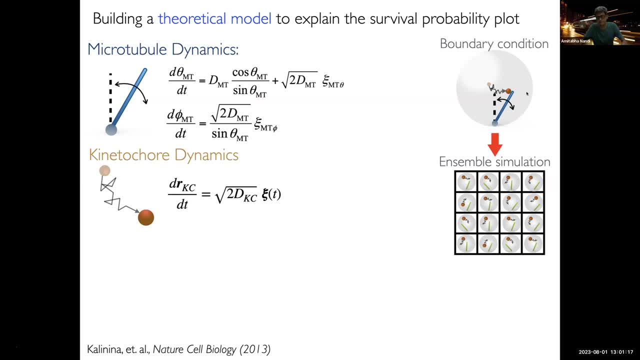 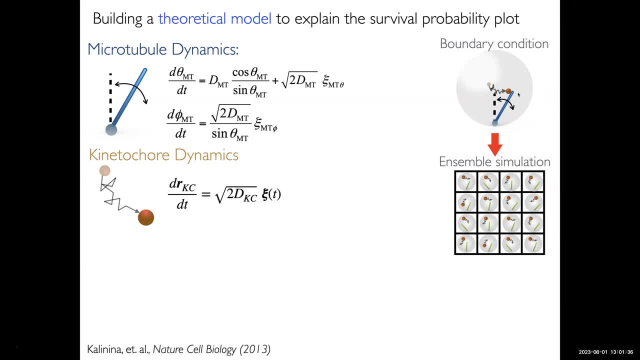 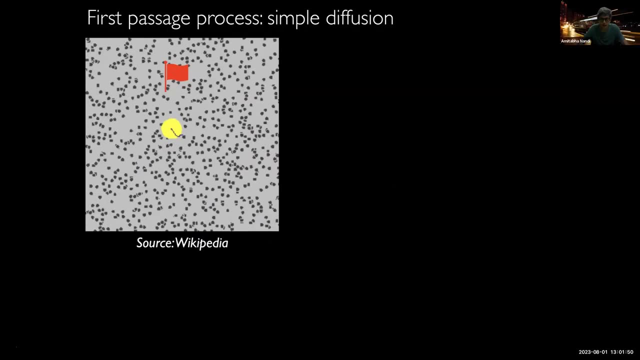 yeah, I will first let me see. Okay, So again, I'm showing this through this cartoon. So consider: I have these two random workers. One is a random worker, another is a target, and they are diffusing freely. 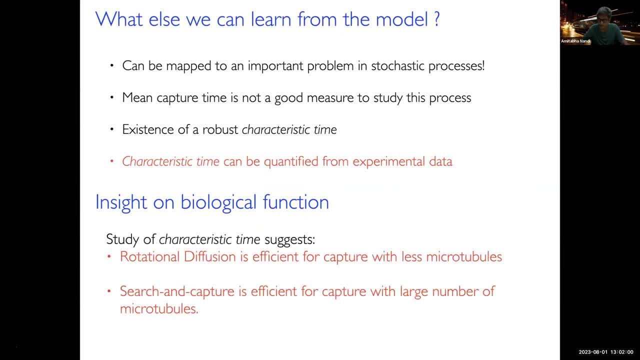 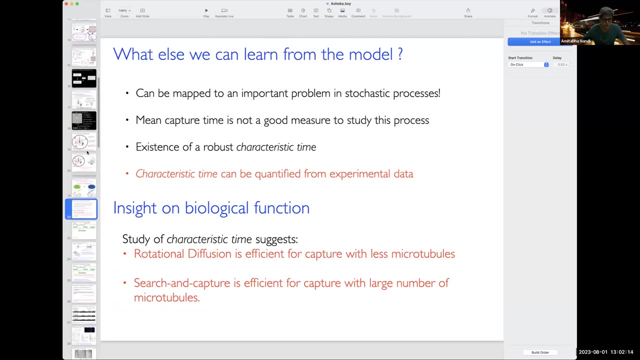 Now they hit each other at some time. t and if I do this experiment again and again, I can find a distribution of this t. Now, as I have said, in free space, one can show that this survival probability will have, at large times, have a power law dependence on the time. so it 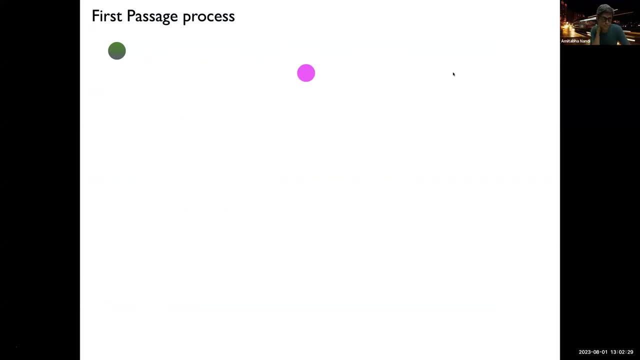 it scales as t to the power minus beta. and this beta can depend on various things. it can depend on the dimensionality of the problem and if you introduce more complexities in the problem, but for the moment, like if it is in free space where you don't have any bounding, any bounds, 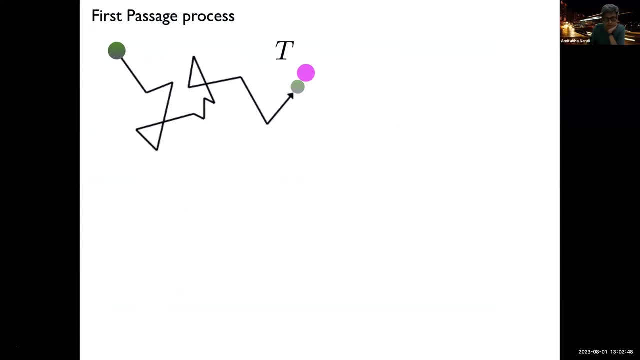 it. at large times it will be some power law. That means now, if I calculate the average time, the average time is nothing. but whatever is the survival probability, it is the total cumulative distribution of the survival probability or the area under the curve. one can show that, So one can also. so if this is, 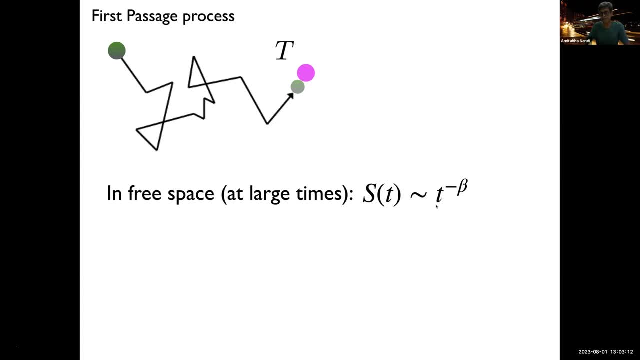 the first passage probability, the average time is t times f. t and this relates to it just gives you an integration over all time, the of the survival probability. So you can see that if you have like a power law and depending on the exponent, for example in like simple, 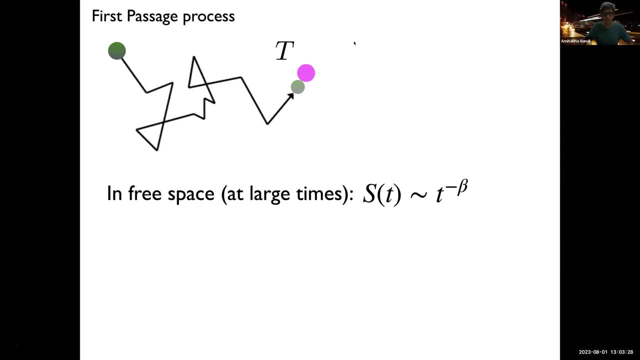 probability Problems. this, depending on the exponent, this mean time can diverge, and the intuitive way to see it is because once in a while, every time you do this experiment, once in a while, this will escape to infinity, so the mean time will be finite. Now the thing is the mean. 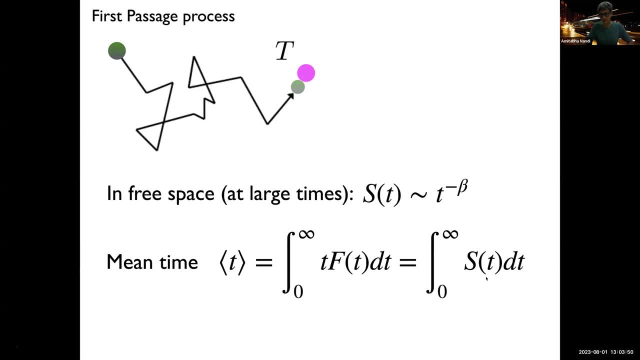 time will be infinite. yeah, now, when you put a box, you will mean time will always be finite, and one is it to get an exponential tail of the survival probability. So whatever is the survival probability form, it can be very complicated. At large times it will reduce it. 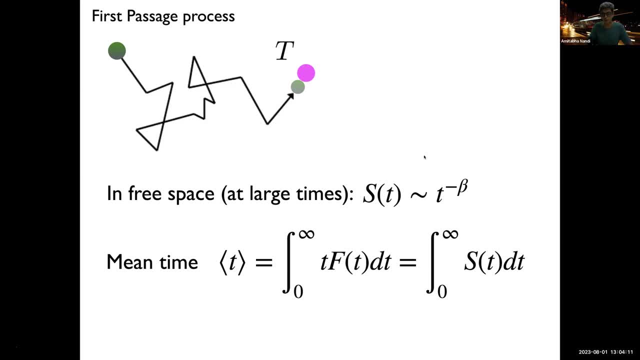 will decrease exponentially fast. Basically, it will have all the polynomial powers in its form, And if you have such an exponential tail at large times you can see that I can write some t by tau, And this tau is nothing but the characteristic time. 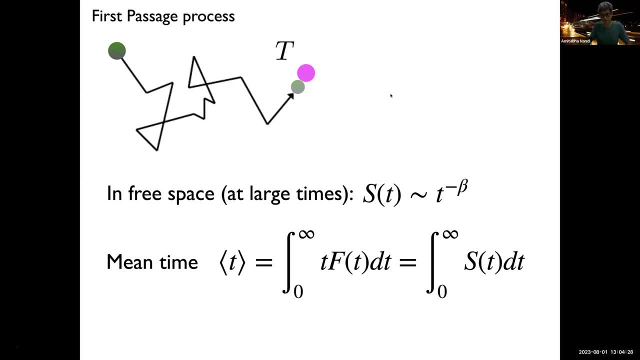 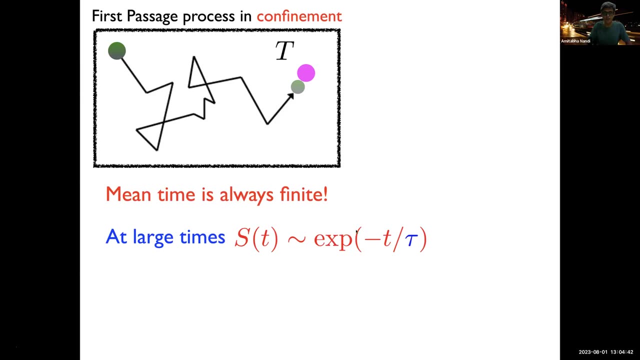 And this tau depends on the intrinsic parameters of the problem. And for some simple cases one can calculate tau, But otherwise you have to estimate it numerically. So this was another thing. I will briefly tell you So in our problem, because it was a numerical problem. 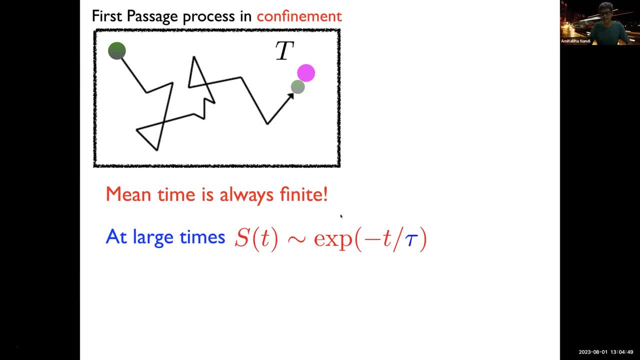 it was very difficult to find tau Because, you see s, the survival probability only has an exponential tail at very large time, Which is very small. when this survival probability has become very small And to computationally extract tau is very challenging, 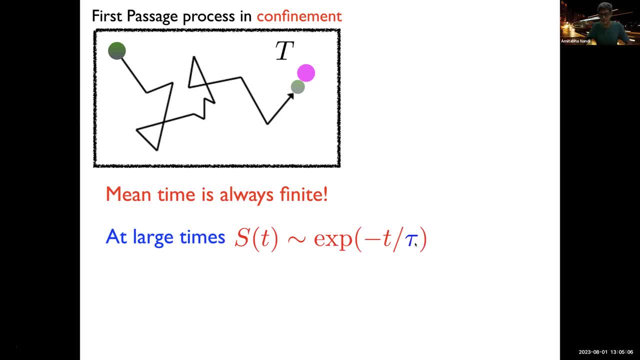 So it is associated with the rare capture events. So what we had was we actually found out an algorithm. I will skip that. We found out an algorithm to find out this tau, Which is like using some kind of a replication. Again, this is I'm not going to discuss. 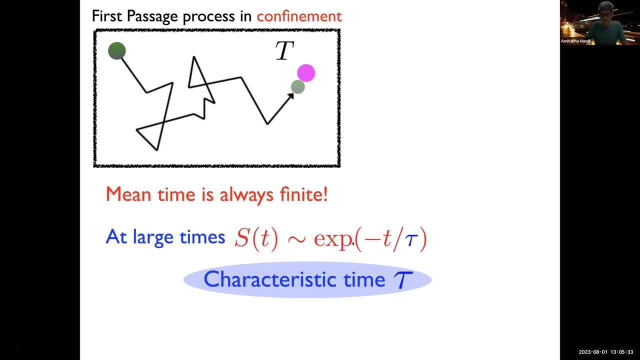 And we found that we can estimate tau up to a fair degree of accuracy and generate the survival probabilities up to a very high precision. So the bottom line is this: characteristic time tau is associated with this exponential tail of the survival probability. So I gave a longish answer. 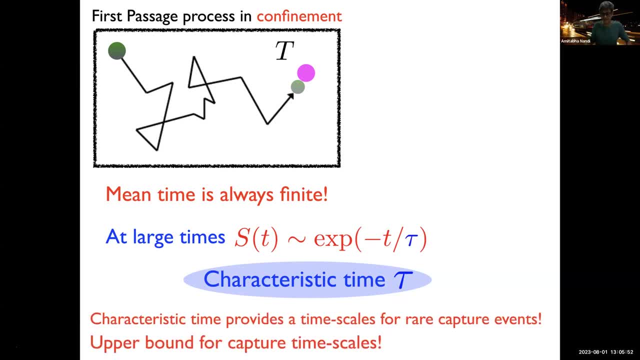 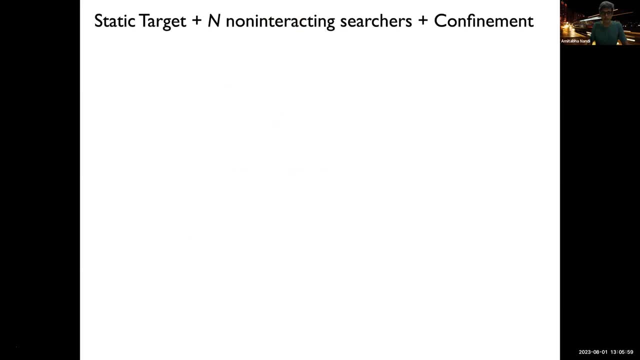 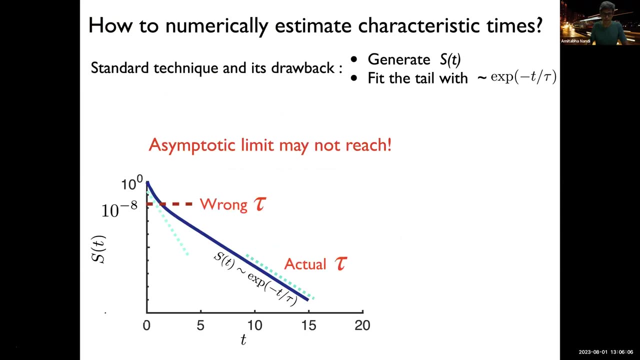 But I hope that addresses your question. Yes, yes, Thank you so much. OK, So let me go back and spend the next 10 minutes or so to discuss this other example. So now that we have discussed at least the first part, 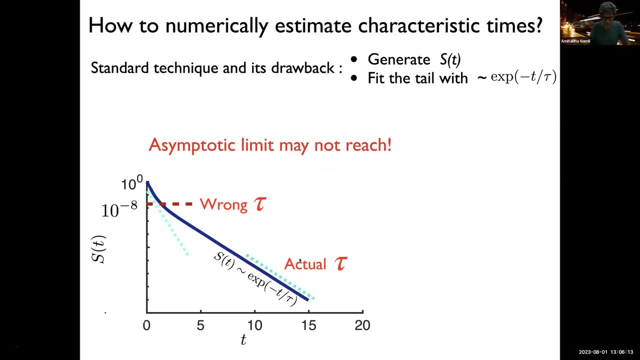 at least the formulation of the problem, rather in details. So this second problem. I will try to go a little faster. So in this problem, what we are interested in, we are, we wanted to see, We want to see transport of cargo along these very specific 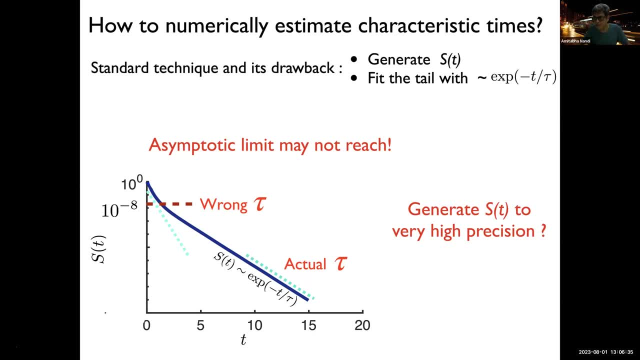 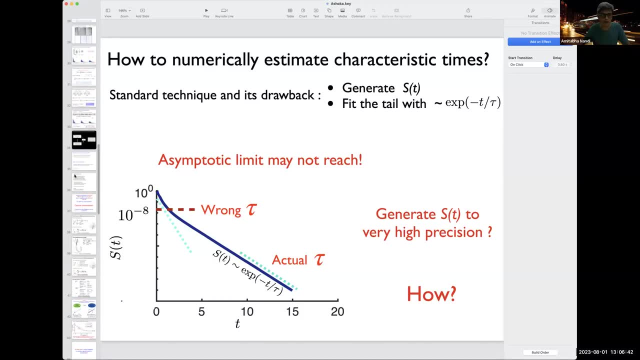 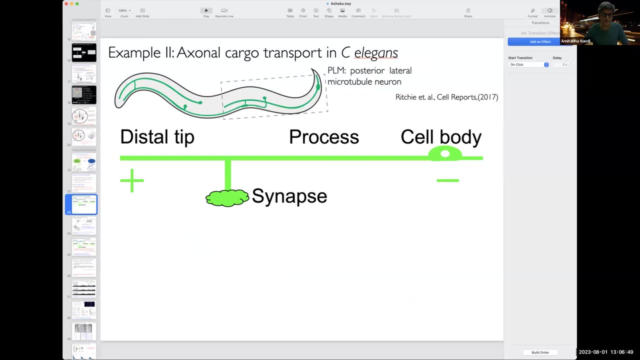 neuronal cells, which are called axonal cells. So this is a warm body, a C elegans body, And this is a cartoon. And what has been labeled inside this C elegans schematic are these different axonal cells. So what we are interested particularly in our study. 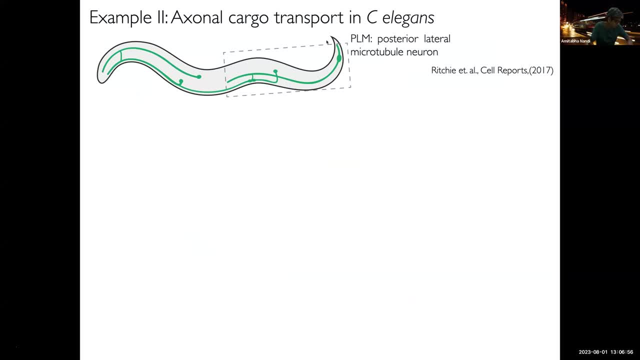 is this particular Axonal cell which originates from the posterior side of the warm body. Now, if I try to zoom in and show a schematic of this axonal cell, it looks like the following: So it has a very long shaft or axon. 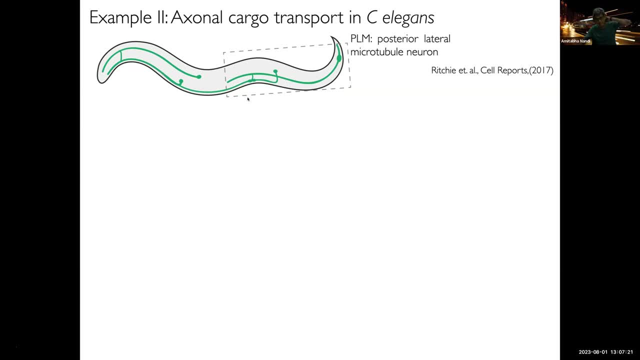 which is made up of microtubules. It has a very condensed cell body And this axon has a polarity And it is the polarity of the microtubule, because the microtubules themselves has polarity, which is a structural polarity, because 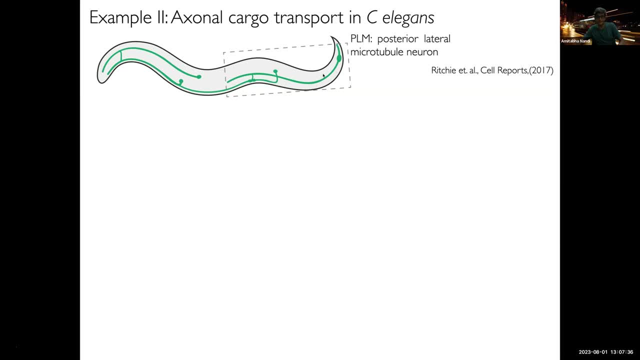 of the way this alpha and beta tubulins are arranged. Now what we are interested here is how these specific motor proteins, namely the kinesin proteins, which always walk from the minus to the plus direction along microtubules, they move along. 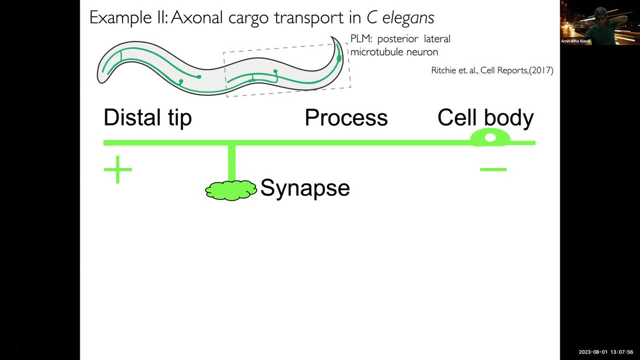 And what we are interested in is how these kinesin proteins are moving along this axon in a directed fashion, And so these are the different parts of this cell body, This is the distal teeth, And so, basically, what these kinesin motors will be doing. 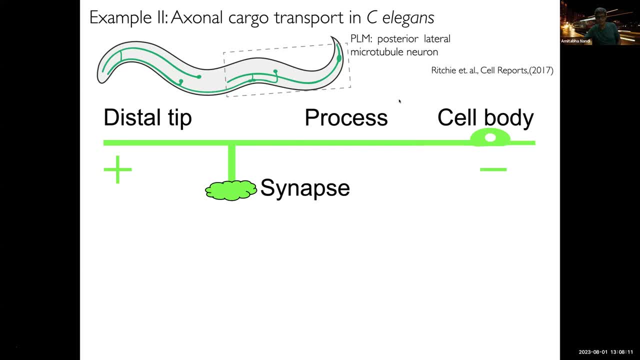 they will be carrying cargos and nutrients from the cell body And they will walk along the microtubule and try to reach the distal teeth. So there are also connections to the other axonal cells through the synapses. And this is just to give you a recap of what these kinesins do. 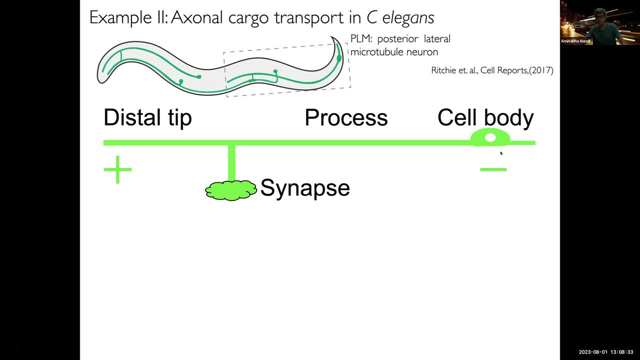 in case, like I'm sure everybody knows. So these kinesin motors. they are able to hydrolyze ATP And whatever energy released. they can use this chemical energy to do mechanical work, in a sense that they can walk along the microtubules carrying 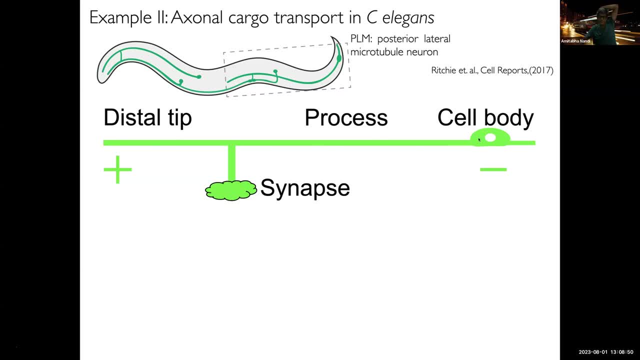 a cargo. So this is like a GIF of this movement of a kinesin carrying a cargo. So they move with a constant speed And this has been very well studied over the last two decades or so And typically this is the typical speed. 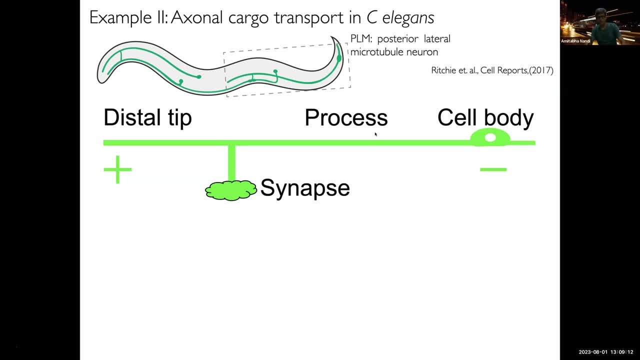 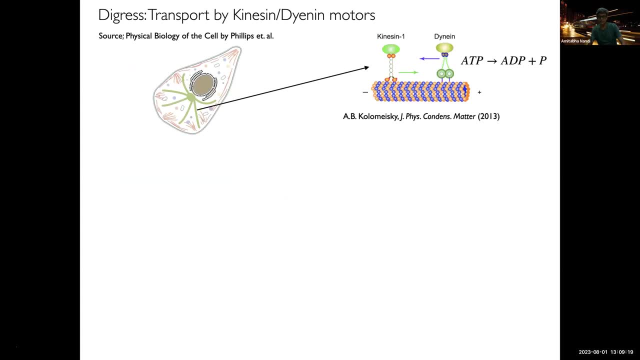 of a motor walking along a microtubule: 1 micron per second. And if you know the diffusion coefficient in free space, one can see that for traversing large distances it is always, again, time efficient to use this kind of ATP hydrolysis. 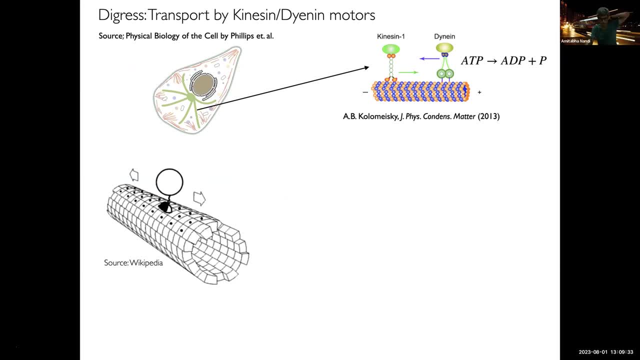 and transport material using these kinesin motors. OK, So one can also model the dynamics of this attachment-detachment of these motors to the microtubule and all these things. So these have all been very well studied over the last several decades. 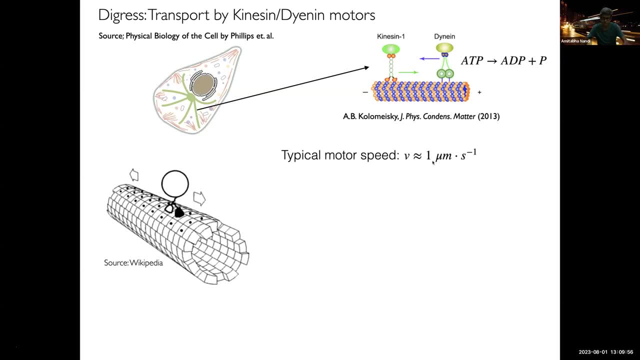 The last two decades or so Now, given this motivation that we are interested in studying how kinesin-assisted transport along these very long microtubule axons- axons made up of microtubules- happen, so we are interested in this following question: 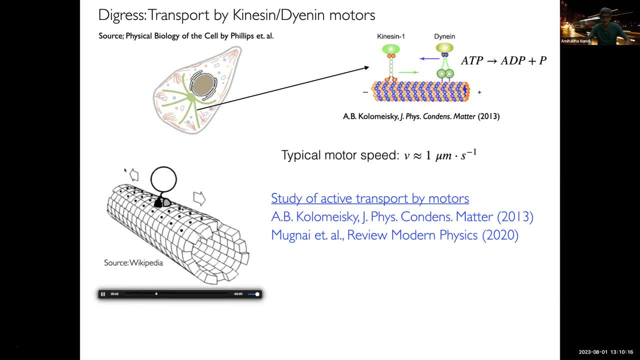 So this is like a biologically relevant question. It's the following: See, think of this- that you have some distribution of kinesin motors. Now these kinesins will carry vesicles or nutrients from the cell body to the distal deep. 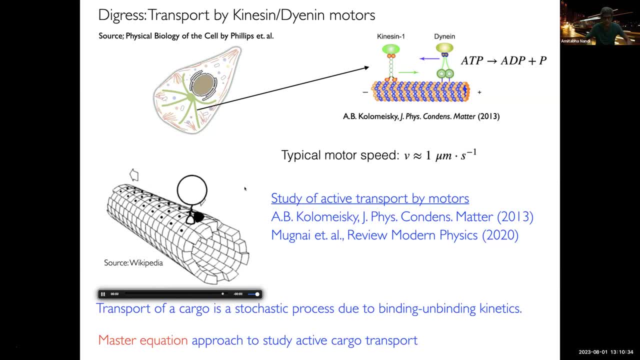 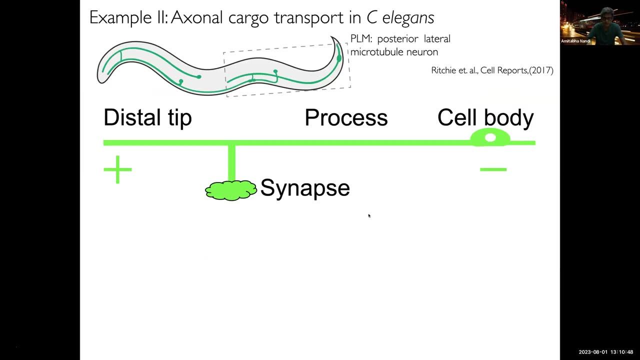 Now you have to strike a right balance of how many kinesin motors you want to use, so that you don't deplete all the kinesin motors Like you don't use up by taking all of them at the same time from cell body to the distal deep, so that later there are 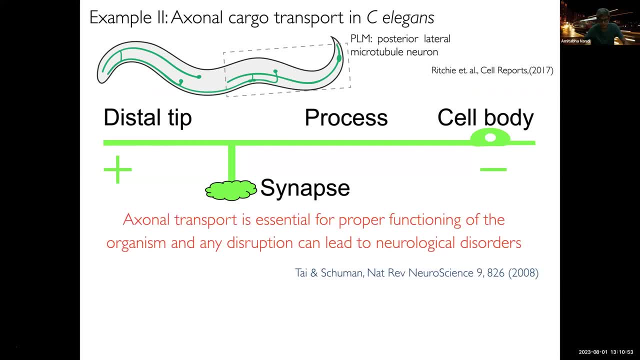 no kinesin motors. There are no kinesin motors available here to carry further nutrients, So regulating the kinesin distribution over the whole axonal length and particularly near the cell body is very crucial. Otherwise this can lead to large-scale disorders. 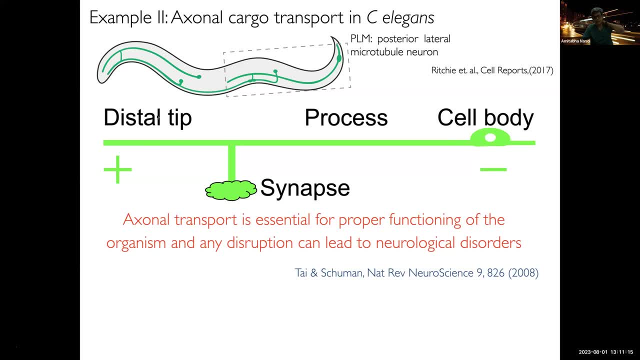 in a grown-up like a proper developed organism, and neurological disorders And one interesting thing. So basically the question is: what is the mechanism of cargo transport And can we build up a model And how it is biochemically regulated? 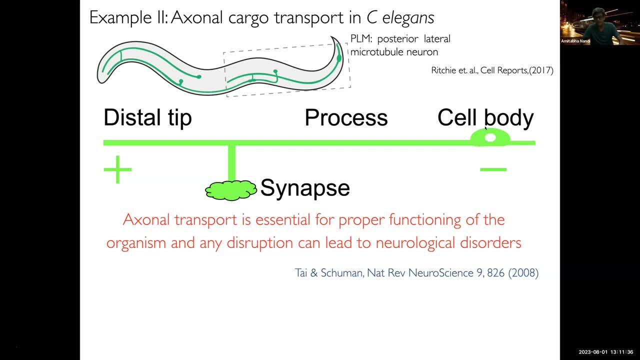 how the distribution of kinesin motors or cargo is biochemically regulated. So in this context, what our experimental collaborators they were interested was to understand the role of a particular protein Which is called ubiquitinine And basically it is ubiquitous everywhere. 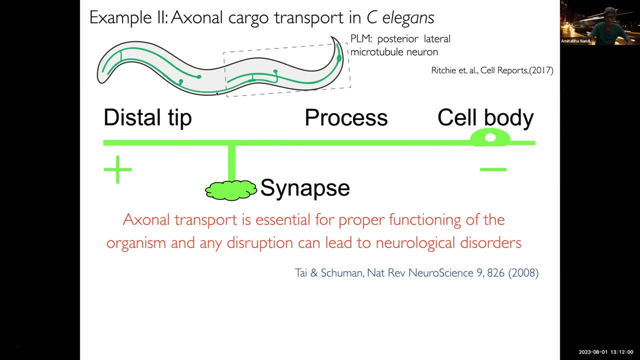 And this protein is known to play an important role in degrading many other intracellular proteins, So, for example, ubiquitinine. if you take proteins and redistribute and accumulate at a different place, so at some point this ubiquitinine will play a role in degrading those proteins. 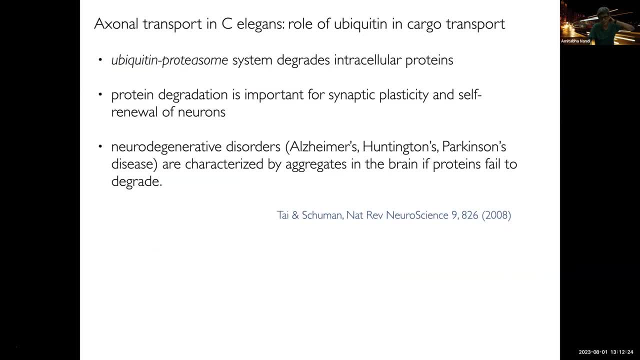 And the other side. So this is known, And it is also known that if you somehow mess around with this ubiquitinine protein concentration, this can lead to neurodegenerative disorders. And so the question we are interested in is: does ubiquitinine also play a role in cargo transport? 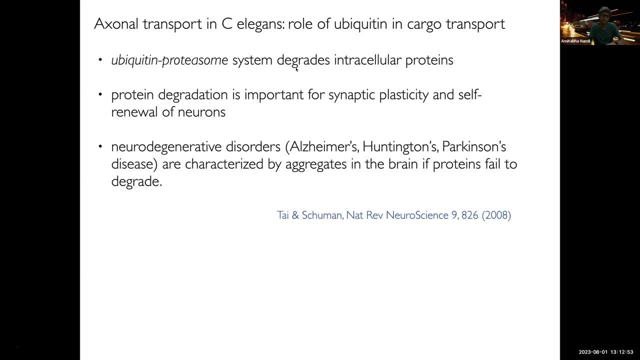 along the axis And if yes, how? So this is the main question. So now, clearly, you can see. the only way to see what is the role of ubiquitinine in cargo transport is to first do an experiment in the normal wild type. 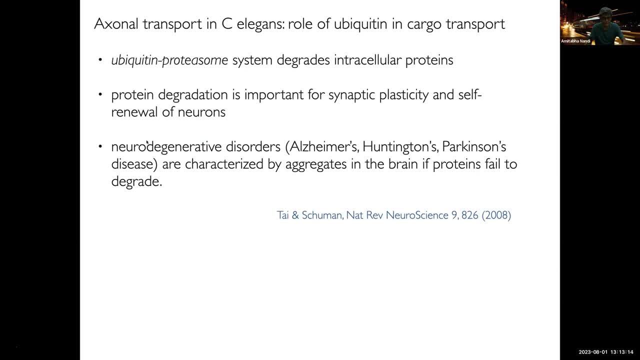 And then repeat the experiment where you have somehow knocked down ubiquitinine or increased ubiquitinine. OK, So this is what is done here. So these images are snapshots of the whole axonal cell at steady state, And the first one is for the wild type. 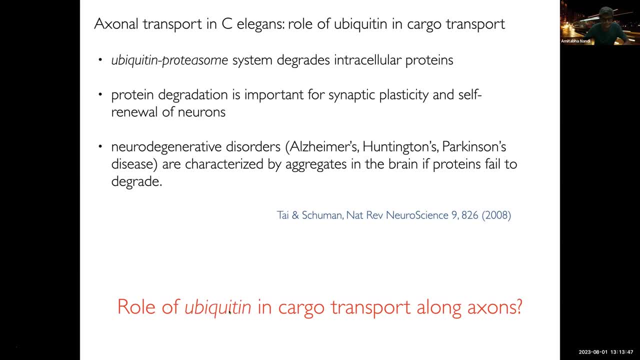 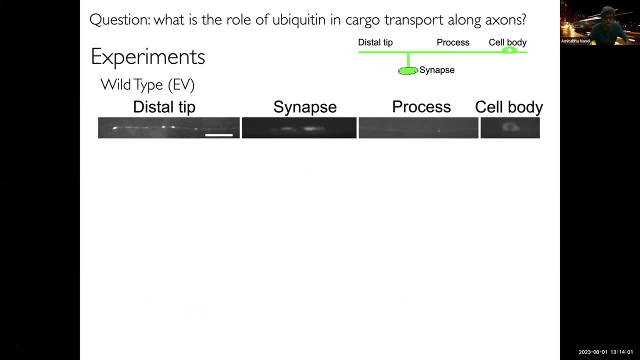 The first one is for the wild type And the fluorescence. what you see here is that of the kinase, And the fluorescence is the number of kinase-en motors. So anywhere you see a bright fluorescence that corresponds to a larger number of kinase-en motors. 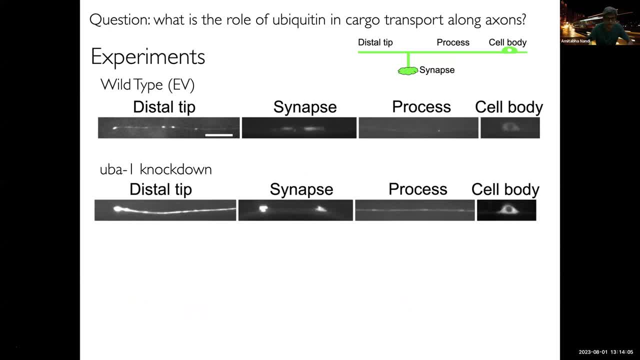 at that point in space. So you can see that this is the cell body. You see some brightness because of the kinase-en motors And at the distal end you see a larger fluorescence. However, if you knock down ubiquitinine, you see that there. 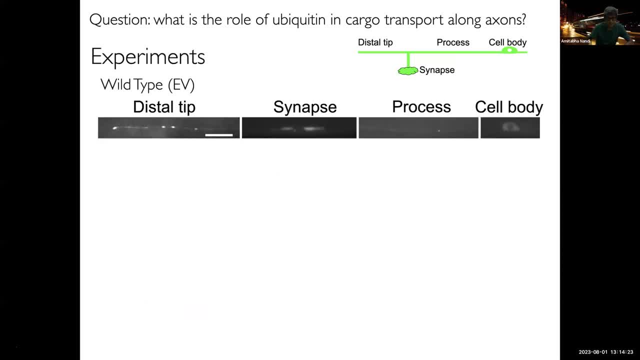 is in this fluorescence, which means that there is more kinesin at the distal end. So somehow the number of kinesins has increased. So there were some other experiments also, which is a more direct control of the ubiquitin pathway. 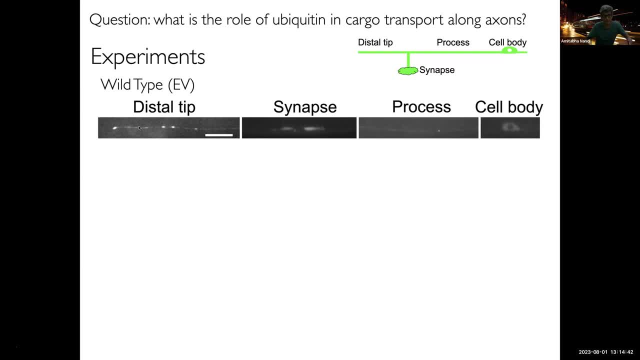 This is this FBX knockdown And in that case also, you see that there is an increase in the number of motor proteins compared to the wild type, these kinesin motors. So I think I'm almost at the verge of like my time. 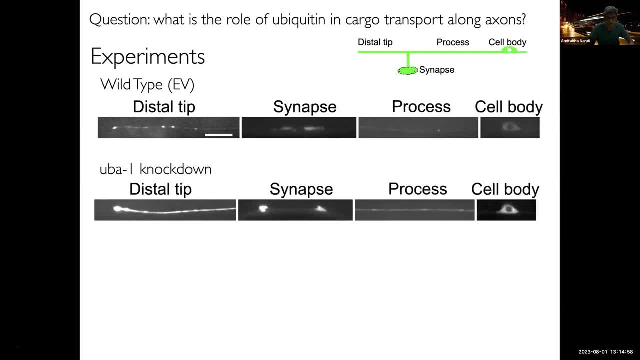 is kind of over, but let me just quickly go to the like. So we have several quantifications which I won't have much time to discuss. But one can do like, because these motors carrying cargo are always moving from the cell body towards the distal end. 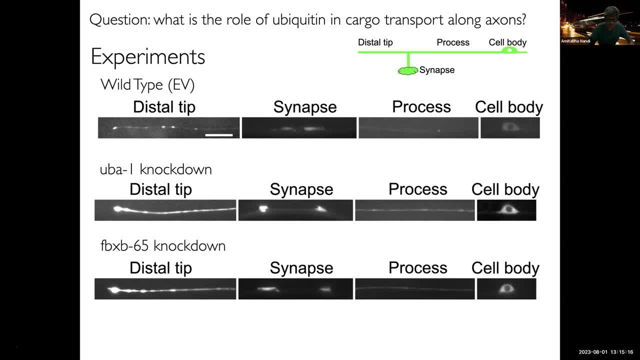 so you can do experiments like make a cut, a laser ablation on the axon And see what kind of distribution you see after the cut And as expected. so you see that as you make the cut, on the left, on the right-hand side of the cut, 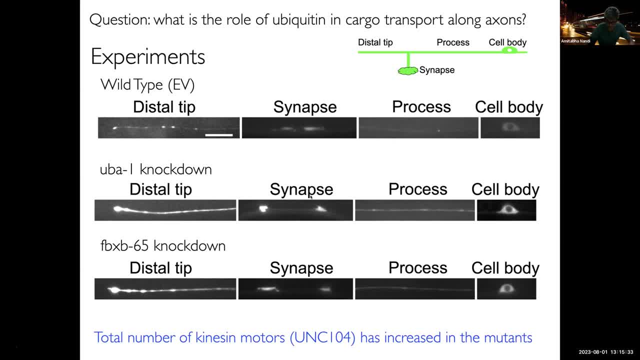 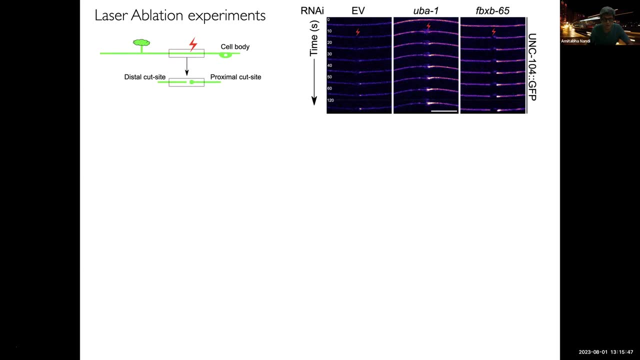 there is an accumulation post ablation, Whereas on the other side you don't see any increase, which is expected because these motors are sources in the cell body And because this is cut, they cannot go to the other side and they get accumulated here. 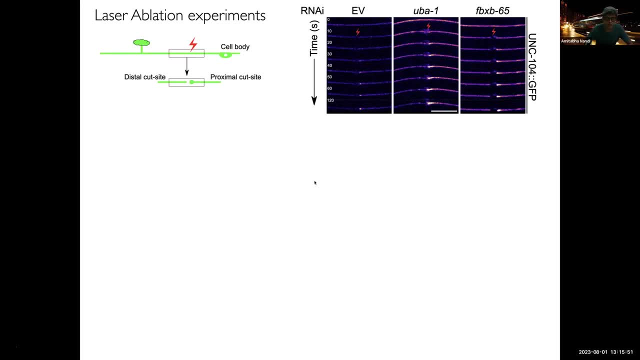 OK, While on the other side they actually, ideally they should drop. But here what you see is they are roughly constant, And one should take this distribution with a pinch of salt, because this intensity level, this normalized intensity level, is almost comparable. 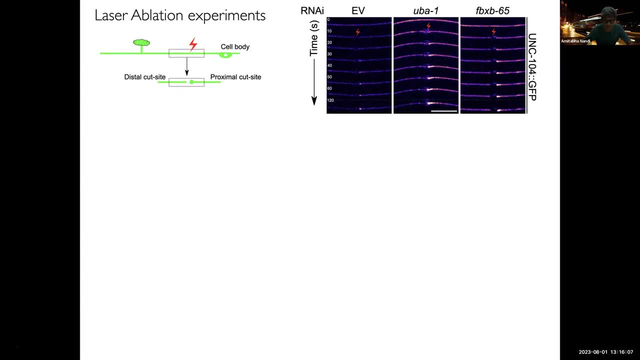 to the background noise intensity. So this is not very reliable. But on the other case you clearly see an increase. So one can do all these statistics, But the important statistics is what Is known as a kymograph, And I will very quickly tell you what is this. 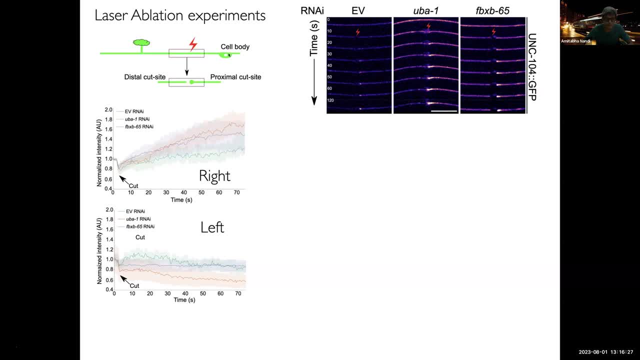 So this is the wild type, This is the mutants, the ubiquitin mutant and the FBXB. So the y-axis is the time axis, The x-axis is the position axis, So one should only focus on these lines which are diagonal. 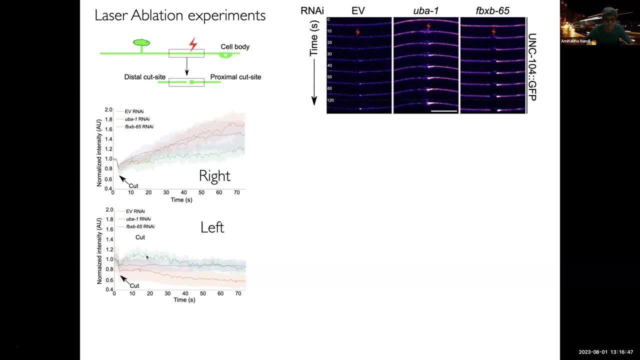 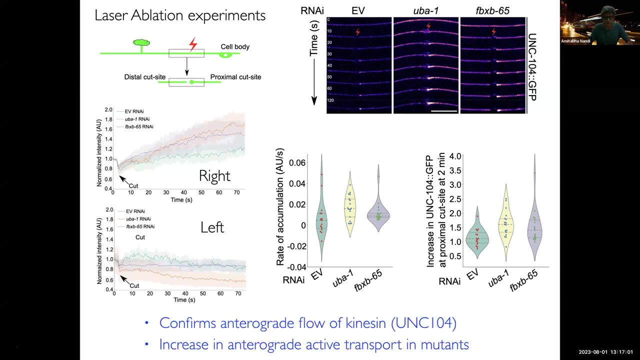 or well, not diagonal, which has a slope non-zero, which are not constant, Which are not vertical or horizontal, Because any line which has a non-zero slope, they indicate cargos driven along the microtubules by the motor proteins with constant speed. 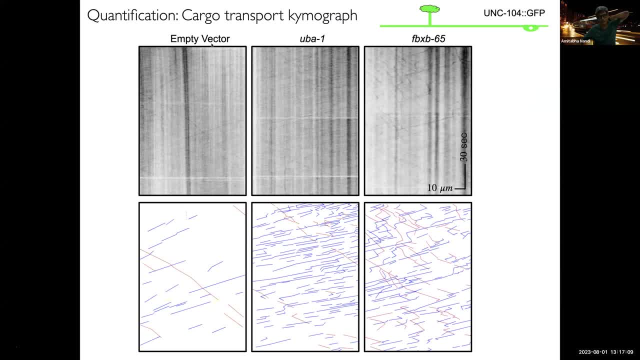 So if I try to find those diagonal lines, these are these blue lines And you see, if I compute the number of, if you compare the number of lines, the number of lines has increased As we go from the wild type to the UBA1 or the FBXB. 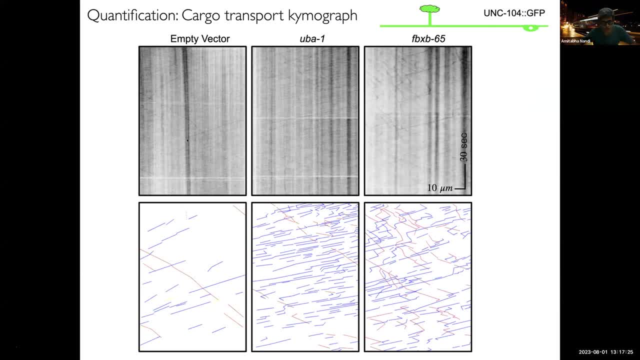 which tells you that now there are more cargos or more motors binding the cargo and the microdubule. That number has increased from the wild type to the mutant. And if I further plot a distribution of these motors attached to the cargo, this is the steady state. 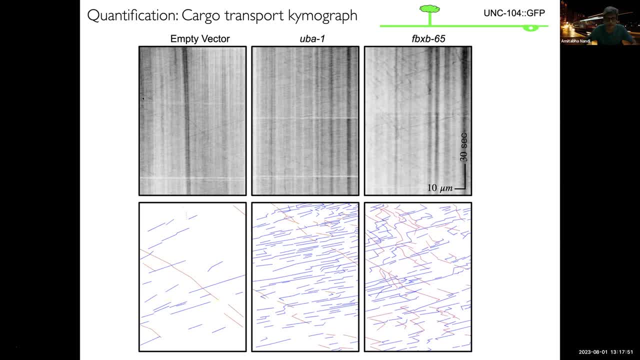 Distribution of the motors attached to the cargo for the wild type, And this is for the UBA1 and the FBXB, And clearly you see they are plotting on the same normalized scale. You see that, as I am going from the wild type to the mutant, 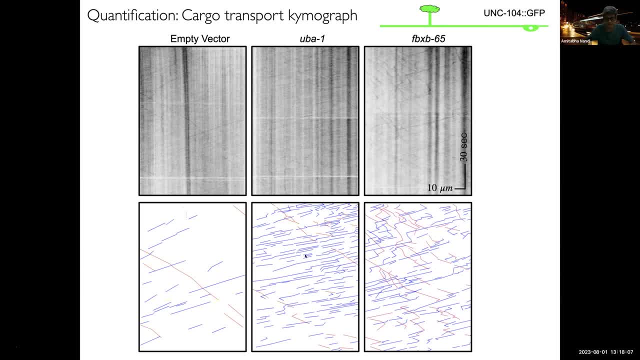 the distribution is getting broader And the mean is also shifting. So it is an indication that the number of motors that are binding to the cargo is increasing with ubiquity. So now I can try to ask a question. So I have this observation that these are: 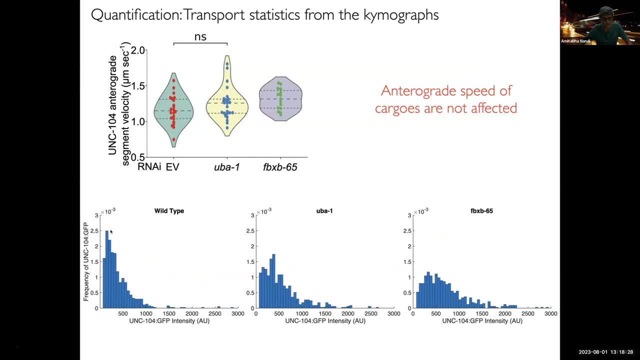 the steady state distribution. Now I can ask a question that: can I construct a model which will at least give me some insight about what is happening? So can I take two or three more minutes? Yeah, sure, sir. OK, And that is what we are going to do. 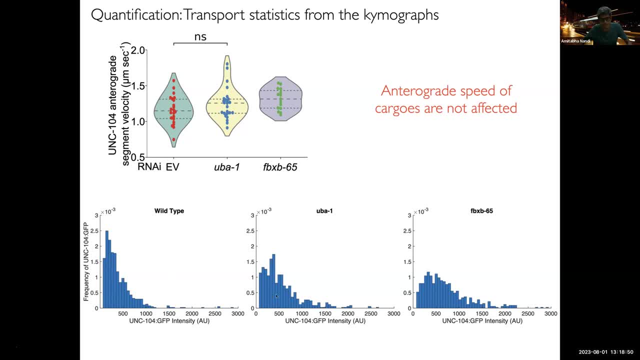 So what we will do is we will look at the time evolution equation and we will write down something called a master equation. So I thought I will explain master equation but I won't have time. But the master equation is basically: you write down the time evolution equation for the probability. 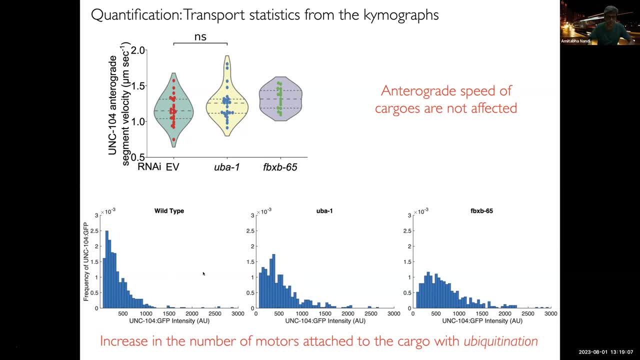 of some configuration, of some observable, with a configuration n, And you ask the question that how it came like, what is the probability of inward transition, where it came and the probability of the configuration in prime was p and prime t and any loss term, which is the second term. 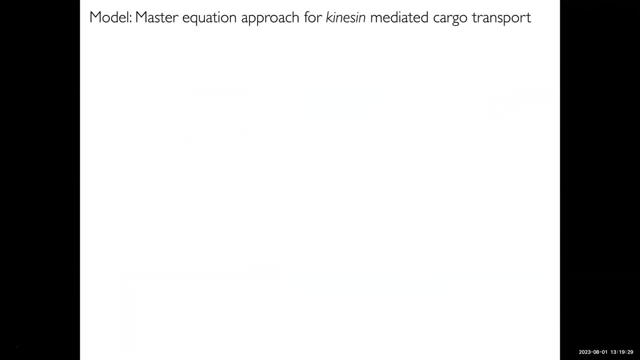 And this is a very standard equation, and one can derive it systematically using these ideas of stochastic processes for time, evolution, evolutionary probabilities, And I will skip this example Now. using this methodology or formalism, what we are going to do is we are 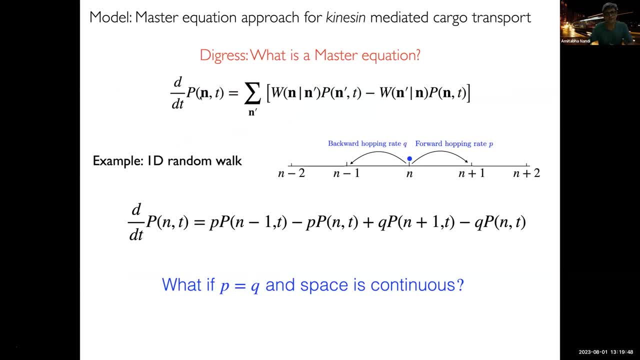 going to write down an equation- master equation for the probability that there are n motors bound to a cargo in between cargo and micro, And using the master equation formalism, I can actually write down that time evolution probability And this time evolution of this probability. 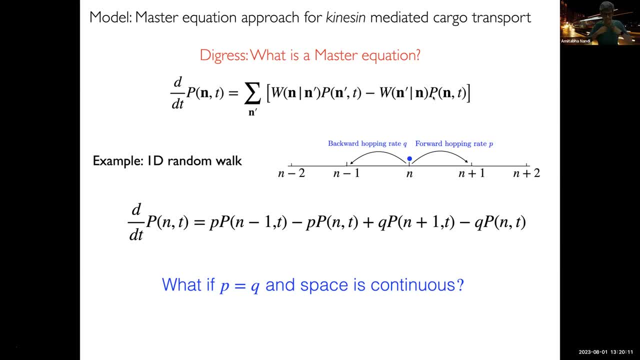 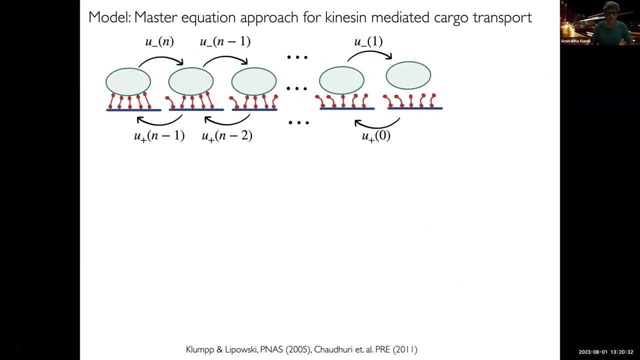 depends on basically a gain term where a motor has attached to the cargo, which is the first term, And basically there were more motors and one motor has detached and reached that number n And this minus is basically the loss term from that state. 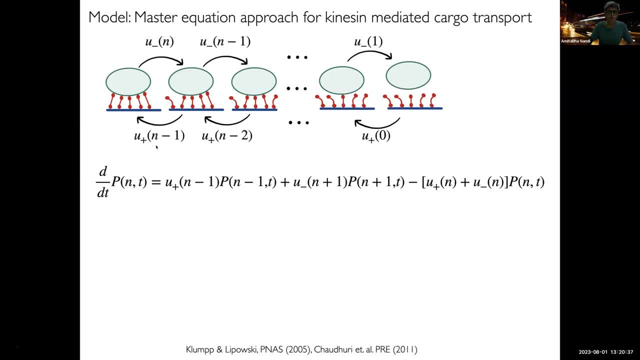 And so this is using very general formalism And these are basically the binding rates. These u plus and u minus are the binding rates And for this problem I will have the boundary conditions. And this is the boundary conditions And for this problem I will have the boundary conditions. 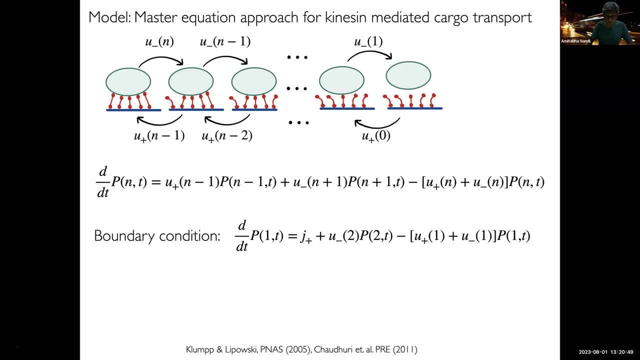 And for this problem I will have the boundary conditions And with all this I can calculate the probability distribution at the steady state, which means the probability is not varying with time, which gives me this recurrence relation which is within the blue box. 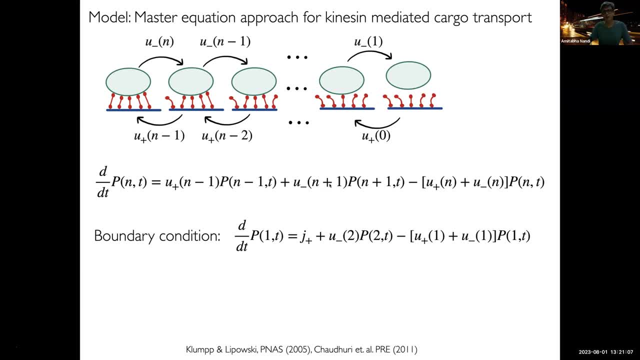 So now the question is here: I still need to know the binding and the unbinding rates, And here I will make a hypothesis, And that is the most important part: that we say that the unbinding rate is unbinding of a motor happens with some rate beta. 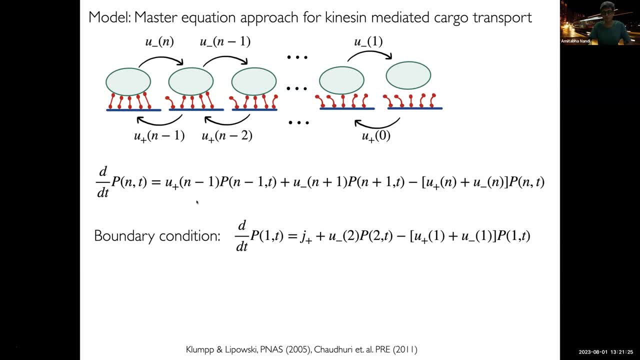 So if there are n motors attached, depending on that number n, it detaches with some rate beta. However, the binding rate is given with this like equations. So if there are no motors attached, a motor can attach to the cargo with some rate A plus. 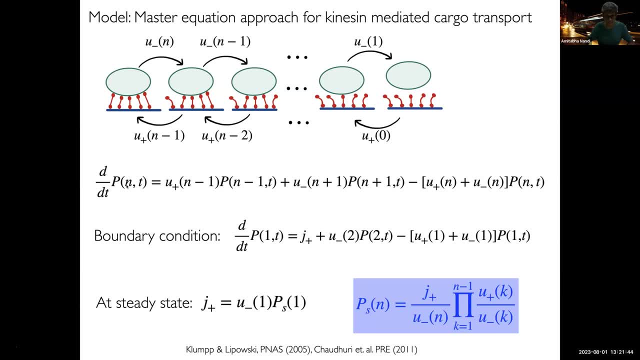 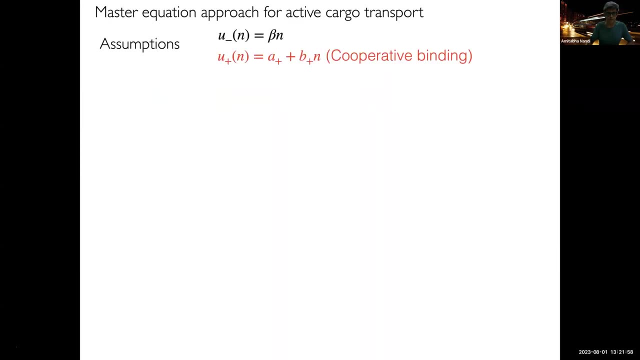 However, I can have a cooperative binding which means that if one motor is already unbinding, already attached, that will increase the chances of another motor attaching. If there are two motors attached, the chances of a third motor attaching is even higher And that is captured. 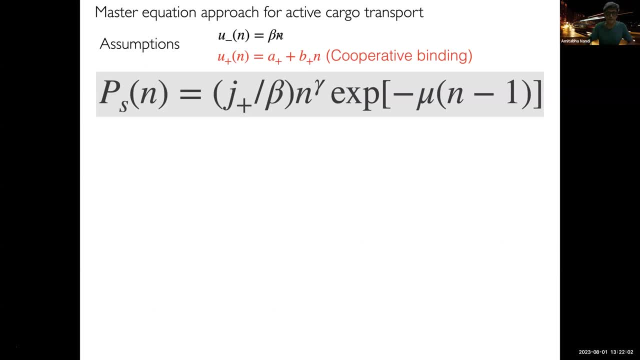 by the second term, And this second term is a hypothesis which we put in the model, And with this hypothesis we can get an analytic expression for the probability distribution at steady state which has this form, exponential form, And what we find is it gives a very nice agreement. 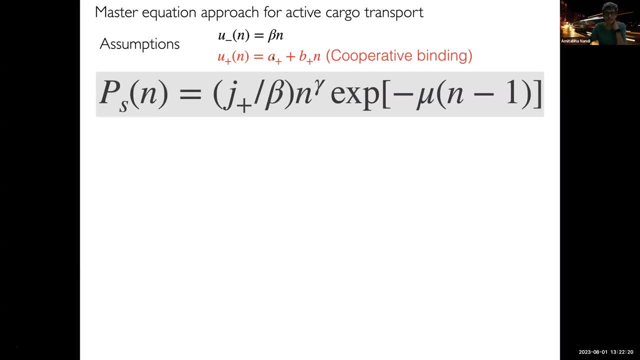 with the single model for all these different cases where these red lines are from the model And what we have, prediction or a hypothesis, that only if we have cooperative binding we can explain this change in the distribution Otherwise. so you can see. So if the B plus was, 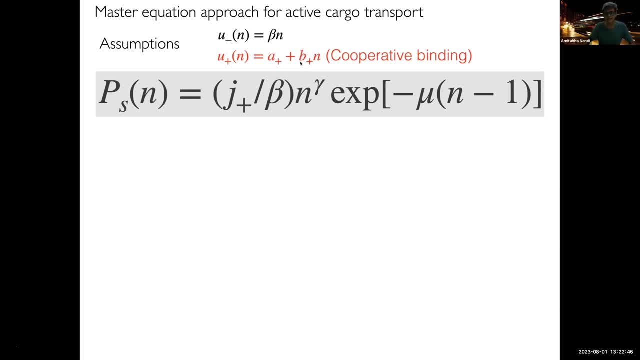 zero, this mu will be one And all the exponentials will be of the same, will have the same decay with number And you cannot capture the variability and the thickness. So the second term, this B plus N, is very important. So this is a hypothesis. 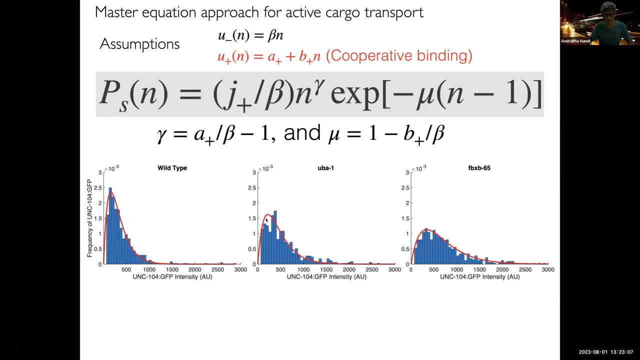 from the model. Now one can go ahead and ask questions that I will skip all this. that. what is the? what is the like? what is the molecular mechanism of such cooperative binding, How it is controlled at a very microscopic scale? And one biological function is very clear that you, in the wild type, you have less. 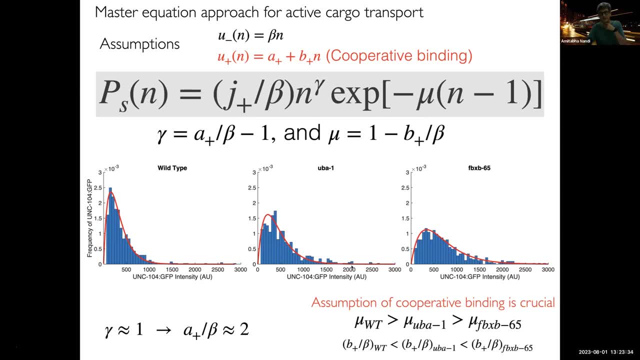 ubiquitination: more, less, motors are binding, And it makes sense because this ubiquitination regulates cooperative binding And you don't want many motors to bind in a cargo and get depleted from the cell body. So so what we see is this ubiquitination or this method of ubiquitination has like a nice way to regulate. 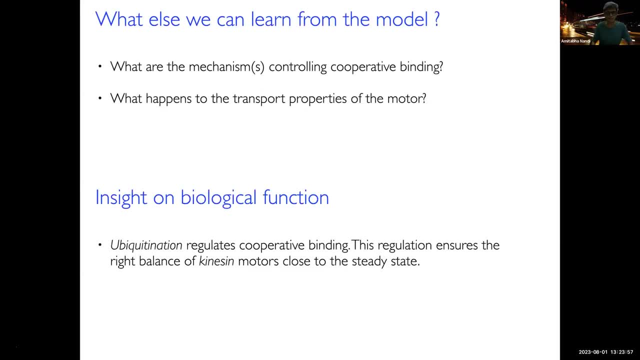 the motor distribution along the axonal length. So I will stop here And let me thank the collaborators. So the first work was- like: this is a continuation of work which I did as a postdoc long back, And then we continued with our PhD student, Imrani, and my collaborator, my colleague 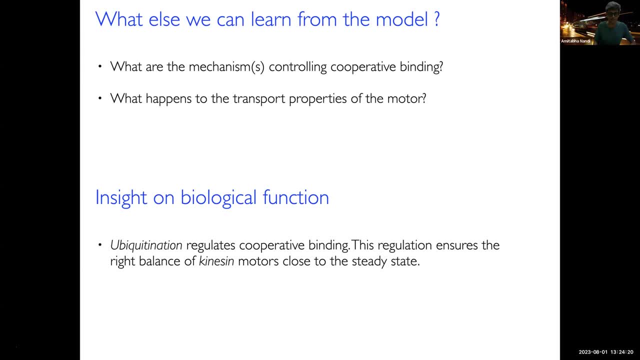 at IIT Bombay. And the second work is an ongoing work with experimentalists from TIFR, from Sandhya's group, Vidur and Sandhya, and my theoretical collaborators Devashish and Amir. And the first part, the work done during postdoc, was like the experiments are done in the lab of 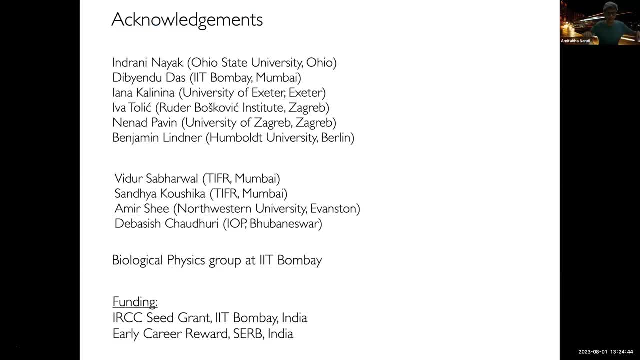 and Nina, then Benjamin were working on the theory part. So, yeah, thank you for your attention. So, yeah, please let me know if you have any further questions. I can already see somebody I know. Hello, Professor Bhattacharya, how are you? 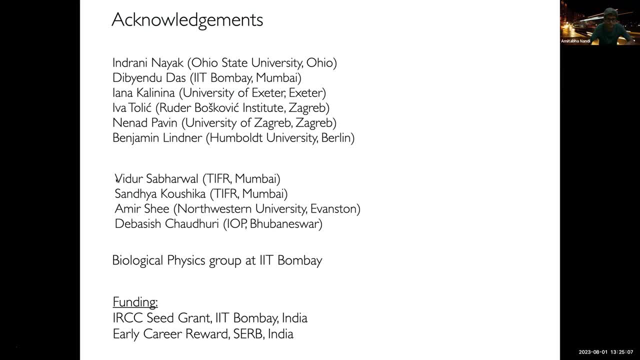 I'm fine. Very good, Amitabh, And thank you for coming and giving this talk. No, thank you for the invite, Because we are going to make it a yearly affair. We will do the major event in this area, So hopefully time will be on campus. 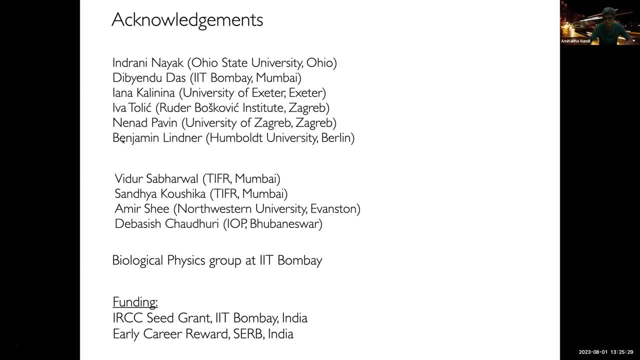 And Professor Amitabh, are you traveling? So especially appreciate you Right now. no, no, no, I'm not traveling, I'm back to the campus, So next time, hopefully we'll have it physically, Okay, great, Great. 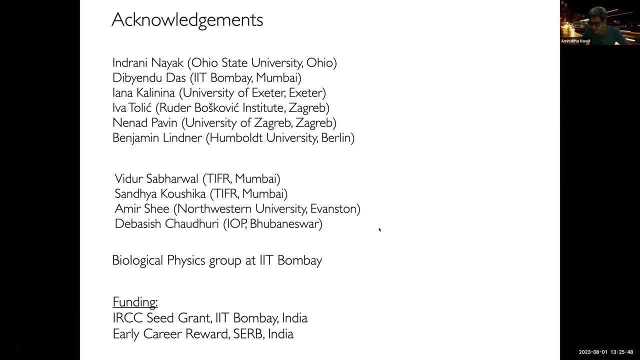 I'll be very happy to like. I have never visited. Oh sure, So sorry. I think I have taken like a lot of time. No, no, no, it's fine, That's perfectly all right. 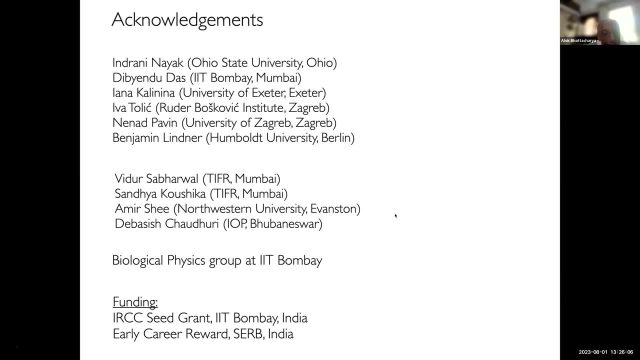 Are there any more questions? So let's take a moment to thank Professor Amitabh for an excellent talk And hopefully, as Professor Alok said, we'll get to see you at the next edition on campus at Ashoka, And look forward to that. 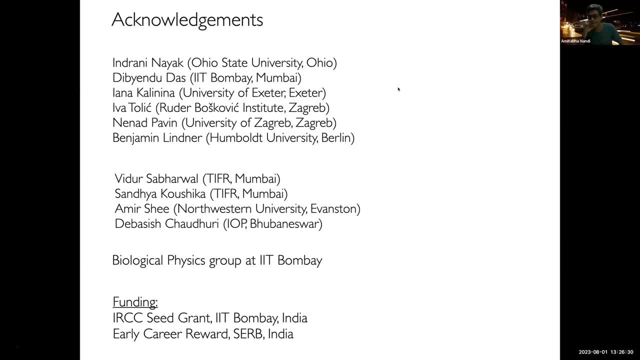 Thank you for the invitation And yeah, so yeah, I look forward to next year. Great, Thank you. And so, Professor Bhattacharya, I will be in touch with you, So I will talk to you. Yeah, yeah, we should talk. 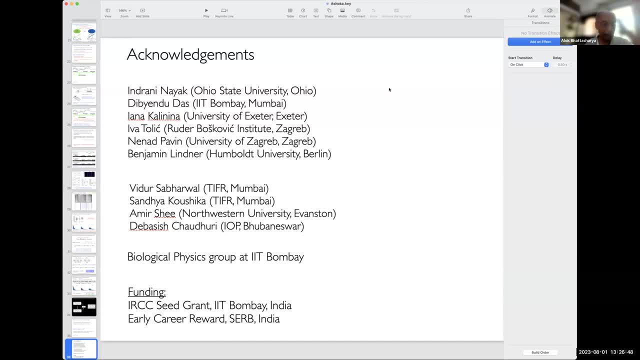 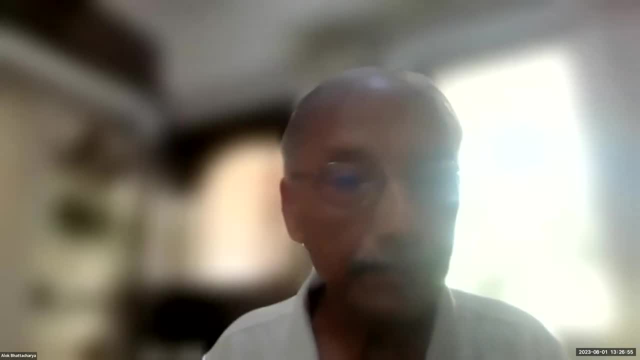 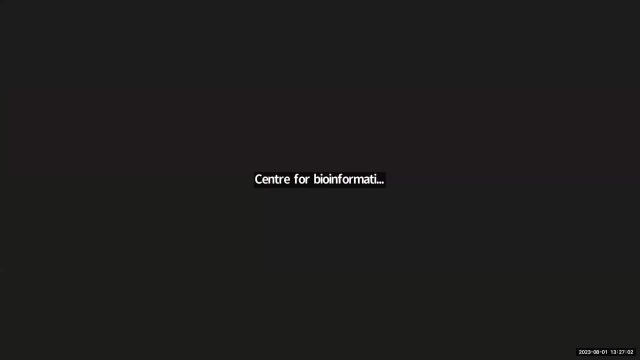 Yeah, yeah, yeah For others, Amitabh and we did some work together long back. Yes, yes, Exactly, He was a student. One of my earlier biology works was with Professor Bhattacharya, One of the first forays into biology that you did. 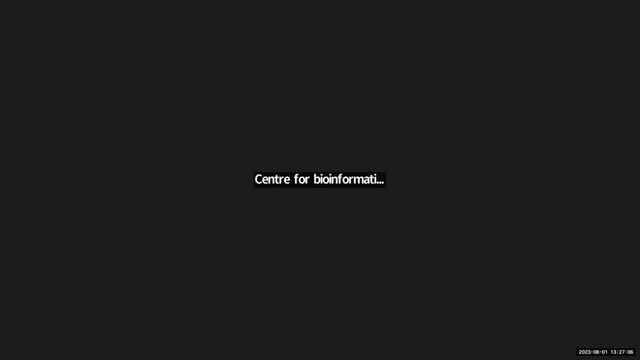 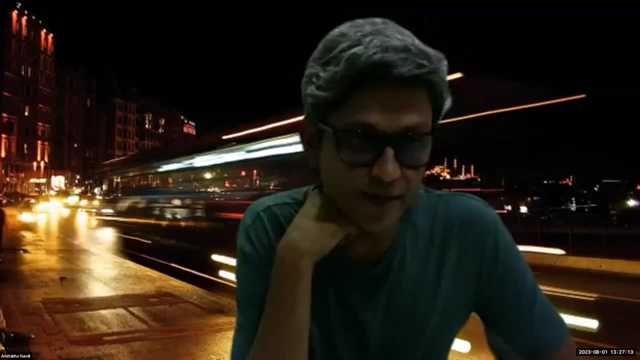 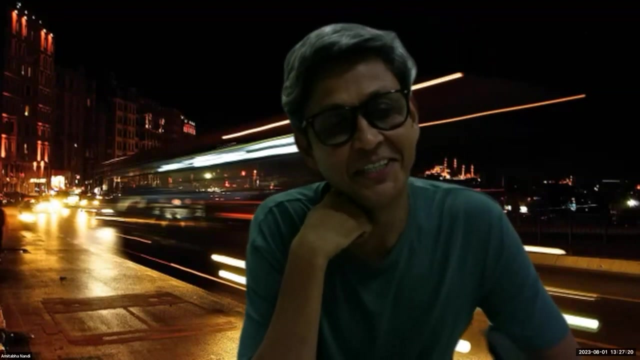 Yeah, yeah, exactly on microRNA regulation. Yeah, yeah, Good, good to see you, Yeah, great to see you. So, yeah, so I guess you will have like a break or next session, So should I just log out or? 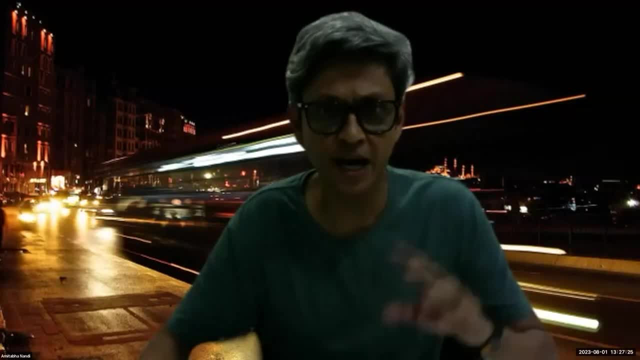 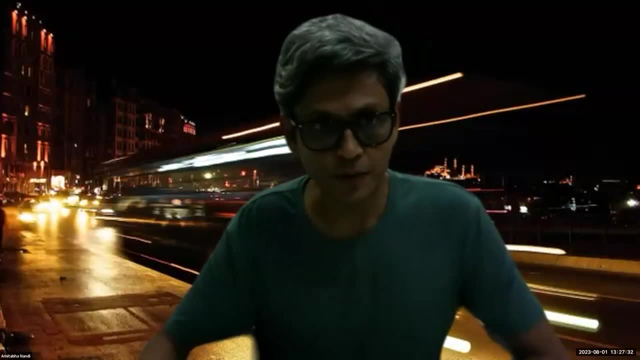 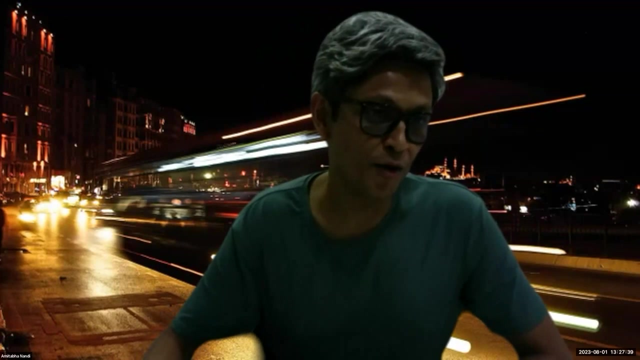 Yeah, yeah, I think log out, Okay. okay, Thank you very much. We'll share the recording with you, sir. And yeah, and participants. the next session will begin at around 1.55.. So maybe tune five minutes before. 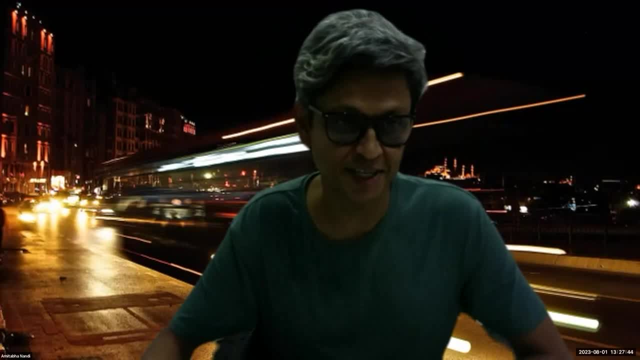 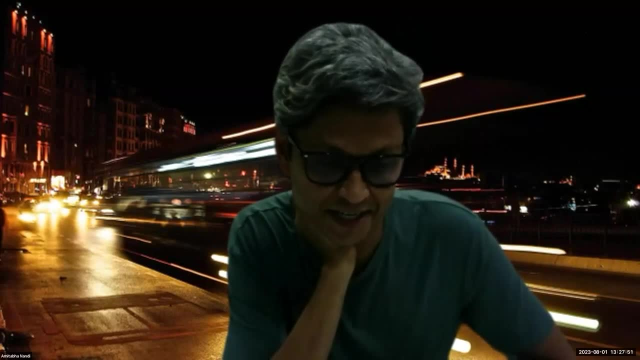 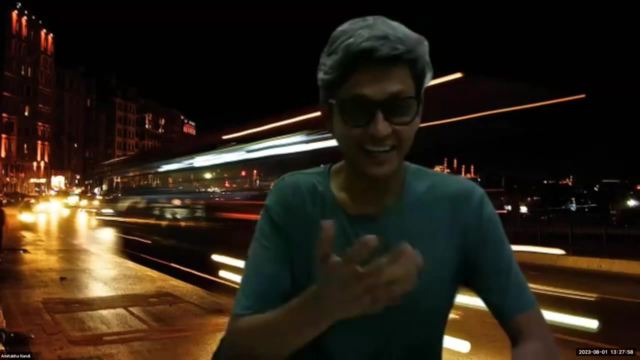 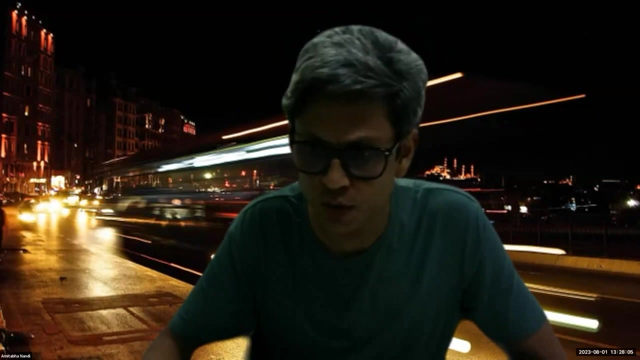 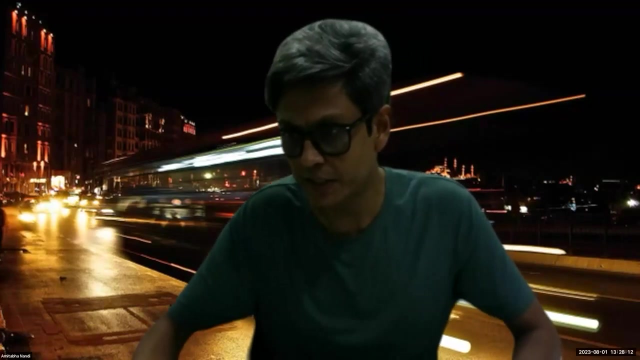 And talk is by Dr Suman Basad of NII National Institute of Immunology. So let's take a quick lunch break and see you at 1.50, 1.55.. Thank you, Yeah, yeah, I can probably see the participant. 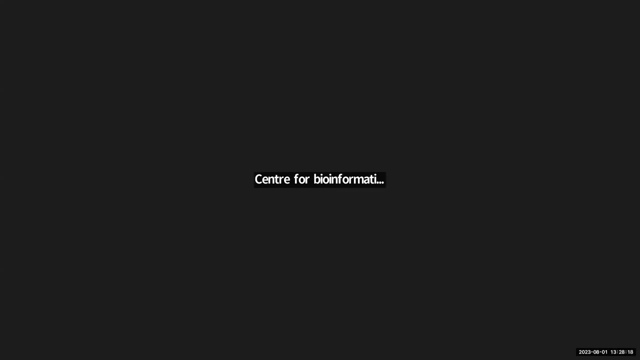 Just let me check the format. I think it should be fine now. Yeah, I think it looks to me. I'm fine now, I guess. Yes, that also. Yes, that's the only thing that I need to change, I believe. 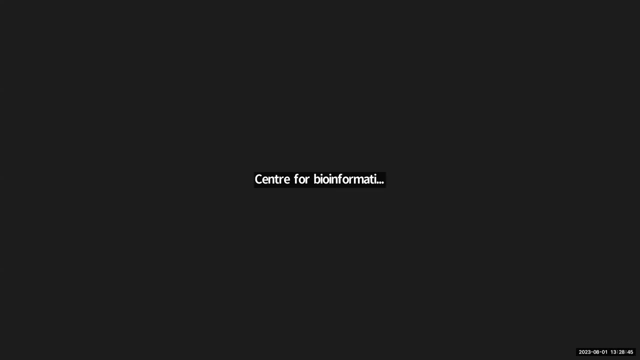 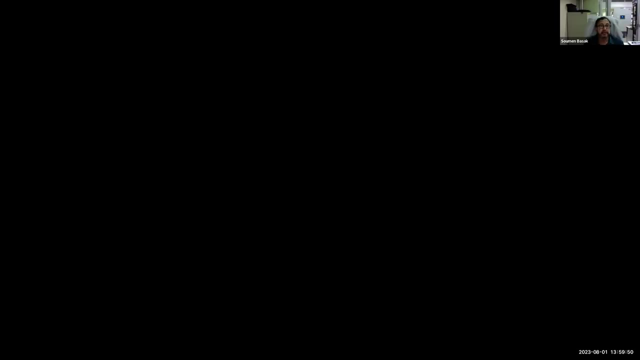 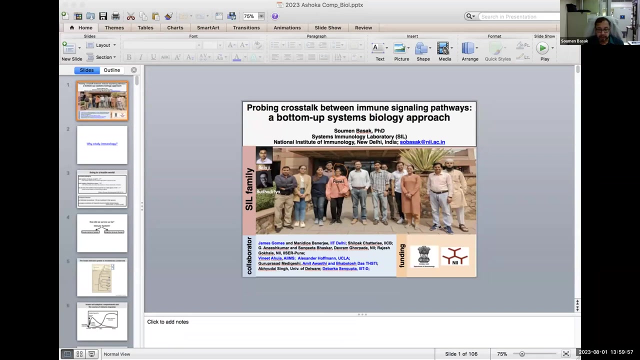 Yeah, let's give it a couple of minutes for people to come back from lunch And then I'll introduce you and we'll get started. Sure, sure, No issues, And I believe I just have a quick question. I know last time also asked. I believe these students are mostly undergraduates. 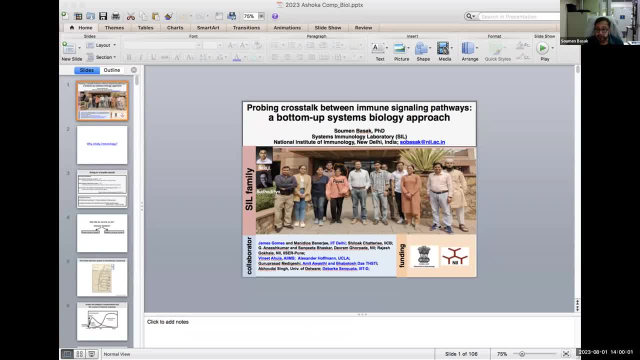 Am I correct, Sir? it's a mix. There are some PhD and master's students. also There are a couple of people who are professors and practicing, you know, like somebody from the Dairy Institute, somebody like we have a mix. But yeah, it would be fair to say that there's a mix of mostly students. 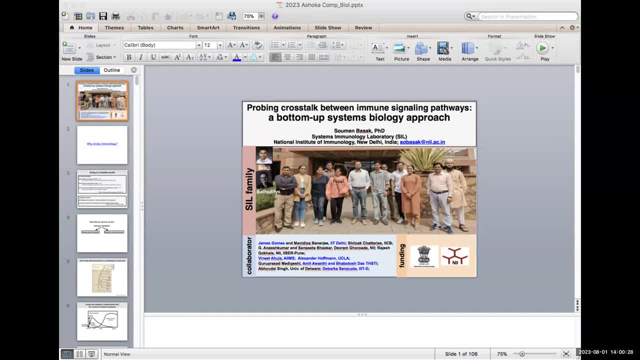 but a mix between undergrads, master's and PhD, And we have some faculty from Ashok And other places as well. Yeah, I see all of that is here. Bittu has also joined. Yeah, yeah, Hi, Bittu. 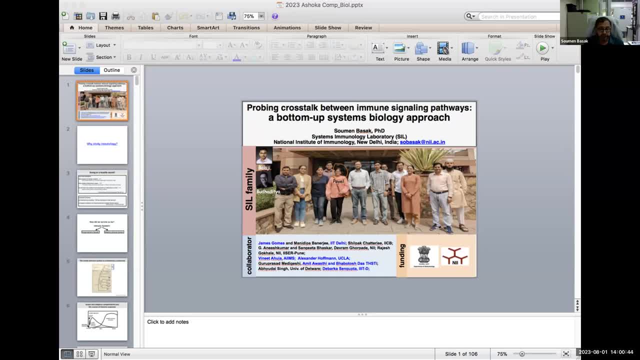 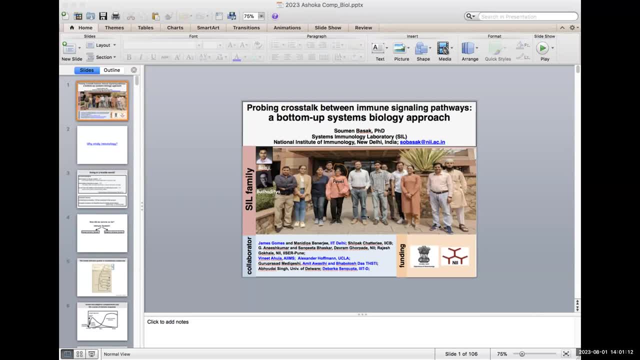 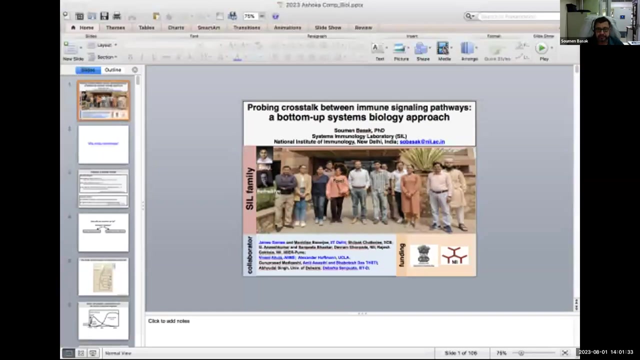 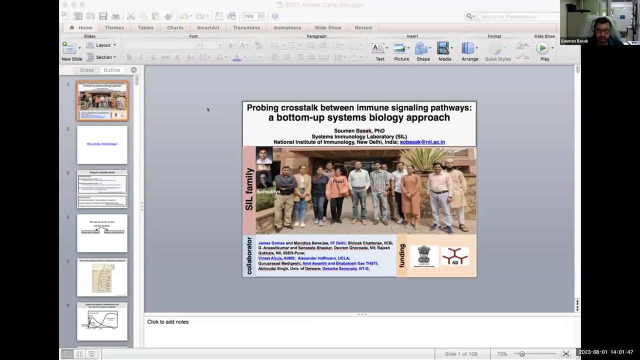 I appreciate it. Thank you, Yeah, of course. How about the last thing you mentioned, the first question we can ask you: what are the most advocated goals for undergraduate and graduate sex? you so, um, i think let's begin um. welcome back everyone from lunch. 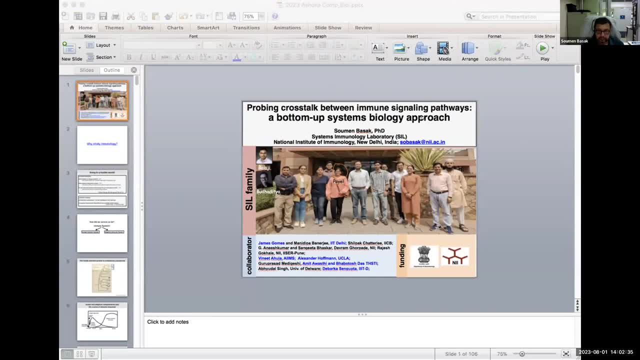 uh, we are excited to have dr somain basak from national institute of immunology, delhi. so dr basak obtained his phd degree from the university of calcutta. subsequently, he carried out his post-doctoral research at ucst university of california, san diego. in 2010, he joined nii. 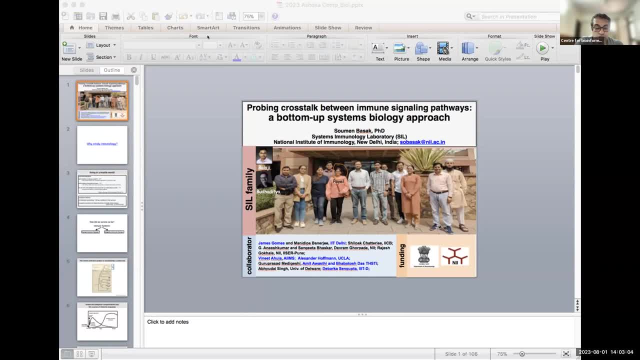 national institute of immunology and set up the systems immunology lab. since then, his research group has been combining bottom-up and top-down systems biology tools to address how information is controlled in physiology and what causes dysregulated, deregulated information in human ailments. his talk today is titled probing dynamical crosstalk between immune signaling pathways. 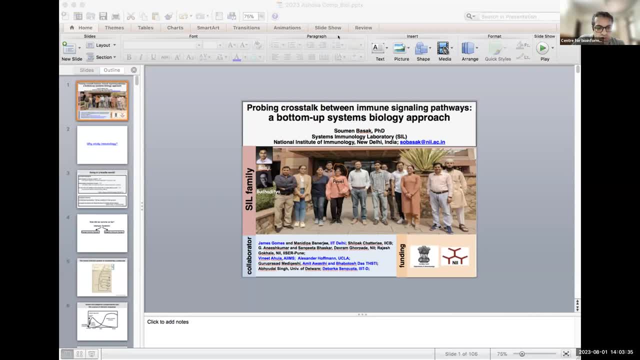 using mathematical tools. welcome, dr basak, and please take it away. a quick question. uh, would you like questions as you give the talk or all of them at the end? i'm finding both, i guess i am. honestly, i have no reservation. if you ask questions in the middle, it might make it more. 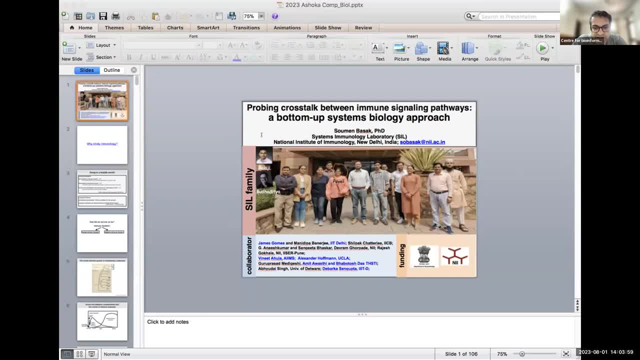 interactive. it can be very useful because if you move along in the presentation with some confusion, sometime it becomes all right. so i'm fine. so so we can uh participants feel free to ask questions. either tap uh, raise your uh, raise the hand in the zoom reactions, or uh just uh unmute and ask for. 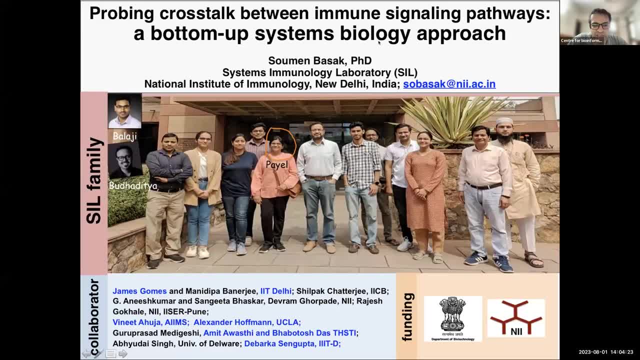 okay, please take it away, sir, okay, okay. so i think, first of all, uh, thank you assist and uh, uh, we have to really admit this wonderful uh program that you guys have set up in ashoka and um, with all of them, both of them, of course, a lot of critics. uh, this is indeed in a very important uh initiative in the ncr region. 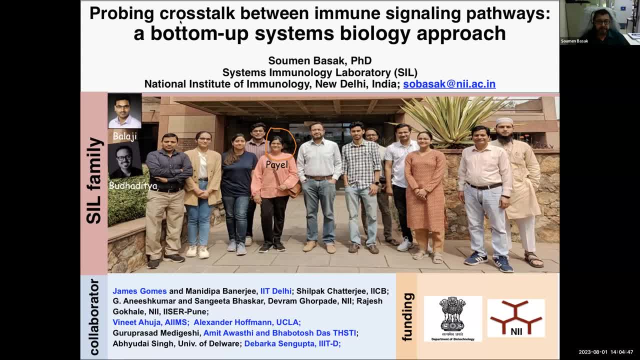 i'm sure that it's already practicing and it will uh go to a level which it uh where it can actually uh feed back into the important research program that ncl carries out. and this is my laboratory, this is the laboratory that i have- systems immunology laboratory- and just a minute i think i could just do actually do. can you see my 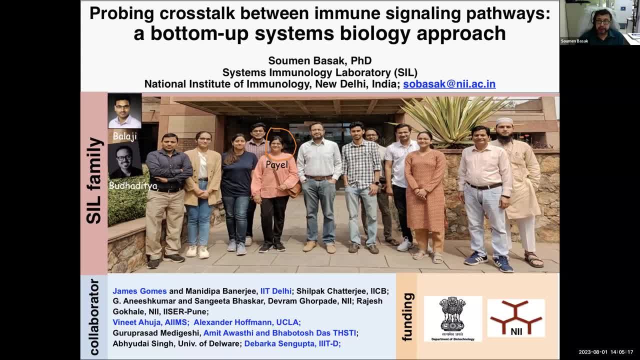 just a minute. i think i have to go back to the paint color. yeah, do you see my cursor? hello, can you answer me, please? do you see my? yes, sir, we see the. we see the cursor, but not in red. are you trying to make it red? i can make it ready. i think it is supposed to be in the idea, i think. 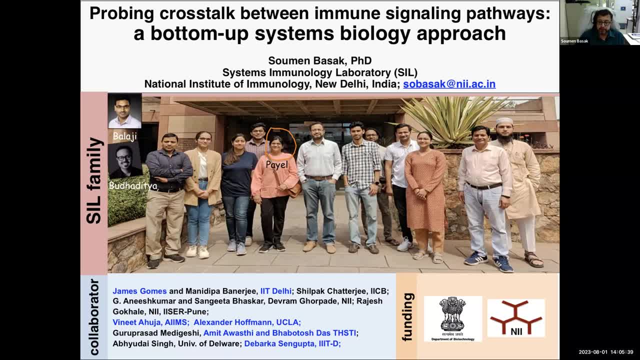 it will look right now. oh no, this is yeah. okay, it will not be. i think this is fine. uh, let's keep it this way. right, you can see the cursor right. so, um, yes, sir, this is a laboratory, the system symbology laboratory. today i'll be talking about probing crosstalk video and i'm going to show you. 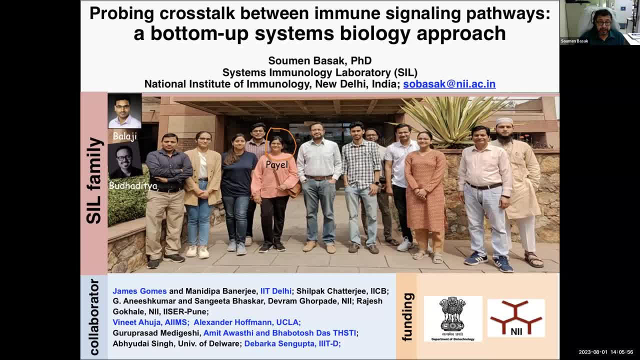 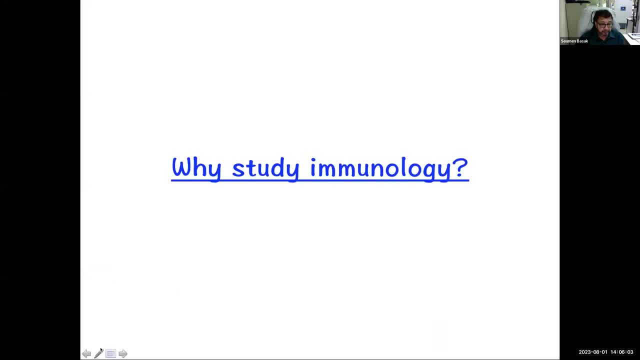 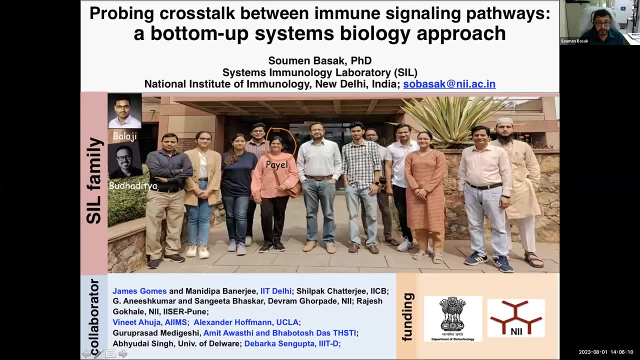 an immune pathways, the bottom of system biology approach. uh, the work that will be describing some of it has been done a long time back and some of these are still continuing in some form and format and, uh, we have a- you know, huge number of different collaborators. of course, this kind of 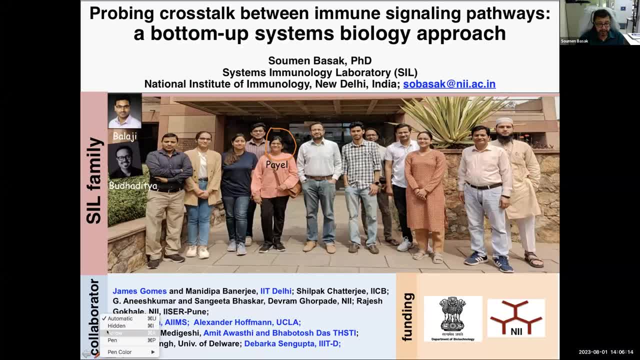 initiatives require involvement of multiple set of peoples. uh, particularly the discussion today. uh, we will uh have, uh, we'll have. i mean professor james chrome's from mighty delhi. he may have. uh, he has collaborated with us in a variety of different program, that where we have. 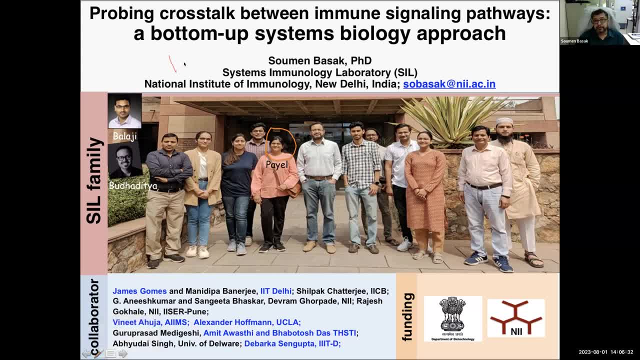 combined competitions and experimental studies and students. balaji was my first phd student on this left. he has left the lab long time back, but i think you still are discussing the work that he has done with udarito. he was a guy who i hired in collaboration with iit as a phd student. he did most. 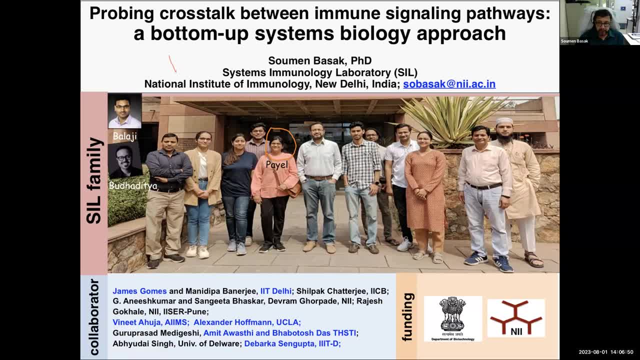 of the competition. biology work and file also has contributed in those earlier days- formative years, experimental analysis, and then of course a lot of students began to contribute, particularly alvin and navik. they are currently with the lab and doing a lot of wonderful work, but today i think we will. 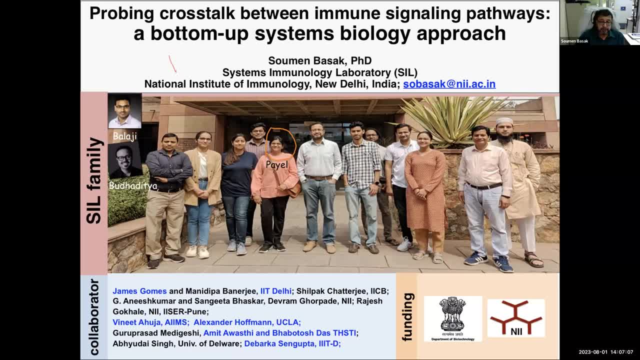 probably discuss immunology and system biology. so maybe you know more of a systems immunology. so we will try to uh sort of focus on those: how computational, what competition tools we can, what one can use and how they might have been useful. before you go into that, 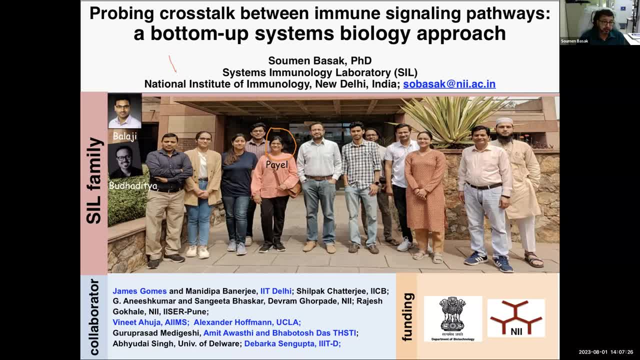 first, i think, because there are a lot of undergraduate students, or some of them are at least- maybe we should start with some very basic questions: why studying nobody? and this is a couple of things. after a little investigation one might find microbial pathogens. you know a total number. 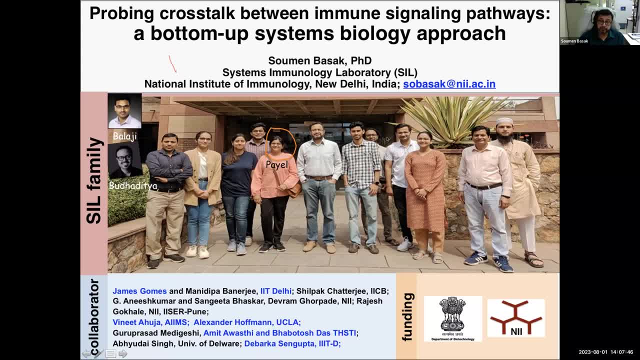 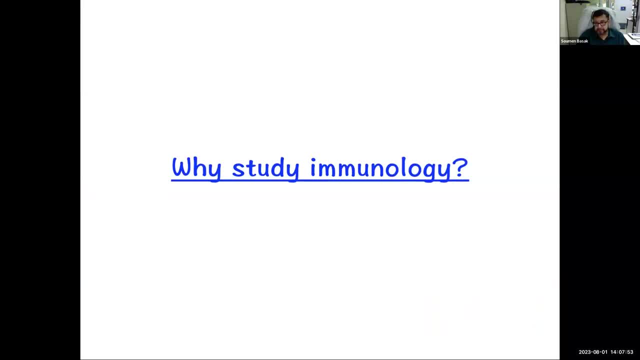 of viruses in our. if you, if you put them next to each other, they would stretch for 100 million light years and total a number of bacteria in water. and they would stretch for 100 million light years and you would see that the ocean is 100 million times more than the number of stars we see in the 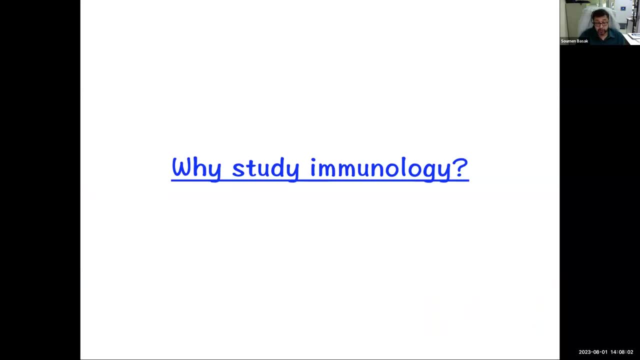 known universe. and if you take a spoonful of soil you'll be surprised. number of microorganism in that spoonful of soil would be almost equal to the number of human being living in the continent africa. so it seems that we're in the submerged in this, in a sea of microbial threats. 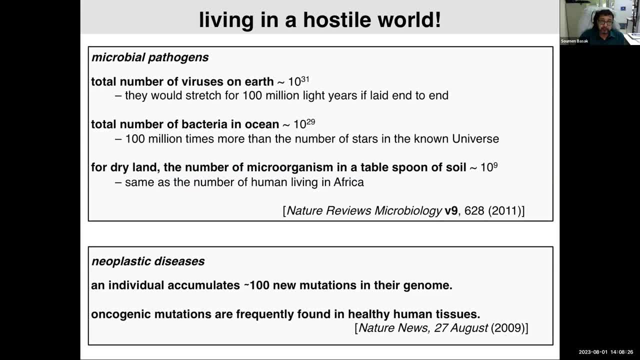 from within. we have issues too. an individual, the time we born and the time will die. between this, there will be around 100 new mutations in our genome each of us. will they be causing cancer? not necessarily, but here see the next information: that oncogenic mutations are far more prevalent. 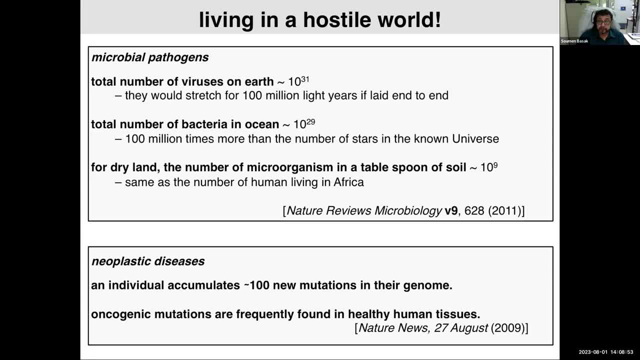 in healthy human tissues. your study was done to look into breast tissues. you see lot more frequency of pre-cancerous lesion in healthy individual population than the frequency of breast cancer in human population, suggesting that you do get developed pre-cancerous lesson every now and then but you do not necessarily develop cancer as 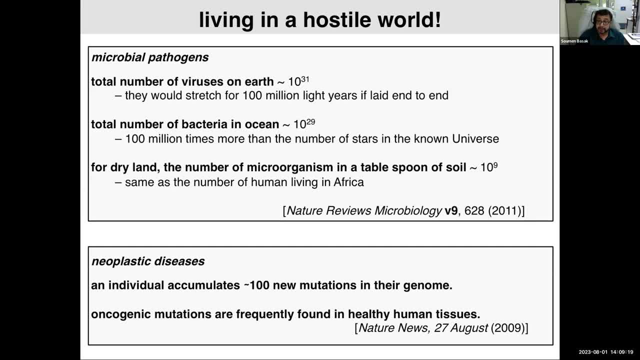 it the same thing. right when you have emerged in a submerged in a sea of uh microbes, you do not get infection every now and then you are, you know, acquiring mutations, but you even pre-cancerous mutations, but you don't necessarily get cancer all the time. and this is the answer: who is protecting? 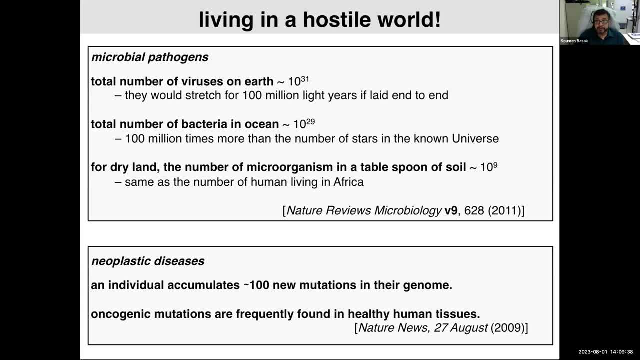 us from those external threats and those from within? the answer is even. the answer is immunology and of course kovid has made it very obvious why he wants to study immunology. but do not forget the internal threats also, that our immune system survey external threats like microbial infections. 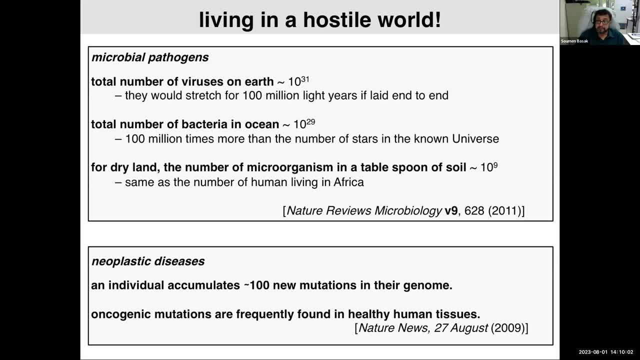 also look into malforming uh malfunctioning cells from within, and and plays an important role to limit them and eradicate them. that's why uh is we should study that's an interesting and the most important uh aspects of uh- our life. and if you see immune system, of course this is very rudimentary of innate and adaptive. 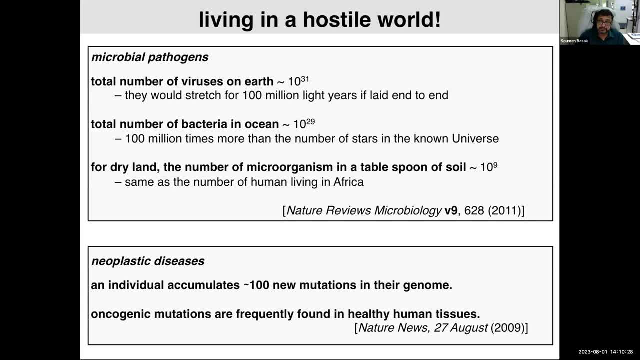 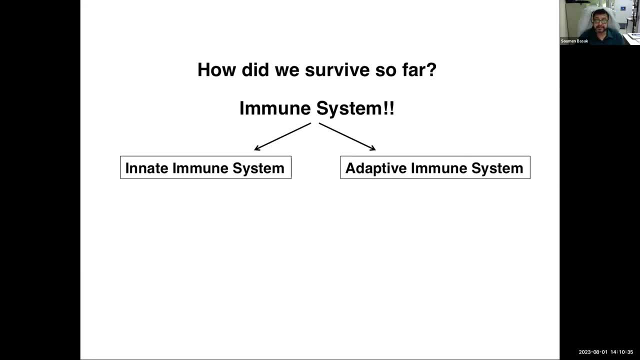 immune system. tell you what. if you look into the evolutionary tree, some of my uh uh- hope some of my colleagues here in asoka would be more interested- you will see the adaptive immune system came a lot later, uh, in early vertebrates, by the time you begin to lose your exoskeleton. some says 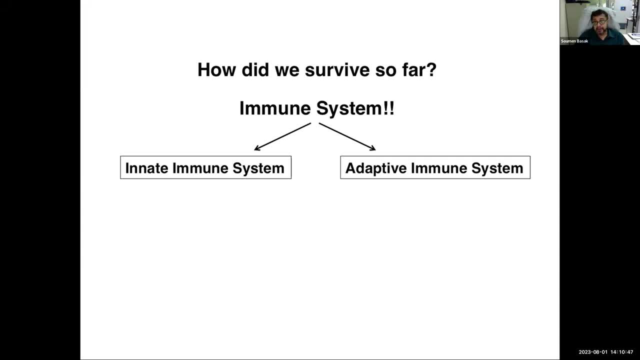 but if you do look into the evolutionary you see that innate immune system was there even uh in a few parts in animatrix evolutionary concept system and if you look into the uh scale of functioning, when you get a microbial infection here you have within minutes. you get of course 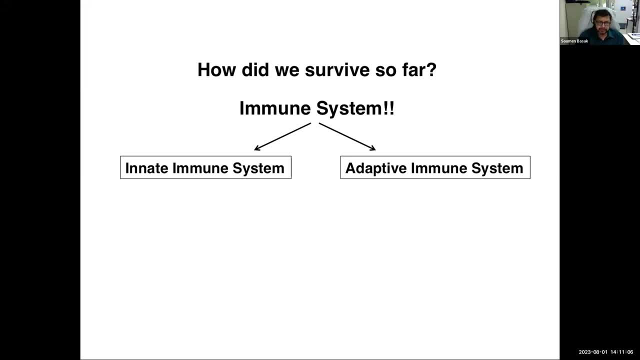 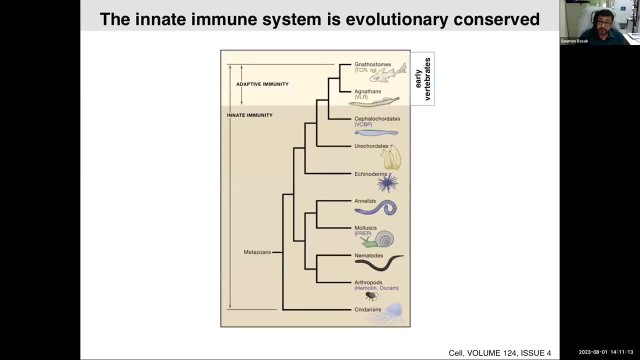 within minutes. the one you probably imagine is operating is your physical body. that's a part of innate immunity: right skin, for example, stomach ph, for example. you have heard all of this, but after that you get an inflammatory immune response- innate immune response, inflammatory immune response. that is the problem of the immune system and that is the problem of the immune system. 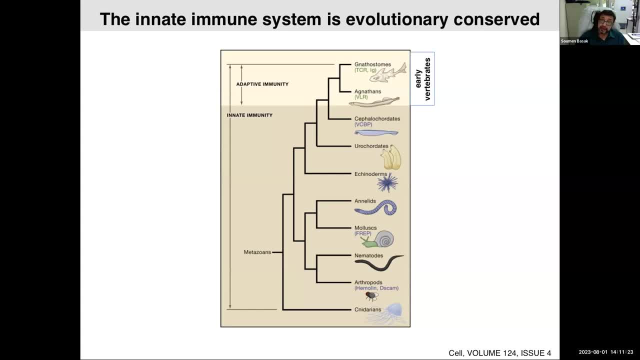 and that is the problem of the immune system. that involves macrophages, neutrophils, so on, and so that involves macrophages, neutrophils, so on, and so that involves macrophages, neutrophils, so on and so forth. you will come to that in a minute. 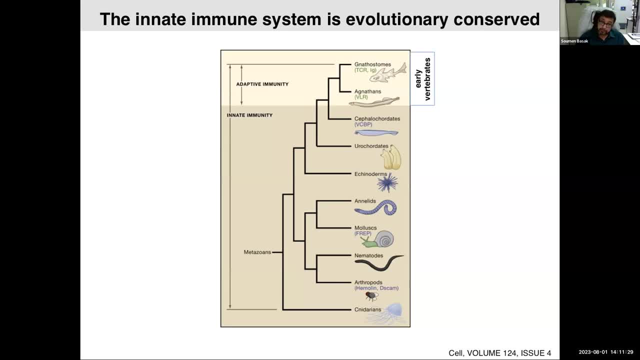 and then only you see, within hours to day scale adaptive immune system picks up and as an imaginary figure here i mean i do not have. this is not experimental data. one might really speculate what would happen if you do not have innate immune system, and it do not have. 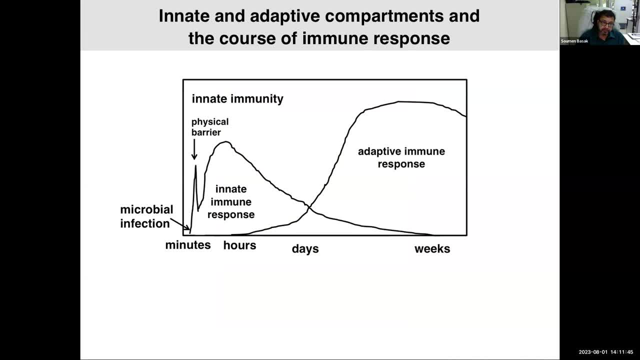 adaptive immune system. if you look into the number of microorganisms in y-axis and duration of infection in, the yellow line says what is the effect of the immune system on the immune system. what happens in normal human being infection? there will be accumulation of microorganism in 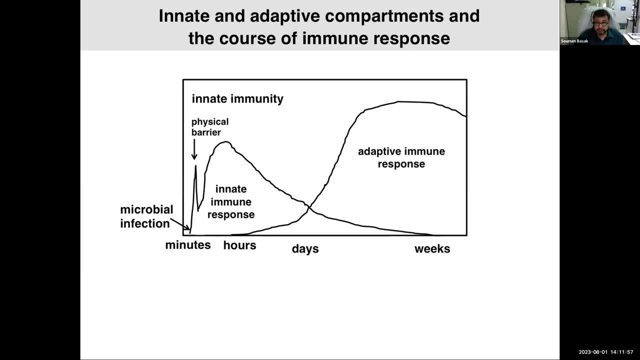 a given tissue or an anatomic nation, they will probably be eradicated and then you get a new line. if you lack adaptive immunity, we'll see that there is a green line where you know this eradication is not happening. but if you lack, in a diminutive soon after infection you will see. 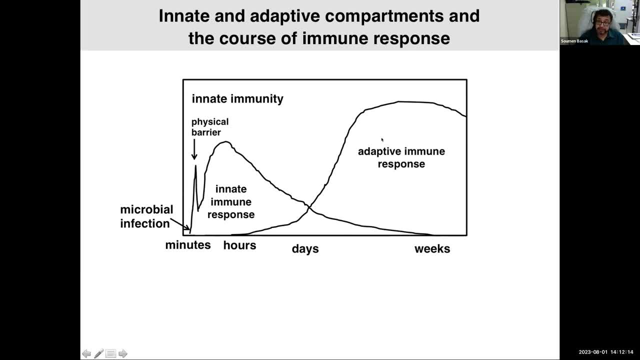 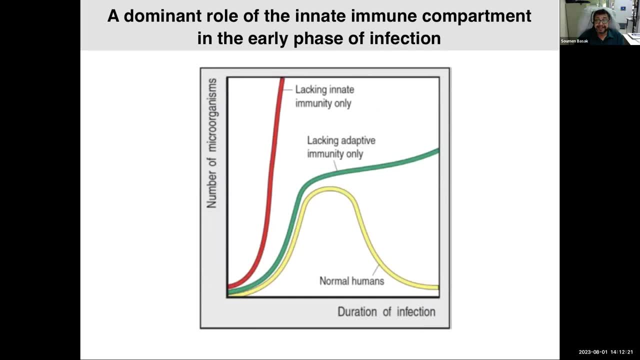 profound replication, profound uh multiplication of microbial pathogen could be one of innate immunity and inflammatory immune system threat and microbes will accumulate too quickly. so this is again innate immune system. you have inflammatory response. that plays a very important role in this innate immune systems and i'm going to really, really talk about those uh, inflammatory response. 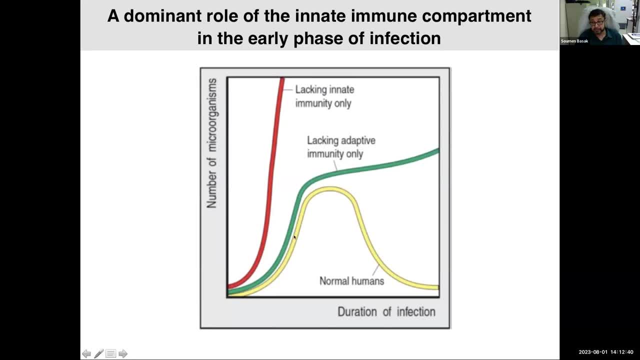 what are they? it's an, of course, form of unit immune response, and i'm going to try to pictorially present it. it would be important for us to later understand what we do and why computational methods were at times necessary, and of course one can uh orchestrate things much beyond the complexity that i'll be. 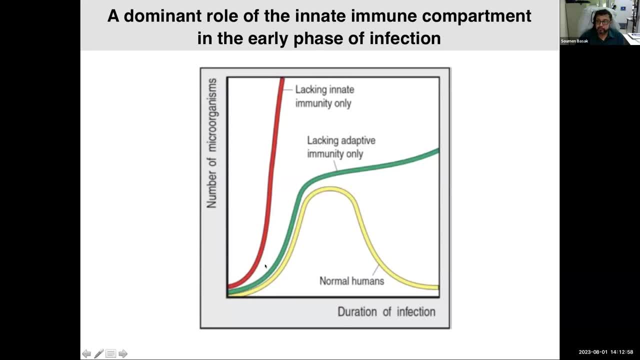 capturing here today. so when you have this tissue- resident cells, for example- it's a macrophage that is sitting in your underneath your skin, in the, in the, in the epidermis, in the, in the, in that layer, endothelial layer- when there is a pathogen, they will of course also cause a lot. 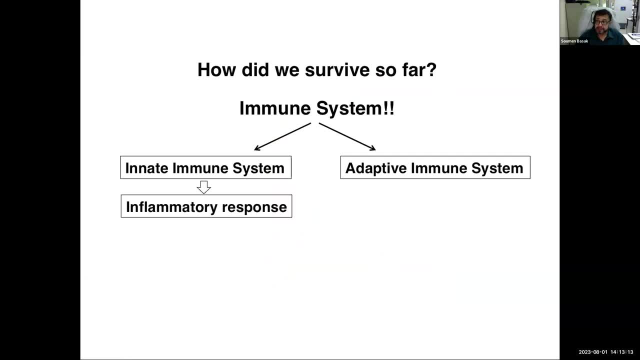 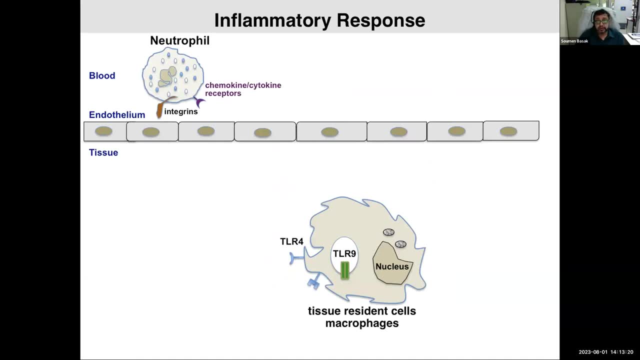 of cells to die. so microbial ligands and necrotic cells that will give you danger associated molecular patterns, where pathogens will give you pathogen associated molecules and they will signal to tlr's. there are receptors that would recognize these threats. this would lead to activation of intracellular pathways and that would transmit a signal in the nucleus provoking 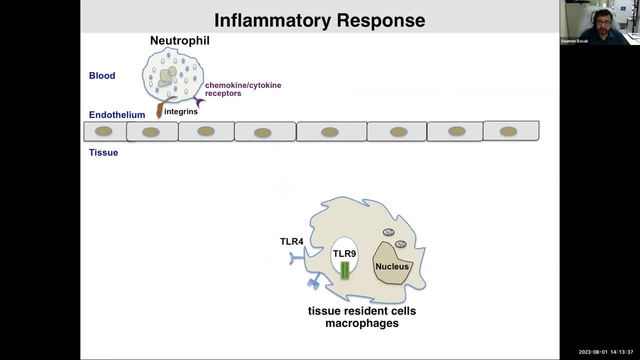 expression of genes, particularly chemokines and cytokines, neutrophils. these neutrophils are very important mediator of inflammatory response but they are normally in the bone marrow. they are only few neutrophils that would be in the circulation and they will patrol, they will. 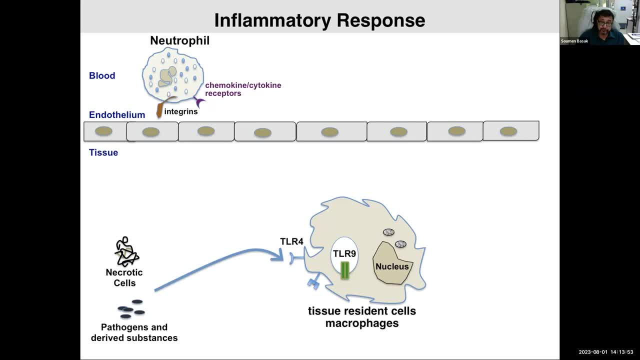 in the blood vessel. they will come in and they go by. but once this chemokine, cytokines are secreted, neutrophils will begin to adhere and then extra verses into the tissue where they will secrete a plethora of neutrophil molecules: saline proteases, myeloperoxidase. they are potent myeloperoxidase. 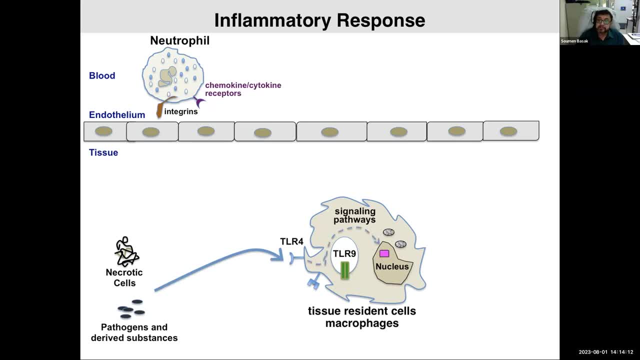 for example, is of course a mediator of reactive oxygen species. there are iron chelating protein that would deplete the tissue anatomic needs of iron, so microbes cannot replicate, and these are very potent neutrophils. they have these granules where they keep those potent molecules and they will heal in uh microbial killing and thereby, uh, you know, allow us a chance. 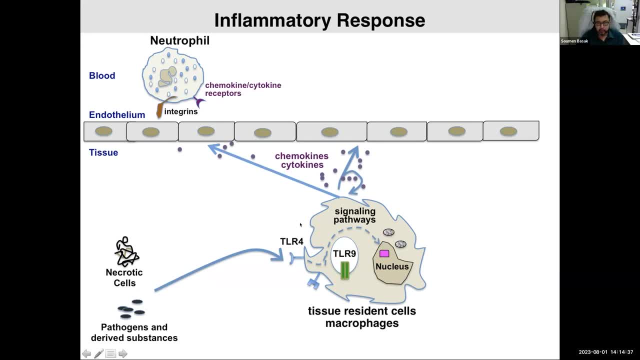 to then trigger adaptive immune response and then completely clean up the mess that may have been caused because of microbial infection. right, so so far, you have tissue resident cells. they must sense microbes and secretly chemokines, cytokine, to drag neutrophils and other potent detector cells at the site of infection. 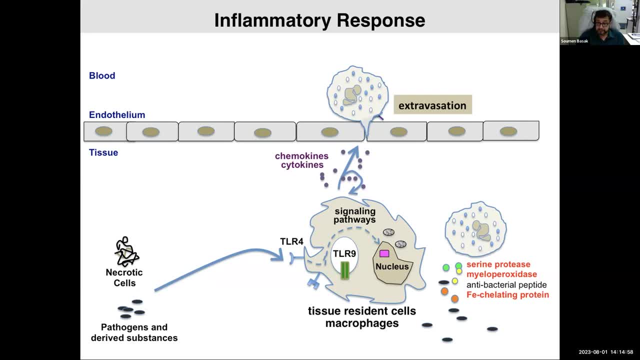 even macrophages. another thing those affected cells would do is phagocytosis. they actually- this is a very nice thing. hopefully it will come up to show you. neutrophils are white blood cells that hunt and kill bacteria. in this spread, a neutrophil is seen in the midst of red 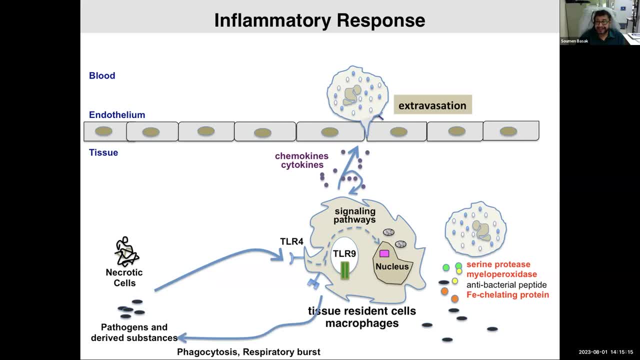 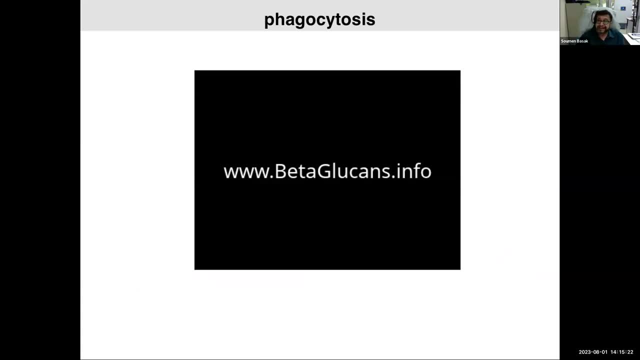 blood cells. staphylococcus aureus bacteria have been added. the small clump of bacteria release a chemo attractant that is sensed by the neutrophil. the neutrophil becomes polarized and starts chasing the bacteria. the bacteria, bounced around by thermal energy, move in a random. 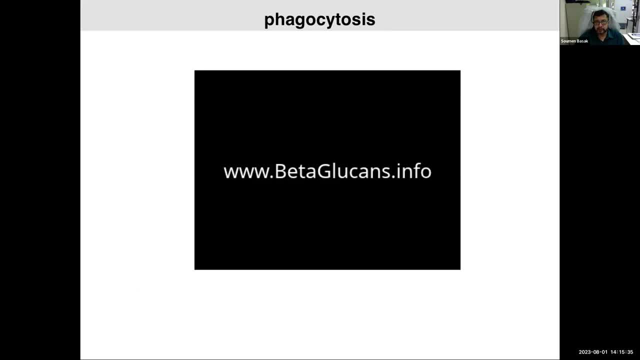 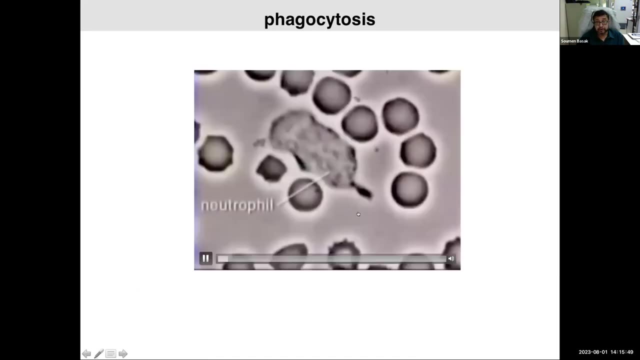 path, seeming to avoid their predator. eventually, the neutrophil catches up with the bacteria and engulfs them by phagocytosis. that was quite a barf, isn't it? so neutrophils are coming at this site of infection because the tissue resident cells? yes, we will take up a question now. 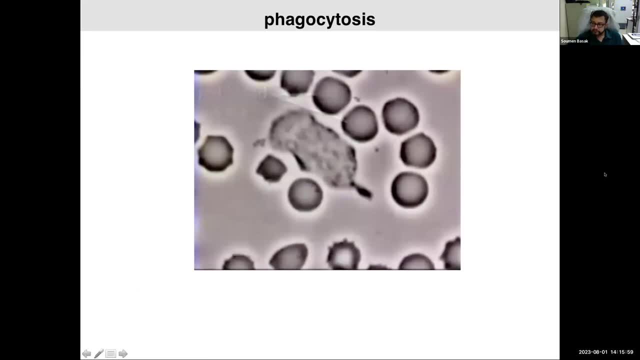 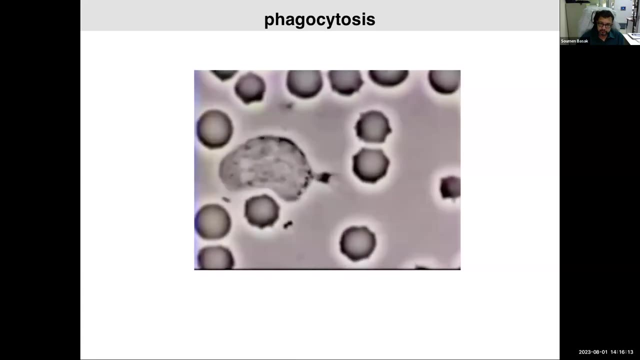 yeah, so i had a quick question. so this engulfing behavior, right? uh, macrophages also tend to do that, right, they also like almost eat up, uh the invader, right? yes, so the point that you're making is true. in fact, neutrophils, the mature mood of their microbial 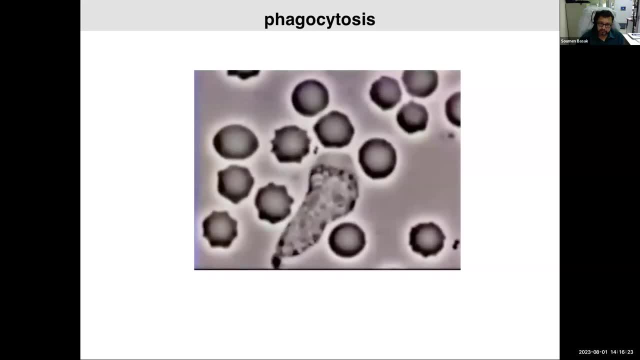 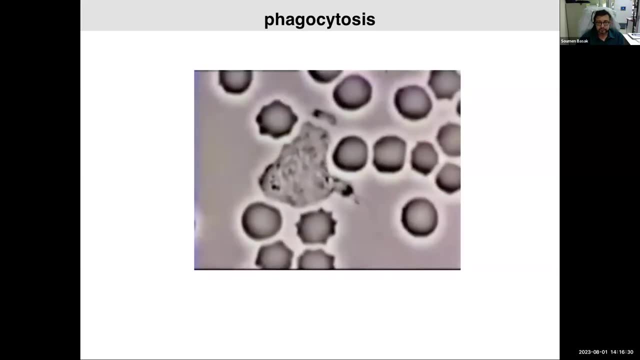 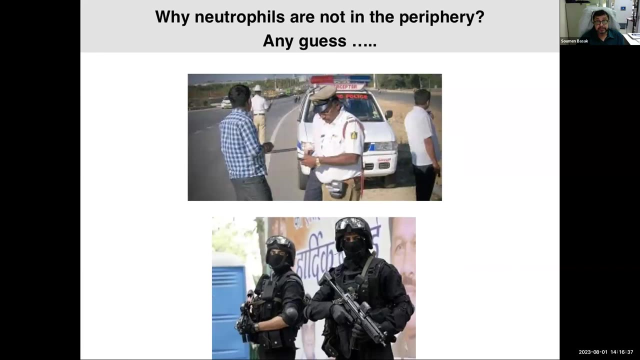 involves those granular proteins, uh, reactive oxygen species, iron chelating proteins, so on and so forth, even ionophores, the secret proteins that would make membrane penetration and disrupt bacteria. actually, phagocytosis is a minor component of neutrophil mediated micro fillings. 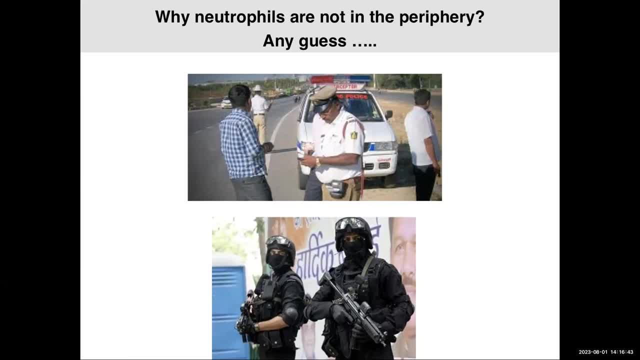 macrophages are indeed more potent in phagocytosis. yes, does that answer your question clearly? yes, sir, yes, sir, thank you. okay, so let's move on to the next one. what is it that we're getting here? is that one question? remember that i was telling you that neutrophils are in the bone marrow. very 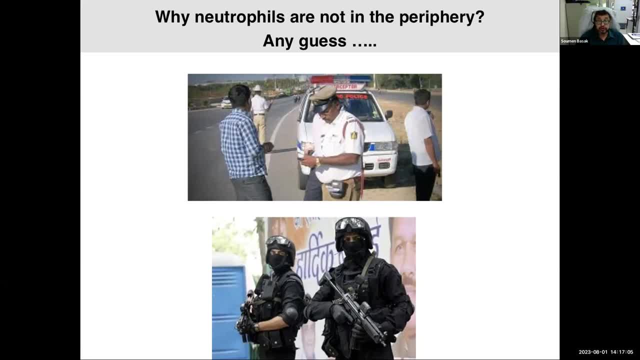 few are in the periphery patrolling the body, and once you got infected tissue resident cells need to call them, uh that please come to the site and kill the bacteria, uh. the question, of course, is a philosophical one, that what is a phagocytosis? 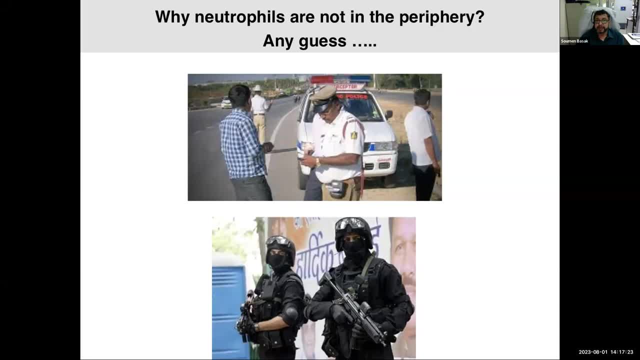 Why they are in the periphery. That is the question, right, Why you have neutrophils- those are so potent- are to be in the periphery, And why are they in the bone marrow and not in the periphery? why? 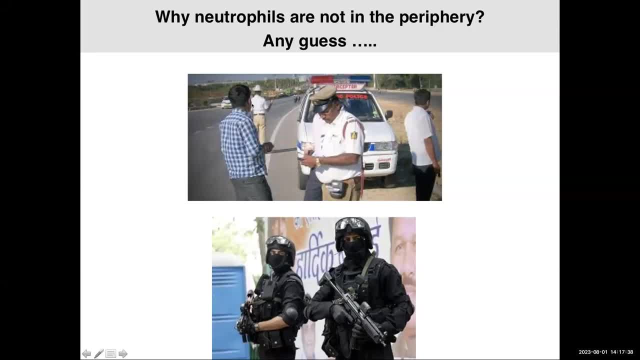 And that, I think, is a cartoon that really clearly makes you understand what goes on in the immune system. is this very striking contrast? Look at this person giving a parking ticket right And then beyond that below it. you see these are our most prestigious black hat commando. 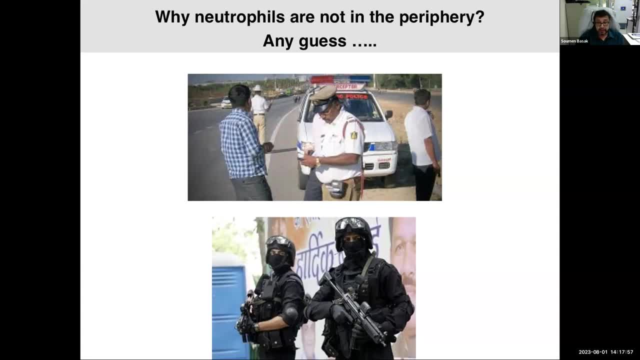 You can one day ask in parking lot: why don't we suit black and commando? Simple reason that is: if you make a mistake in merely parking, they'll shoot in your head. They tend to do that. Neutrophils are killer and small perturbations in the body system they would not recognize. 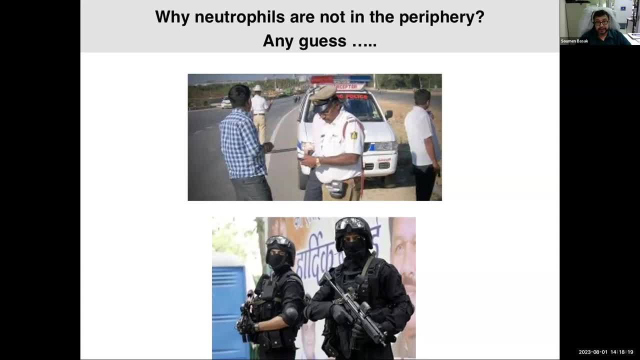 and they would be unrecognized. So you have to be alerted and secrete all those damaging molecules. Those are not only, as I say, innate immunity, those are not only directed to microbes, but they can also cause tissue damage. So one learning is that neutrophils are deadly. 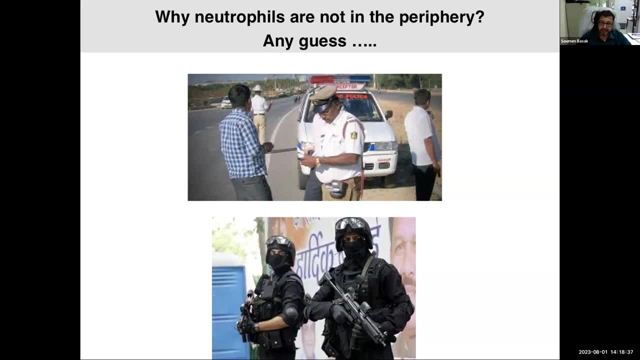 They have to be recruited. We have kept them in the barrack, like we do for black hat commando. unless there is a real emergency, we don't deploy them. And second, that neutrophils do not discriminate when they act. their action might cause harm. 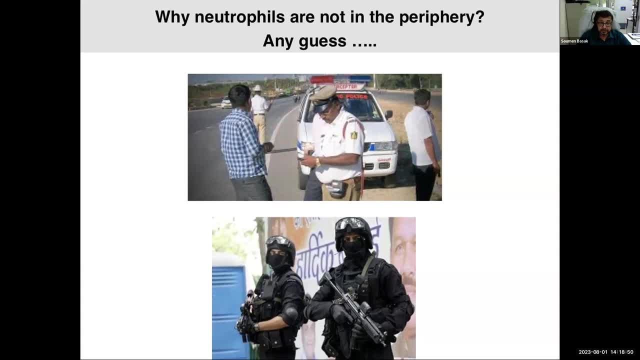 too. So that's a very important point, which will come as to the next part of this. So this is, you see, the response. expression of pro-inflammatory cytokines thereby must be transient, and pathways controlling them must be dynamic. You see that you have a pathway that must go up and then there must be a post induction. 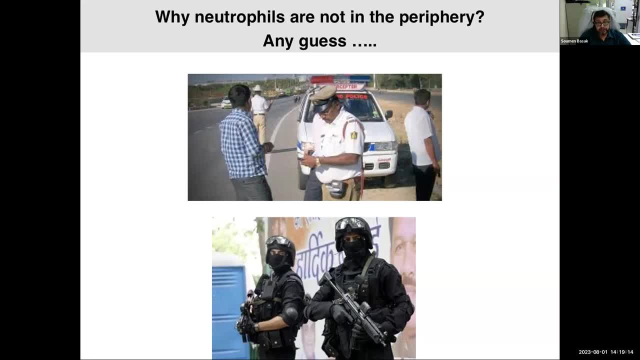 termination of the pathway very controlled. otherwise you will have too many of those pro-inflammatory cytokines. There are too many cytokines and chemokines and too many of the neutrophils coming into the anatomic niche where infection has occurred and this will cause damage to the body. 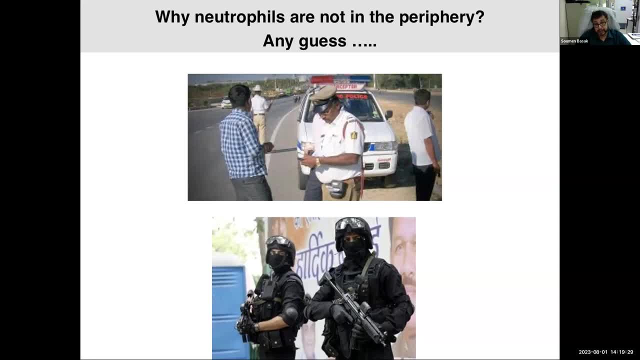 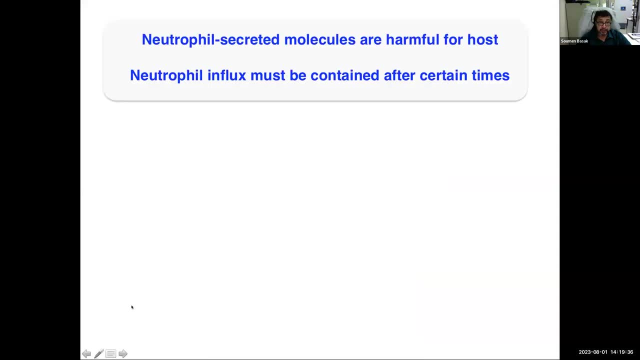 So this is the very basic of bringing back to the computational model. because of this very notion that the very heart of the immune system, there is a requirement that it must evolve better dynamical control. And you know, I don't, I think this is not going to be and this is the signaling pathways. 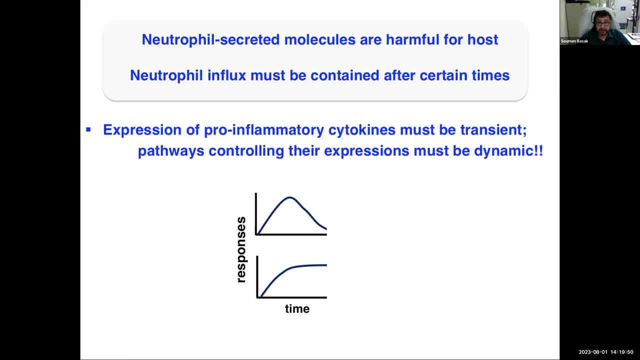 that transmits signal from peripheral receptors that are present in the tissue resident cells to the nucleus, and that signaling pathway must be dynamically controlled, which controls the expression of cytokines and chemokines, And then, obviously, how signals are transduced from pathogen recognition receptor to the 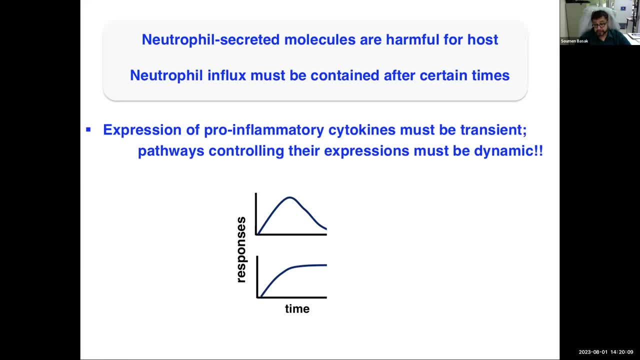 nucleus and how this signaling is dynamically controlled. that's something we will study in a minute. But question is that what exactly we do study in cytokines? I mean, this is of course a general question and a lot of people have studied a lot of. 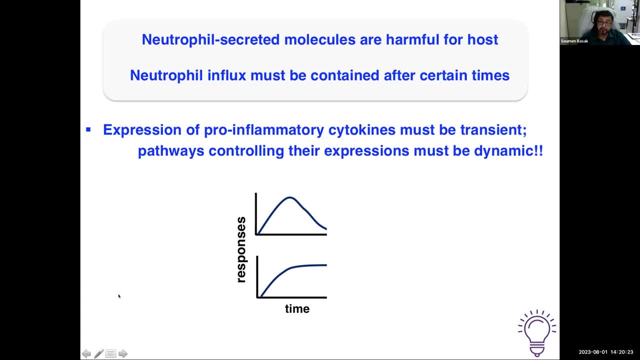 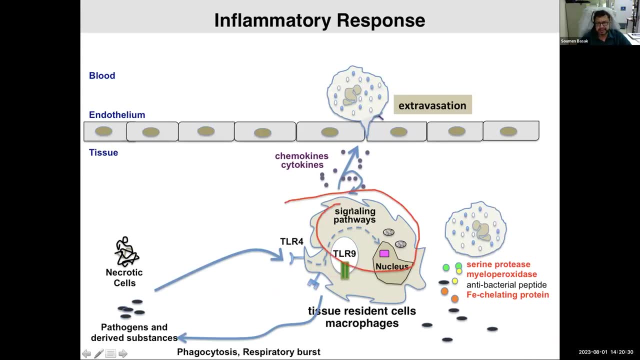 pathways. that actually is involved in regulating expression of chemokines, cytokines, and people have, you know, their own study. they have shown how dynamical control is mediated. Let's see in our laboratory here in the National Institute of Immunology Systems: Immunology. 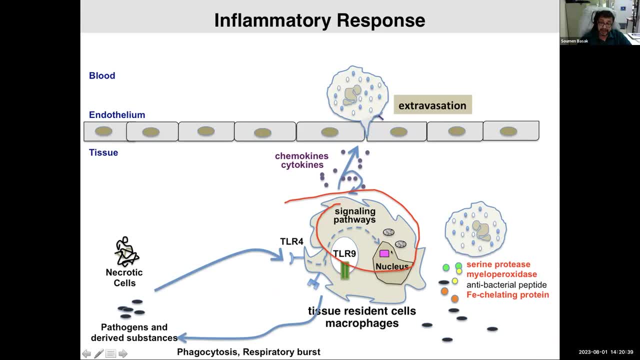 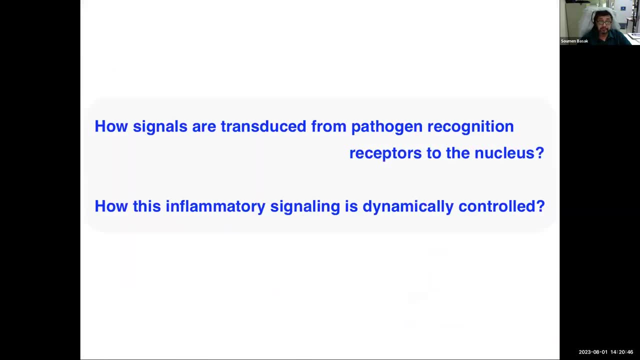 Laboratory SIL. what do we study? So this is the concept that I'm going to. we have been nurturing it for over 10 years, 15 years, I believe, almost, And that's a key thesis, that's a key notion that we have been nurturing to claim a fundamental. 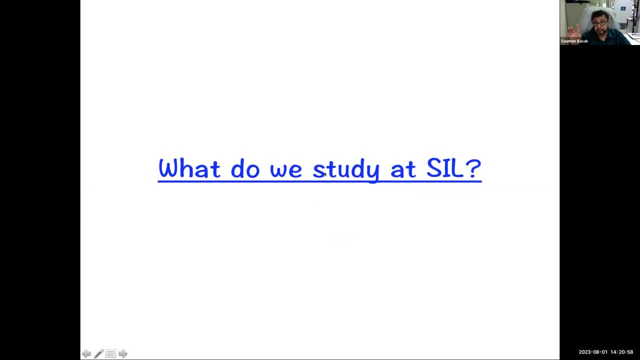 contribution to immunologic research. Now you have signals, right. Pathogen 1 and pathogen 2, one can say: well, pathogen 1, for example, a virus would elicit different gene response than a microbe, let's say bacteria, right. 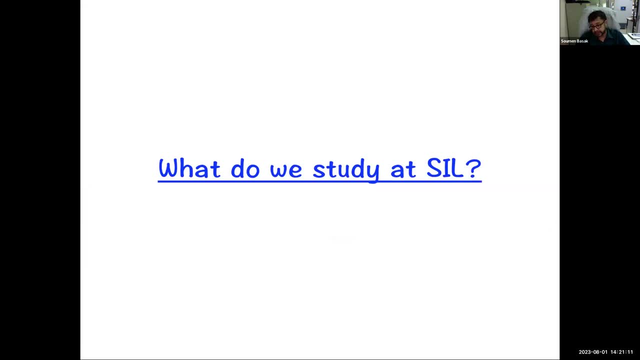 So you can imagine that there is a pathway A for virus and there is a pathway B for bacteria and that leads to response A and response B. We used to once upon a time, maybe many years back, many decades back- we used to think: 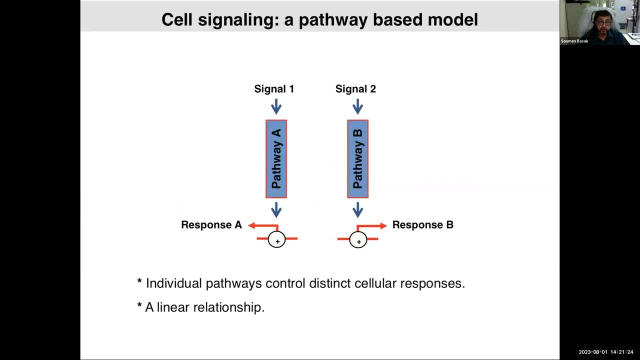 there are individual pathways and that control distinct cellular responses. You know, the problem is there are not that many pathways. You have, as I mentioned, you have hundreds and thousands of different microbes. You don't have that many pathways. And then how do you achieve such an curated response that is curated for individual microbial? 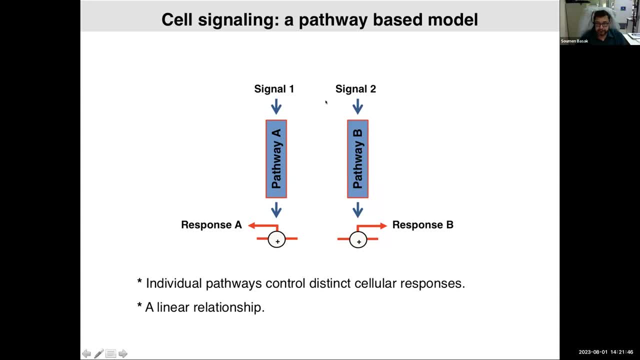 entity. So this individual pathway is centric. It's not just a single pathogen. It's a single pathogen, It's a centric model We can begin to challenge And by last decade I think- 2005 to 10,, the first decade of the century- was a very meaningful 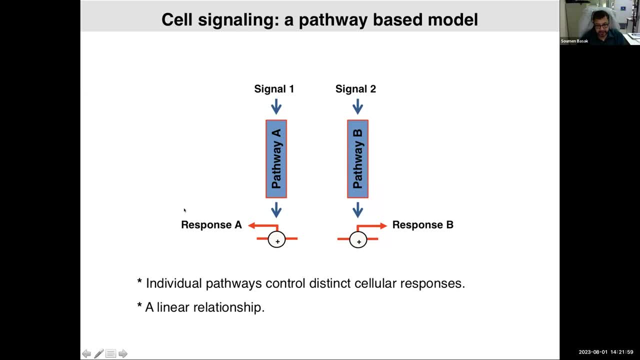 journey. in this People started doing mass spec analysis. They would use a protein and then pull it down and see what else interacts with them by mass spec And you get a huge number of different proteins. You see that pathway A proteins. many of them interacts with the molecules that belong to. 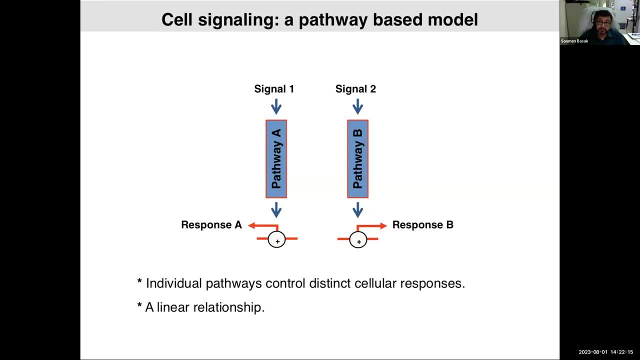 pathway B. That was confusing. You don't see insulated pathways. You don't see those anymore And this sort of experiment. this is one of my favorite papers published in Molecular Cell in 2006.. It's a genome-wide shRNA. 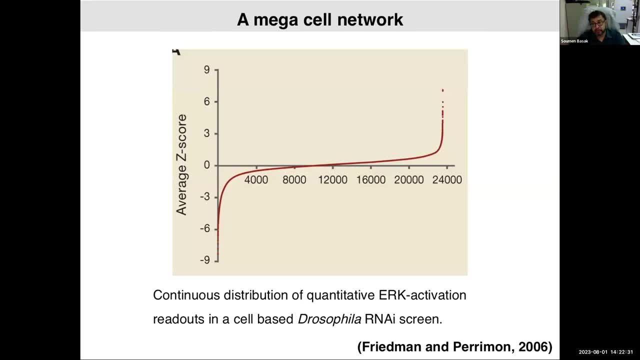 So you have begun to learn how to do small hairpin RNA mediated gene knockdown. Once you learn, you begin to make a library for the entire genome, And this is one experiment where they are actually in the x-axis what you have? One or the other gene of the drosophila genome that has been subjected to knockdown. 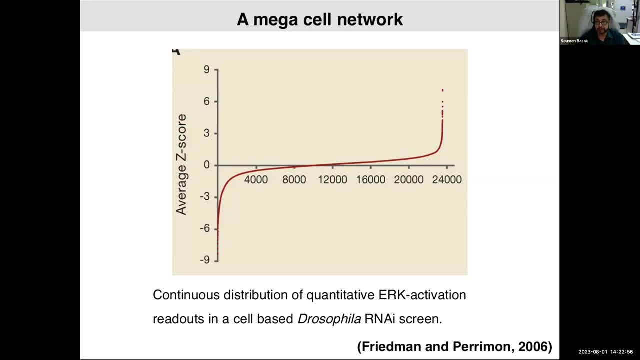 Around 24,000 entities could be found in the x-axis And y-axis. what you measure is activity of map kinase, ERK. in case right, There are three map kinases. This is the ERK. You measure average G-score. 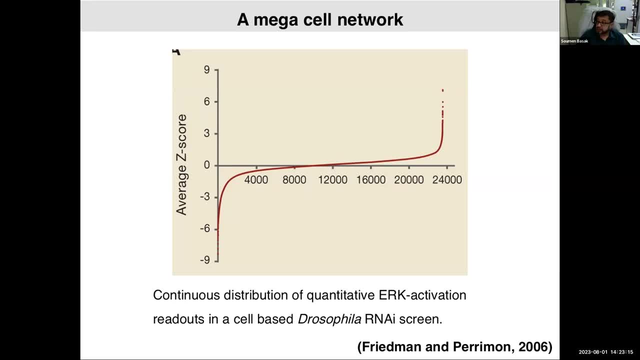 To simplify it to my audience: if G-score is zero, that is zero. That is zero, That is zero. The shRNA did not impact map kinase activity upon knockdown of the target gene And a non-zero value means this has substantial impact right. 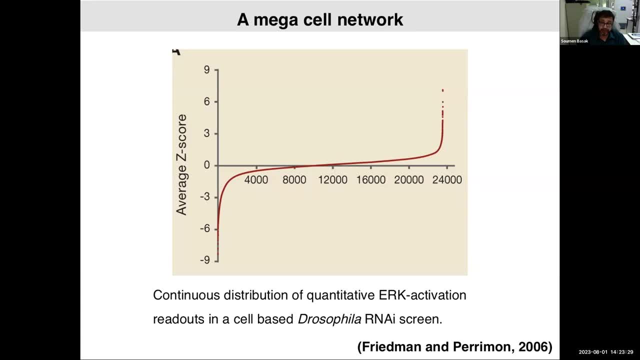 I mean if the knockdown led to increase in the G-score, that means that this particular gene must be inhibitor of map kinase And if the knockdown led to decrease in the G-score, those might be stimulator of the map kinase activity. 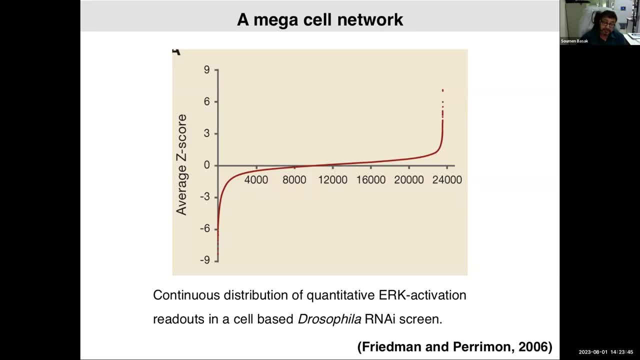 And I see this is the extreme left of the graph and the extreme right of the graph. They look pretty familiar, these molecules, these genes people later identified. they are all known, non-regulated, of map kinases. What is astonishing, though, that is a continuum of this line. 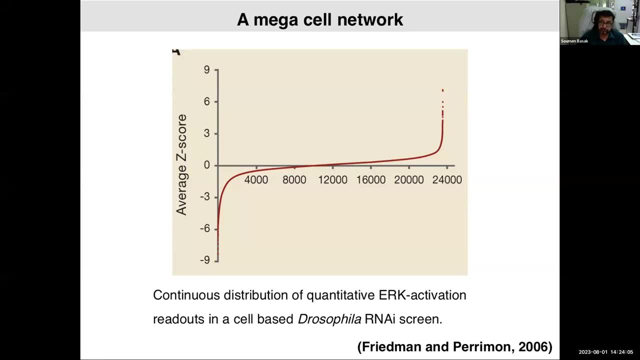 And it was later reproduced with many such shRNA skin. This is actually a typical what you get in a shRNA skin, for, whatever you measure, What does it say? It's very interesting That every gene in the drosophila genome may have a non-zero contribution to map kinase. 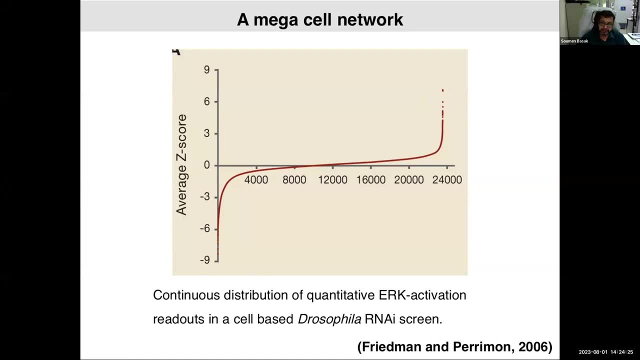 activity And that's very different that those A and B, two pathways doing things for us. It appears that in their genome is expressed and forming a network and controlling a particular phenotype, in this case map kinase. So sooner or later we began to have these depictions that there are multiple pathways. 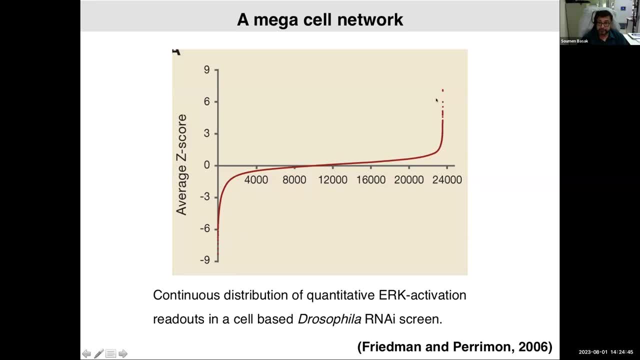 they're interconnected, Sometimes they share molecules, Sometimes they don't. Sometimes they're connected to feedback loops, meaning one pathway is making some protein that actually is acting another path- Sometimes there is feedback, negative feedback regulation, And sometimes there are simply as simple as a functional connectivity which is not physical. 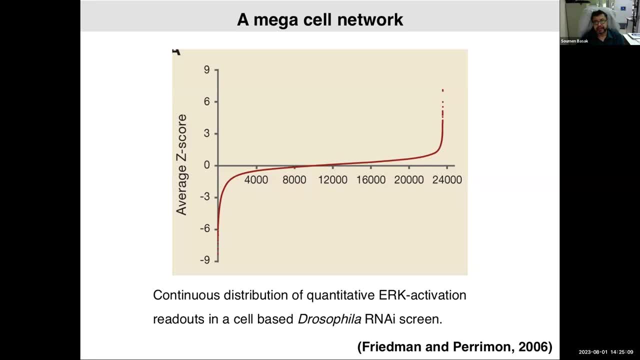 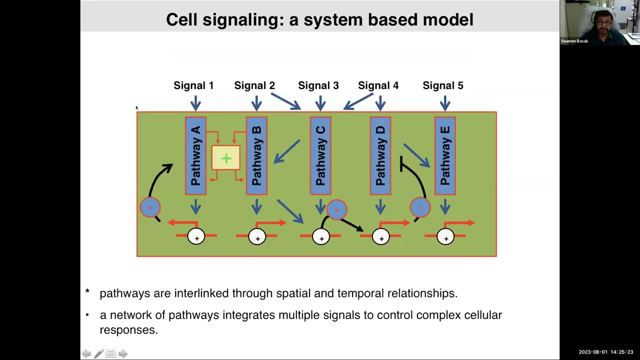 in nature, but we know that there is a connectivity. So we slowly realize that pathways are interlinked to spatial and temporal relationships and it's not a single pathway or network of pathways which integrates multiple signals and that is responsible in complex cellular responses. 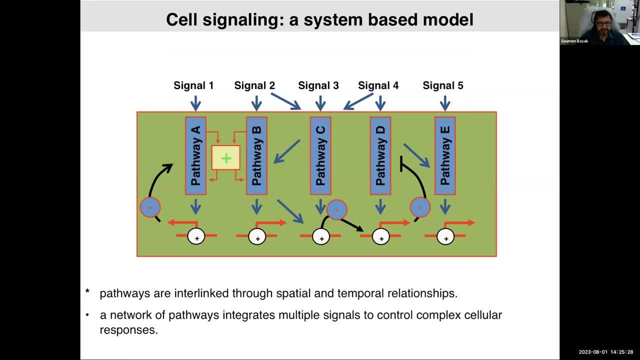 And from then onward we began to see the system biology. Of course, the term came up and we began to see there are two components of the system biology. I'm going to keep this again. One is omics-based system biology. 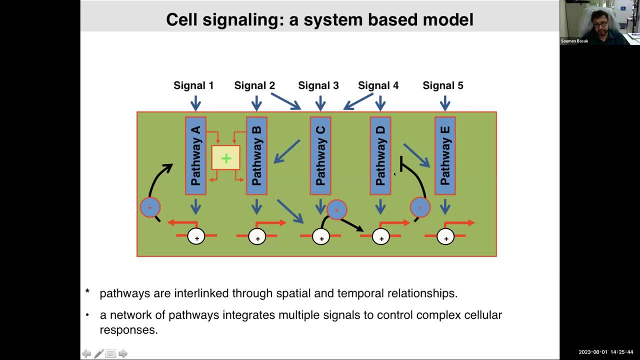 You have heard of it: transcriptomics. I'll talk just two slides today on transcriptomics, Thank you. genomics: This is called top-down system biology. You, of course, understand the same thing in system biology: It's a network of pathways. What you do? you take genome-wide readout. 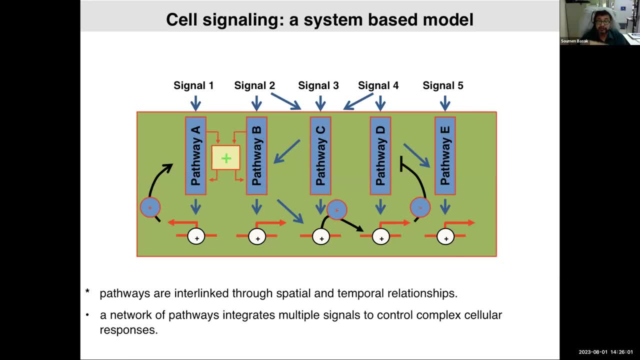 and from there you, you know, put forward a hypothesis about the network, how it might be working, And another one started working at the same time, the end of the last decade or middle of the last first decade of the century, the bottom-up system, biology that began to get.